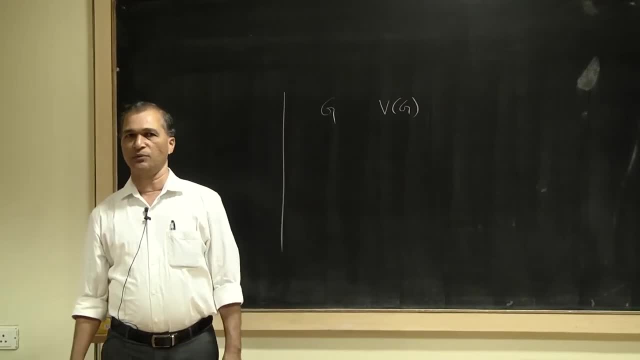 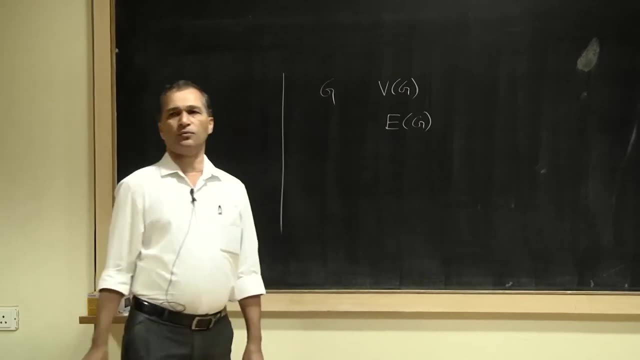 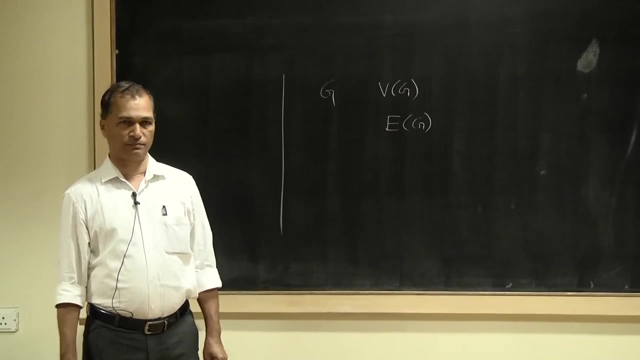 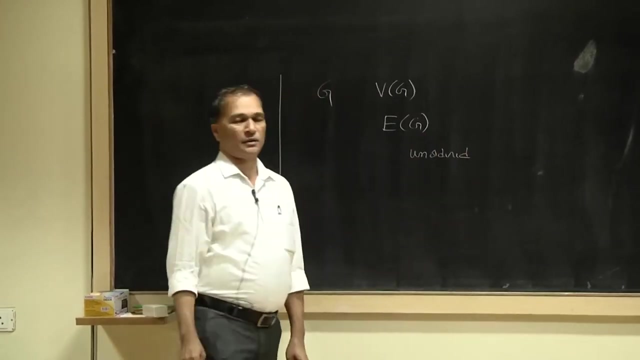 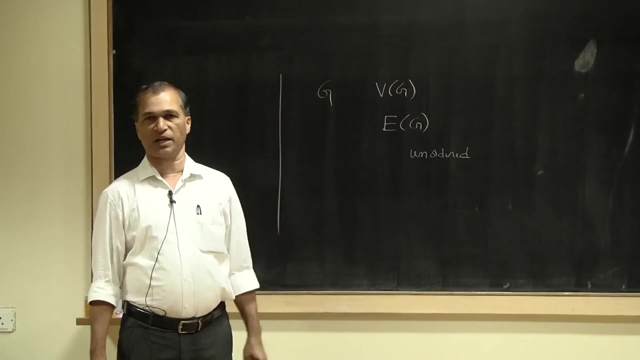 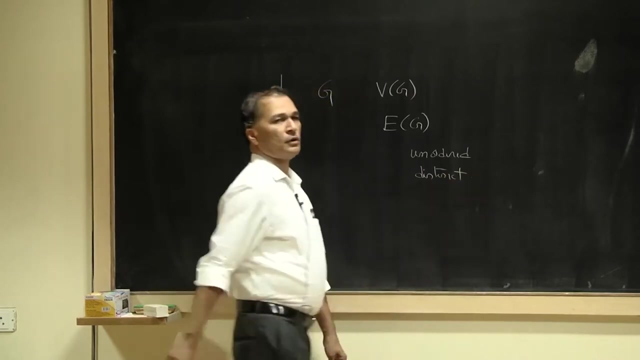 is called the vertex set, elements of which are called vertices, and a set E of G of unordered pairs of distinct elements of the vertex set. I repeat, it is unordered, which makes the graph a non-directed graph. If we take the directed ordered pair, it becomes a directed graph and distinct elements which 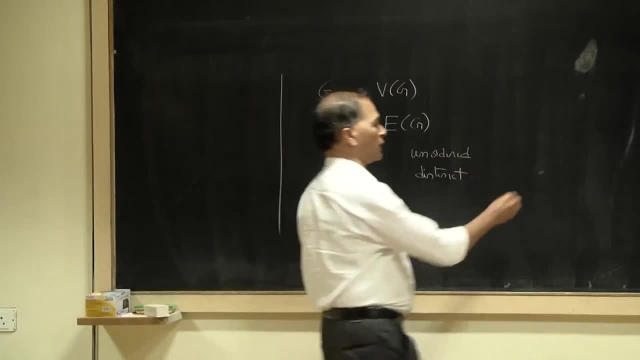 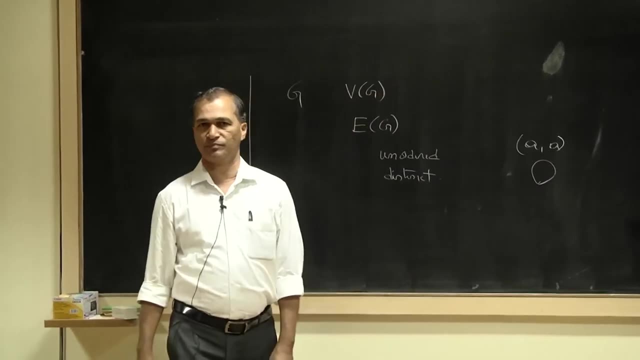 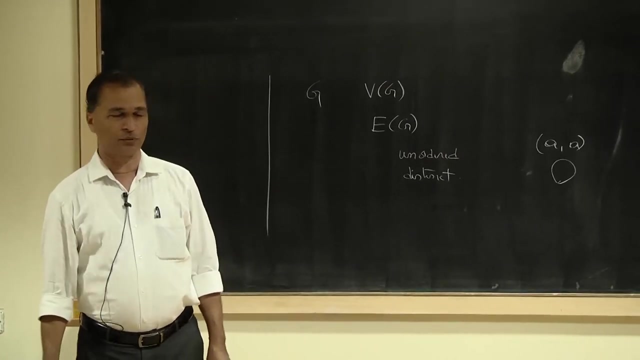 says that the loop is not included. If we take the unordered pair A- A, there will be a loop from A to A. this is excluded and it is a set. If A- B is an element of the set, A B cannot be repeated. 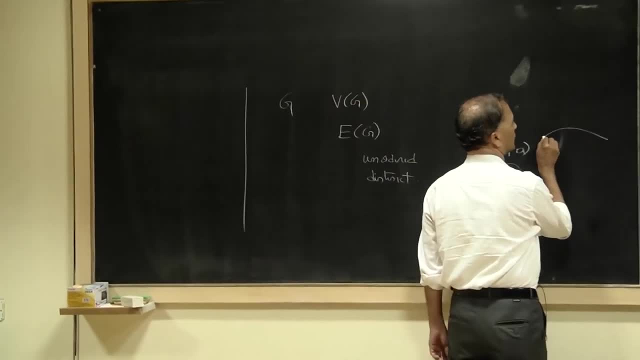 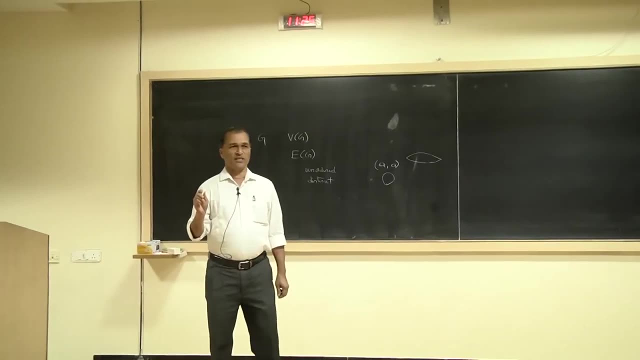 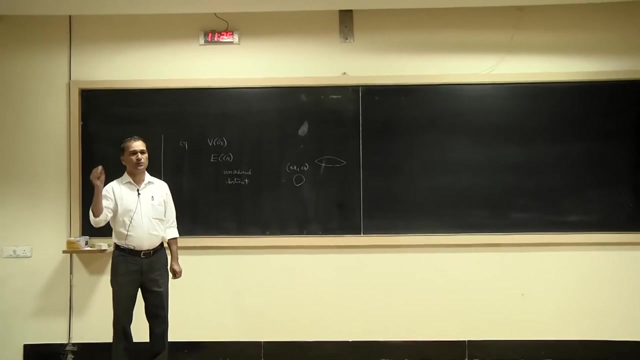 So if there is an edge from A to A, it is not included. If there is an edge from A to B, we cannot have another edge from A to B, So parallel edges are removed. So we consider only the graphs which are called the simple graphs, which do not have self loops, which 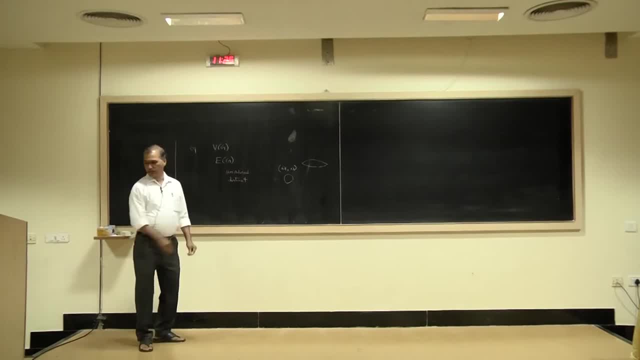 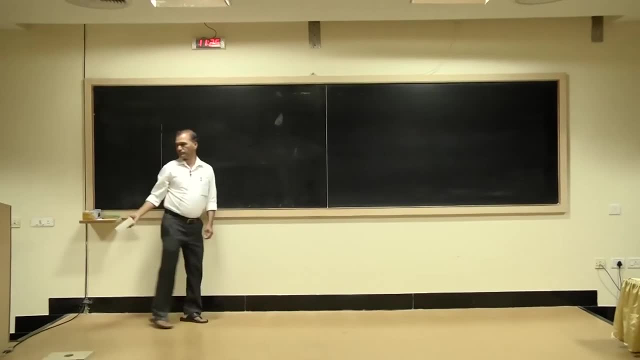 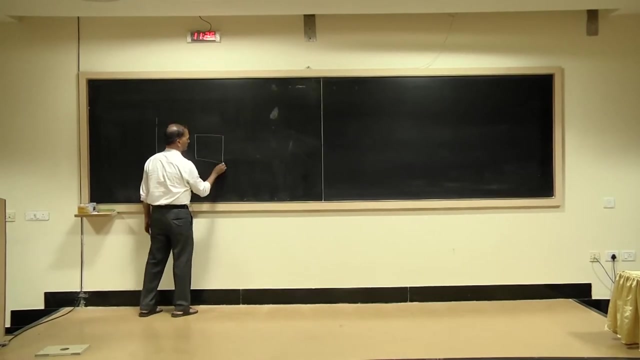 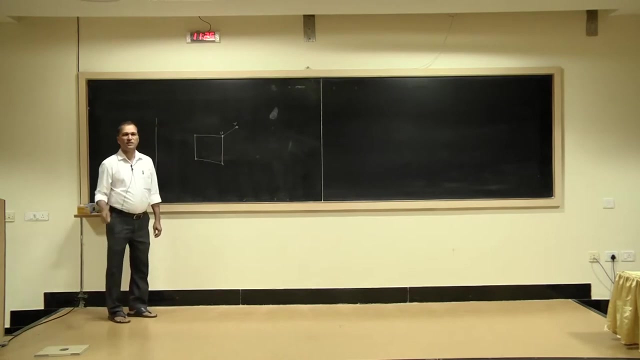 do not have parallel edges, So the graph considered are simple graphs, Thank you. For example, these are vertices and these are edges. This is an example for a graph. We say that these two vertices, U and V, are adjacent in the sense that there is an edge between. 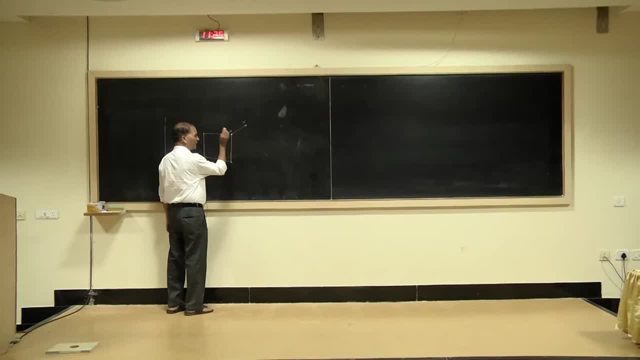 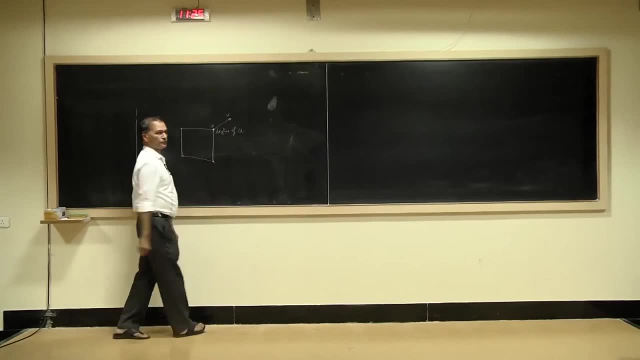 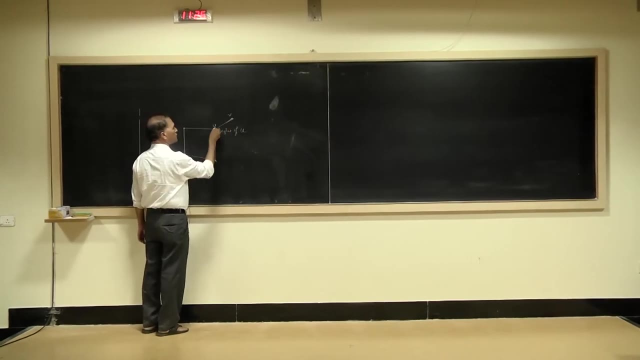 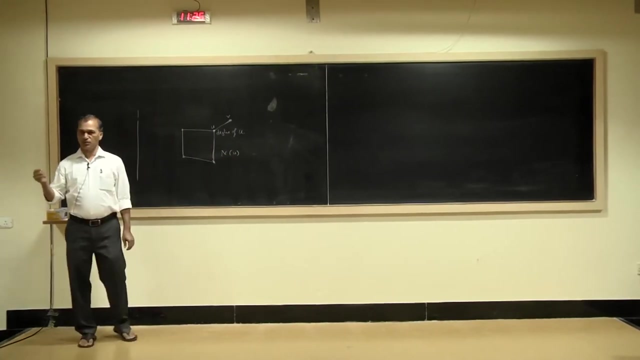 them and number of vertices which is adjacent to the given vertex is called sqrt. So sqrt called degree of u. We can define neighborhood of the vertex u. It is all the vertices which are adjacent to the vertex u. We define n of u to be the set of all vertices which are: 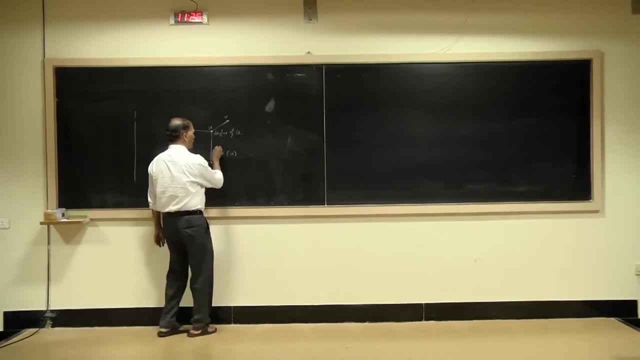 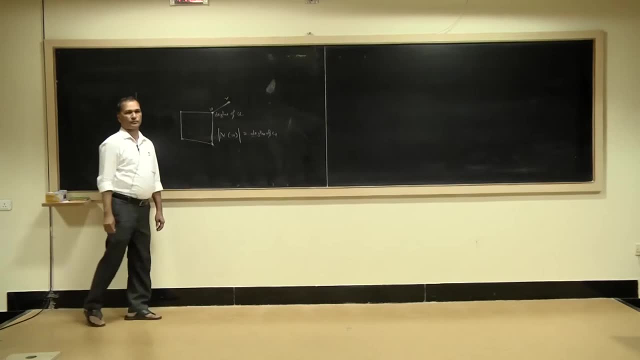 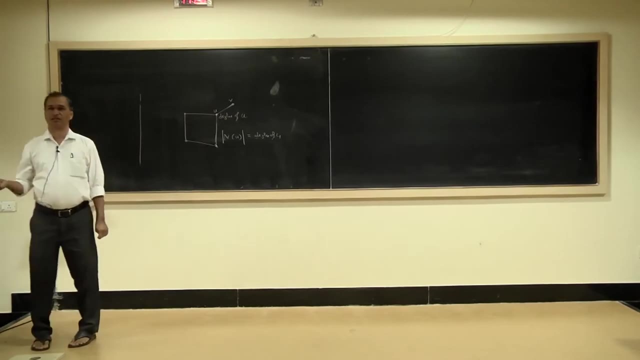 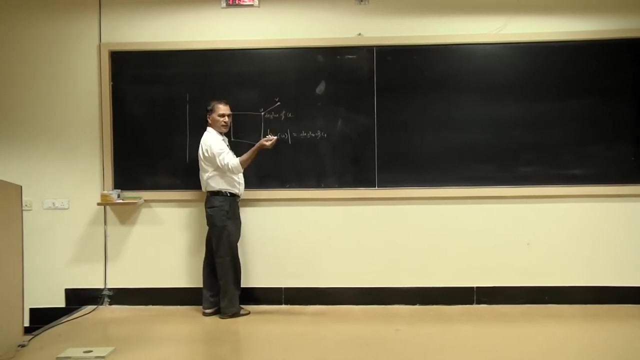 adjacent to the vertex u right, And number of elements in n of u is nothing but degree of u right. It is very simple to observe that sum of the degrees is always even right, Because every edge contributes degree 2 to the total degree, one at this vertex and one. 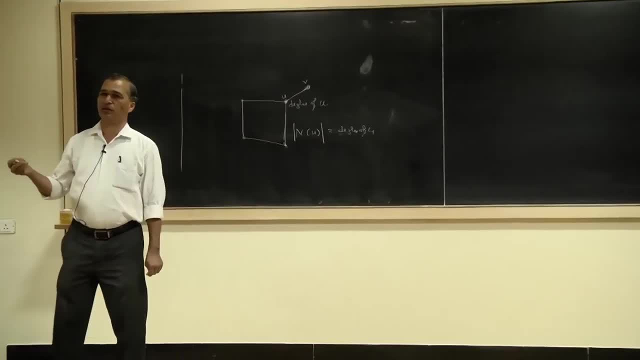 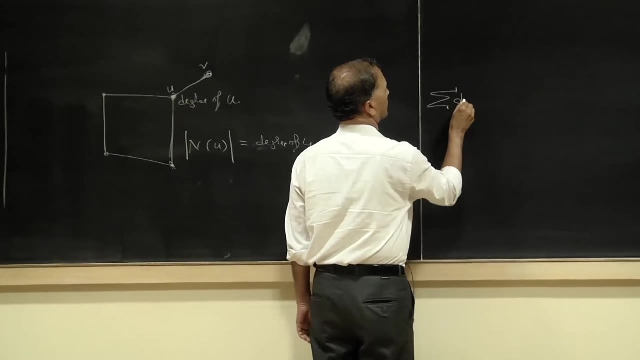 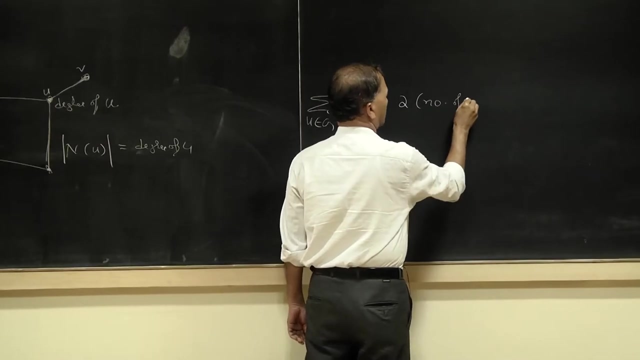 at this vertex. Therefore it is always even and it is equal to twice the number of edges. right Sigma degree u is equal to n of u, u belongs to g, if we say is equal to 2 times number of edges, And we usually say that number. 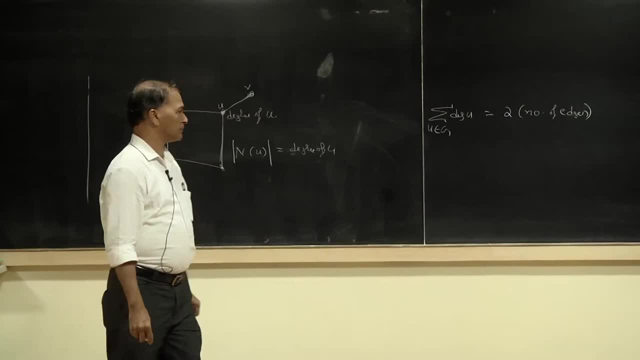 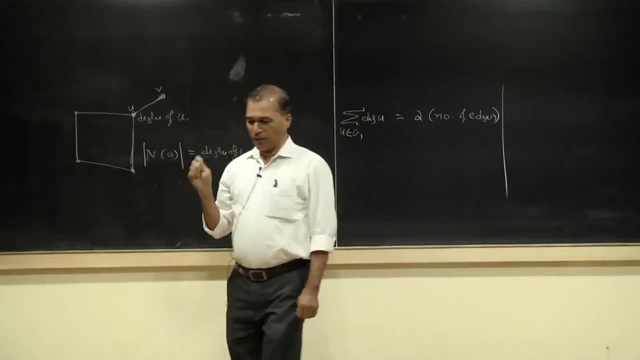 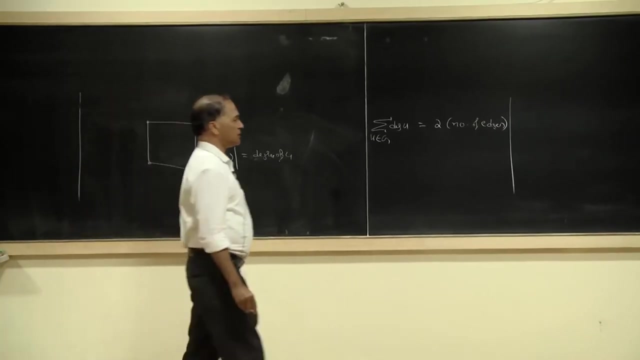 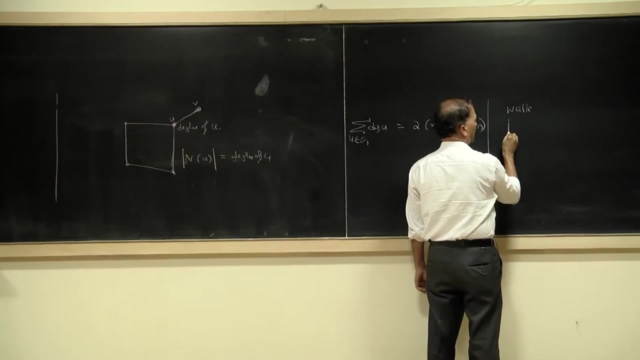 of vertices is n and number of edges is m. right, And one of the most important concepts in graph theory is that of distance between two vertices. To define the distance between two vertices, we define a walk in a graph and a path in a graph. A walk is a sequence. 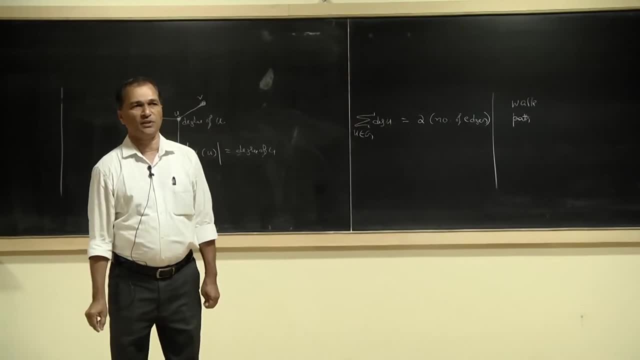 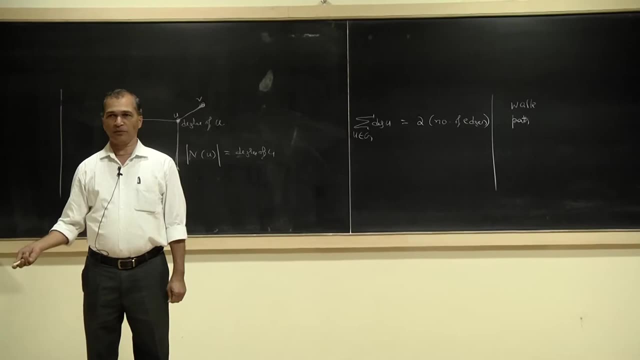 of vertices and edges starting with a vertex and ending with a vertex right. There is no restriction. Vertices may repeat, Edges may repeat right. Number of occurrences of edges in a walk is called length of the vertex. The distance between two vertices is length. 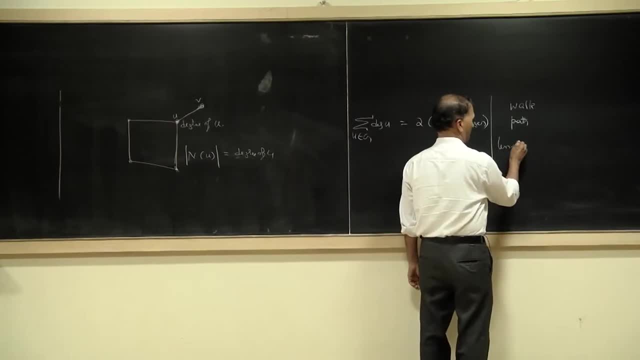 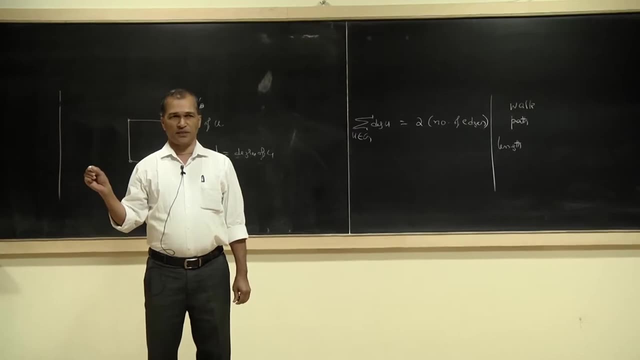 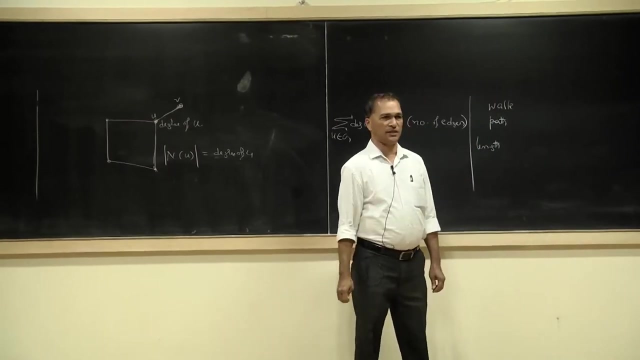 of the vertex right. The length of the vertex between two vertices is called length of the length of the walk, number of edges in a walk. If in a walk all the vertices are distinct, we say that it is a path. a path is a walk in which all the vertices are distinct. Now 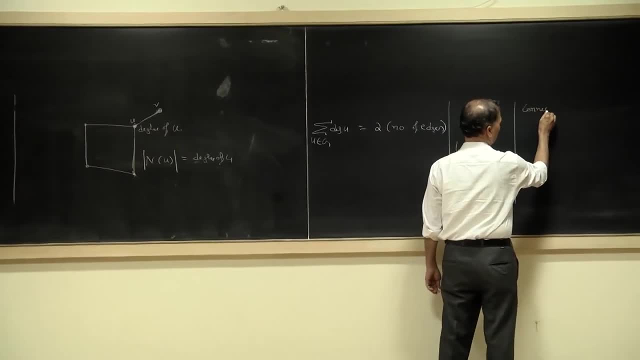 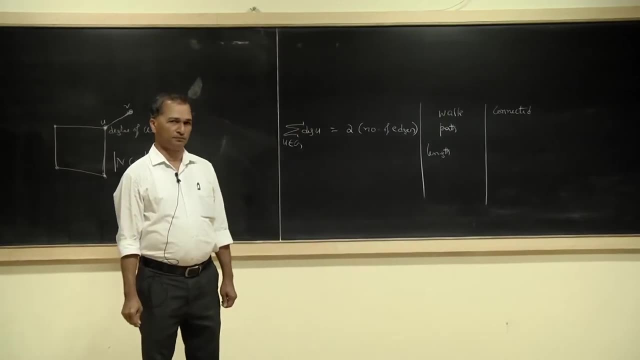 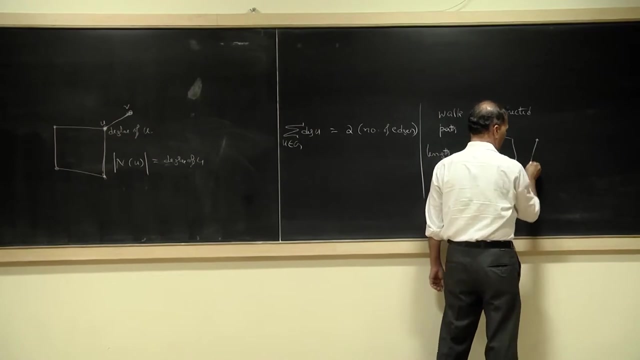 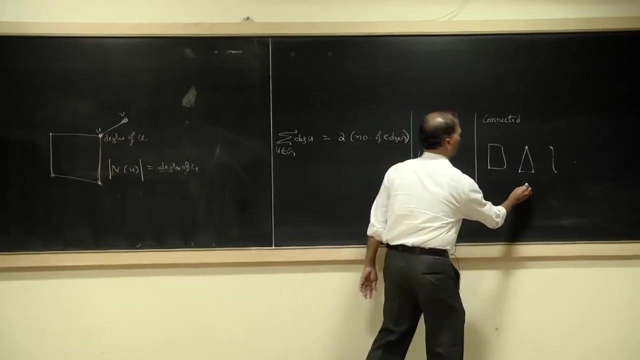 we say that a graph is a connected graph if between every two vertices there exists a path. If you take this graph, for example, maybe this also If you take the entire thing as a graph, this is a part of the graph, this is another. 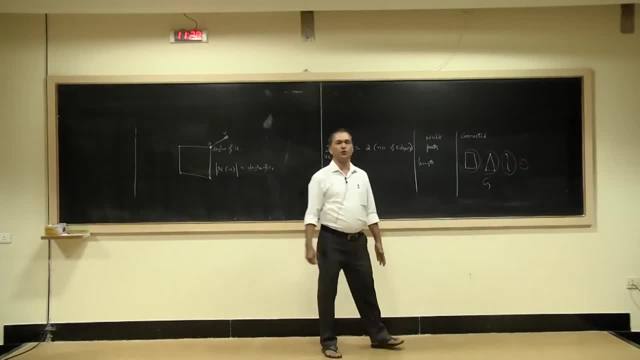 part. this is third one Grape, common root수가 E of 1 by 2.. And here it is a step, the stopping point, and Y is the starting point, Etcетc. this is the fourth part. with the usual sense, This part of the graph is connected because 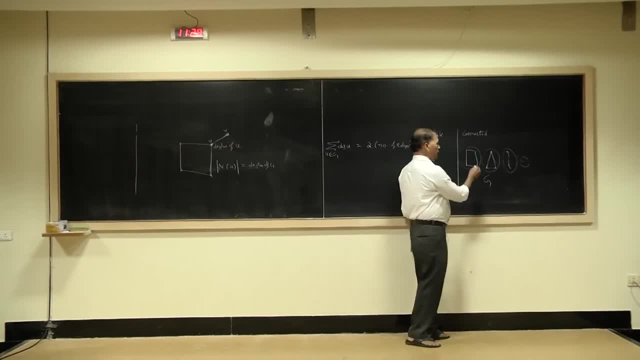 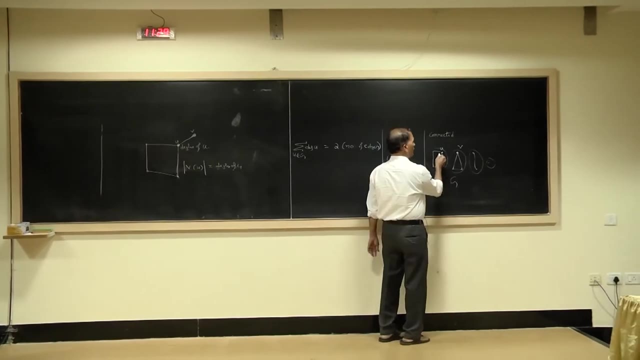 between every two vertices there is a path, But if we consider this vertex u and this vertex v, there is no path between u and v. Therefore, the entire graph is not connected. It is called a disconnected graph, right, And this part of the graph is connected. and if you include v to this, 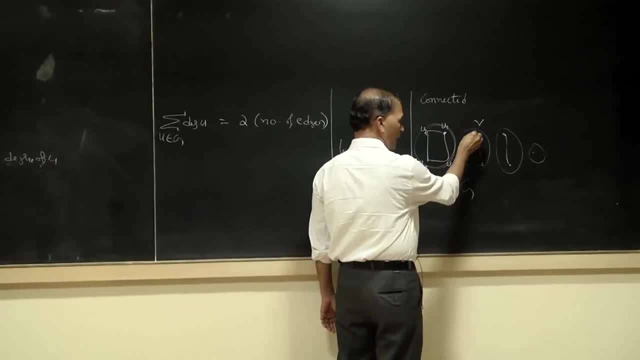 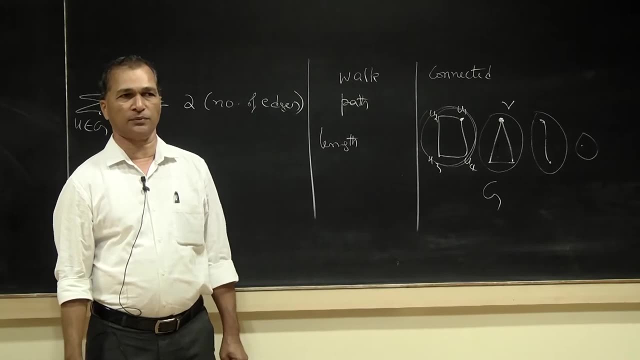 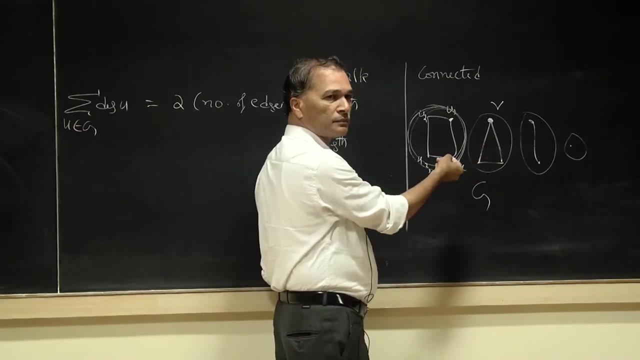 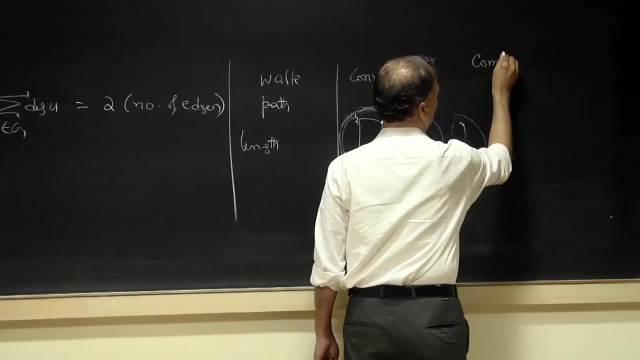 one say u1, u2, u3, u4, include v to this one, then the graph ceases to be connected, It becomes a disconnected graph. So it is a maximal connected graph. If we include one more vertex, it becomes disconnected, The maximal connected part. this is called a component or it is called a connected. 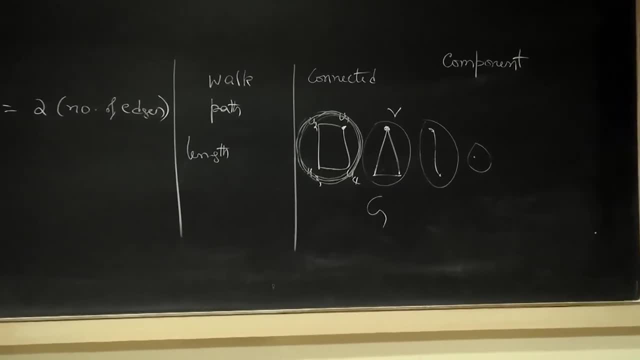 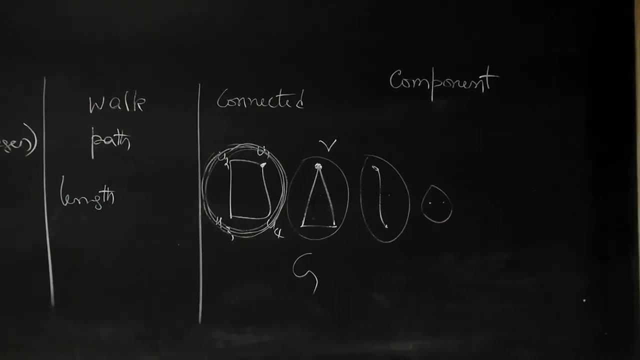 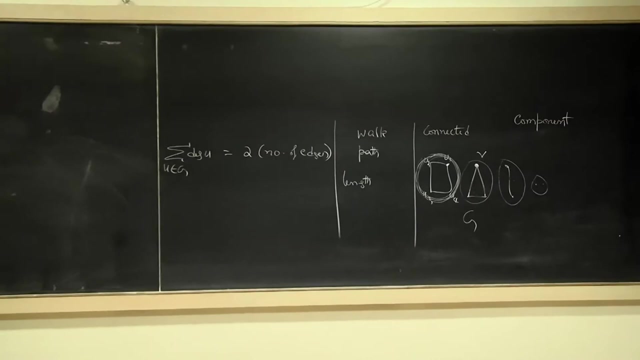 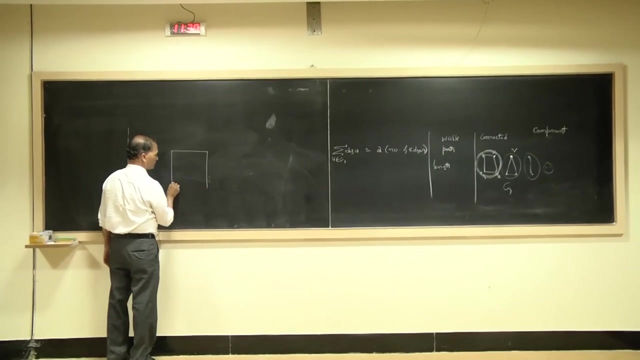 component. What is the momentum of the graph? There are four connected components, four components: One is this component, this one, this one and this one right? If you consider a graph, we can think of that graph in which every two vertices are connected, And if we include v to this one, say u1, u3, u4, include v to. 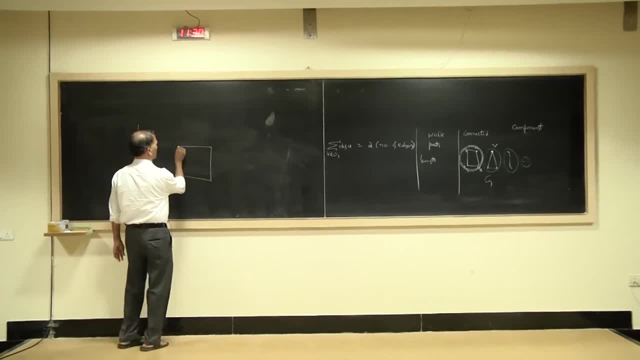 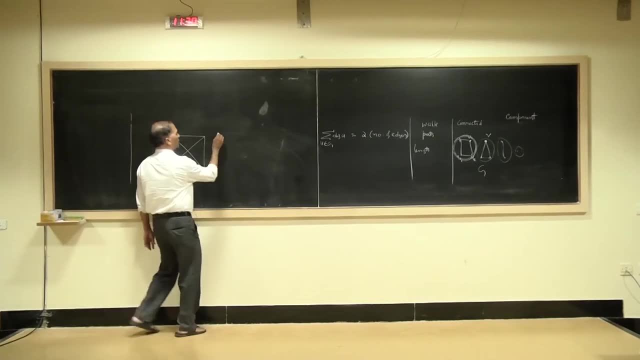 it. If we include v to this one, say u1, u3, u4, include v to this one and this one, and this one and this one vertices are adjacent. For example, if you consider this graph, it is a graph in which every two vertices are adjacent and such a graph is called a complete graph. Now, in this, 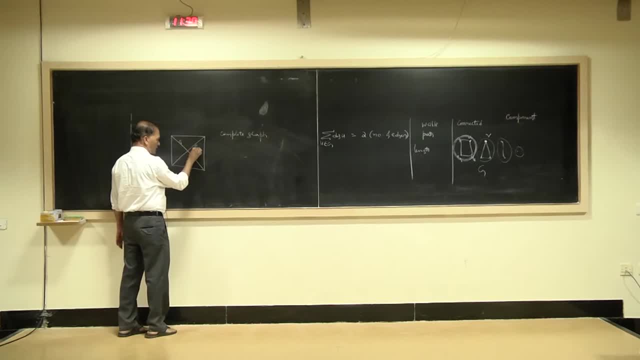 complete graph if you consider this G1 and this is E2, this E1, E2 itself is a graph, which is called a subgraph of the graph, A subgraph. if G is a graph, H is called a subgraph of the graph. if vertex set of H is contained, H should be a graph. a graph, H is called a. 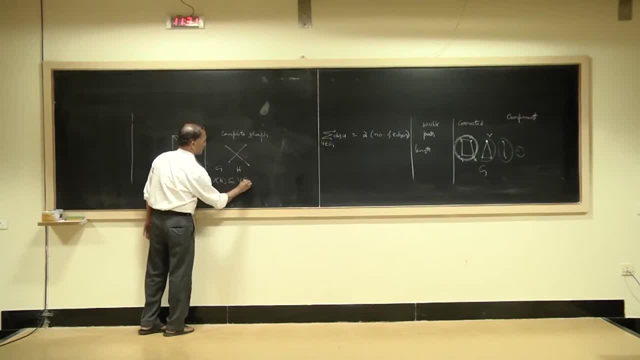 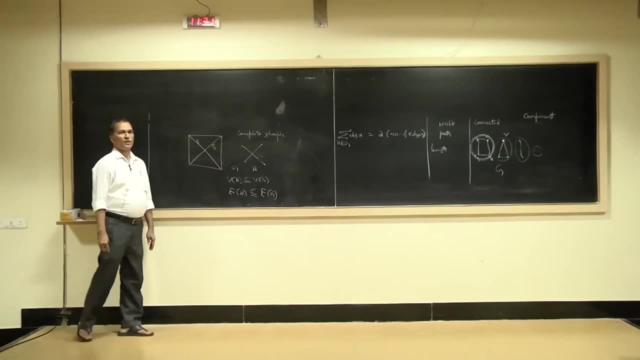 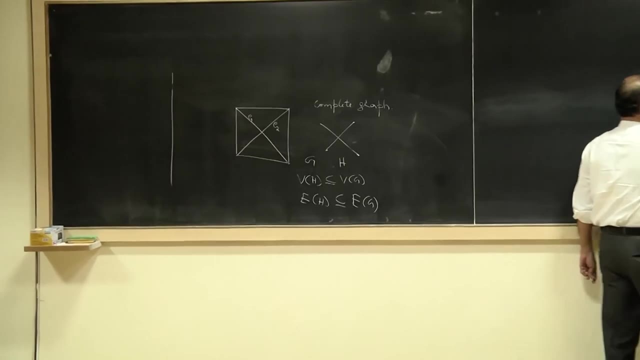 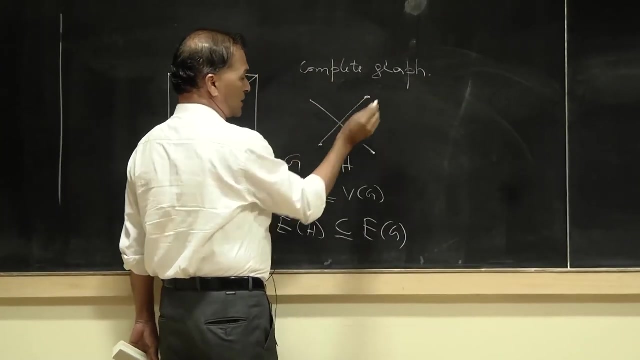 subgraph of G. If V of H is contained in V of G and E of H is contained in E of G, the vertex set is a subset of the vertex set of the graph G and the edge set is the subset of the edge set. This subgraph, for example, it consists of all the vertices of this graph. There are: 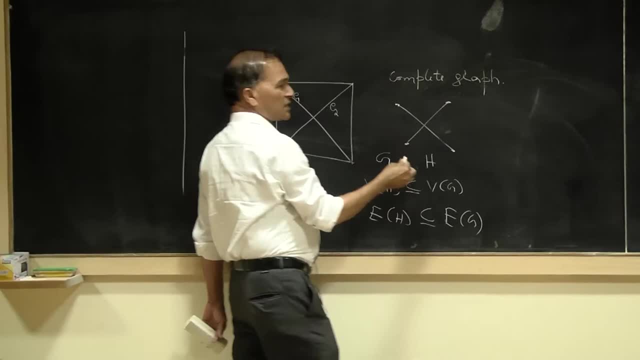 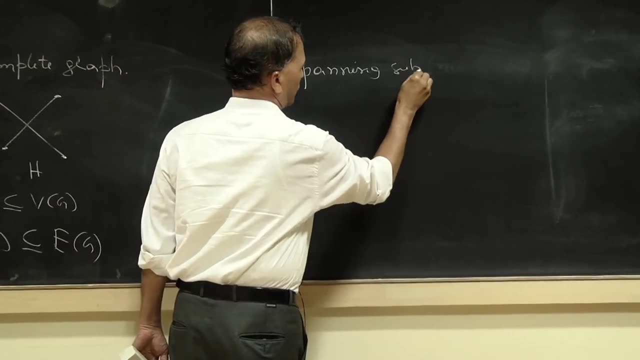 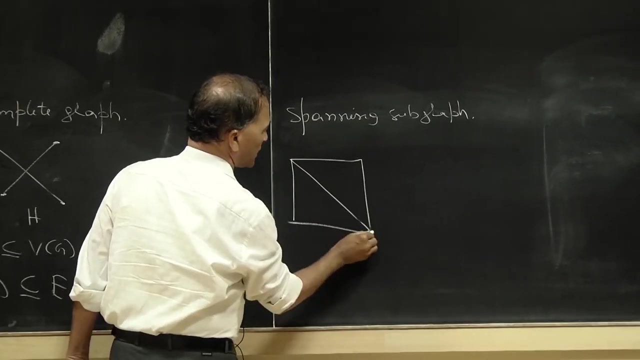 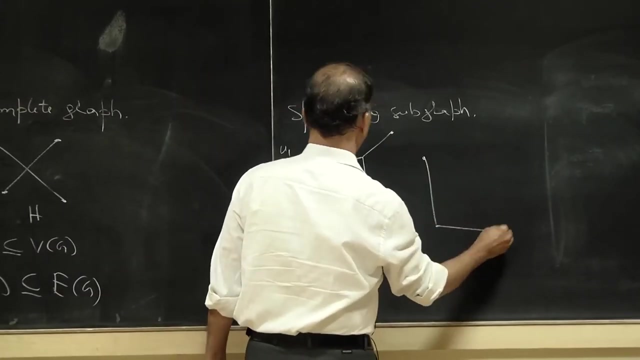 four vertices here, all the four vertices. So these are included in subgraph. Such a subgraph is called a spanning subgraph. If we consider this graph, if we take this as U 1,, U 2,, U 3,, if we consider this U 1,. U 2, U 3 as H. this is G. H is a subgraph of J. this is for H, very simple one, as we know now that that we have to write G because the vertex set will be G as G in subgraph. So we have typically a behavior of H explorer in this particular situation, that if the vertex is declared in enoughopposites and we have added numbers, then theuc entsprechance will be greater. Now we have to take a proportion of those effects because each graph will be. 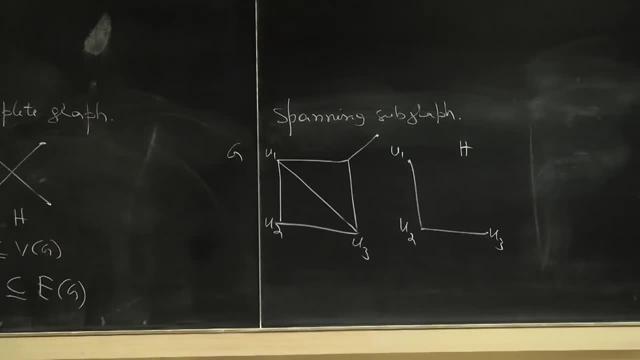 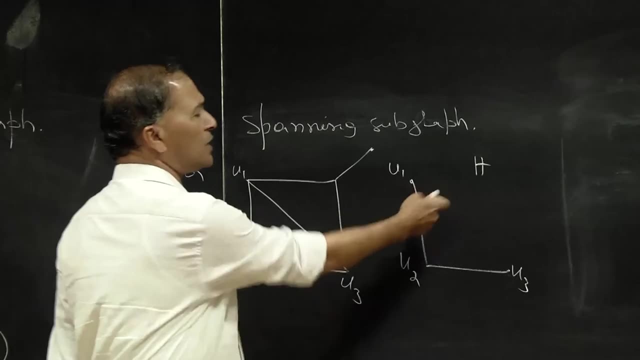 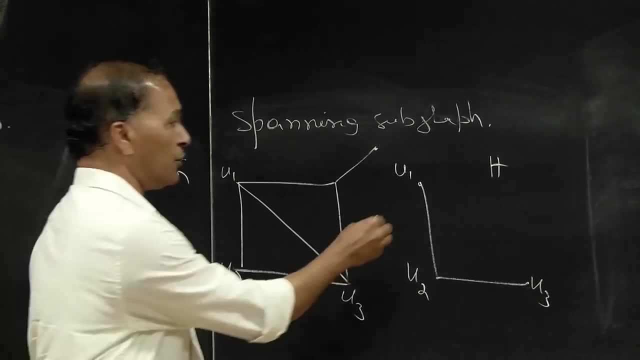 certainly variegated and we are going to convert them to vertical up niż. So this is the g, but h is a subgraph where the edge u1, u3, which is an edge in g, is not there in h, right, In that sense it is not a maximal subgraph of g with the vertices u1, u2, u3,. 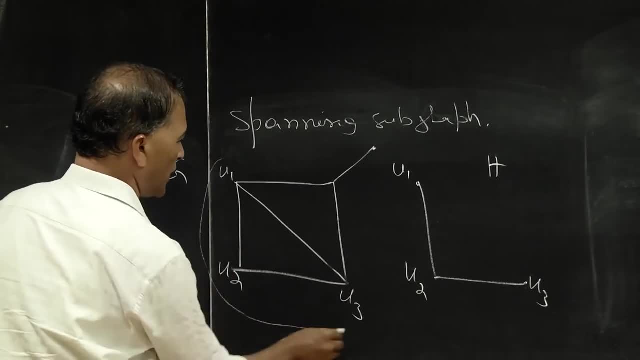 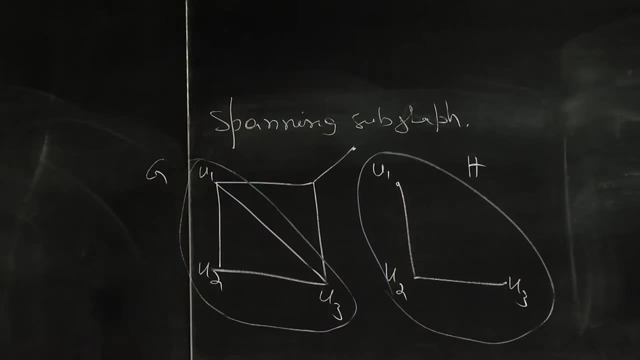 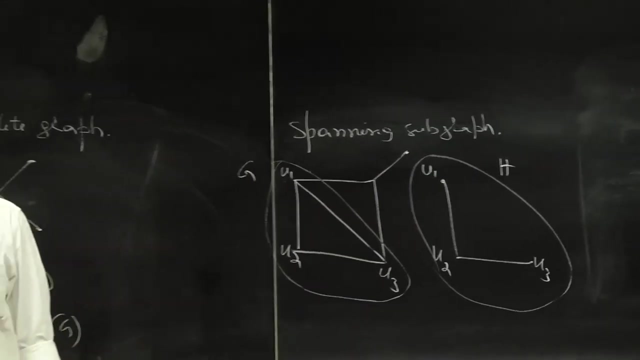 right. If we take the set u1, u2, u3 and if we consider this subgraph in the sense that it does not contain the edge u1, u3,, it is not a maximal subgraph of g. So what is a maximal subgraph? 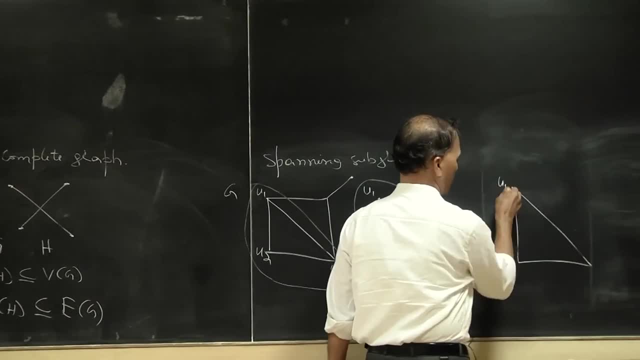 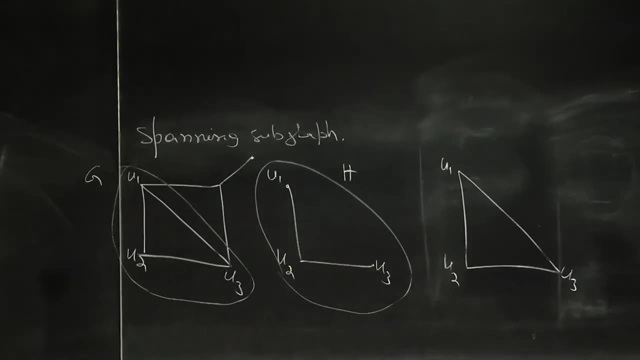 If you want the maximal subgraph, this should be the maximal subgraph u1, u2, u3.. So this is the maximal subgraph with u1,, u2, u3 as this vertex set. Such a maximal subgraph is called induced subgraph. 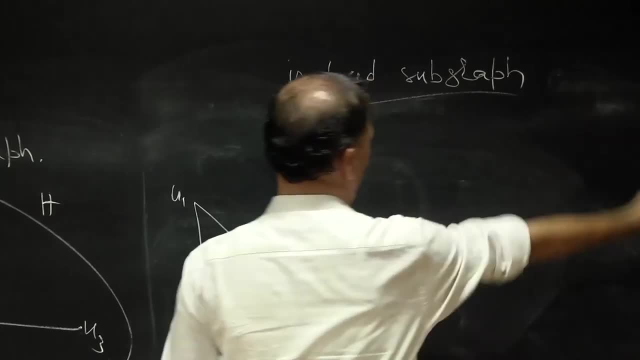 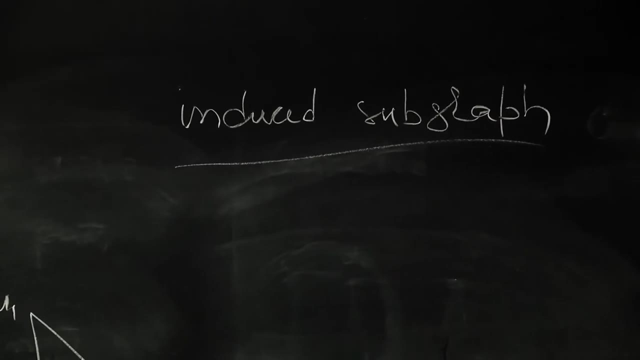 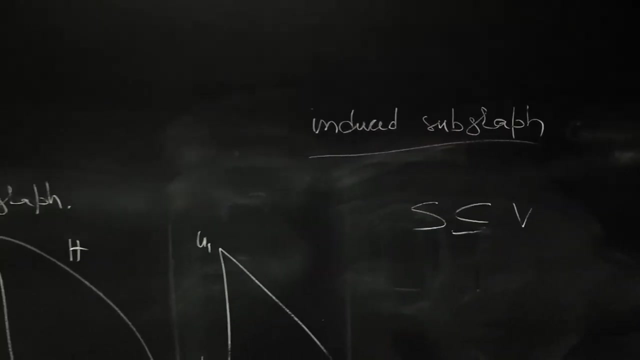 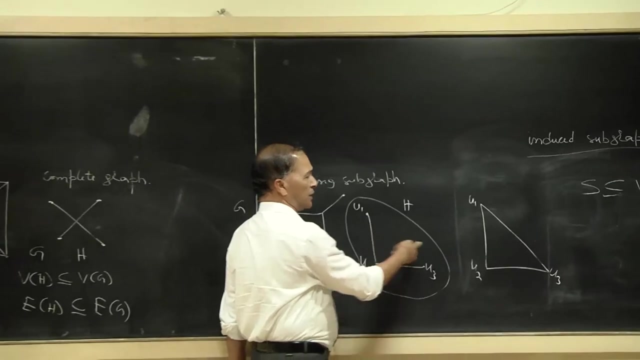 It is a very important concept. induced subgraph. A induced subgraph of a graph induced by the set S of v is the maximal subgraph of g, with S as the vertex set. This is not the induced subgraph. it is a subgraph which is not induced. This is 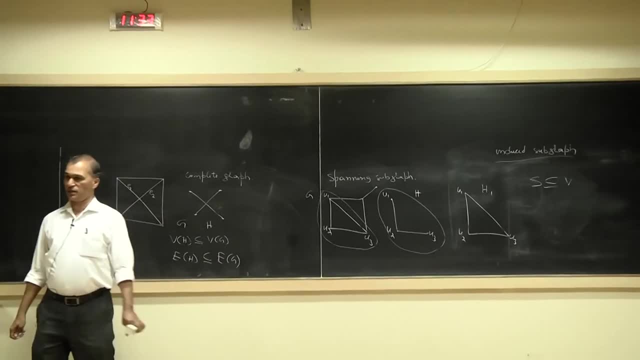 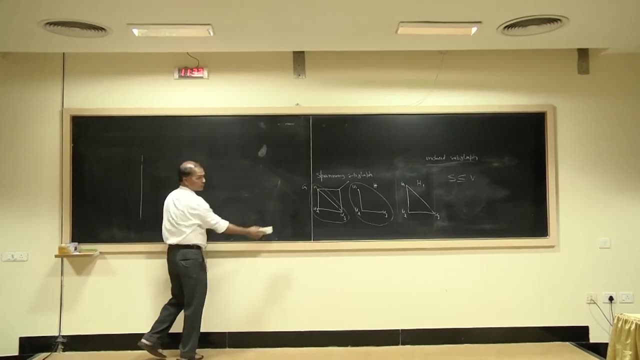 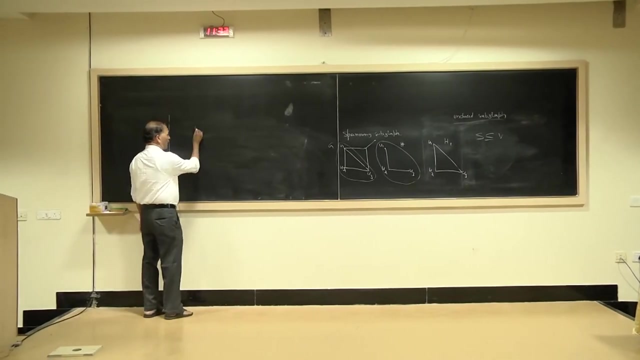 the induced subgraph of g, induced by the vertex set. So this is the maximal subgraph of g, with S as the vertex set: u1,, u2, u3.. Now we can go back to this concept. We can take this graph and: 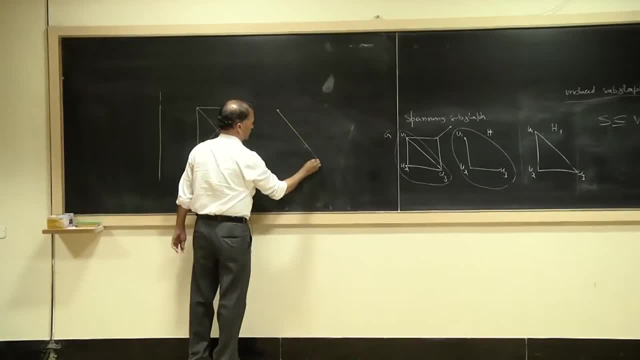 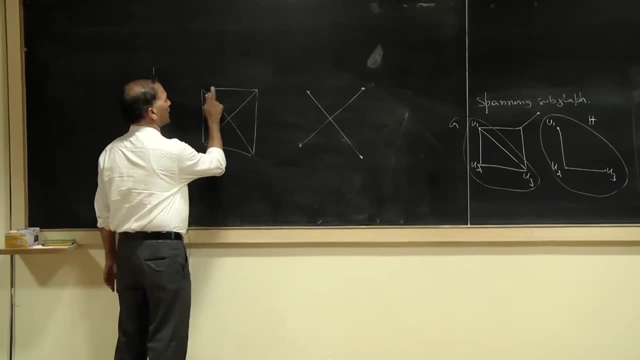 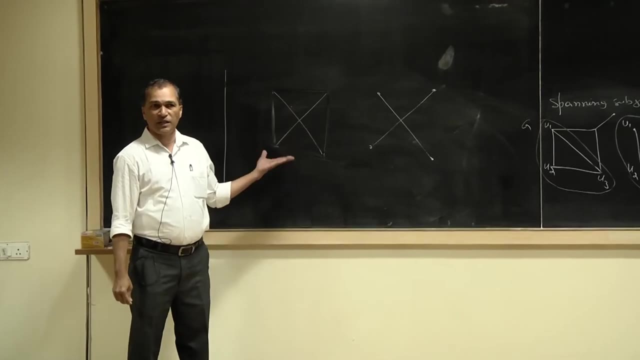 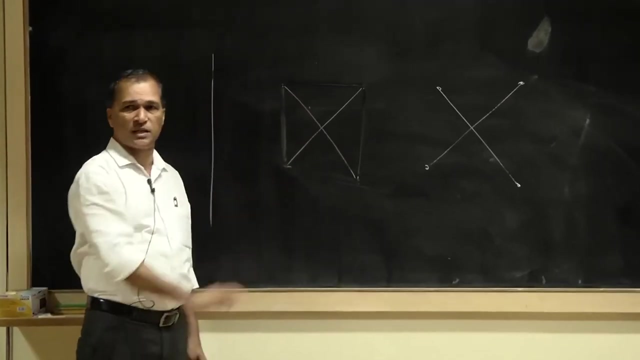 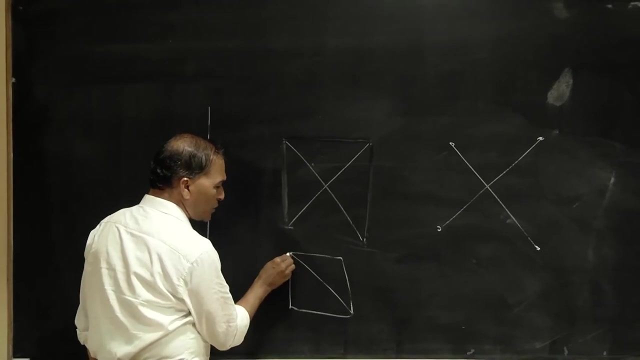 we can consider this subgraph. This subgraph is obtained from this graph by deleting these edges. What do you mean by deleting an edge? Deleting edge is just deleting the edge vertex. that remain same and remaining edges will be as they are. But if you consider the concept of deleting a vertex, if you delete this vertex, for example, 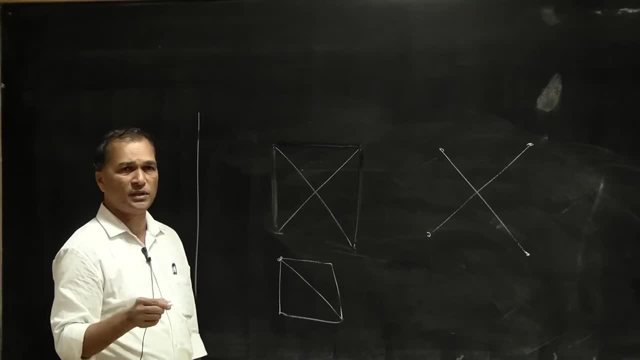 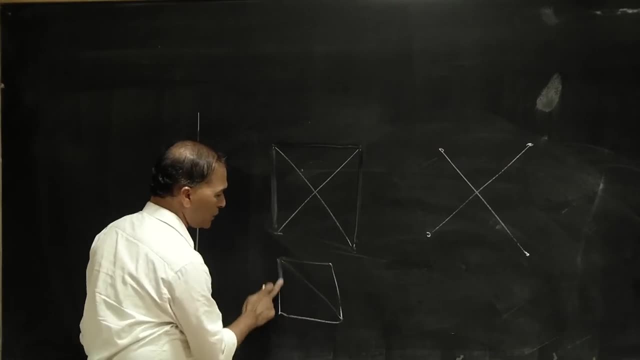 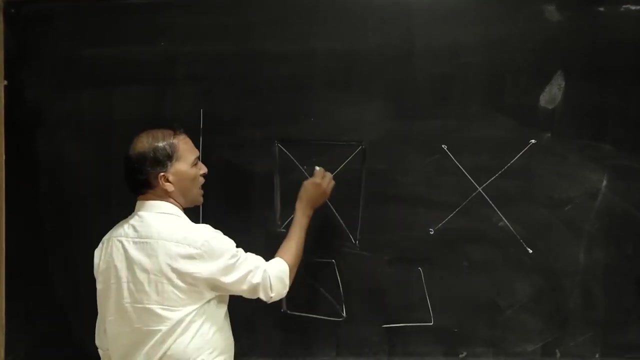 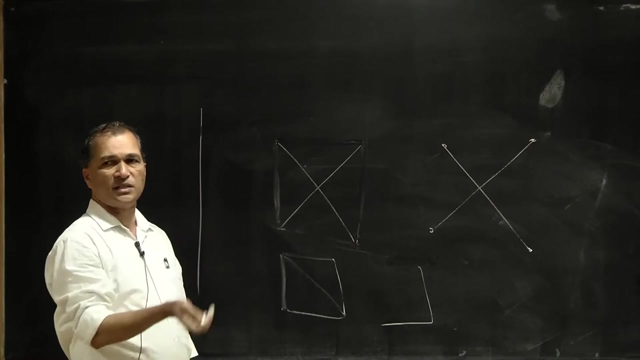 Deleting the vertex means deleting the vertex along with all the edges incident with that vertex. If we delete this vertex, this edge will go, this will go go, this will go, this will go. you get this graph. so this graph can be treated as a graph obtained from the original graph by deleting these edges in that. 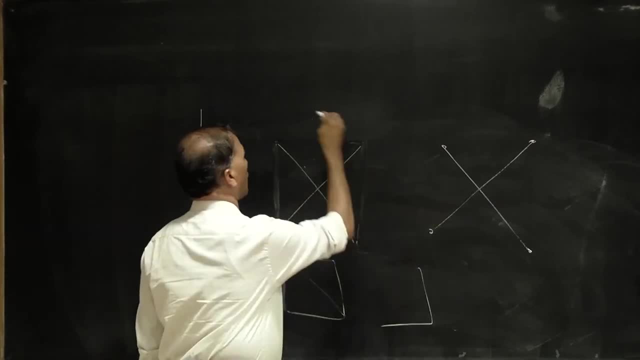 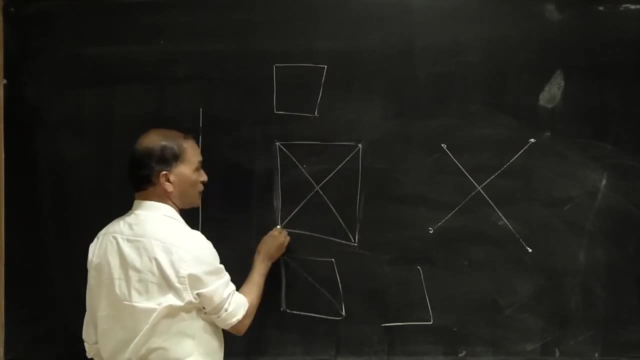 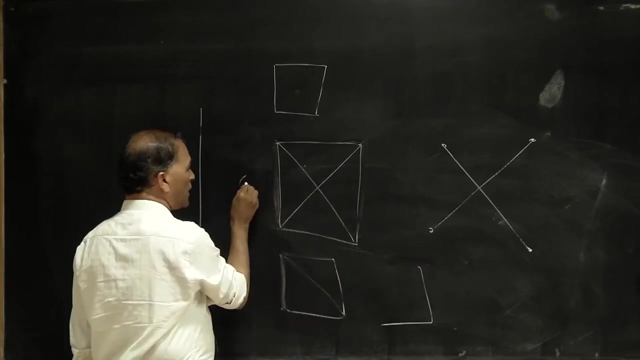 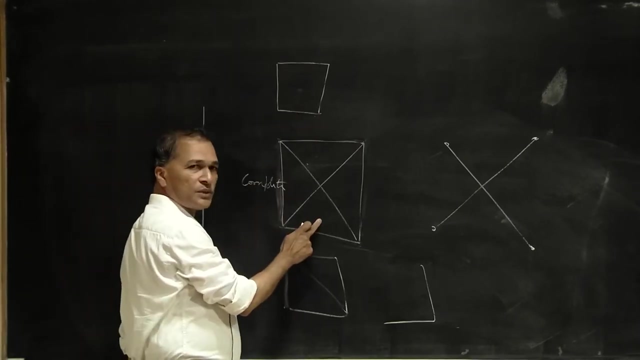 sense we say that this is complement of this graph. original graph is this: we have a subgraph. if you delete these edges from the original graph, we get this graph. this is the corresponding complete graph. complete graph on four vertices. this is subgraph of this graph. if you delete the edges of this graph, 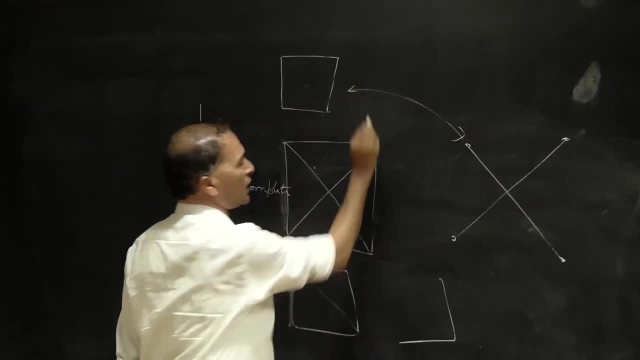 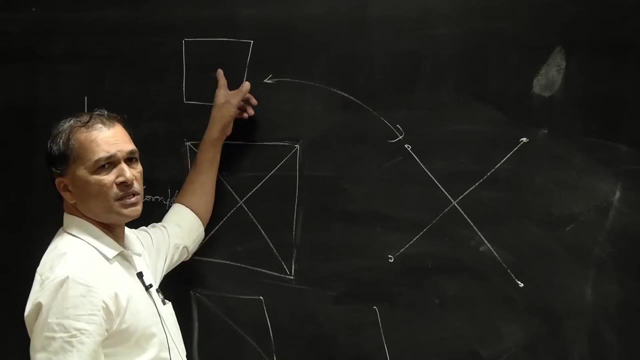 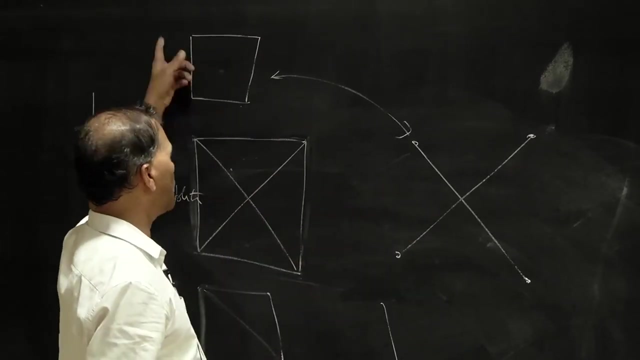 from the complete graph, you get this graph. therefore, these two graphs are called complements of each other, right? this is complement of this graph. this is complement of this graph. this is obtained by deleting these two edges from this graph. this is obtained by deleting these four edges from. 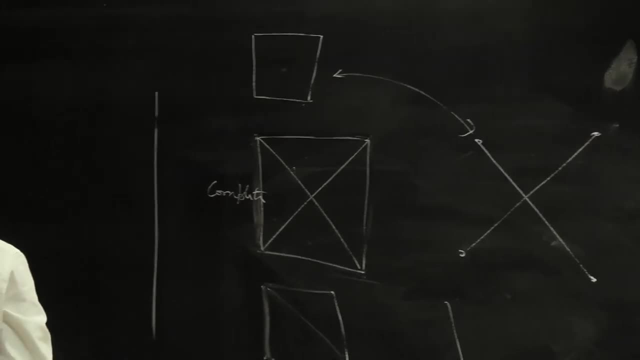 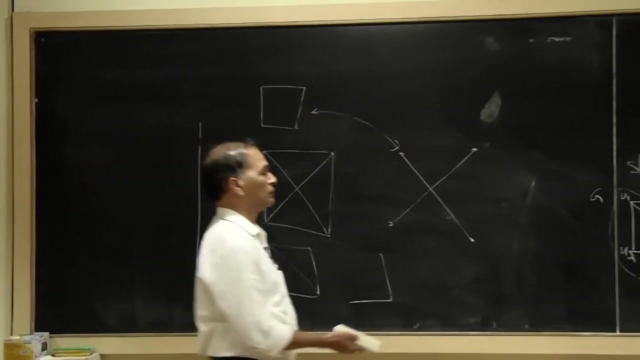 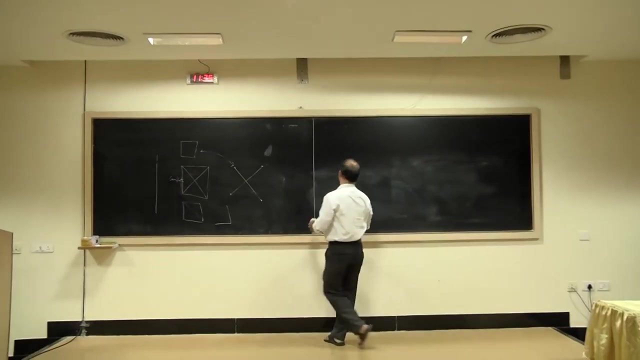 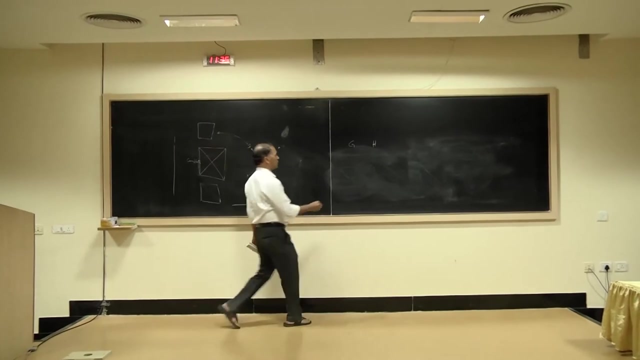 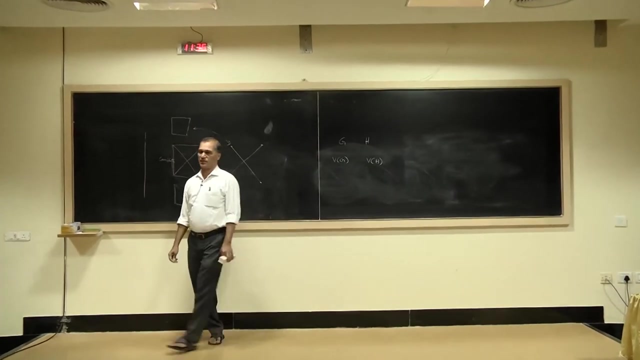 this graph. So whenever we say complement of a graph, it is complement with respect to the corresponding complete graph. right Two graphs, G and H, are said to be isomorphic to each other if there is a one-one-none-two correspondence from V of G to V of H which preserves adjacency. 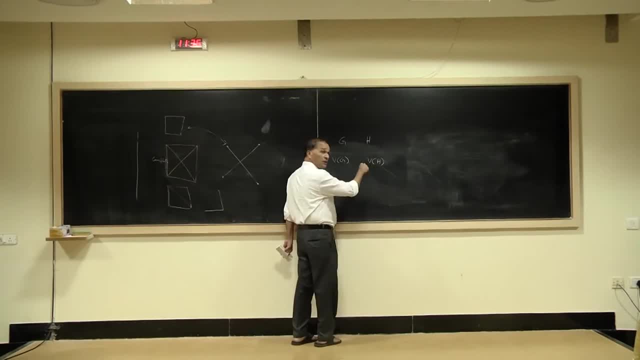 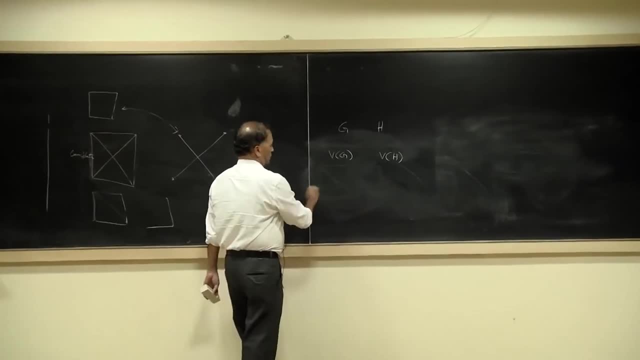 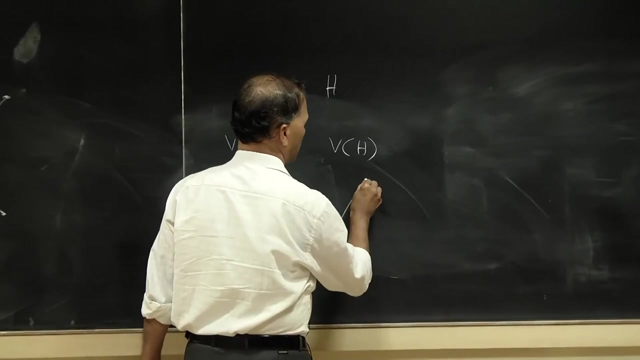 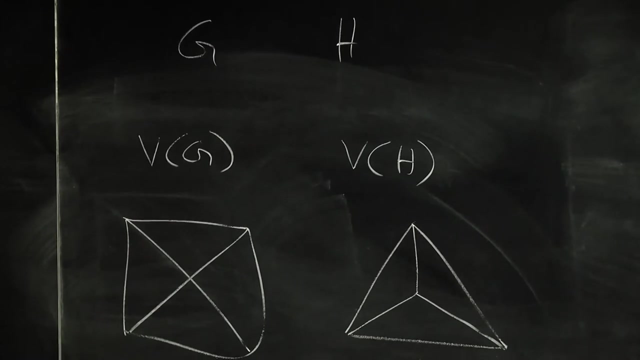 Two vertices are adjacent in G, if, and only if, the images of those two vertices are adjacent in H, right, So you can consider this graph, the complete graph on four vertices, drawn in a different way. Even though they look different, they are isomorphic. We can define an isomorphism from: 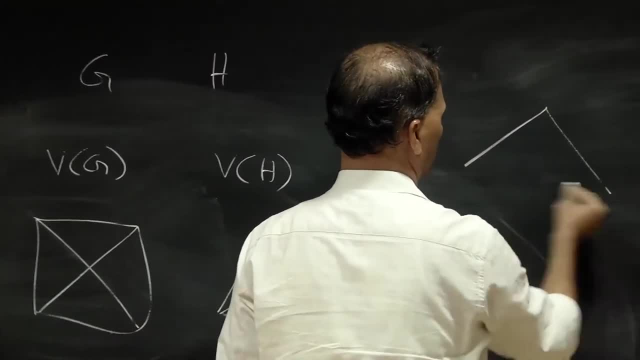 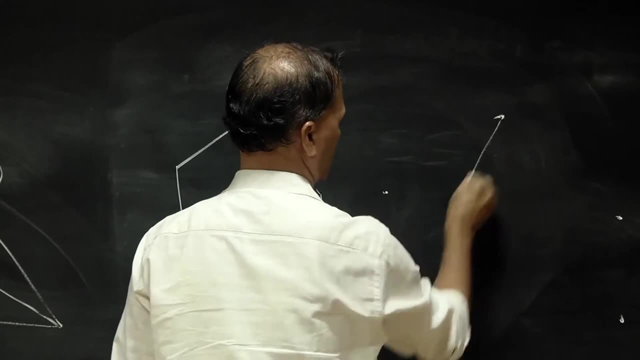 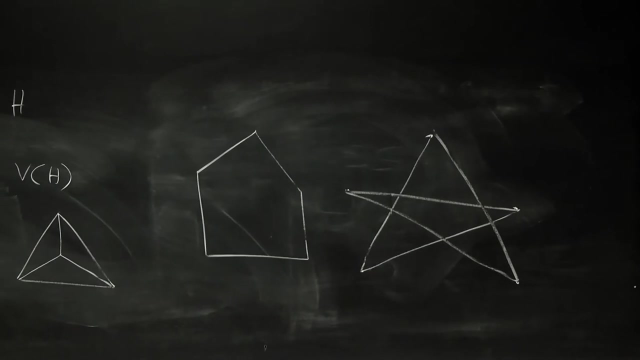 this to this, or you can consider this graph and take the complement of this graph. One can observe that these two are isomorphic. We can define an isomorphism if we say: this is U1 and U2, right, So we can define an isomorphism from these two. So we can define an isomorphism from: 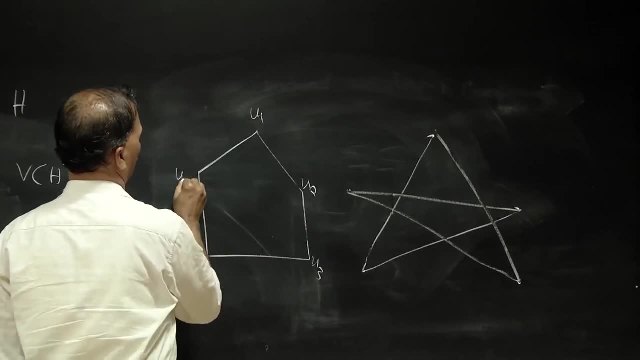 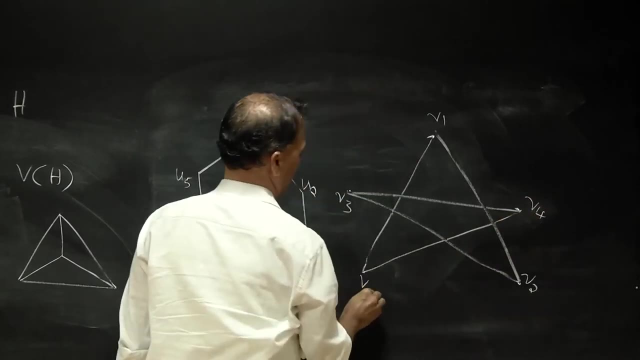 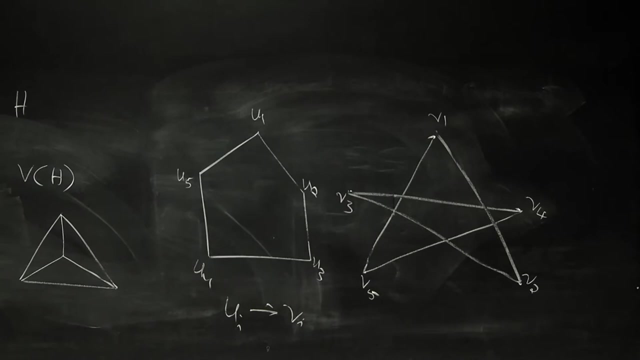 this to this, or we can consider this graph and take the complement of this graph and took the tbsp, these as the isomorphi. So what is a isomorphism from this to this? or can be understood? Bern's equation, that is, where is the�동, Where is the هو? queern's equation is equal to u1, u2, u3, u4, u5. 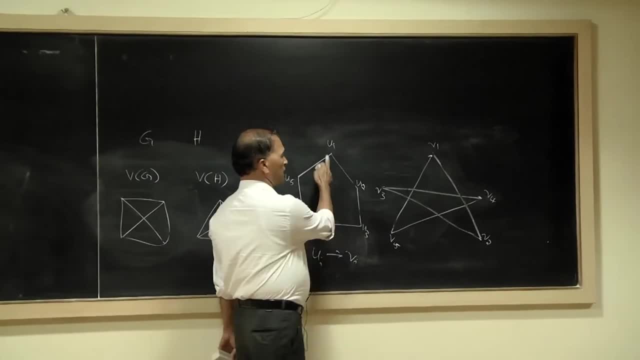 and this is v1, v2, v3, v4, v5.. Ui going to vi is: the isomorphism is equal to 1 to n, 1 to 5, right, So it is a one-one-none-two correspondence between the vertex sets which preserves adjacency. 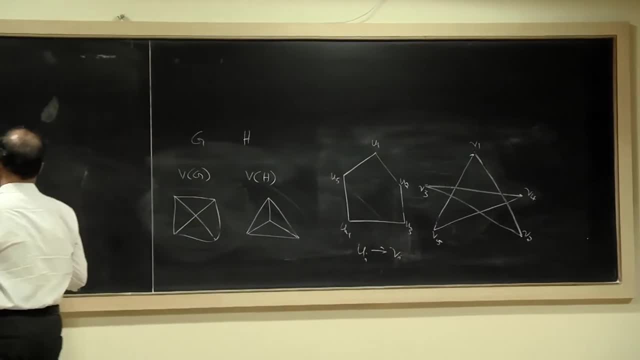 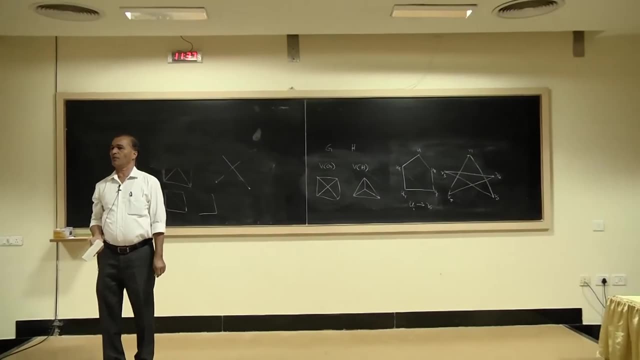 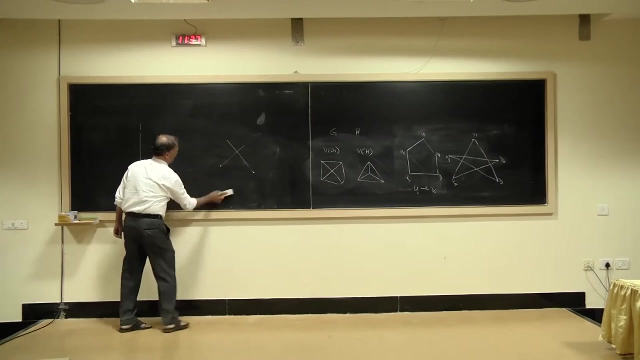 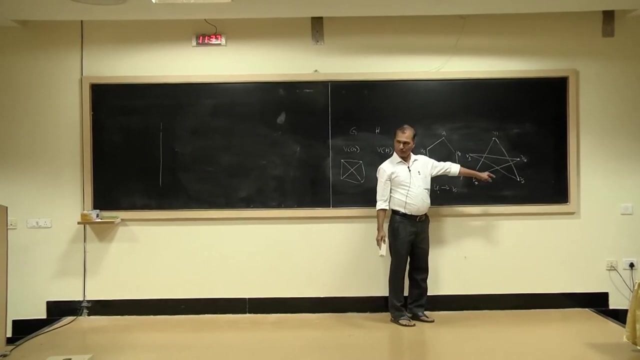 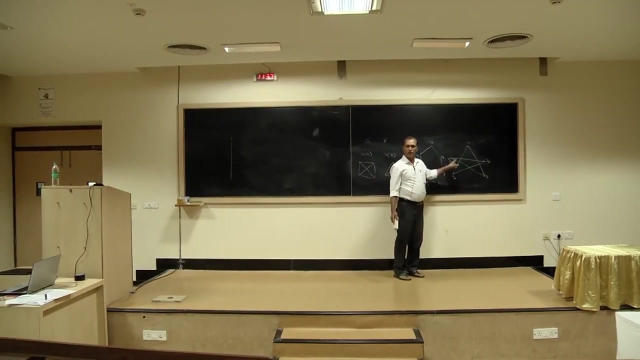 Two vertices are adjacent if there are corresponding images are adjacent, if, and only if, vertex RTC. no, let this be a graph G1, this be a graph G2. I say the G1 and G2 are isomorphic. then we observe that G2 is nothing but complement of G1. 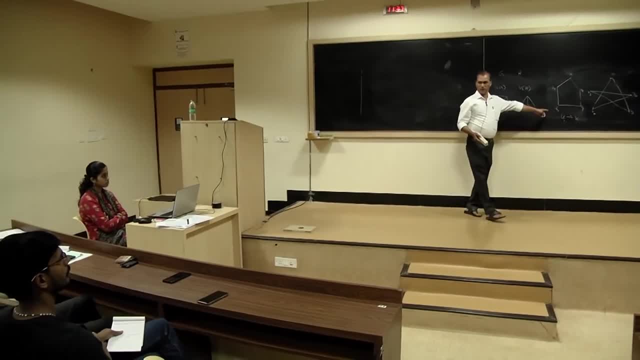 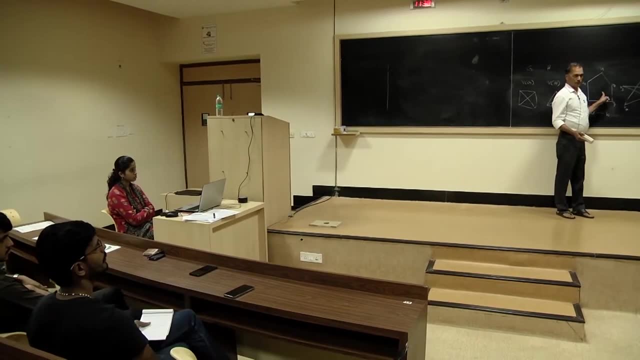 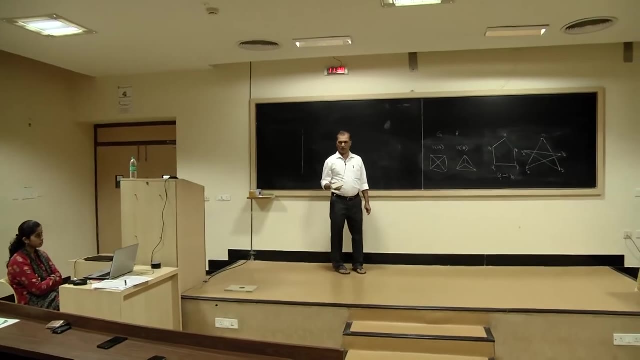 so I have not defined self complementary graph. I was just defining isomorphism. this is isomorphic to this. then we can observe that this is nothing but complement of this. if G is isomorphic to its complement, we say that the graph is self complementary. right, so this graph is self complementary. 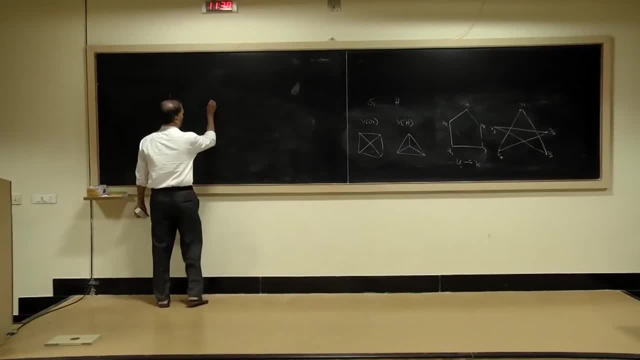 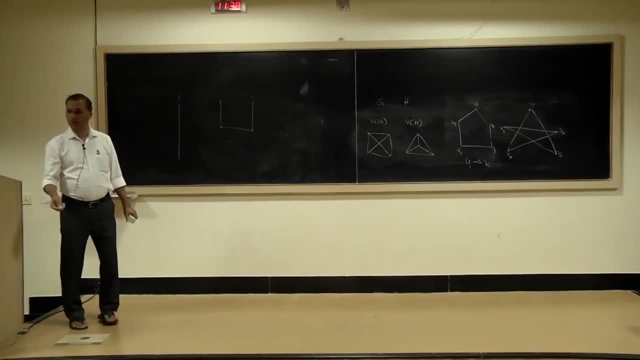 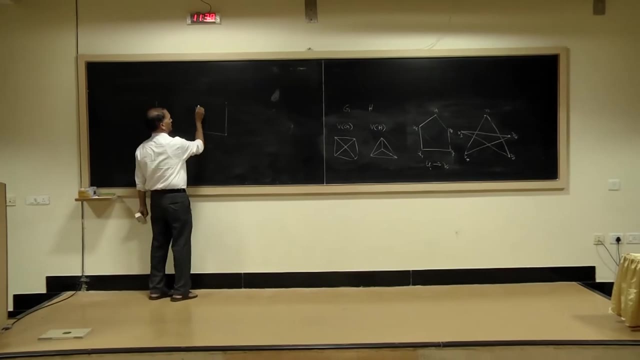 and G2 may be that this graph is also self complementary. this is the smallest graph- smallest in the sense that number of vertices is 4- and it is the smallest of which is self complementary. complement of this graph is nothing but this, which is isomorphic to the original graph. 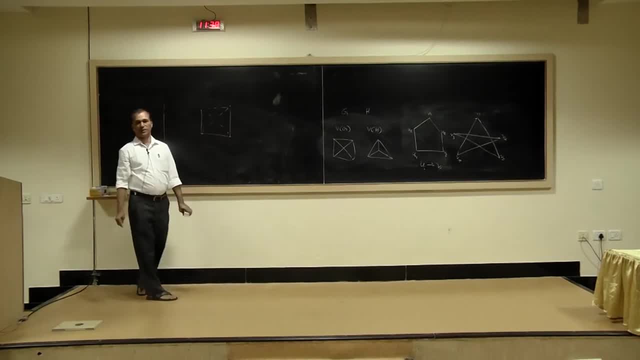 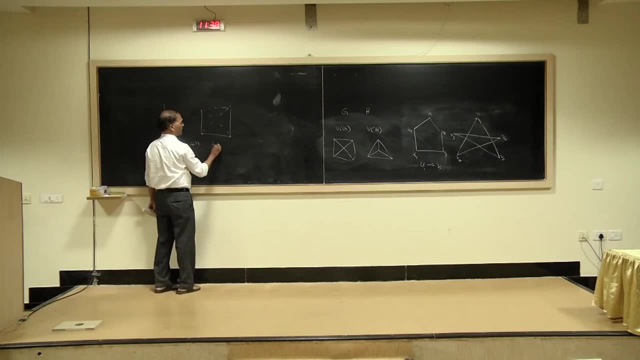 and next graph is that which is self complementary, and one can easily prove that if a graph is self complementary, then the number of vertices should be either 4n or 4n plus 1, either 4 or 5. there is no self complementary graph on 6 vertices. 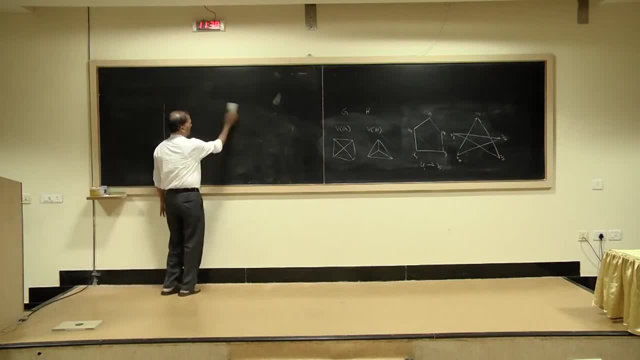 right, there are many, many results on self complementary graphs. we are, which we are not going to do- then we can define the most important concept in graph theory, that is, the distance between two vertices. if we take a graph, if this is U and this is V, if this is U and this is V. 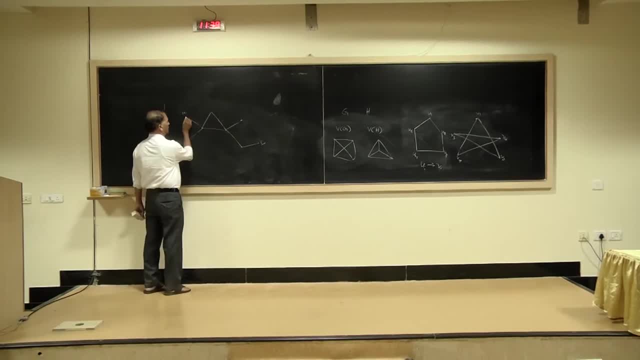 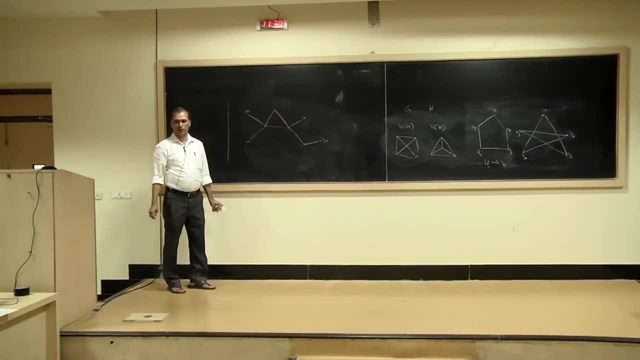 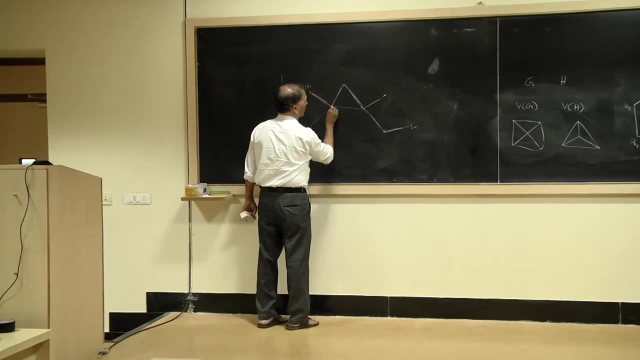 from U to V. we have to move along the graph. may be that we can go like this, then go like this, then go like this, then along a path, not along a walk, along a path, right. so this is one path possible. this is the other path possible. 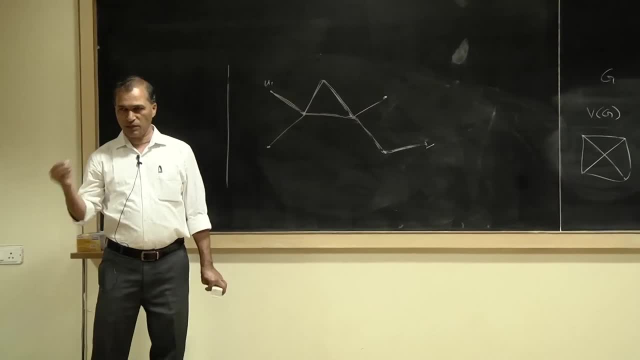 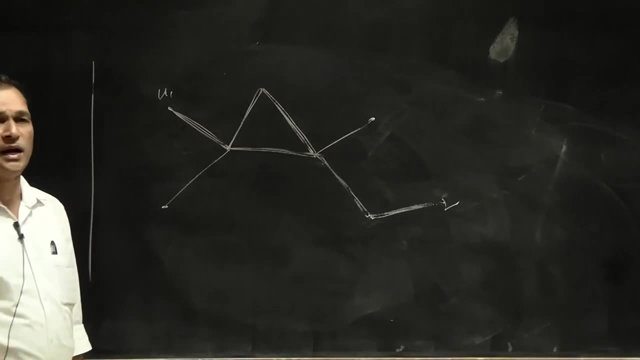 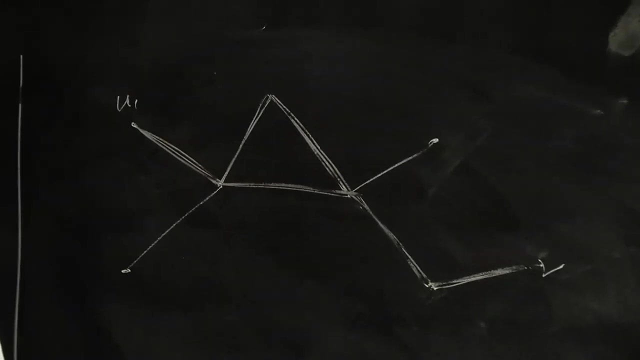 they are of different length. length is nothing but number of edges in the path, so we can define. once they are of different length, we can find out that path with minimum length, which has minimum number of edges. such a path is called a shortest path if a G is connected. graph. 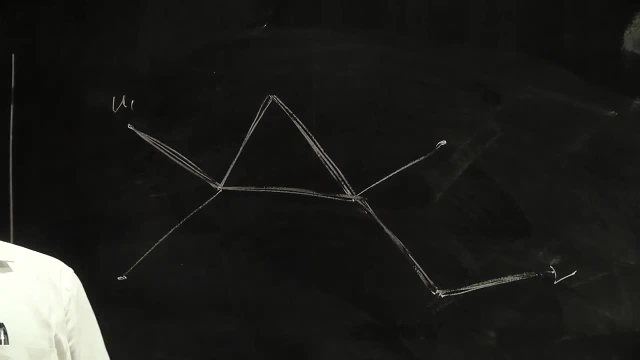 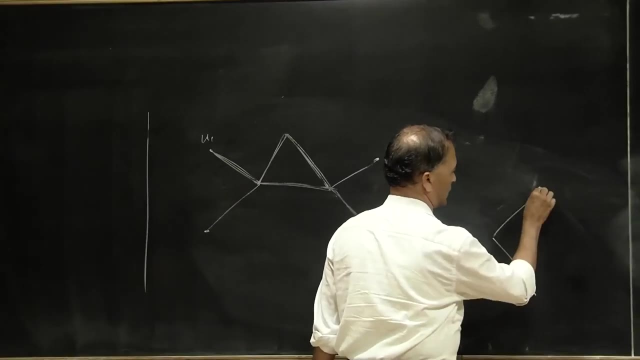 between every two vertices there is a path and, obviously, between every two vertices there is a shortest path. may be that there are many shortest paths, may be. the graph is like this: this is one shortest path, this is the second one. this is the third one. this is the fourth one. 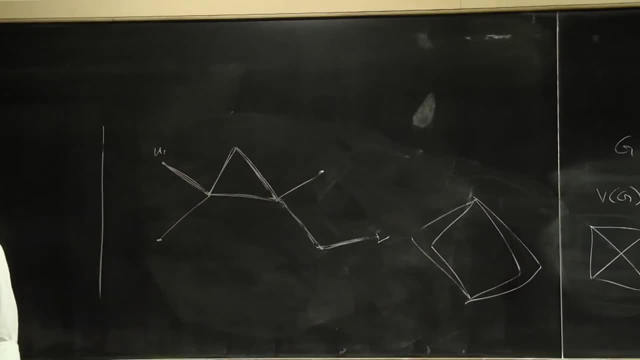 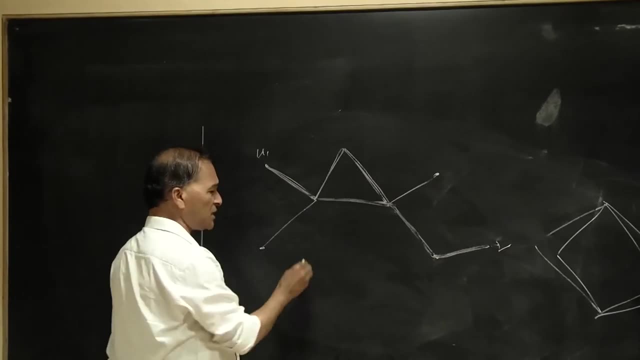 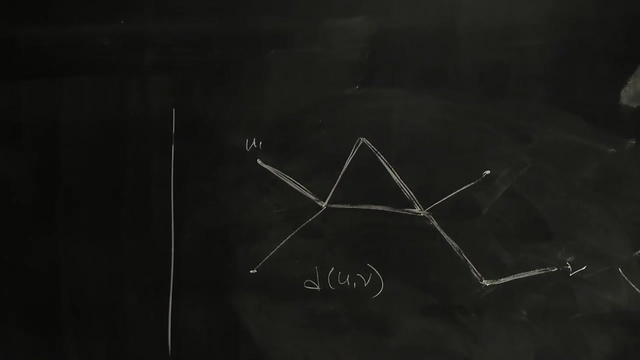 between these two vertices can have any number of shortest paths. right, the length of the shortest path. length of a shortest path is called the distance between U and V. dUV is length of a shortest path between U and V in the graph G. as I said, there may be any number of shortest paths. 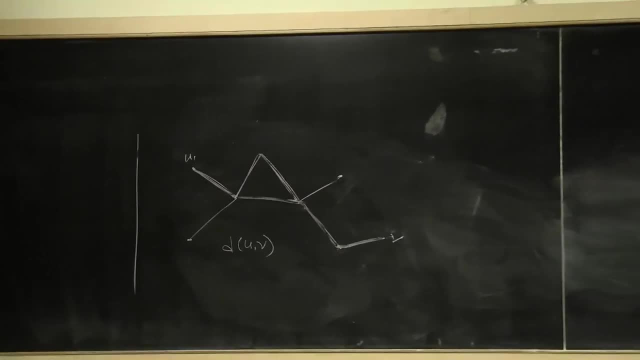 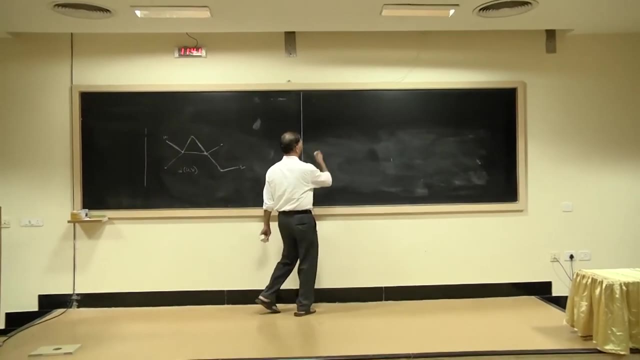 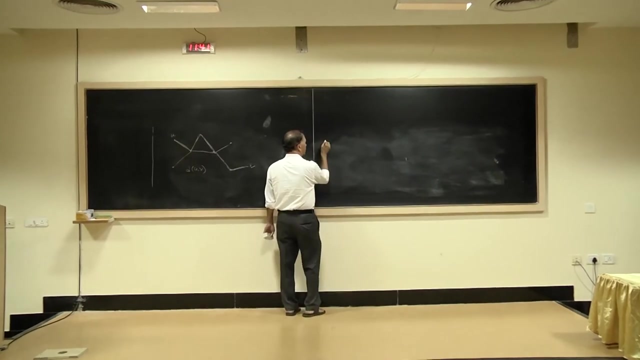 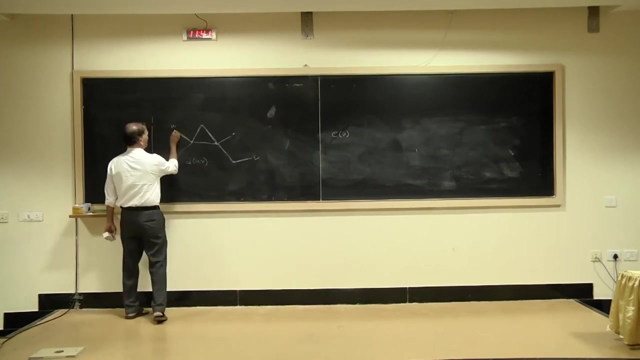 and again. obviously, any two shortest paths should have the same number of edges. they have the same length. once we define the distance, we observe that it is symmetric, and we define something which is called eccentricity of a vertex U, for example, this vertex. the distance between this and this is one. 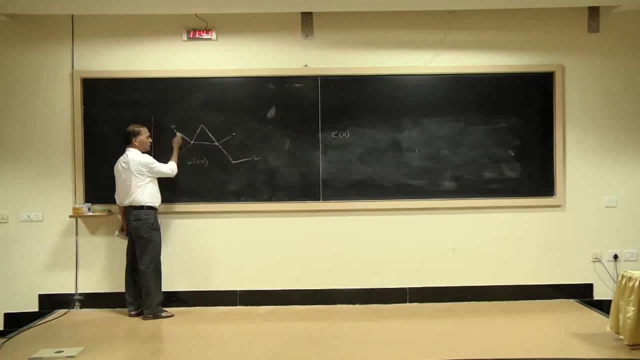 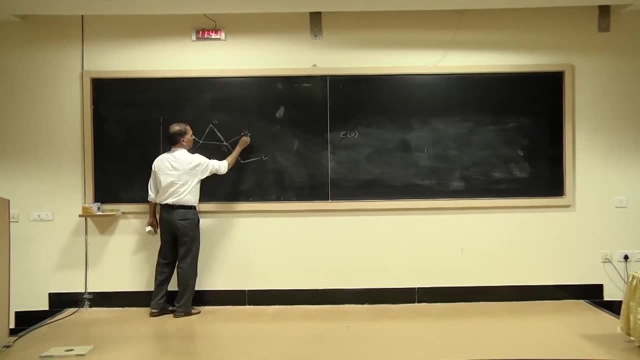 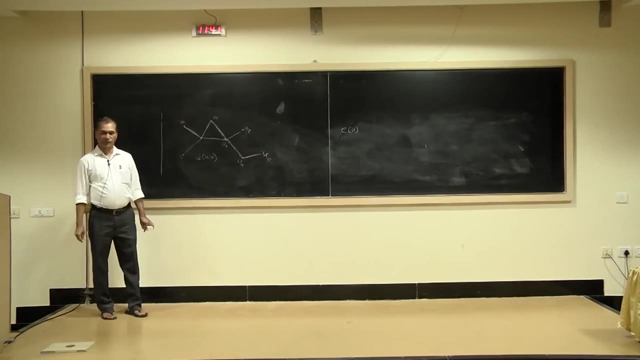 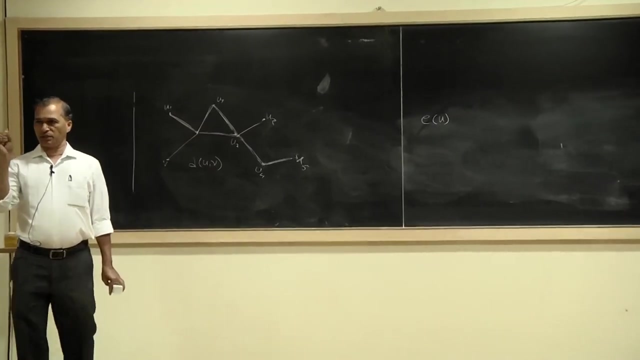 distance between this and V is two. distance between this is: U1 is two, U2 is two, U3 is three, U4 is four and U5 is five. right. one, two, three, four. this is four right. so we can find out the distance of a given vertex. 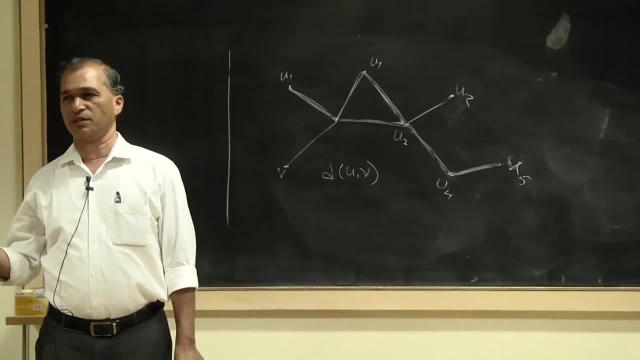 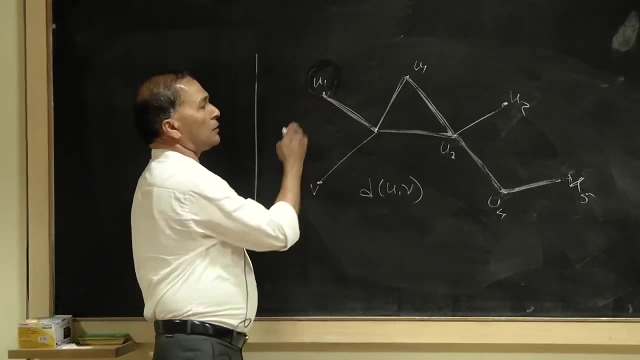 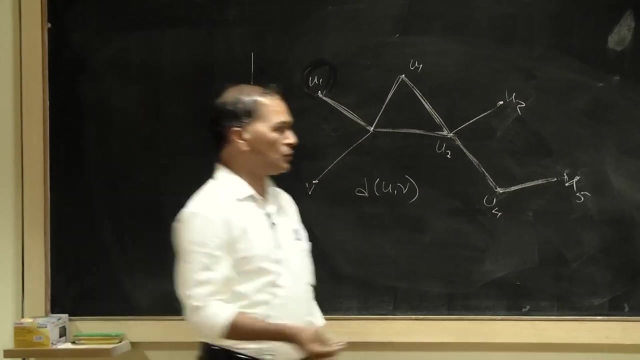 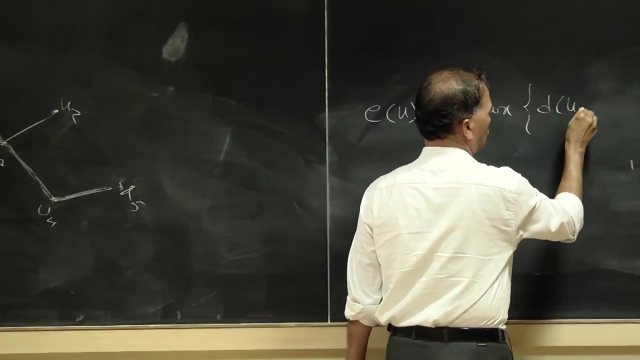 from a given vertex to all other vertices, with the assumption that distance between U1 with itself is zero, right, so we can find out all the distances. out of these distances, what is the maximum? so eccentricity of U is defined to be equal to maximum of dUV. 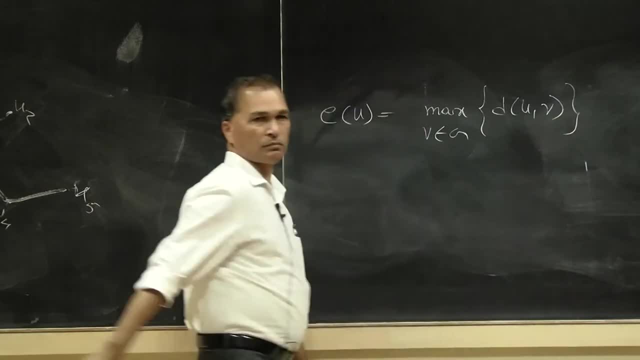 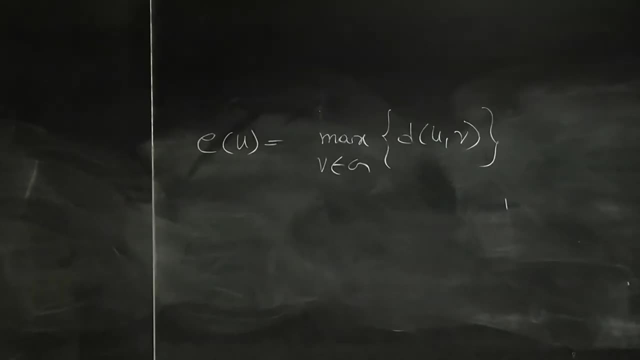 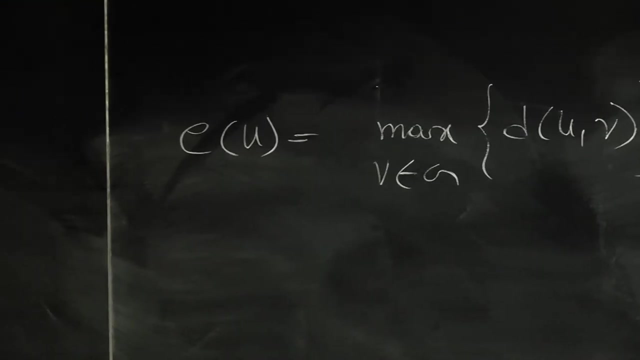 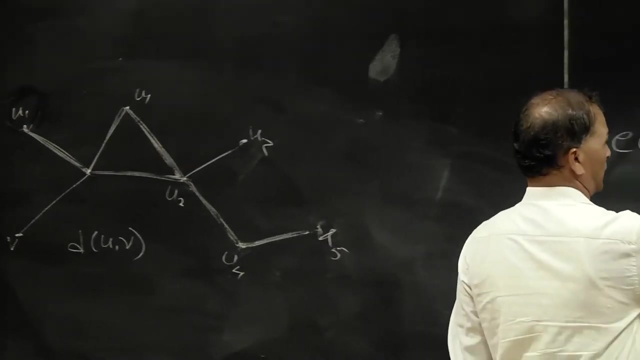 V belongs to G. consider all possible vertices. V. find out dUV for every V. find out maximum of that. that is called eccentricity. that is the distance from this vertex to that vertex which is farthest from this vertex, right? so we define eccentricity to be equal to maximum of dUV. 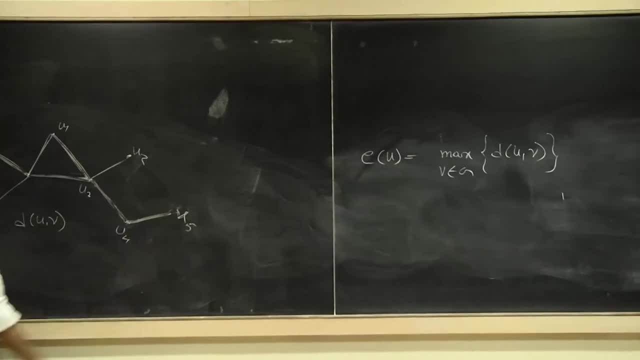 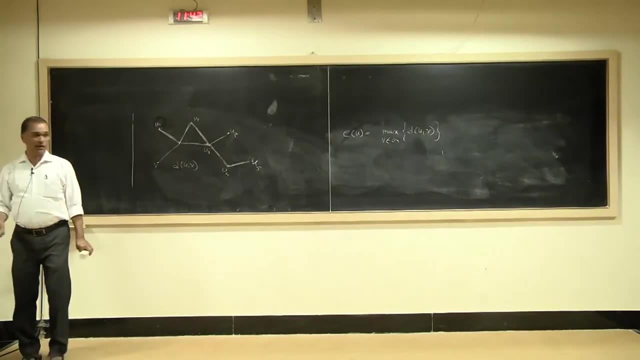 eccentricity of this vertex which is farthest from this vertex? eccentricity of this vertex one, two, three, four. maybe with every vertex we can find out the eccentricity of the vertex E of U for every U right E of U. if you consider it is set of all. 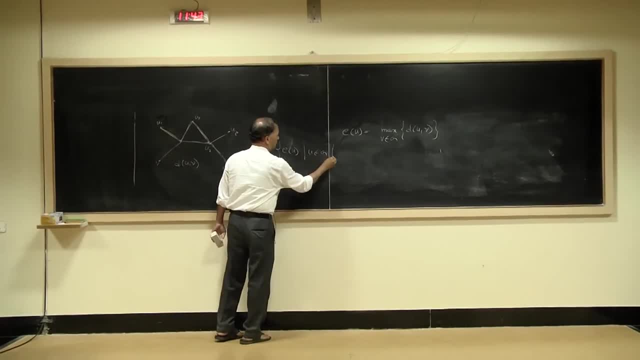 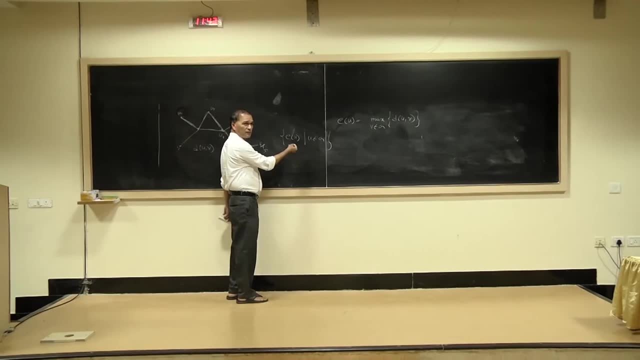 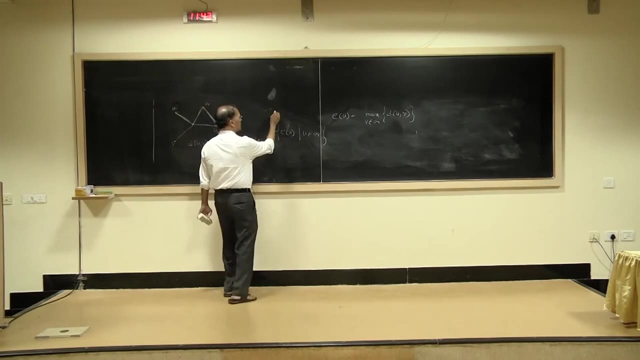 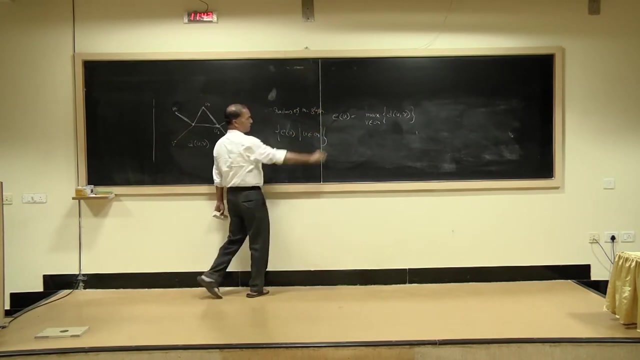 E of U, such that U belongs to G. it is a set of positive integers. right it has a minimal element, smallest element, that is a vertex with the smallest eccentricity. right, that is called radius of the graph. we consider all the eccentricities, find out the minimum of them. 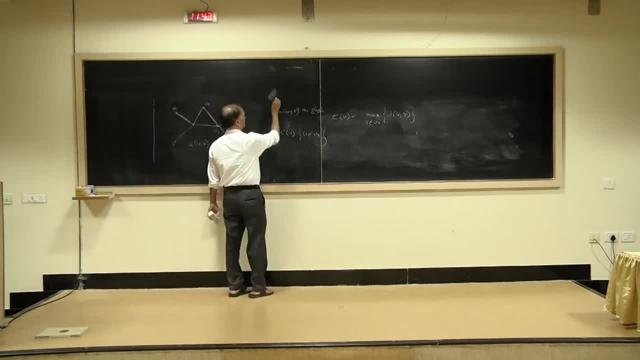 that is called radius of the graph, and find out maximum of them. that is called diameter of the graph. right? for example, if we consider this graph, eccentricity of this vertex is 1, 2, 3, this also 3, this also 3, this also 3. 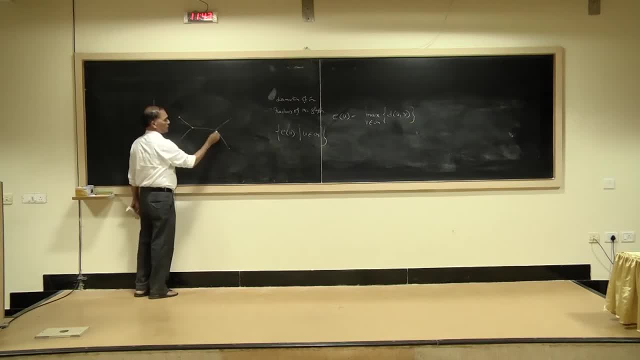 for this one. it is 2, this is 2, this also 2. so the eccentricity of this vertex is 2. eccentricity of this vertex is 2. that is a minimum for all this vertices. the eccentricty is 3, right, right. So this vertex, 2 is radius of this graph r of g. radius of g is equal to 2. 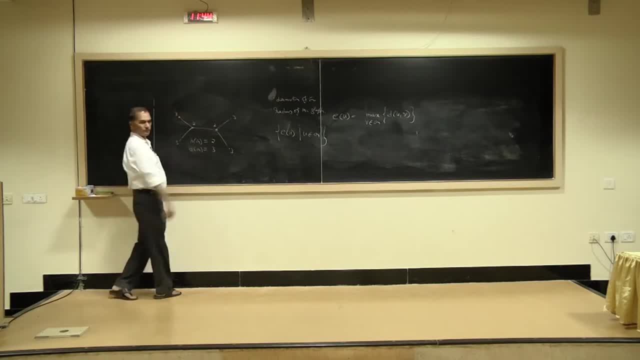 and diameter of g is equal to 3, right. This vertex a? u, eccentricity of which is equal to radius of the graph, is called a central vertex. A vertex is called a central vertex if its eccentricity is same as the radius or, equivalently. eccentricity is the minimum right. This v. 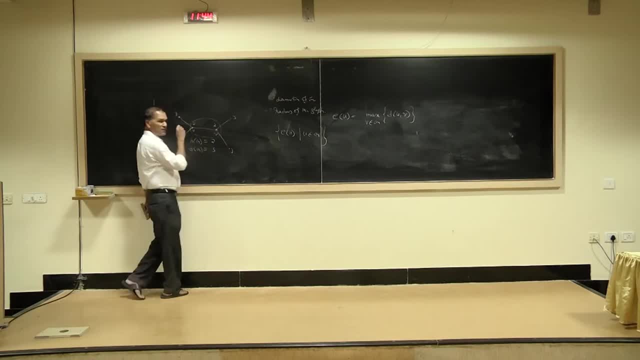 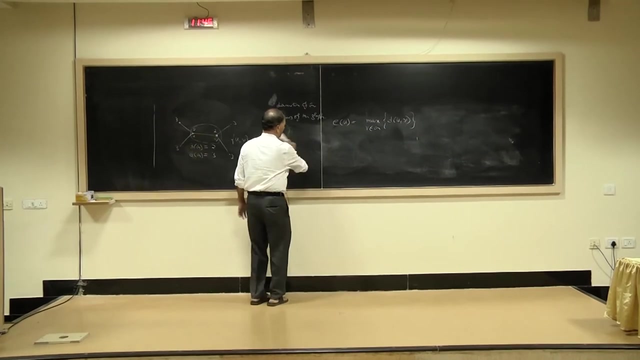 also has that property. The set of all central vertices in a graph is called center of the graph. Center of g is, for example, for this graph, center is u comma v. this is the center right. So a graph is said to be self-centered if the graph itself is the center of the graph. 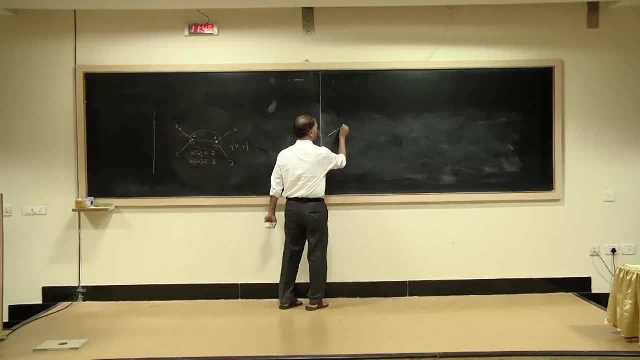 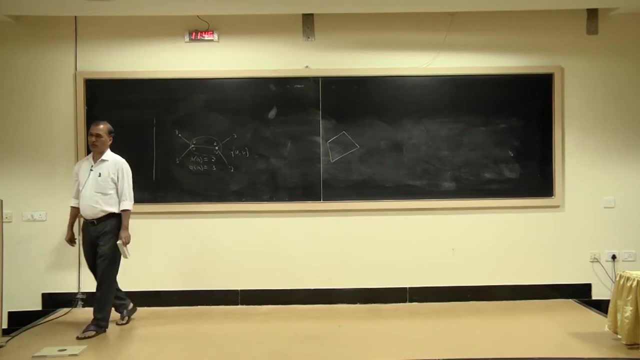 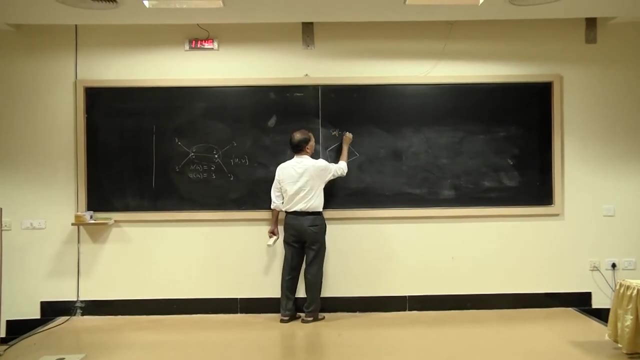 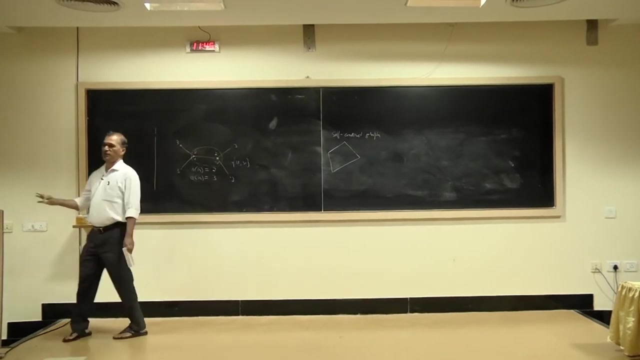 All the vertices are there in the center. for example, if you consider this graph, may be this graph, All the vertices are of eccentricity equal to 2.. So this is a self-centered graph, A graph in which all the vertices are of same eccentricity. right Again, characterization. 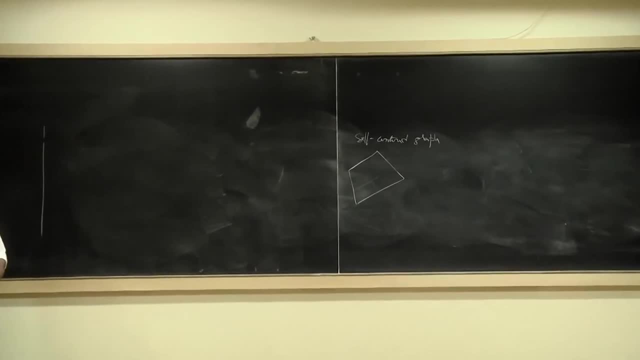 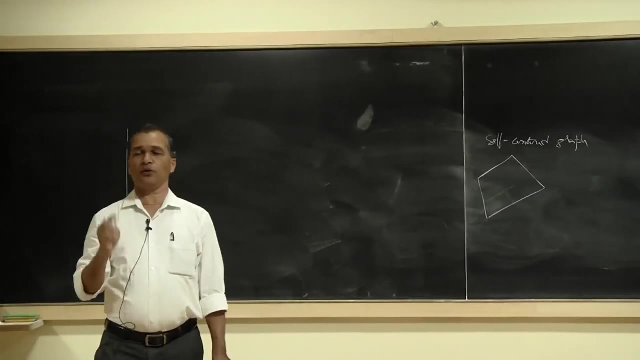 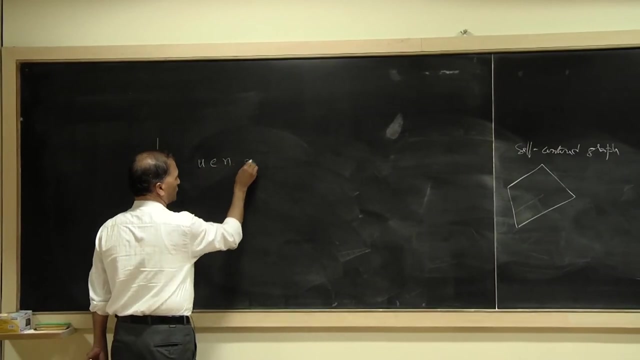 of self-centered graphs and all those things are there in the theory. those who are interested can refer. And the one other concept is required. that is called unique eccentric node graph. A graph is called unique eccentric node UEN graph If for every vertex in the graph there 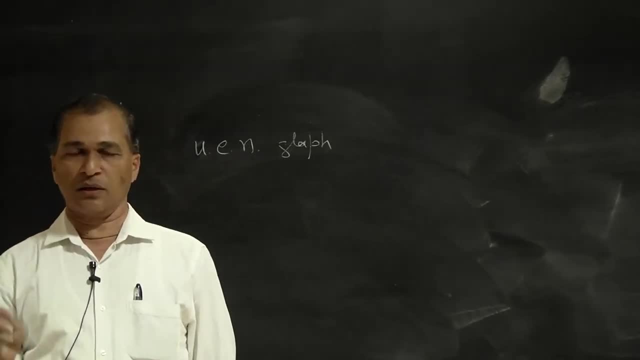 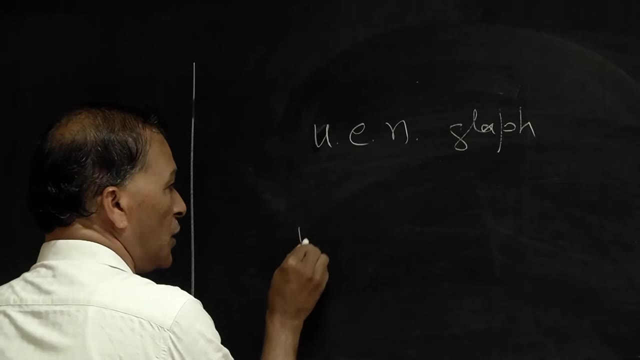 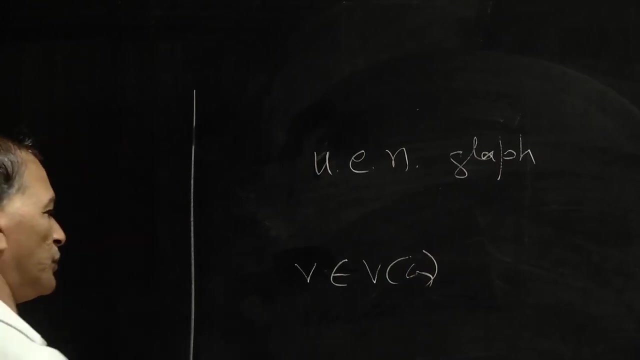 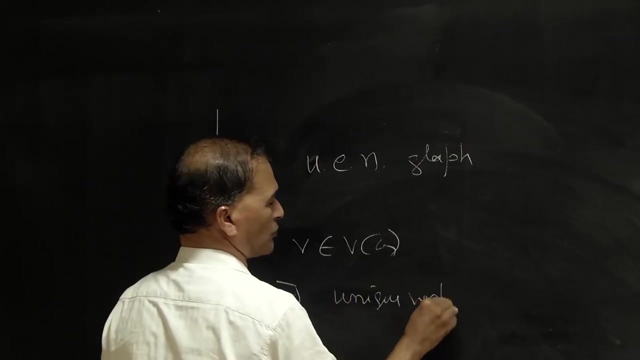 is a unique vertex, the distance between them is equal to the eccentricity of the vertex: U percent. that's excруго, For example, you. if v is a vertex, in the vertex set of the graph g, there exists exactly one vertex or a unique vertex, v, such that it is equal. 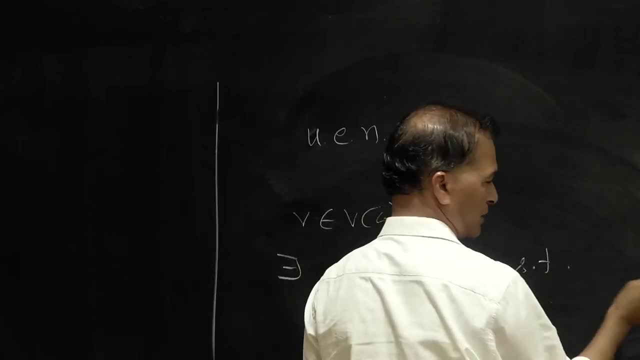 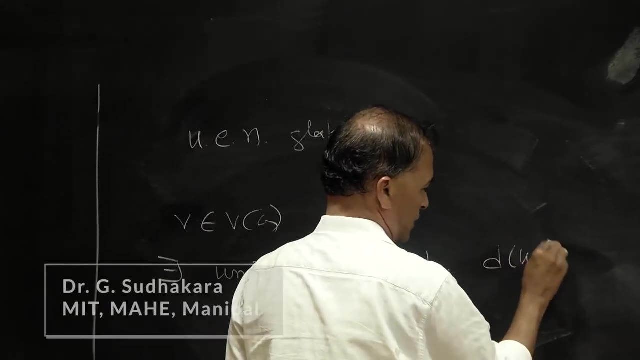 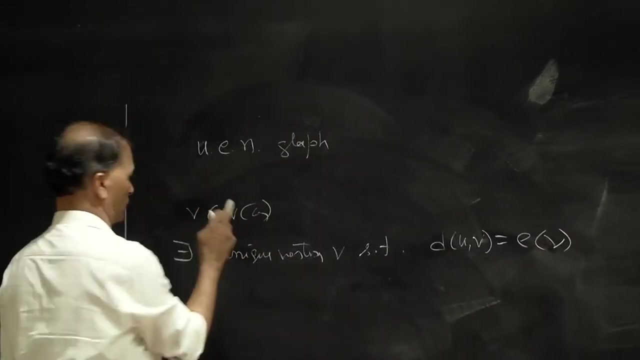 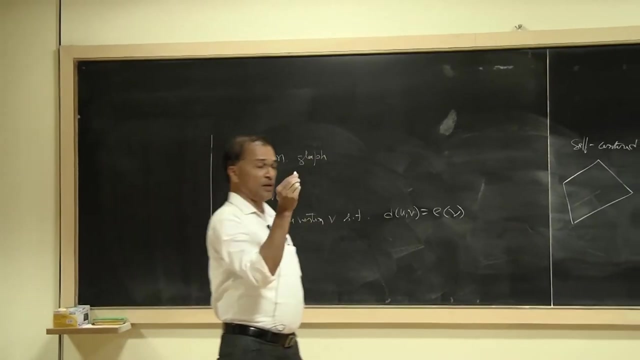 to the eccentricity of the vertex u, vector u equal to vertical u. That can be noted that eccentricity duv is equal to eccentricity of u. eccentricity of v for every v belonging to J. Eccentric node means what For a vertex v? a vertex u is called an eccentric node. 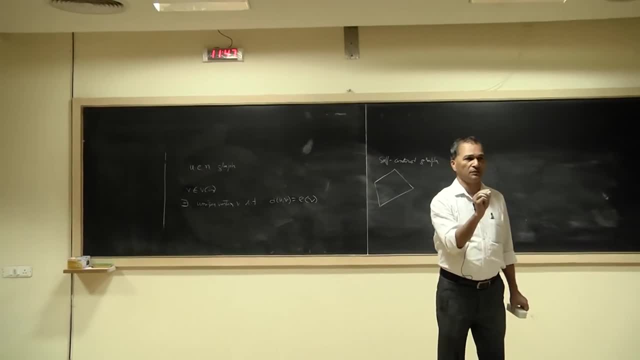 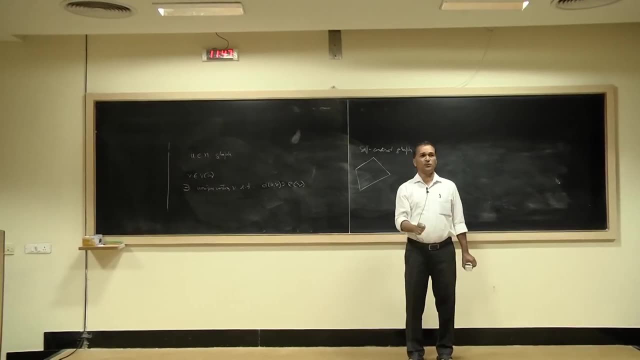 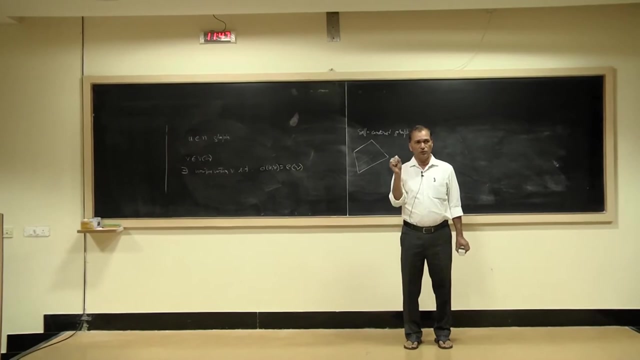 if distance between u and v is equal to eccentricity of v right. Eccentric node graph means what For every vertex there is exactly one vertex, such that every vertex v there is exactly one u, such that dvu is equal to eccentricity of v right. 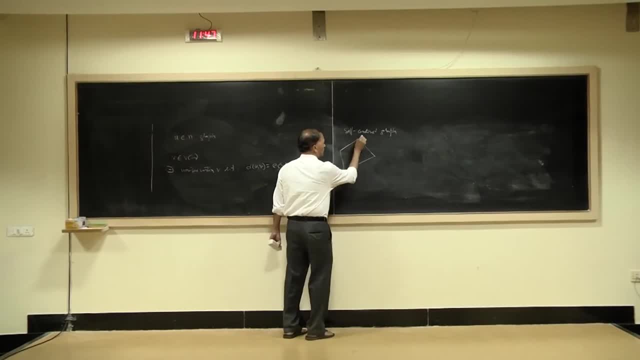 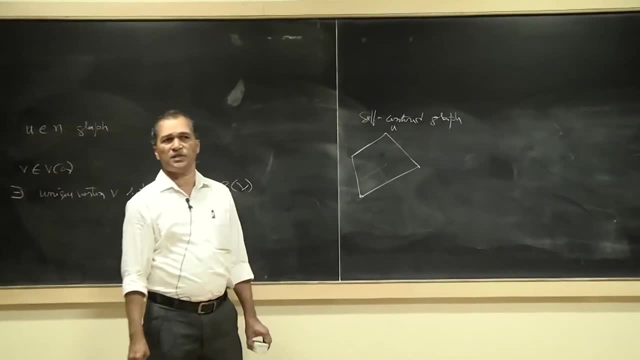 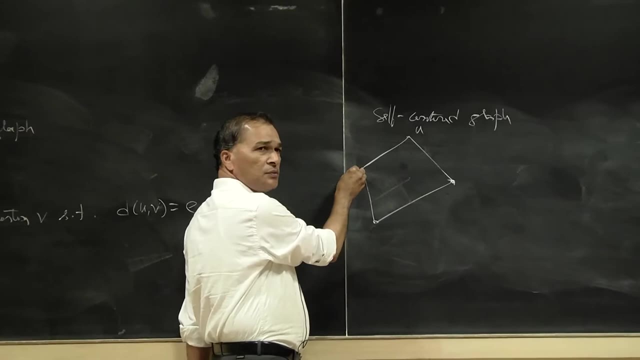 Again this graph. for example, if we consider u, eccentricity of u is equal to 2, there is exactly one vertex which is at distance 2.. For every such vertex, every vertex u is equal to u. there is exactly one vertex which is at distance 2.. So it is a unique eccentric. 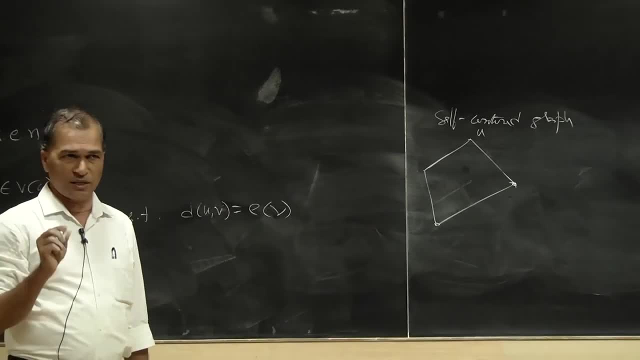 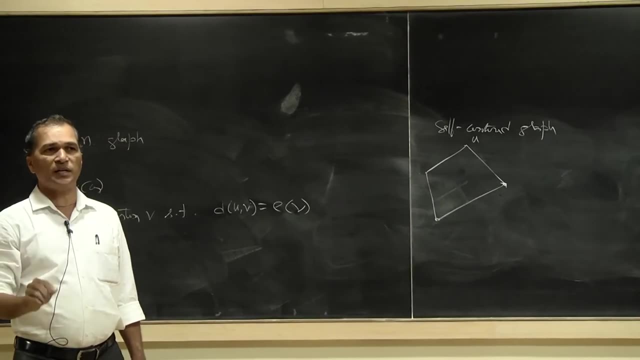 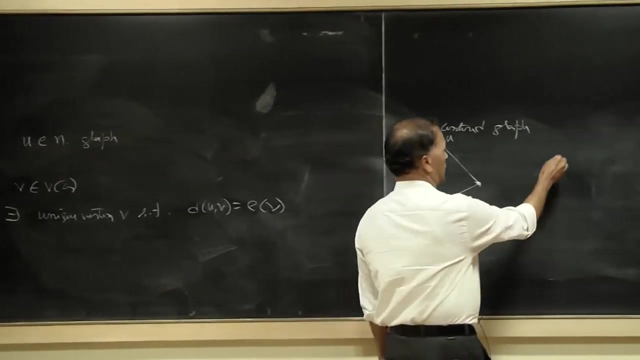 node graph. right, A unique eccentric node graph is a graph in which, for every vertex, there exists exactly one vertex which is at distance equal to eccentricity of that vertex. right. We can generalize this concept, for example this graph we can consider: You take: 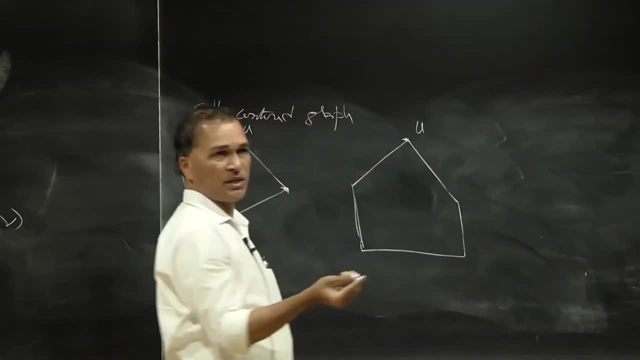 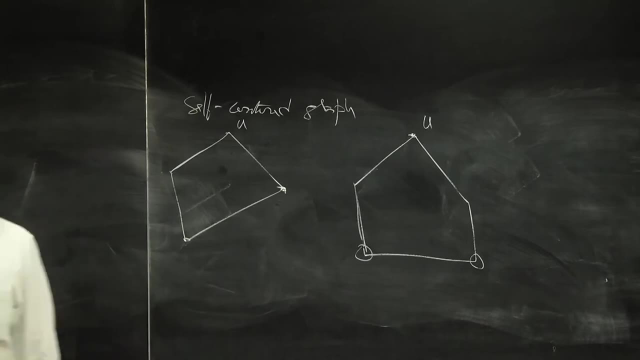 the vertex u. what is eccentricity of u? Eccentricity of u is 2, right For every u. here there are exactly two vertices, which are the eccentric vertices, right? So there are exactly two eccentric vertices for every vertex, If G is a graph such that for every vertex there, 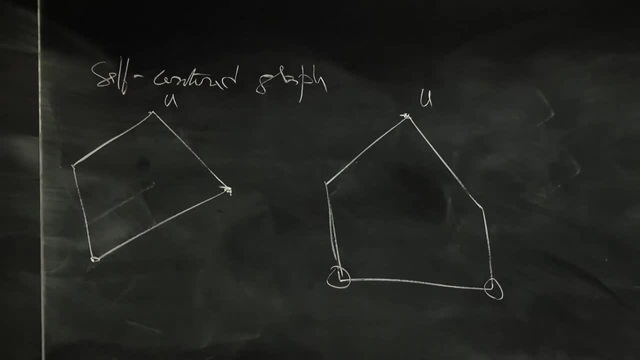 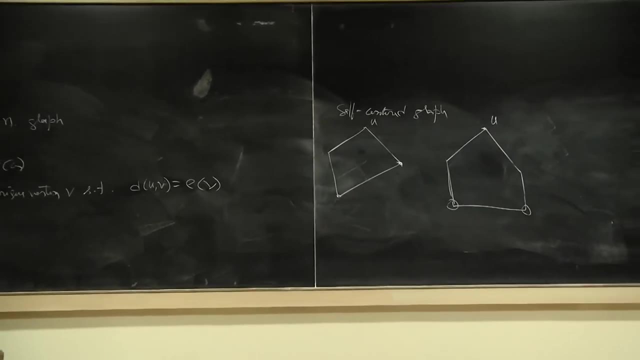 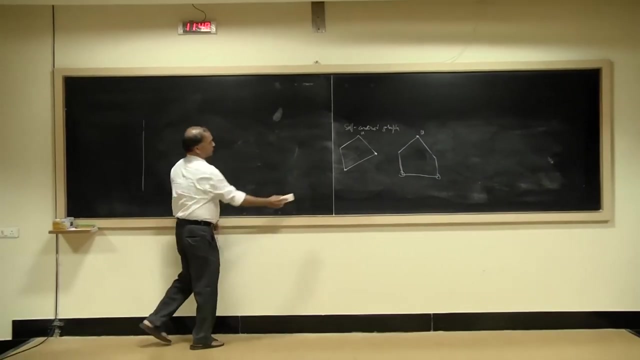 are k eccentric vertices, then instead of unique eccentric node vertex we can say that it is k eccentric node vertex. We can try to characterize such graphs. maybe that the characterization is not there so far. So that is k eccentric node graph. The example is: 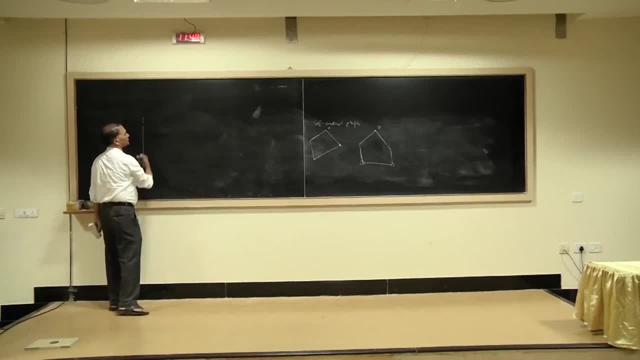 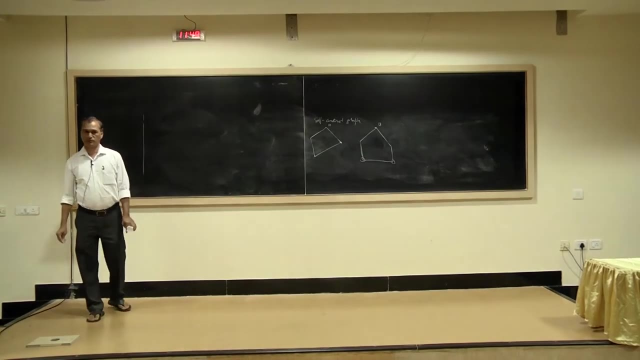 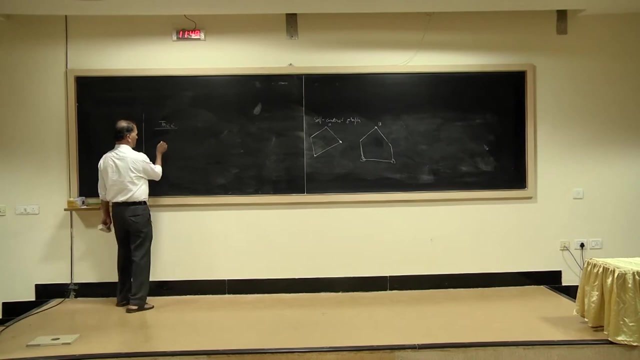 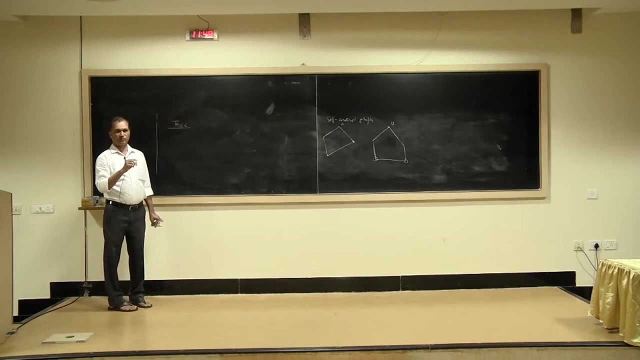 that that is, 2 eccentric node graph, Self complementary graph, we have defined and this we have defined. Maybe that the most important type of graph is called a tree Tree is most important because it is the most simple graph. Most simple in the sense that there are only two properties to be satisfied by a tree One. 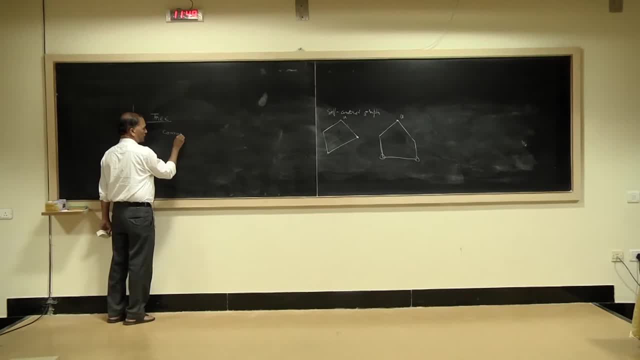 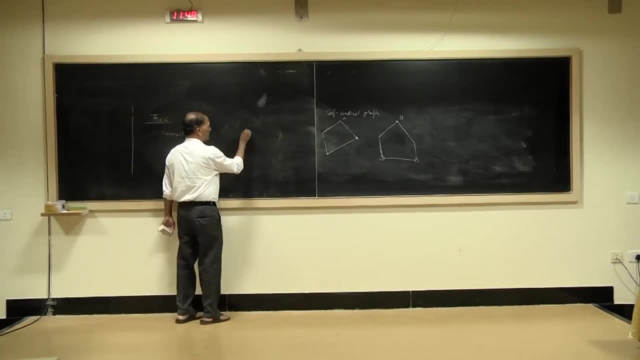 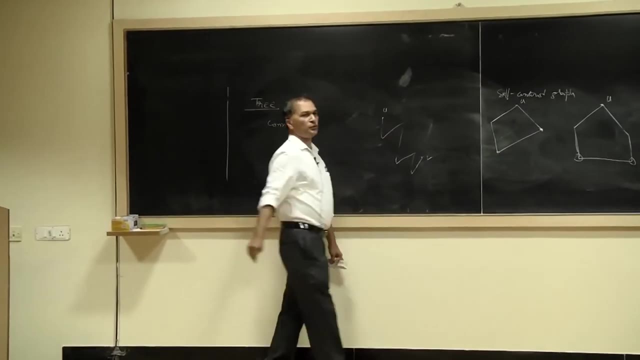 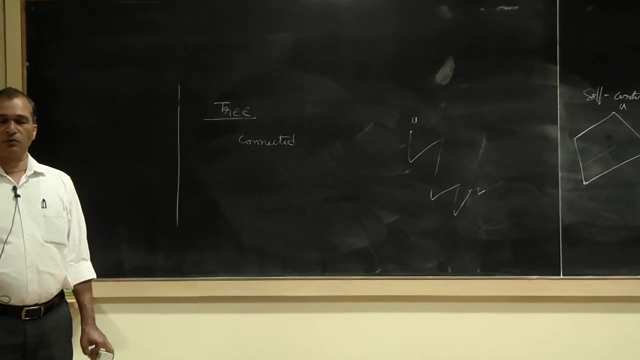 is that it should be a connected graph. We know what is connected. We know what is connected. Right, When we say it is connected, a graph is connected. we know that there is a path between a very two vertices. When we say there is a path between a very two vertices: one. 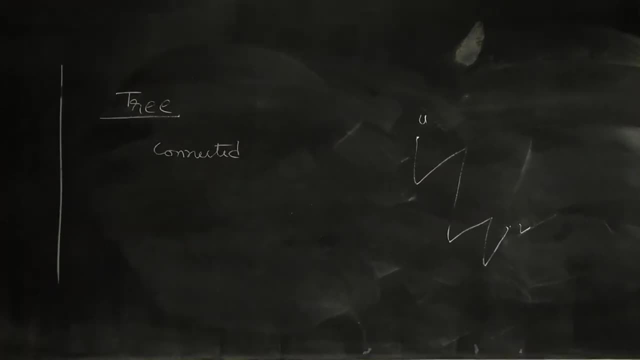 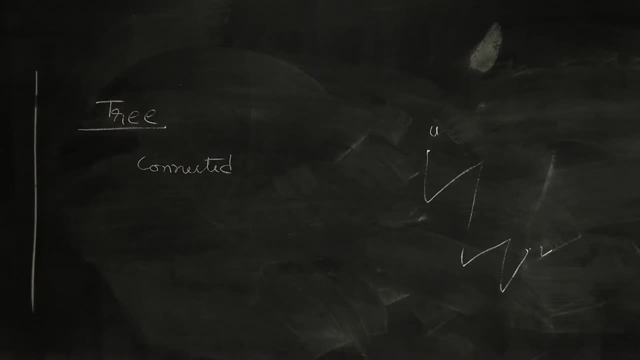 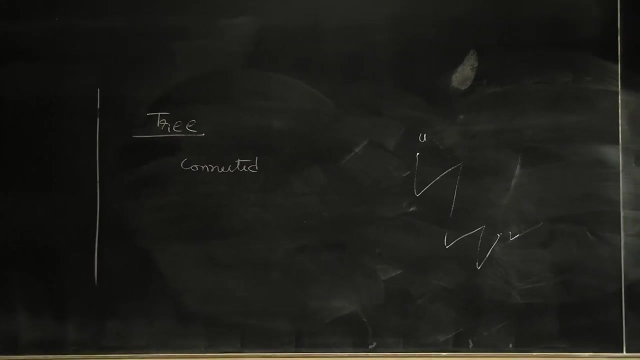 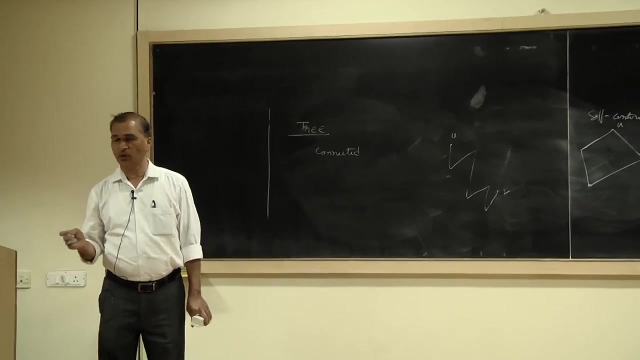 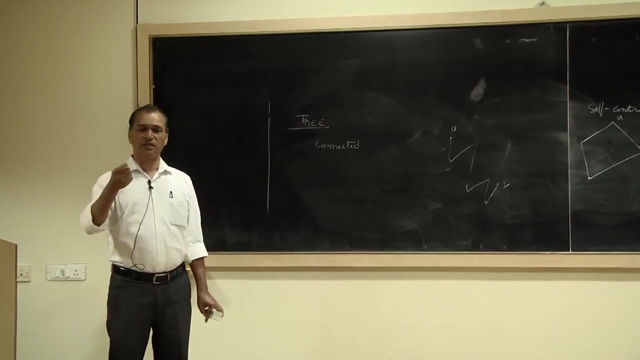 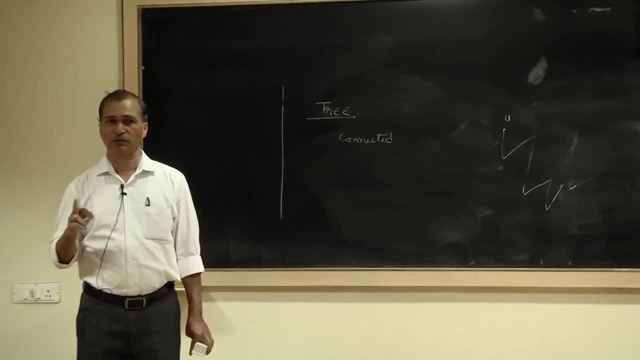 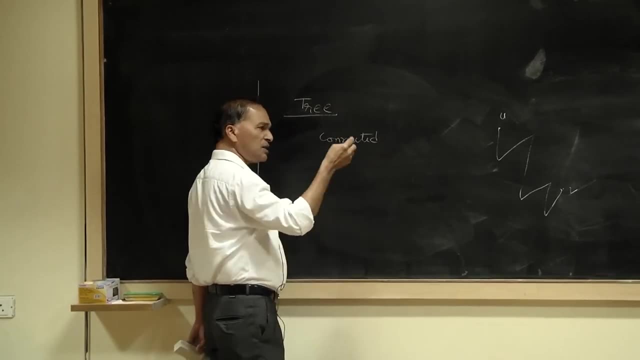 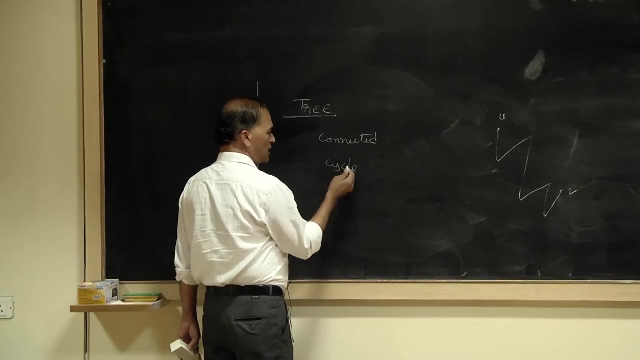 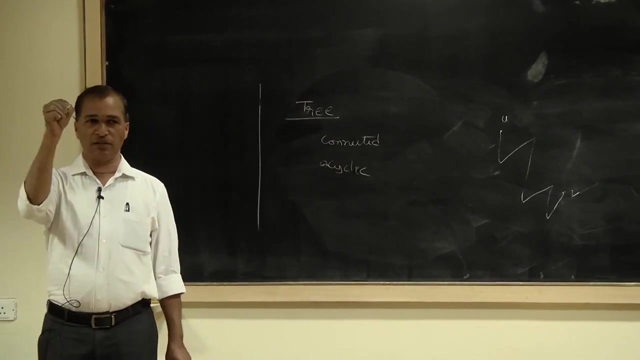 simplest one is: between every two vertices there is exactly one path. that is a tree. By definition, we say that it is a connected graph and because there should be only one path between every two vertices, it should not have a cycle. So we say that it is a cyclic. if we take a path and if the starting point is same as 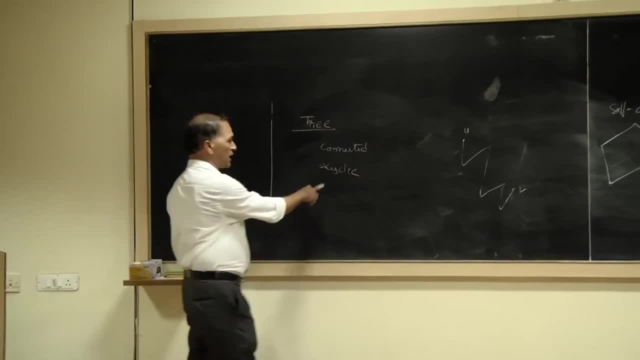 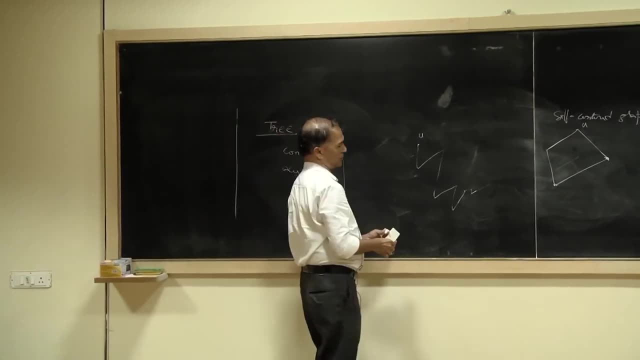 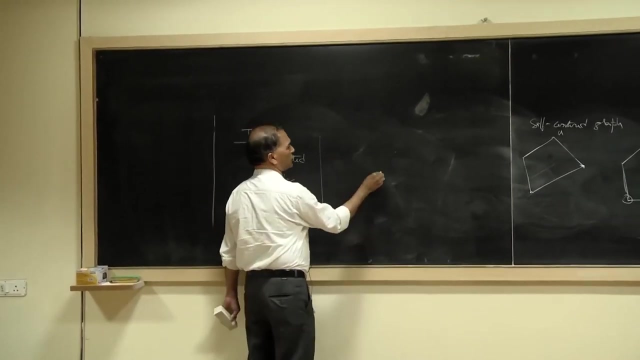 the end point, we say that it is a cycle. If the graph has no cycle and it is connected, we say that it is a tree. and there are many, many characterizations of tree. most important of them is that between every two vertices, there exists one and only one path. there exists a path and there exists one and only. 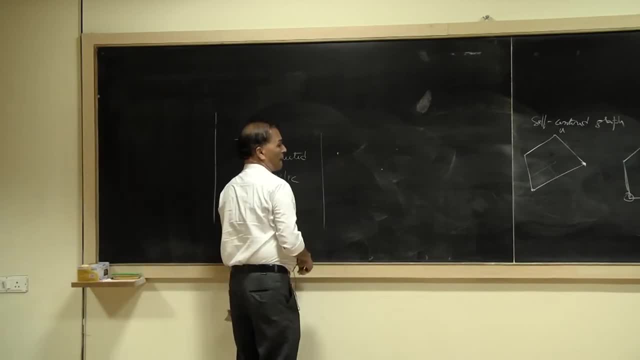 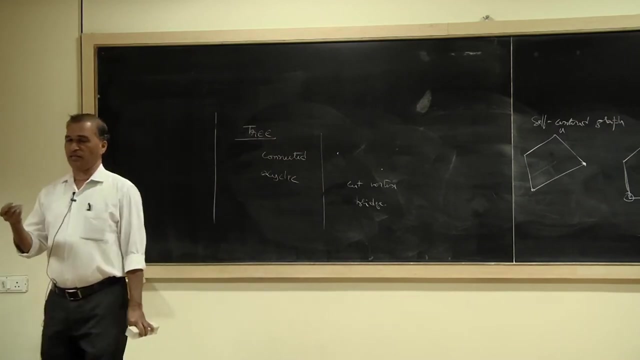 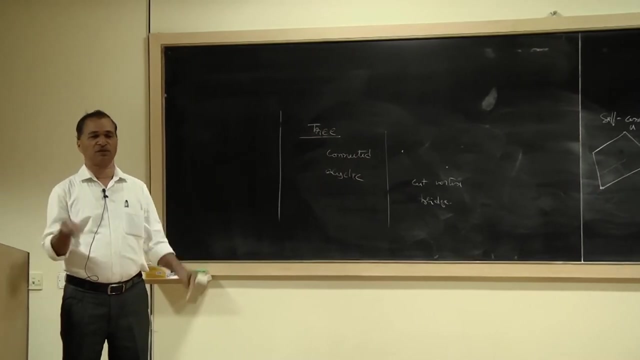 one path Maybe that we can define. We should. Let me show you so many things. this is: we can define a vertex, cut vertex and bridge. What is a cut vertex? It is a vertex such that removal of the vertex disconnects the graph. 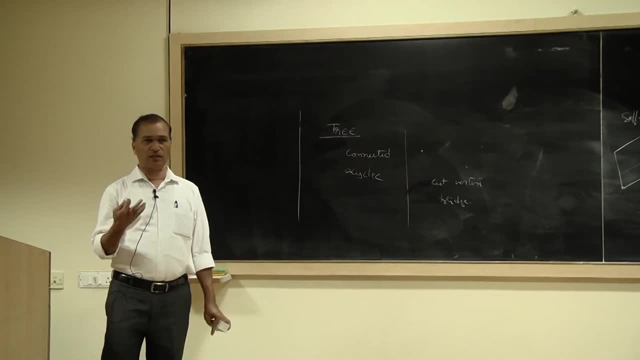 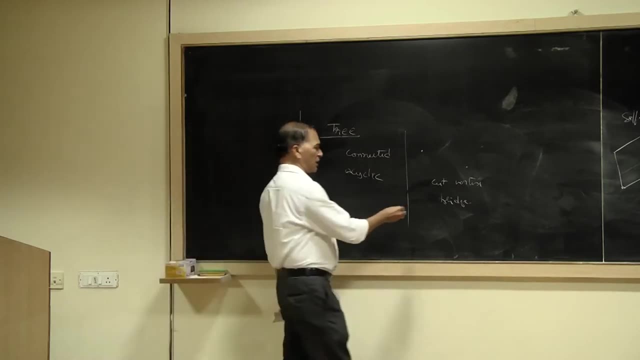 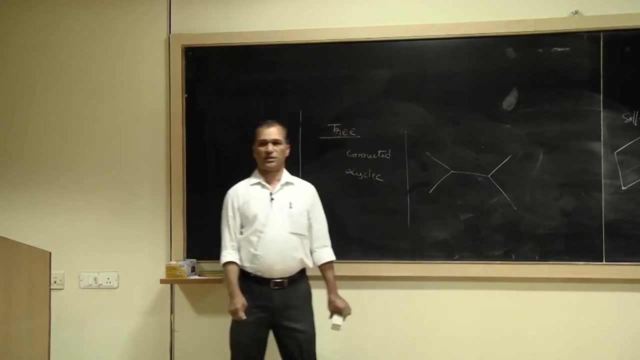 Suppose that we started with a connected graph. if G is a connected graph, a vertex V is called a cut vertex. if G minus V is disconnected, If G is a graph and edge E is connected. So what is a tree? A tree is a graph in which every edge is a bridge. every edge is a bridge you remove. 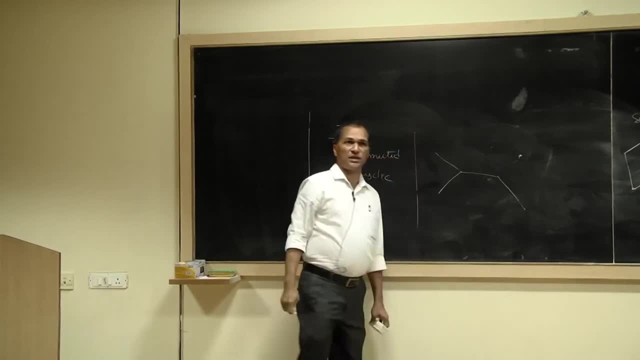 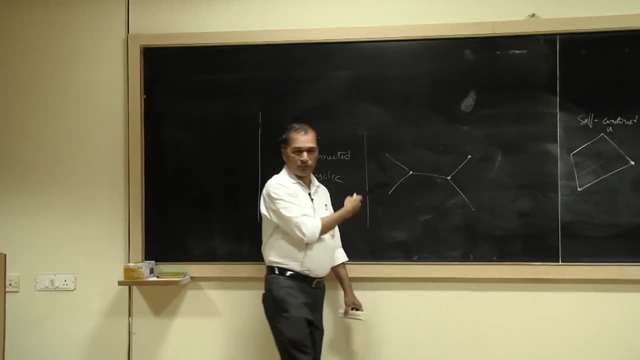 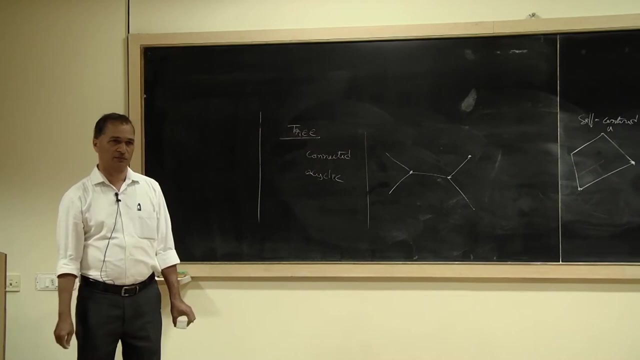 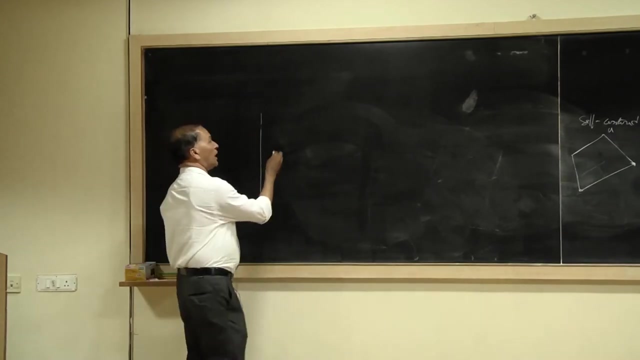 this edge, for example, then graph resulting graph becomes disconnected. And if you consider the vertices which are not end vertices, vertices which are not of the order of 1, every such vertex is a cut vertex Right. There are so many characterizations of tree and these are few of them. 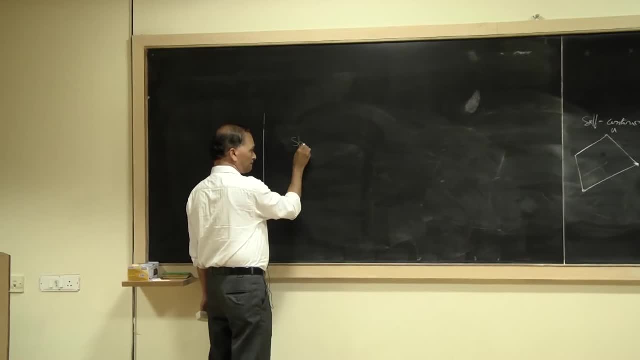 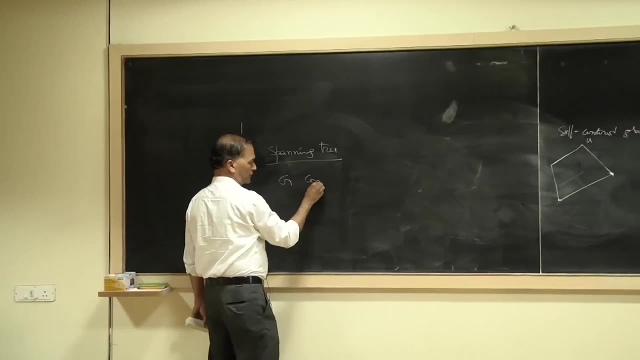 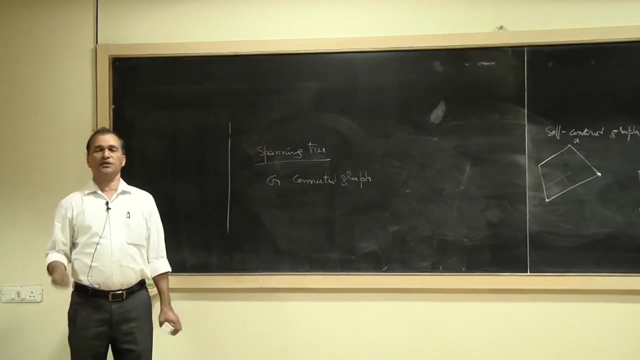 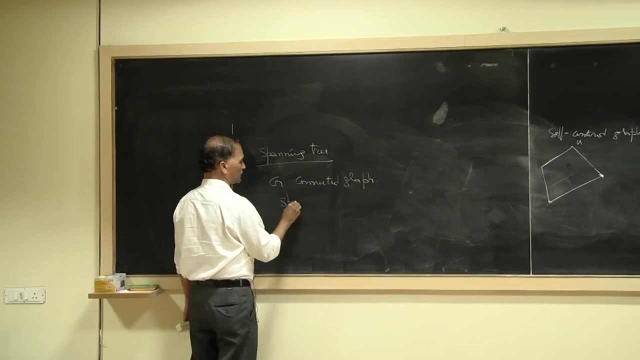 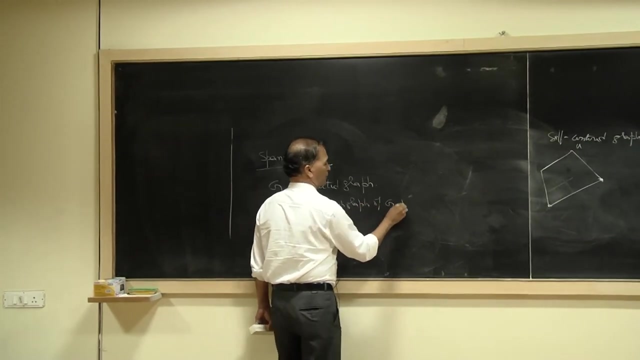 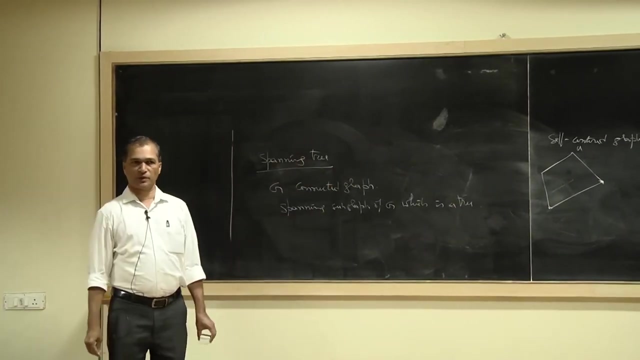 And next important concept is that of spanning tree. Let G be a connected graph. What is a spanning tree? It is a spanning sub graph. Let G be a connected graph, graph of G, which is a tree. Spanning tree is a spanning sub graph of G, which is a tree. 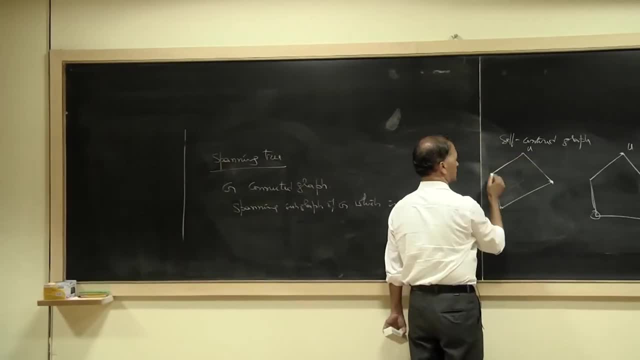 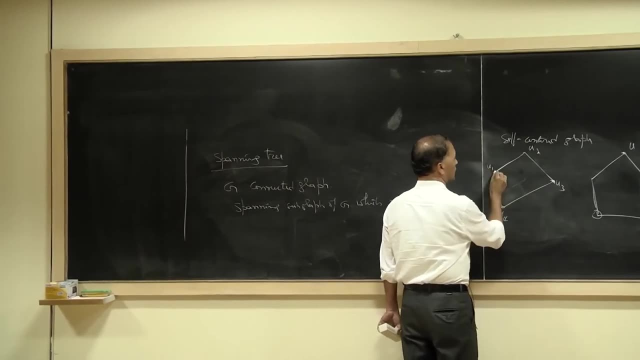 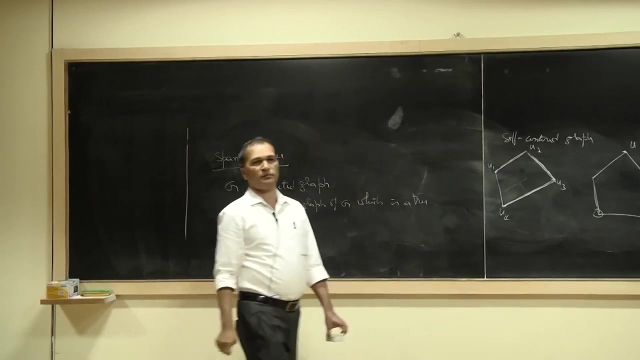 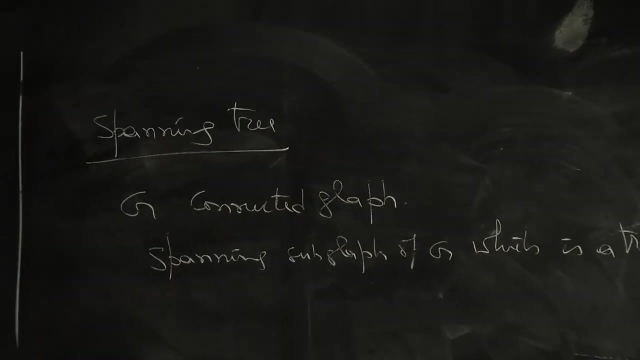 It should be a spanning sub graph and it should be a tree. for example, if you consider this graph, it is a connected graph. If you consider this as U1, U2,, U3, U4, then this is a spanning sub graph, which is a tree. Therefore, it is a spanning tree. One can easily observe that. 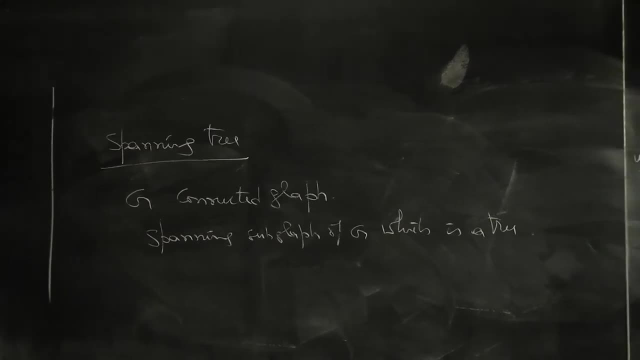 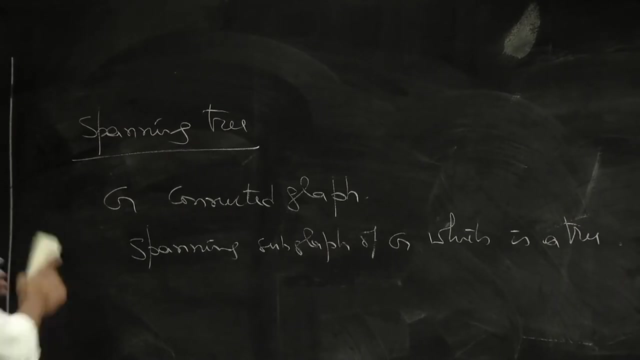 a very connected graph has a spanning tree, and converse is also true. If G is a graph which has a spanning tree, it has to be connected. So it is connected. we can say if, and only if, it has a spanning tree. If you take this: 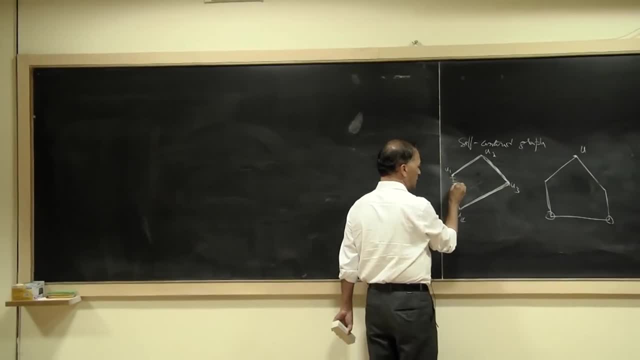 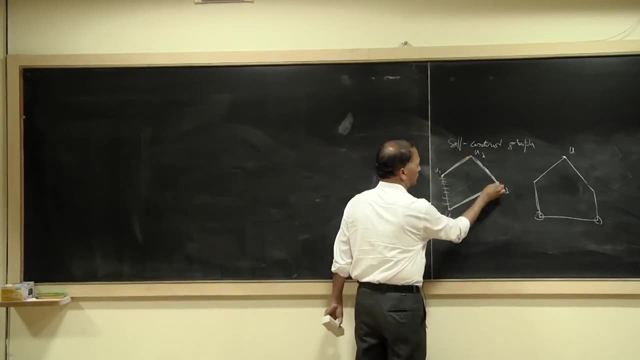 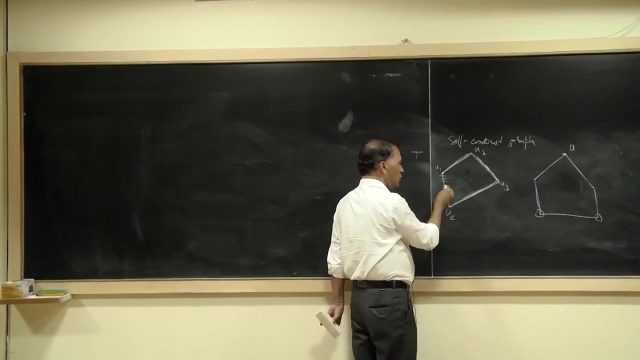 spanning tree and, with respect to this spanning tree, this is an edge which is not there in the spanning tree. These edges, which are edges of this particular spanning tree, are called branches, This edge which joins a vertex of the spanning tree to another vertex of spanning. 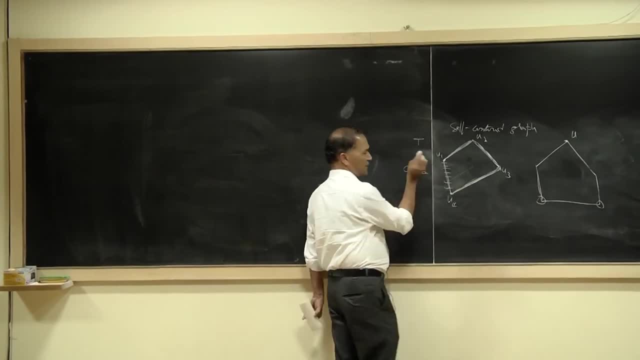 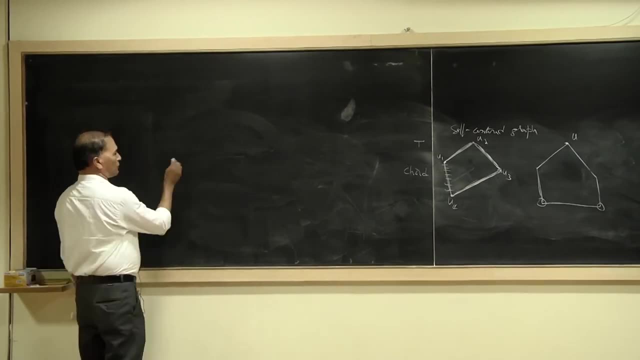 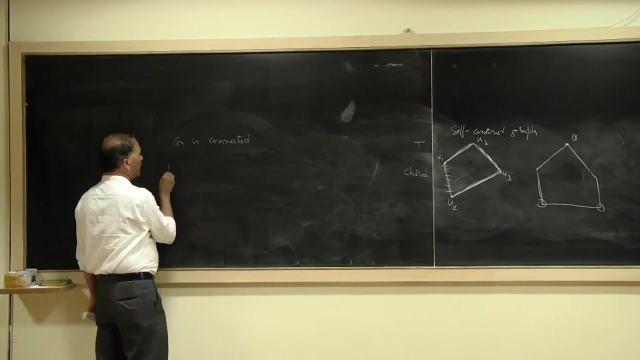 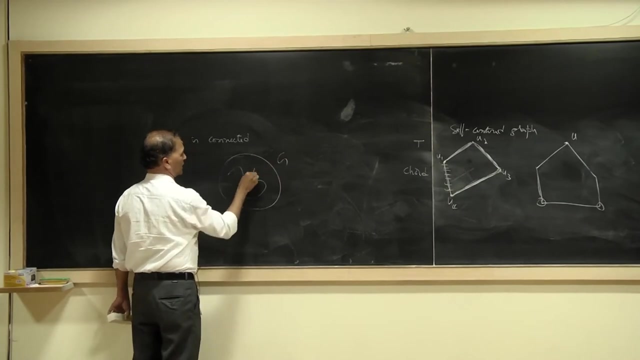 which is not there in the spanning tree is called a chord with the usual sense right. Suppose that G is a connected graph, G is connected, T is a spanning tree of G. we have the graph G and we have the spanning tree T. 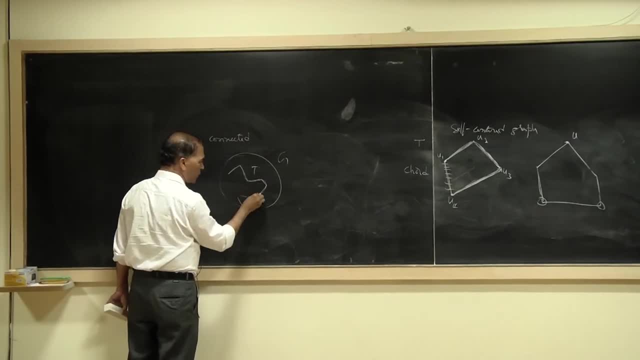 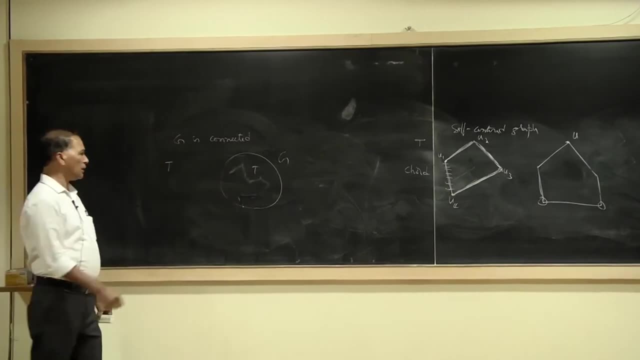 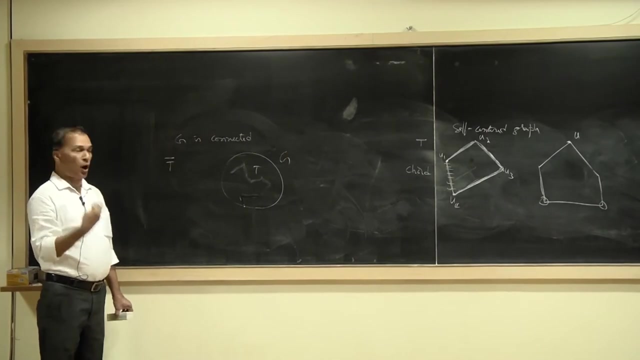 If you remove all the branches, all the edges of the spanning tree from G, we get a subgraph of G. these edges are removed, right, And that subgraph is denoted by T bar. T bar in the sense that it is the complement of. 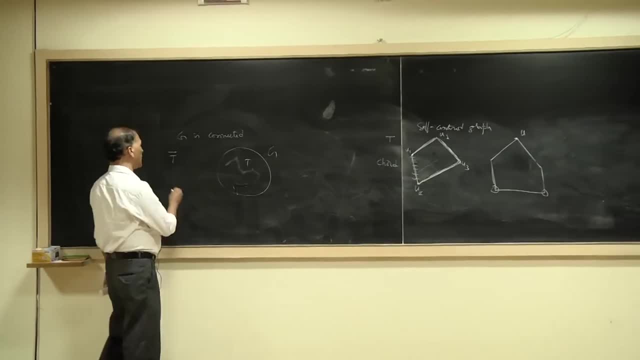 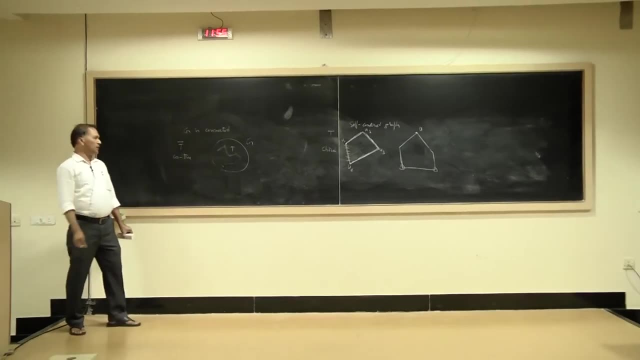 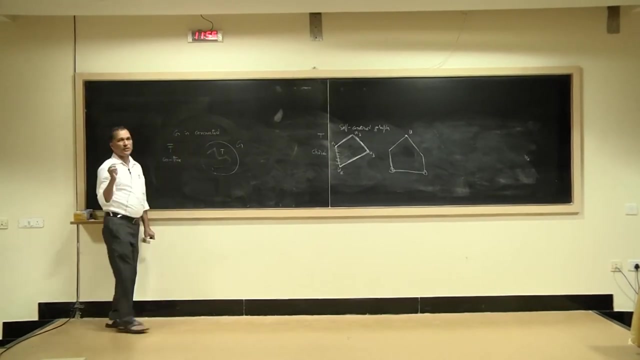 T in the graph G or with respect to the graph G and T, bar is called a co-tree, complement of the given tree, A co-tree. A co-tree is the graph obtained from the connected graph G by deleting the edges of a spanning tree in G. 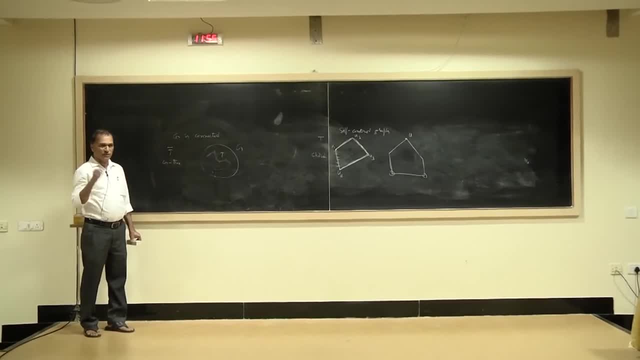 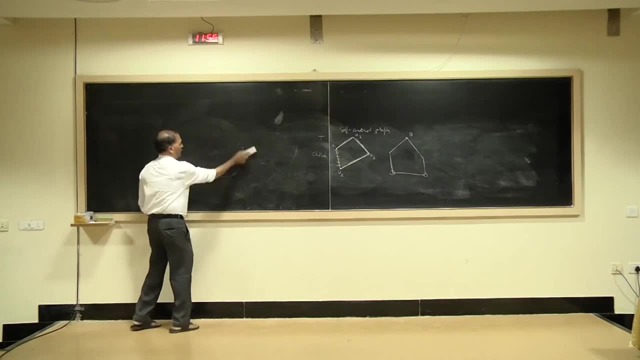 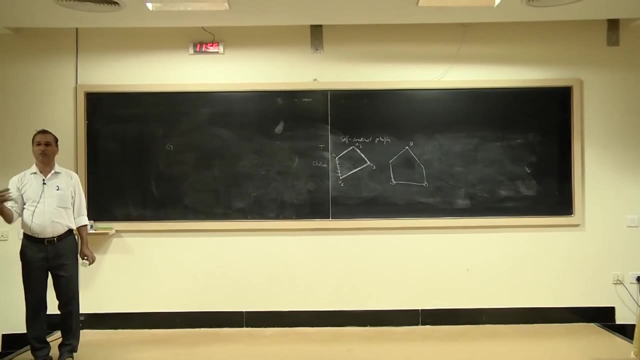 You take a spanning tree. delete the edges of the spanning tree from the graph. what you get is a co-tree. right Now we define a graph G. you remember, in complex analysis there is a concept called doubly connected. right, What is doubly connected? 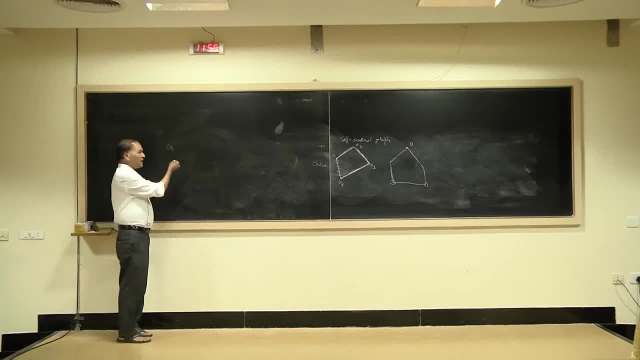 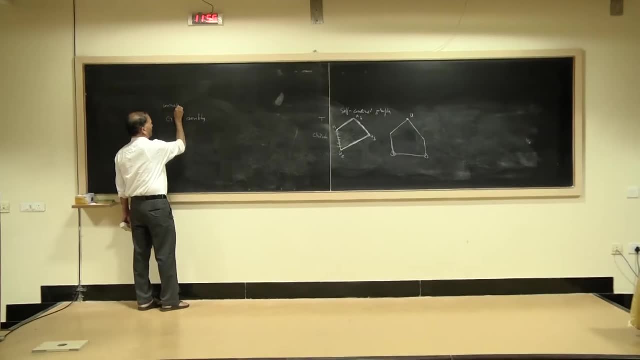 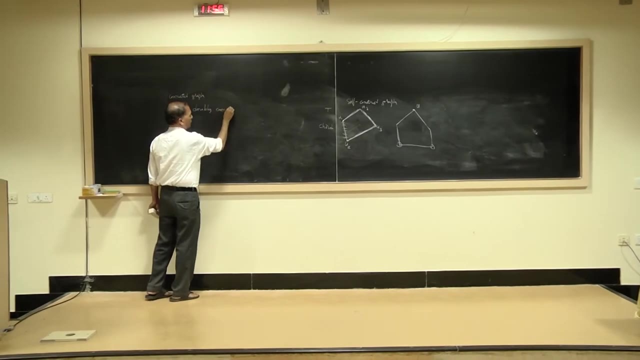 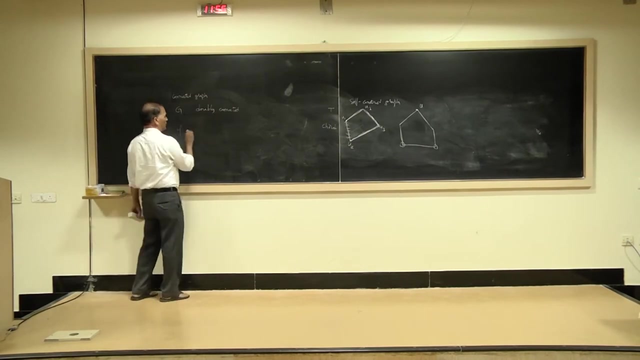 Let us not worry about what is doubly connected. in complex We define G to be a doubly connected graph. a connected graph, G, is doubly connected. We remember that every connected graph has a spanning tree right. doubly connected if there exists a spanning tree. 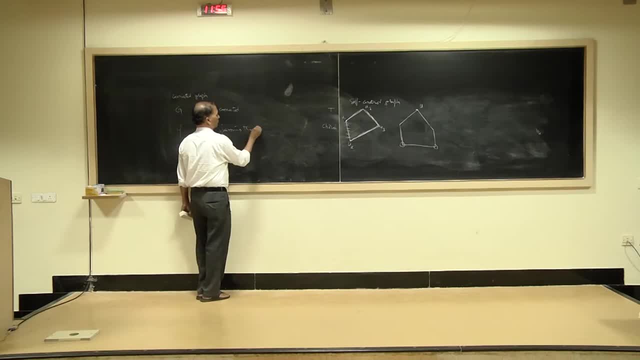 Right, So you say you define a corresponding value of a spanning tree of t, such that G minus t, that is equal to T bar, is connected. T bar also has a spanning tree, right? It need not happen always. if you take out the edges here, this is not connected. but 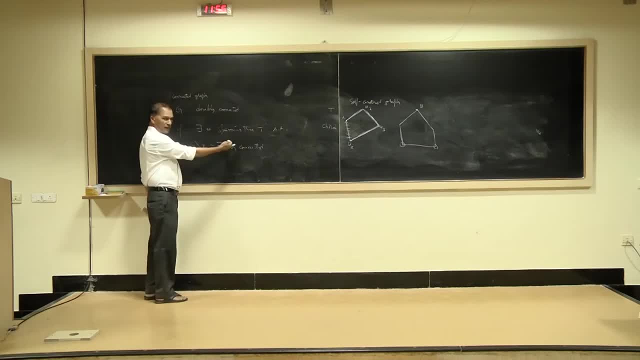 if there exists a spanning tree T such that G is not connected, such that T bar is connected, we say that it is doubly connected. say that it is weakly doubly connected. what is strongly doubly connected? If it is true that for every spanning 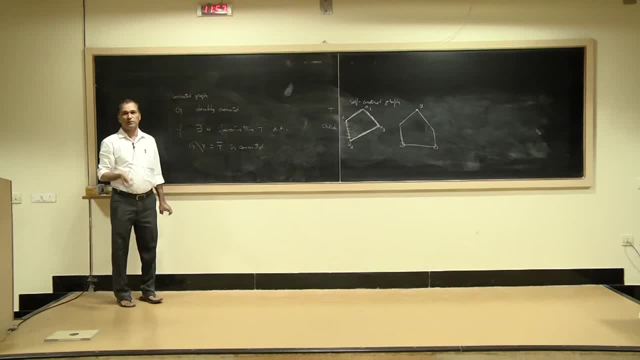 treaty T bar is connected, then we say that it is strongly doubly connected. right, These are new definitions. randomly I have taken: doubly connected is there in complex analysis. we can, I mean, expand it, extend it to this one. Can you give an example for 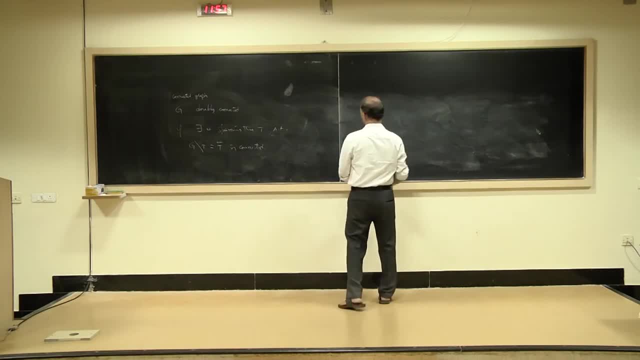 a weakly doubly connected graph and strongly doubly connected graph One can easily construct. in fact, if you take this graph, this is one spanning tree, right? If you remove this one, we should get T bar, We should get a spanning tree so we can make it connected. we can take this graph, this. 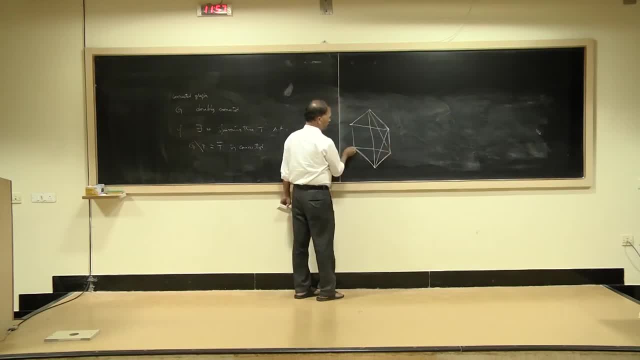 one, 2,, 3,, 4,, 5, one can construct, is it not? We can remove these edges. still, the graph is connected. as it is connected, it should have a spanning tree. therefore it is. this is weakly doubly connected. Can you give an example for a graph which is strongly doubly? 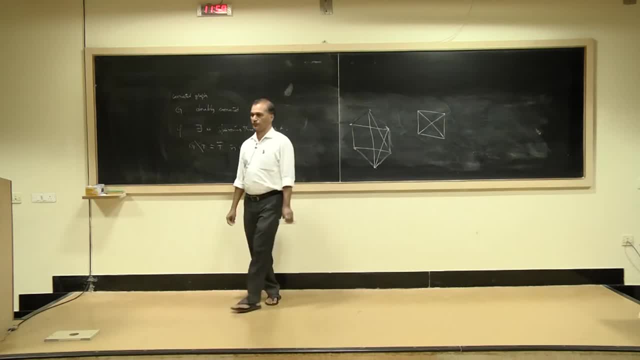 connected. Take this complete graph. you take a spanning tree. may be that you take this spanning tree, remove the edges of the spanning tree. what you get is again a spanning tree. therefore, it is connected. You take any spanning tree and remove the edges of the spanning tree. 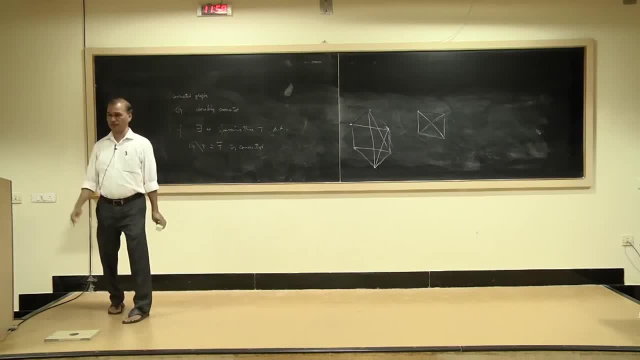 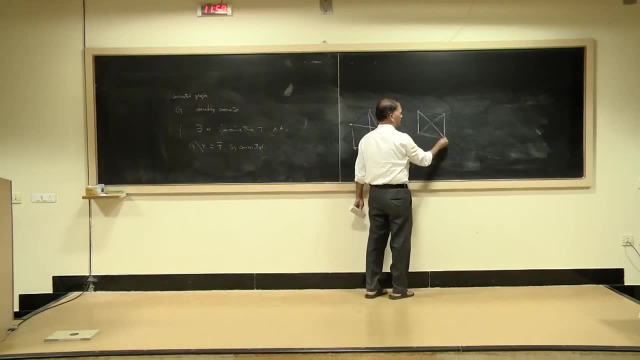 resulting is- again, it is true with every complete graph, because there are so many edges. If you take this spanning tree, Hmm, Hmm, This one, what you get, then this is gone, this is gone. this is gone. this is not a. 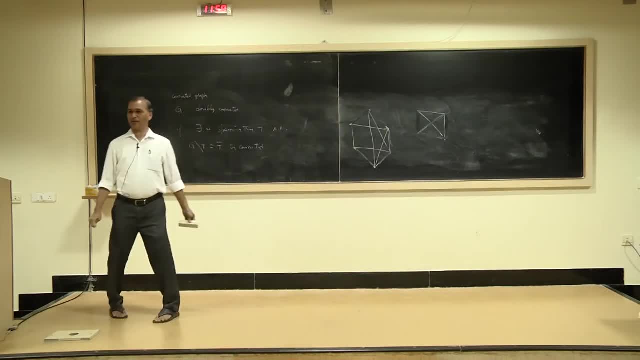 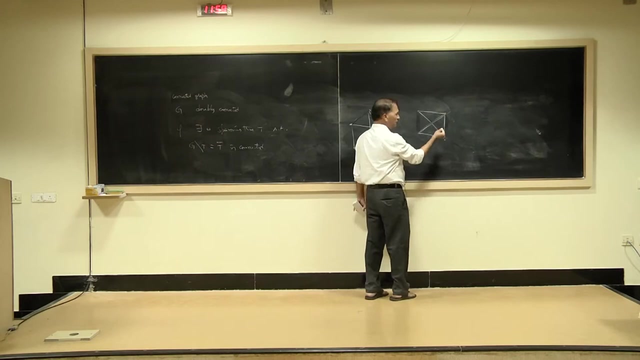 spanning tree, but it is connected. T bar is connected. it has a spanning tree if you remove the edges. So that is not the example. So try to get an example such that for every tree, T G minus T, T bar is again connected right Here, if you remove this tree, it is connected. if 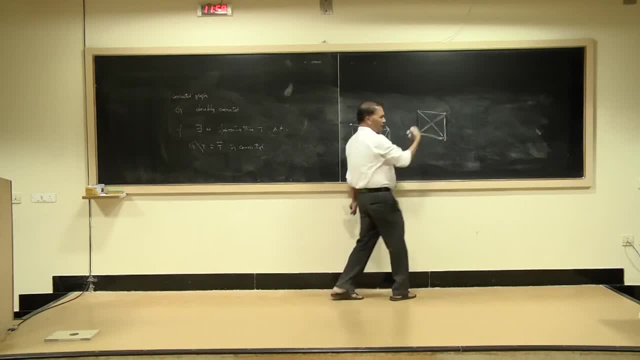 you remove this tree, it is connected right, except for may be this one. if you remove the edges of this one, that two vertex becomes disconnected, Hmm, Hmm, Isolated, and it is not. So you can think of characterizing a weakly doubly connected. 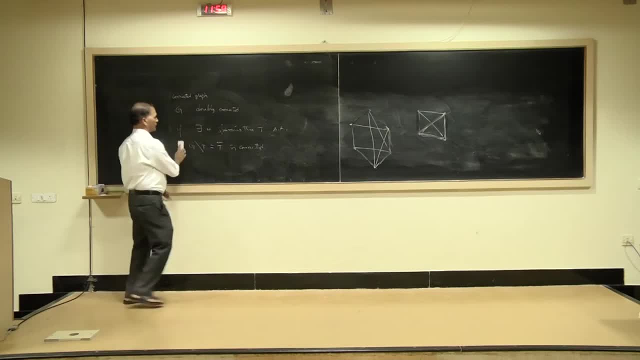 graph and strongly doubly connected graph right A tree, is a particular type of general graph which is called a bipartite graph. Hmm, Hmm, Hmm. What is a bipartite graph? A graph G with a vertex set V and edge set E is called a. 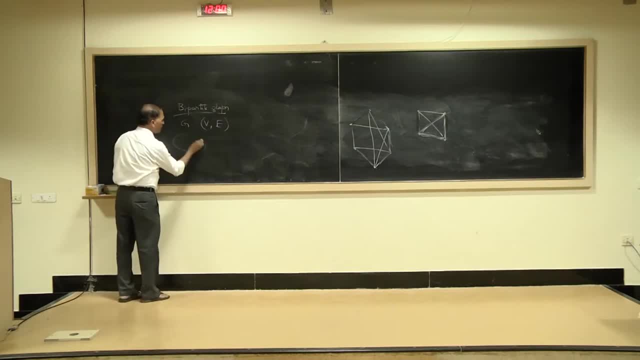 bipartite graph if the vertex set can be partitioned into two sets, say V 1 and V 2, such that every edge has one end vertex in V 1 and other end vertex in V 2.. A bipartite graph is a graph vertex set of which can be partitioned, say V 1 and V 2, such 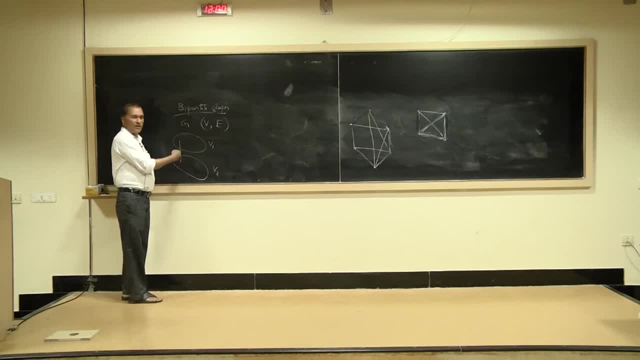 that every edge is in between V 1 and V 2.. Equivalently, no two vertices in either V 1 or V 2 are at distance 1.. No two vertices are at distance 1 means what they are not never adjacent right. So any vertex you take, all the vertices will be at distance 1.. So 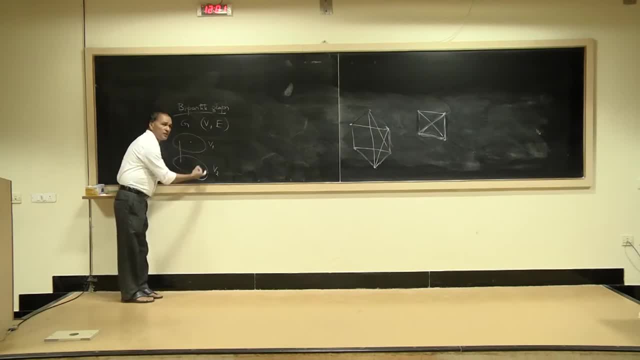 any vertex you take, all the vertices will be at distance 1.. So any vertex you take, all the vertices which are adjacent to this vertex are in V 2.. Same is the case with any vertex in V 2, all the vertices which are adjacent to that are in V 1, right. 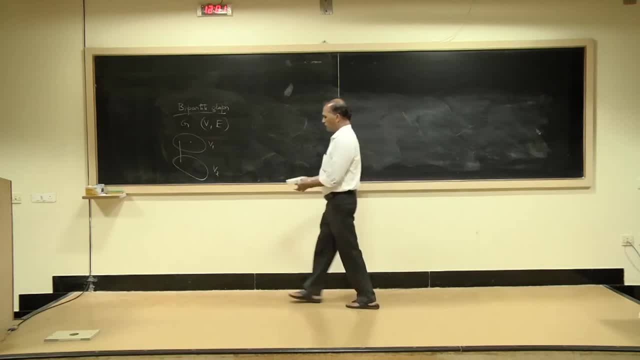 A tree is a. one characterization of bipartite graph is that every cycle is of even length. A graph G is bipartite if, and only if, all of its cycles are of even length. If we take a tree, there is no cycle at all. We can say that length of the cycle is 0. So we can. 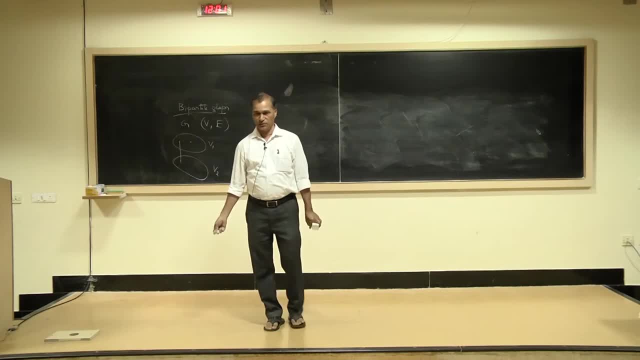 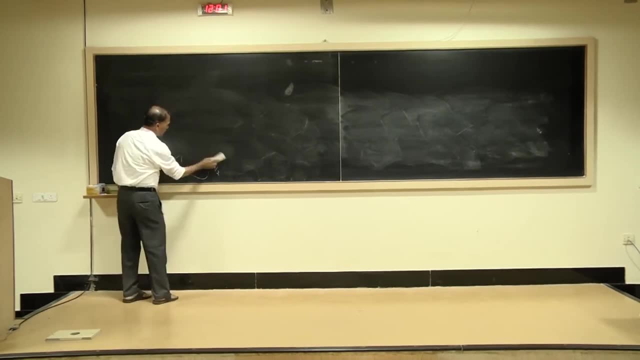 say that length of the cycle is 0.. So we can say that length of the cycle is 0.. Which is an even integer. Which is an even integer. So every tree is a bipartite graph. Bipartite graph is one. 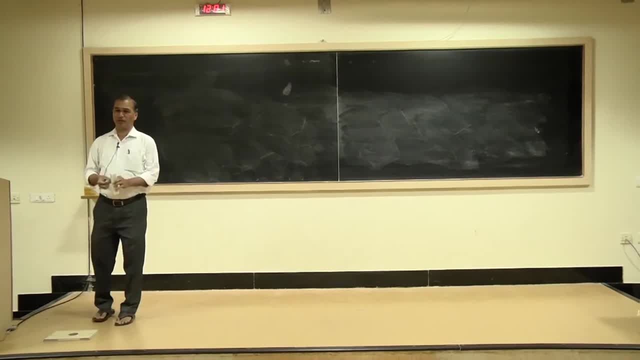 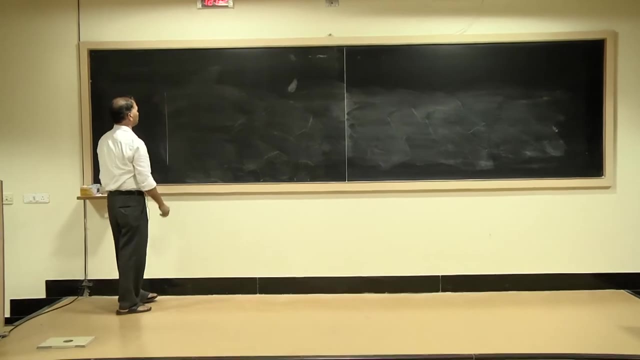 of the most important graph maybe, on which there are many theorems, using the adjacency graphs, adjacency matrices or incidence matrices, right? Maybe that next concept required is like this: That A has cells in between, You have volley contracts, brackets, batt substructures, These 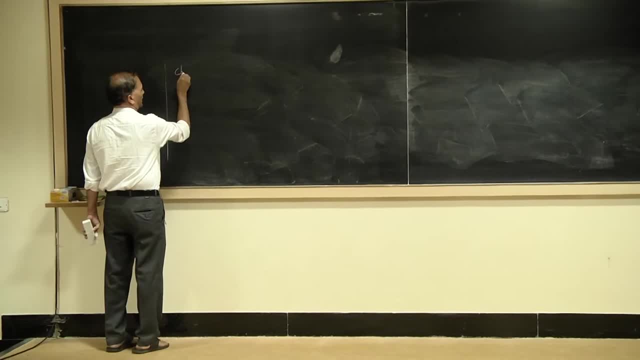 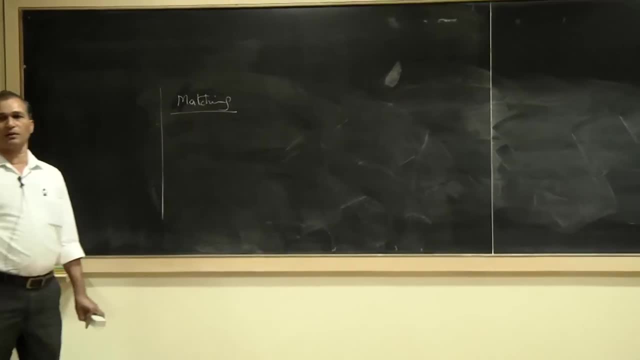 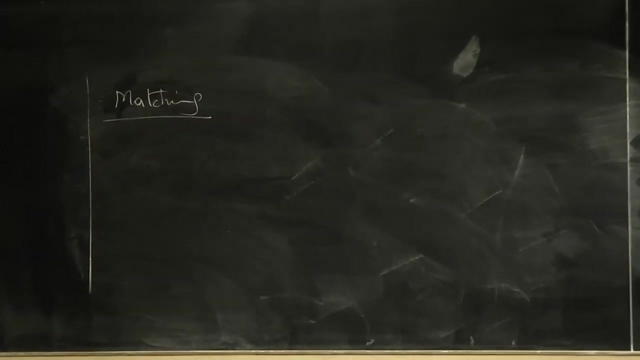 are on branches of tree And B perfectly egalitarian along the entire tree, дерев, mindset, all together Chromatic, or we can say matching chromatic number. we can take it afterwards. What is a matching in a graph? A matching in a graph is a set of edges which are independent. 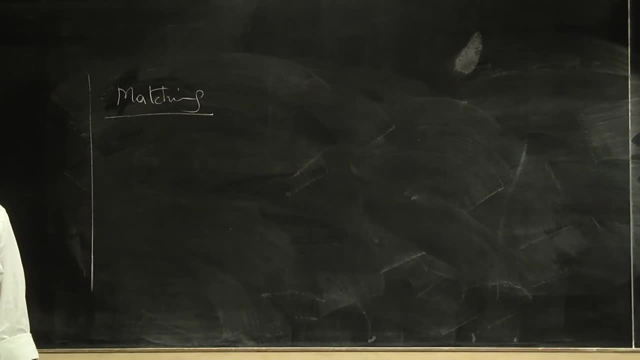 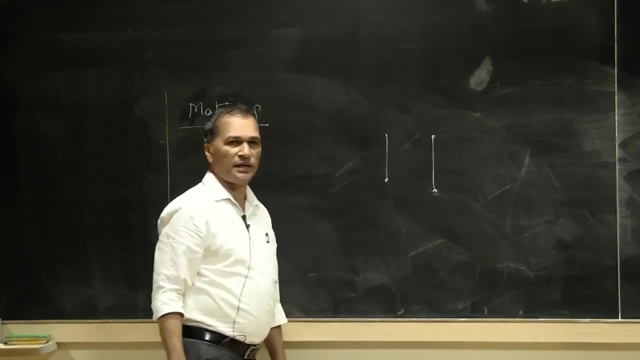 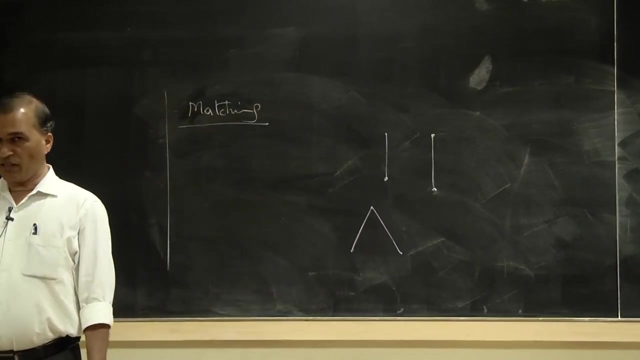 When do you say that two edges are independent? If they do not have any vertex in common. For example, if we take consider these two edges, they are independent. If we consider these edges, they are not independent. Right, A set of edges is said to be independent if no two of the edges in the set have a point. 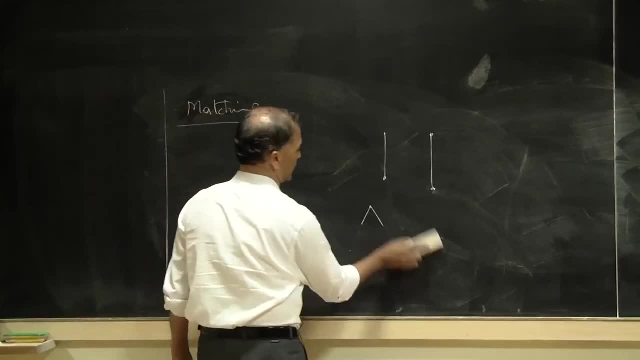 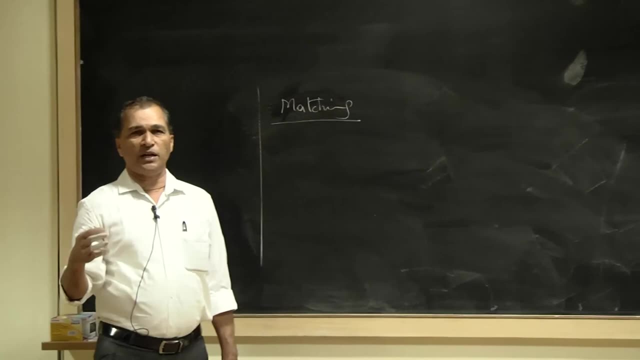 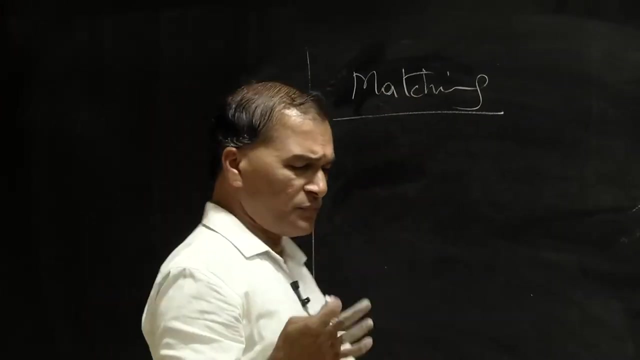 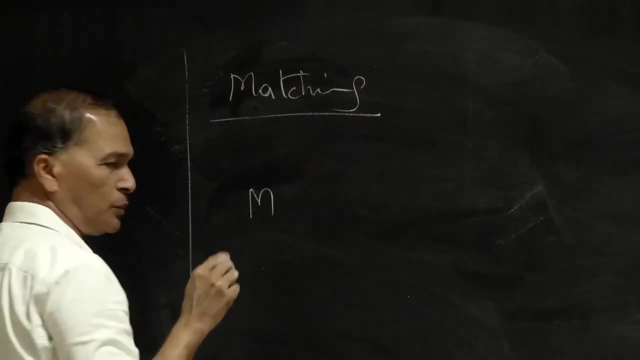 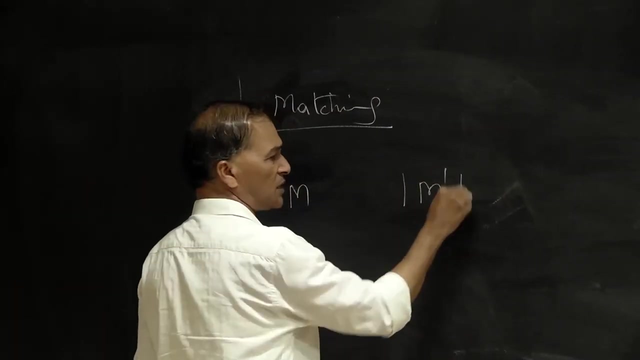 in common: Right Edges in the set are all independent. every two edges are independent. So a matching is a collection of independent edges. Right A matching: the size of the matching is nothing but number of edges in the matching. A matching m is said to be a maximum matching. if there is no matching m, dash such that number. 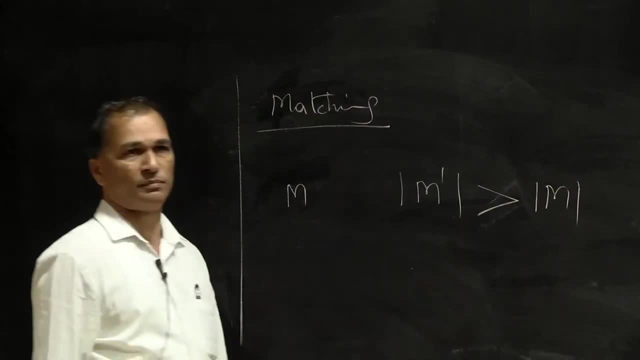 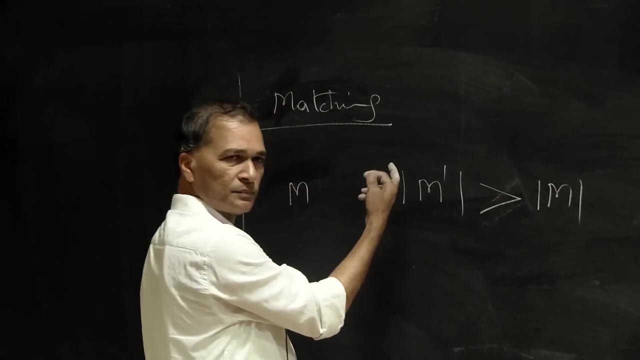 of edges in m dash is greater than number of edges in m. Right. Size of m dash is greater than size of m. There is no such m dash. If we take any other matching, the size should be less than or equal to size of m. 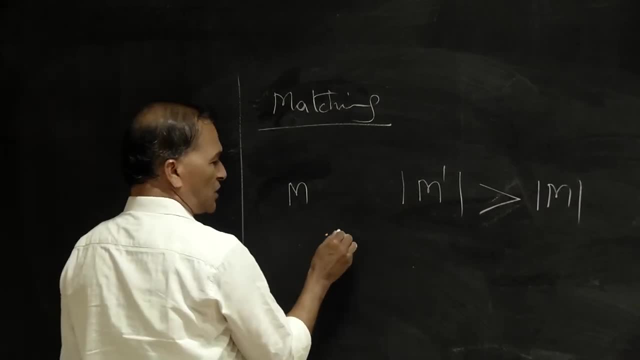 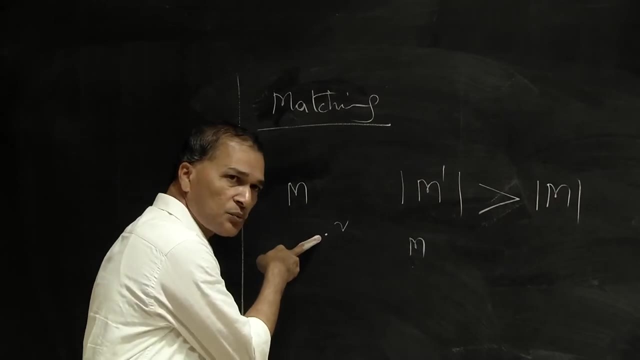 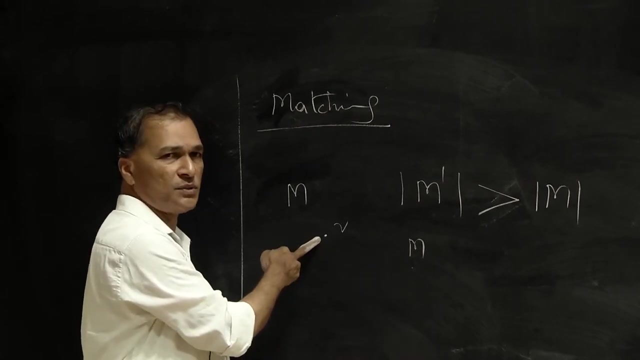 Right. If we take a vertex v and a matching m, we say that the matching m saturates this vertex v. if there is an edge of m, which is incident on this vertex v, Right, A vertex v is said to be saturated, Right. 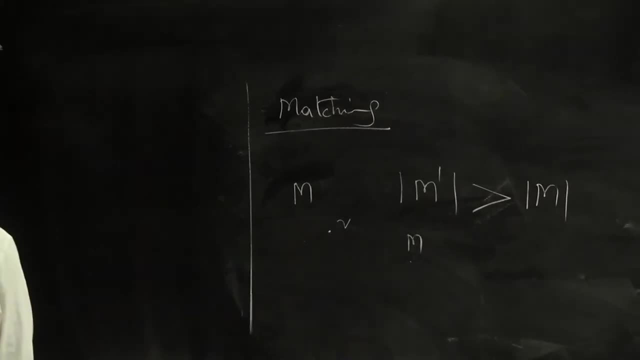 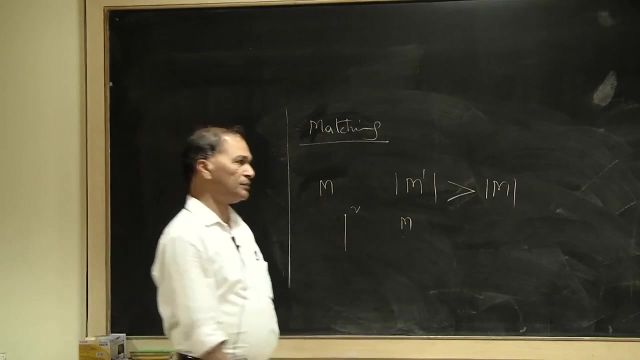 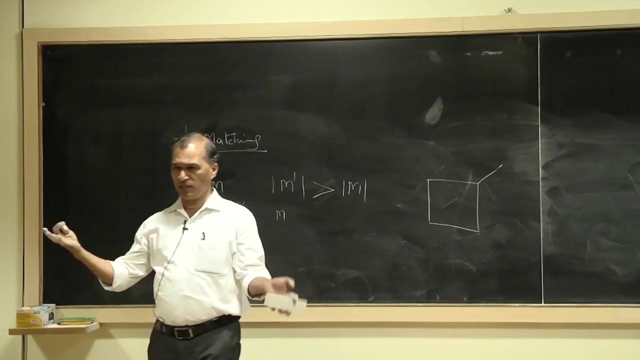 A vertex v is said to be saturated Right. A vertex v is said to be saturated with respect to a matching m. if there is an edge in m which is incident on the vertex v Right. Every graph has a maximum matching. We can take all the matchings and find out the matching with maximum number of edges. 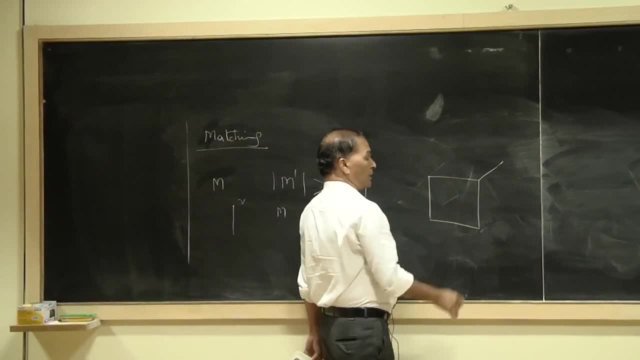 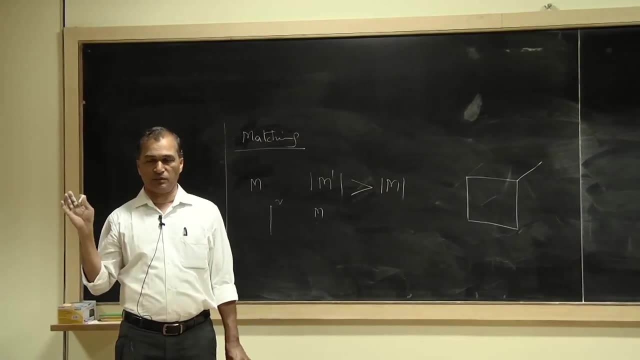 in it. So every graph has a maximum matching. A perfect matching is a matching which saturates all the vertices of the graph. A matching is said to be perfect. A matching is said to be perfect if it saturates all the vertices of the graph. 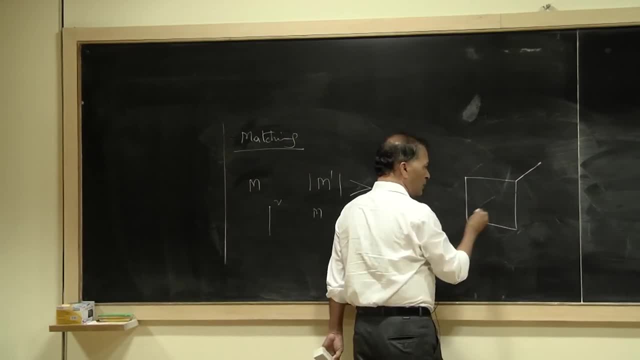 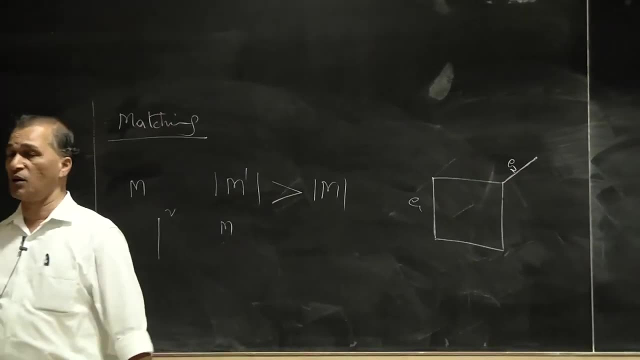 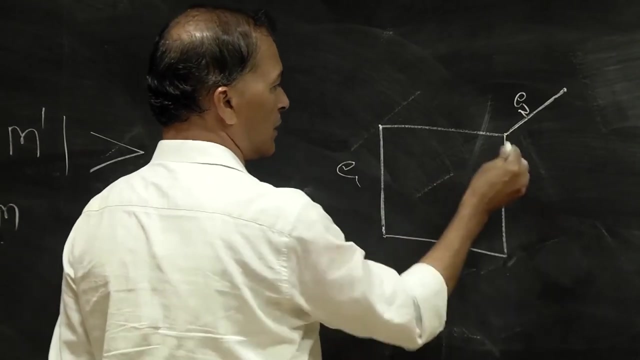 For example, if you consider this graph, if you consider this and this, it is a maximum matching. If you take E1, E2, it is a maximum matching. You cannot find a matching with more number of edges, Right, But it is not a perfect matching in the sense that this vertex is not saturated by any edge. 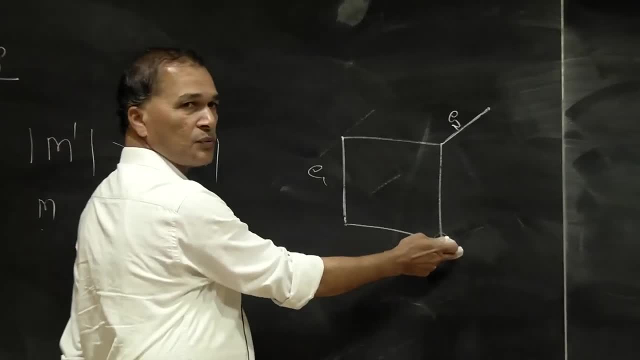 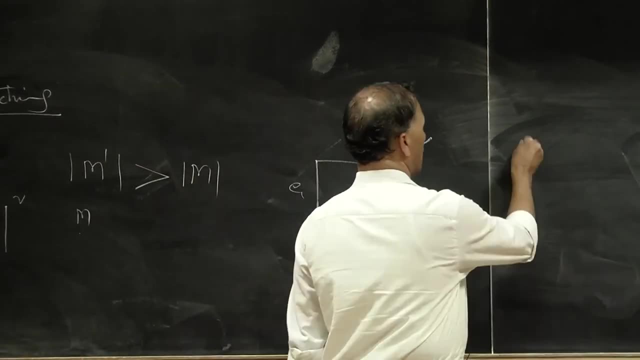 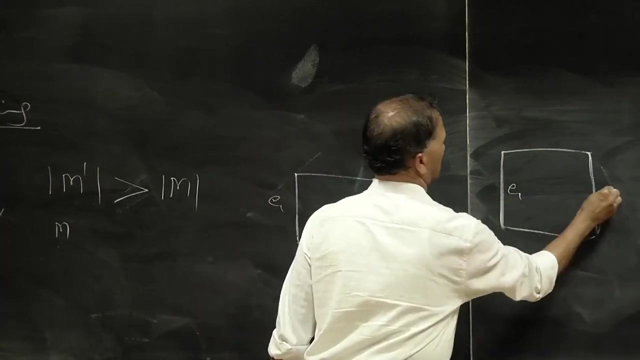 of the matching. There is no edge which is incident on this vertex Right. Therefore, it is a maximum matching, which is not a perfect matching. If you consider this one, this is a perfect matching: E1, E2,. it saturates all the vertices. 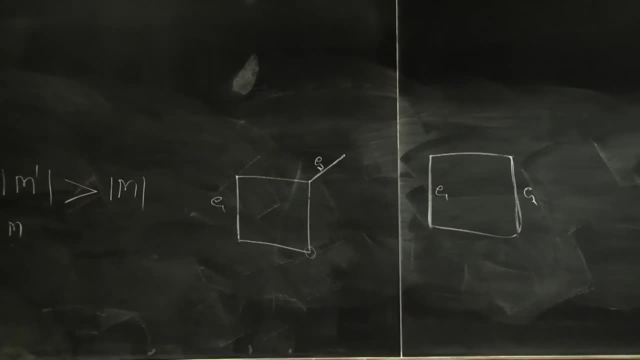 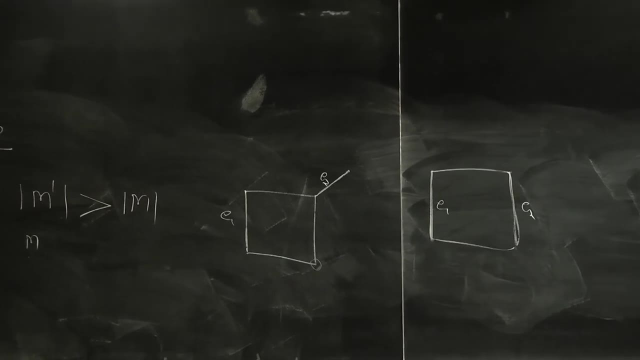 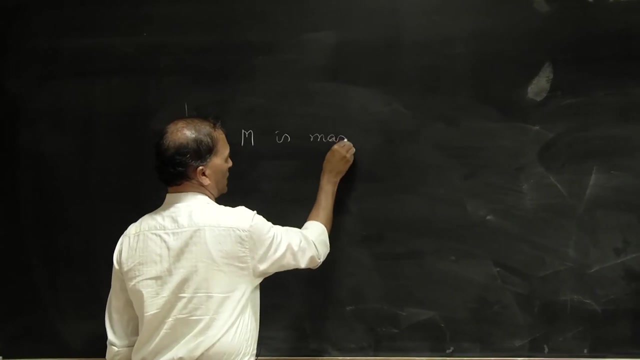 Right. Then the question is how to decide whether a given matching is a maximum matching or not, Right? So there is a theorem which says that Right, Yes, G is a connected graph, M is a matching of G, then M is a maximum matching. 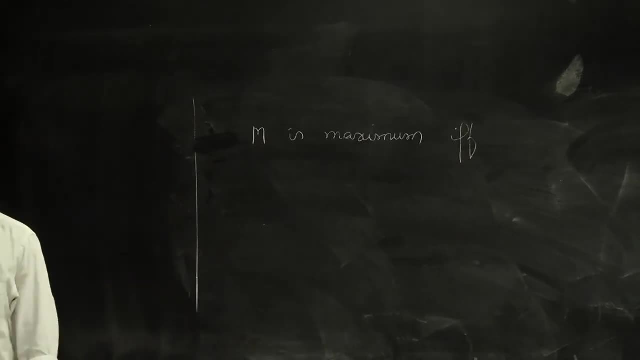 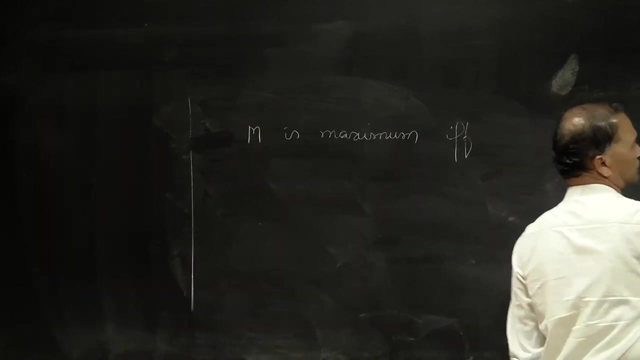 If, and only if, maybe that before that we have to define M argumenting sequence Right? What is an M alternating sequence? Suppose that M is a matching. there are some edges. consider G minus M. Let it be M dash. 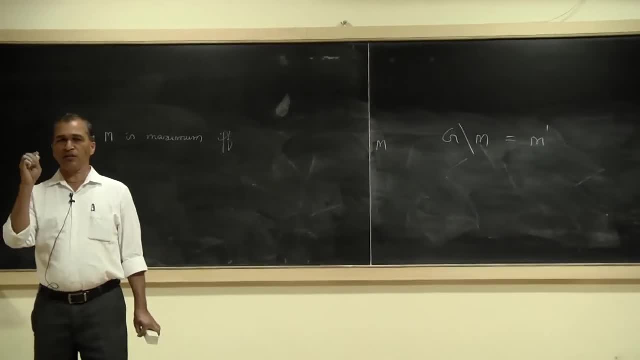 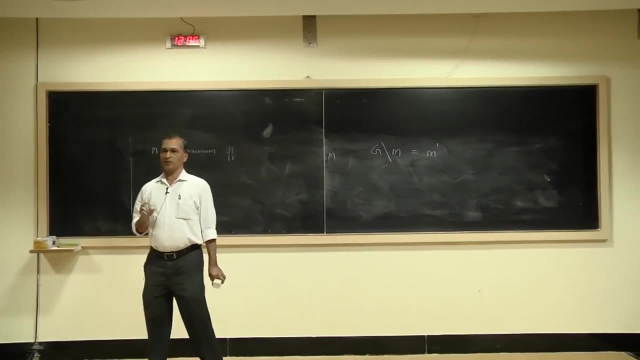 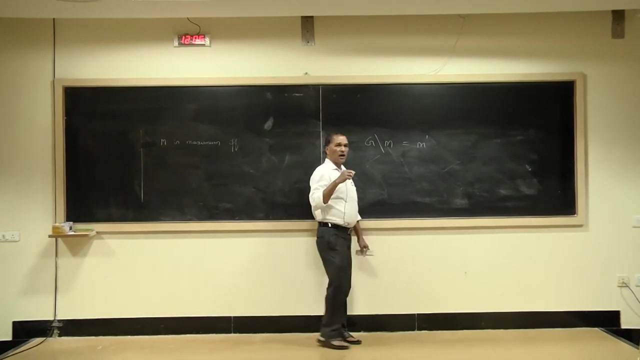 What is G minus M? All the edges of G which are not in M complement of M Right An M. alternating sequence is a sequence of vertices and edges where edges are alternatively in M and M dash. M dash is G minus M. 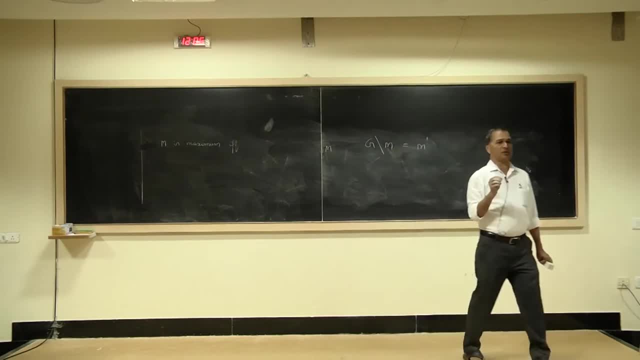 Right. An M alternating sequence is a sequence of vertices and edges Right. So M is a matching If and only if. maybe that before that we have to define M argumenting sequence is a sequence of vertices and edges starting with a vertex, ending with a vertex where the edges are. alternatively, 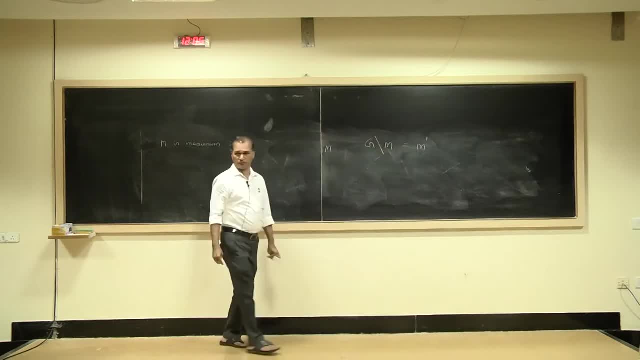 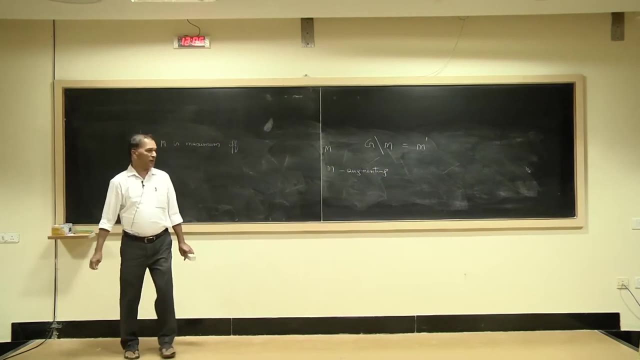 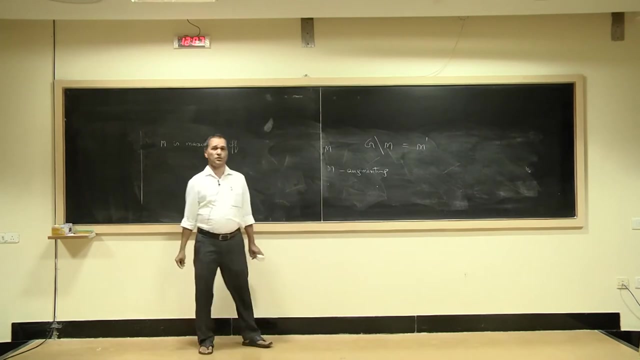 in M and not in M, In M and in M. dash Right. If you consider M alternating sequence, it is called an M argumenting sequence Is called an M? M argumenting sequence If, If the starting vertex and the last vertex, ending vertex are M unsaturated. 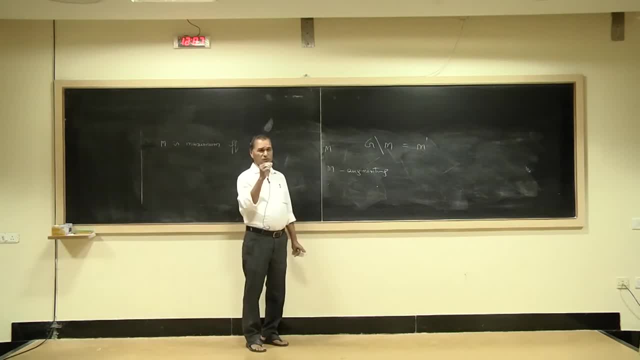 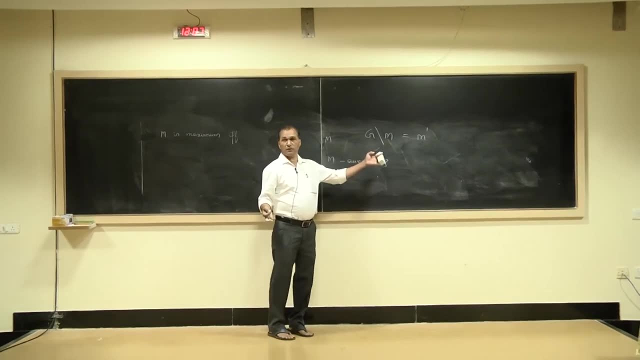 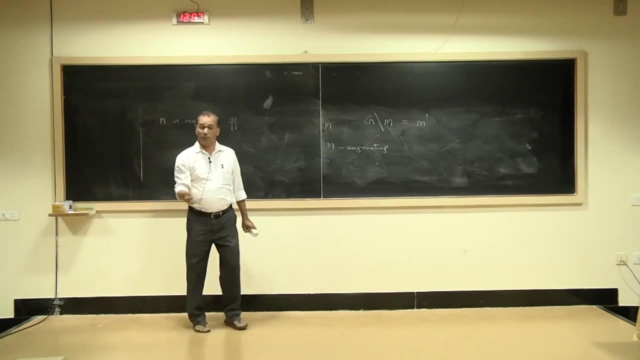 It is M alternating sequence, that is, it is a sequence which starts with a vertex, ends with a vertex and, alternatively, edges are from M and M dash. and there is an addition condition: that the starting vertex and the ending vertex are M unsaturated. M unsaturated means what? 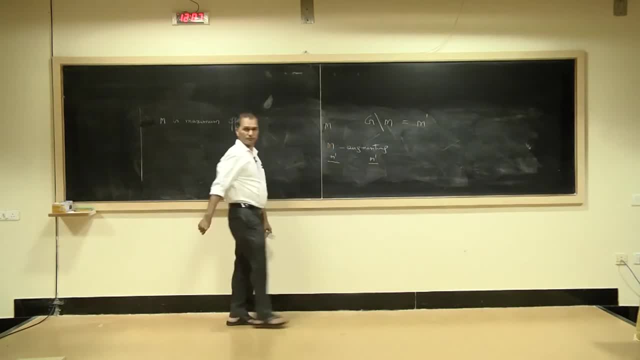 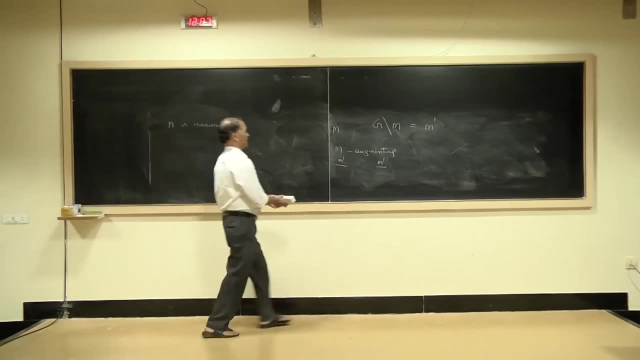 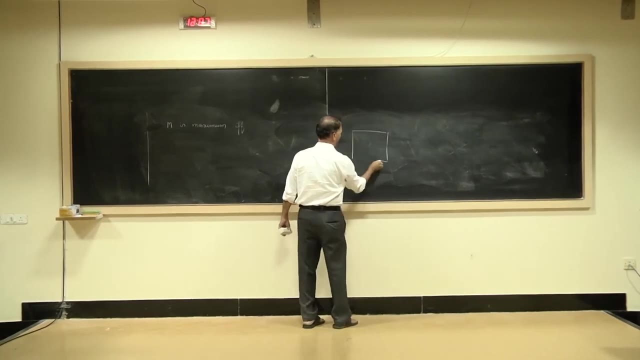 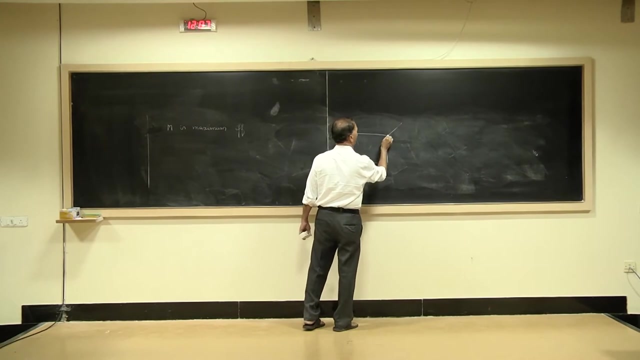 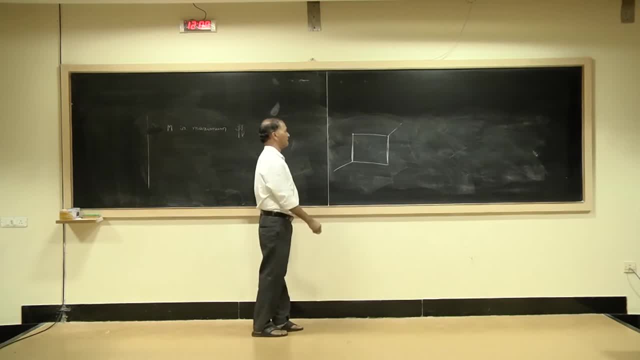 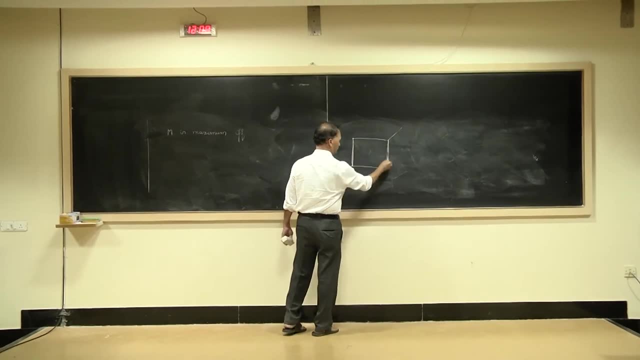 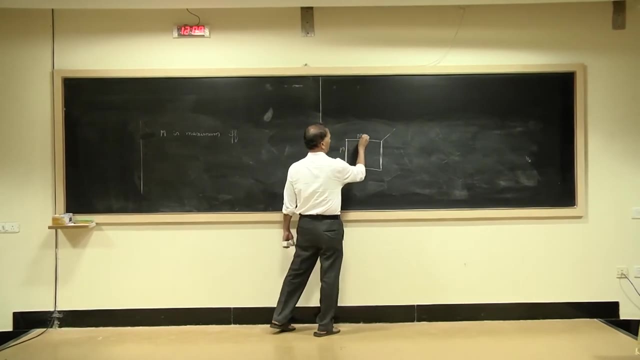 M saturated, M saturated And this is M matching. And if you take this from M dash, this from M, this from M dash, It can take this. It is a M argumenting path: Starting M, Starting M, Starting M. 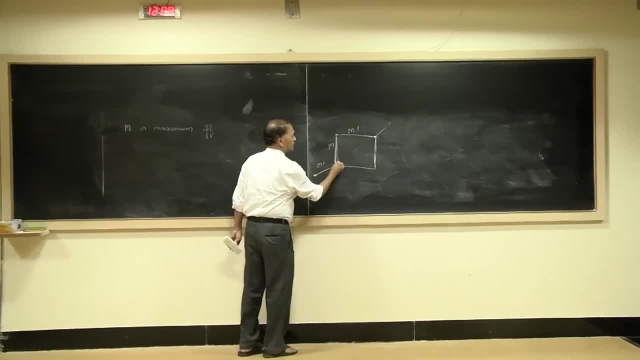 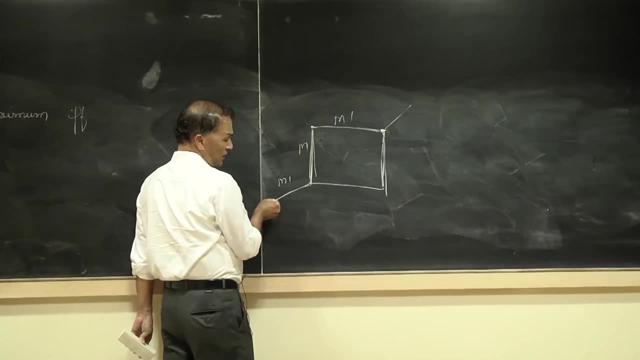 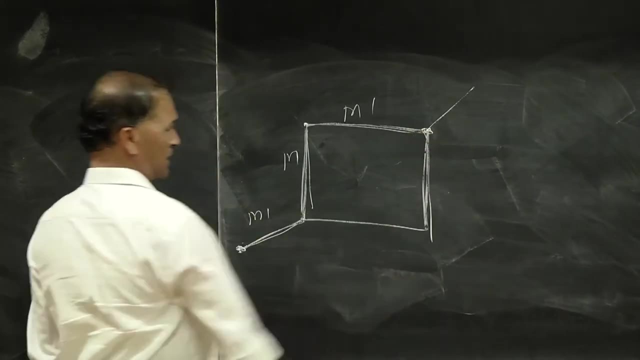 path starting from M dash. this is M unsaturated. this is my matching. You do not need to use all the edges of the matching You can take. this is M unsaturated. it is M dash edge of M dash. this is an edge of M. this is an edge of M dash. so this also M unsaturated. 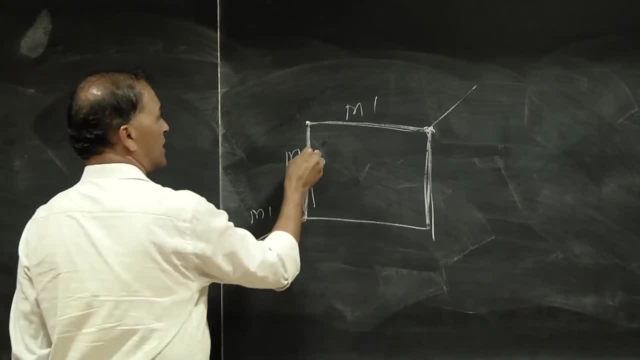 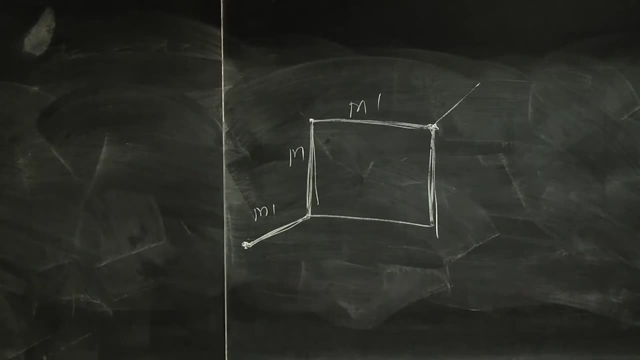 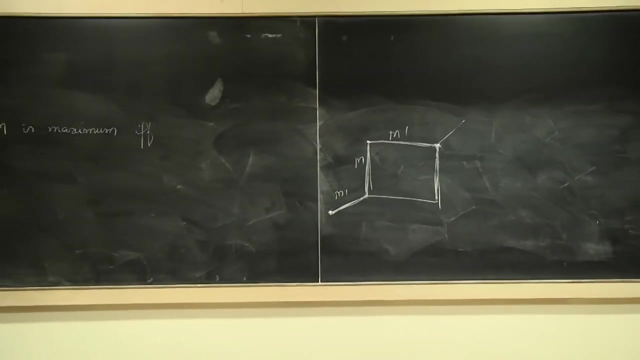 It is a sequence of edges where the edges are, alternatively, from end M M dash. If the starting edge and the last edge are from M dash, that equivalently starting vertex and the last vertex, ending vertex, are M unsaturated, then we say that it is a M argumenting path. 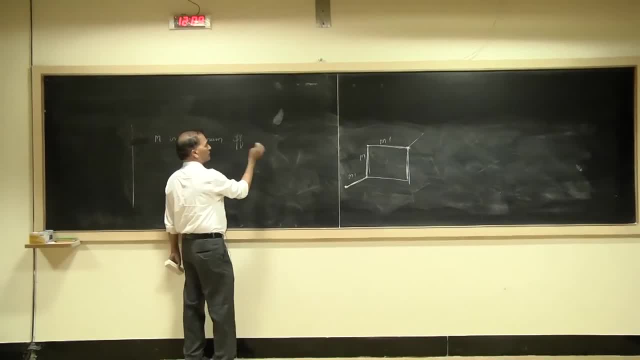 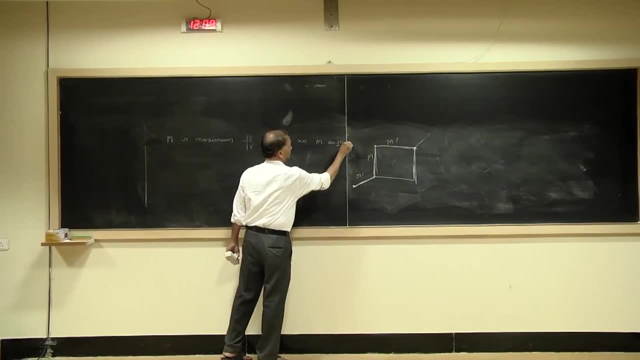 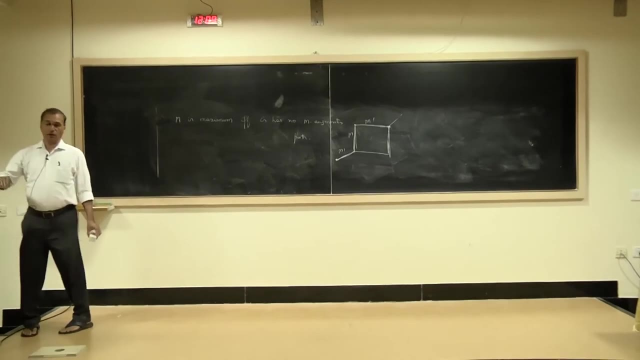 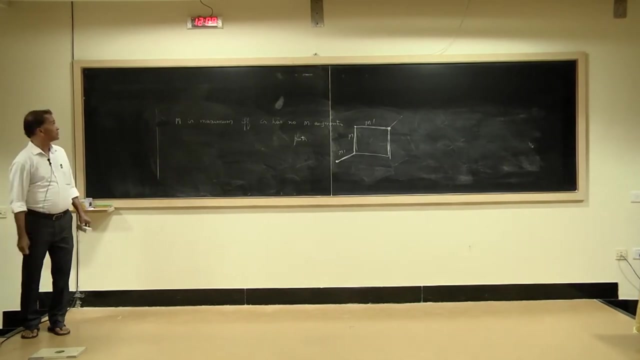 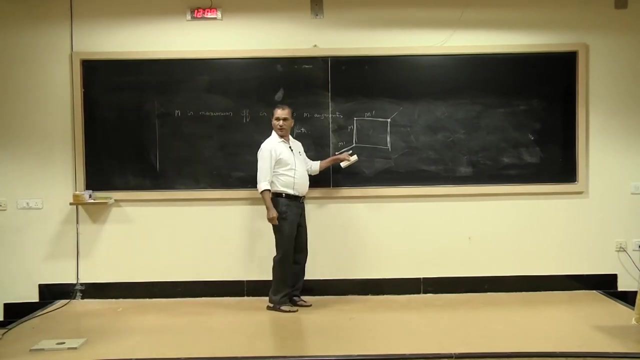 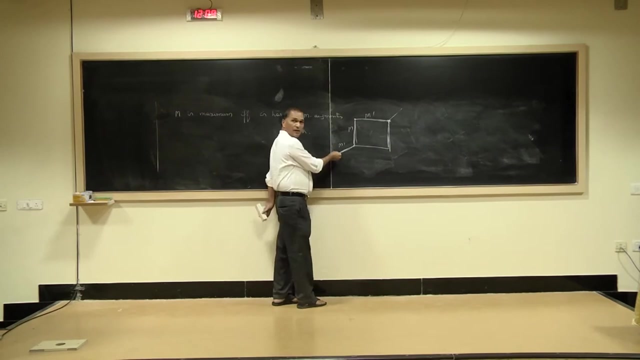 So a matching M is maximum if, and only if, G has no M argumenting path. A matching M is maximum if, and only if, G has no M argumenting path. what is it like? so we have this example, this one. I will explain. this vertex is not incident with any edge. 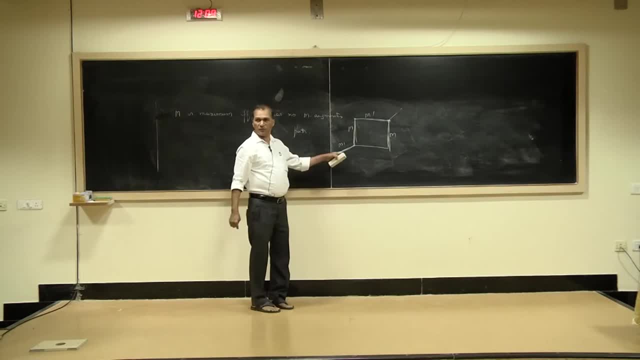 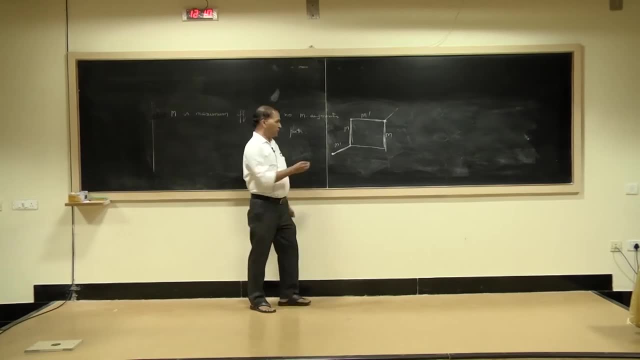 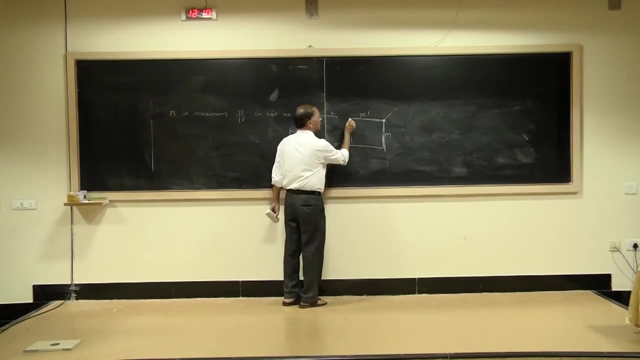 in the matching. This is the matching M M. this is M dash. so this vertex is M unsaturated. right, We start with the M unsaturated vertex. move along this edge which is in M dash, then go to the edge which is in M, then go to the edge which is in M dash. this is M unsaturated. 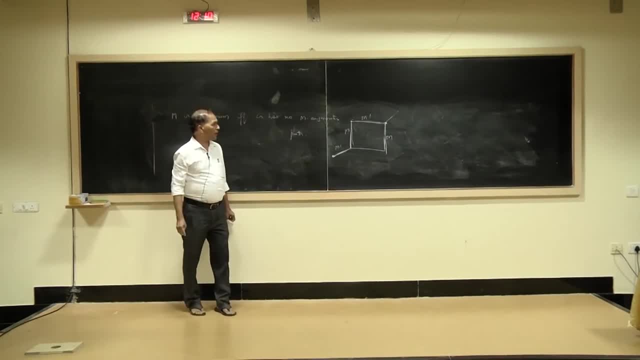 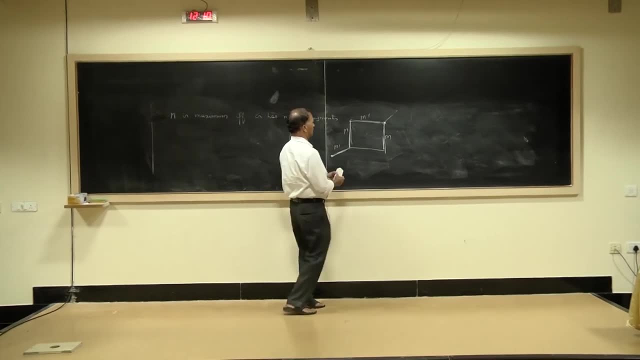 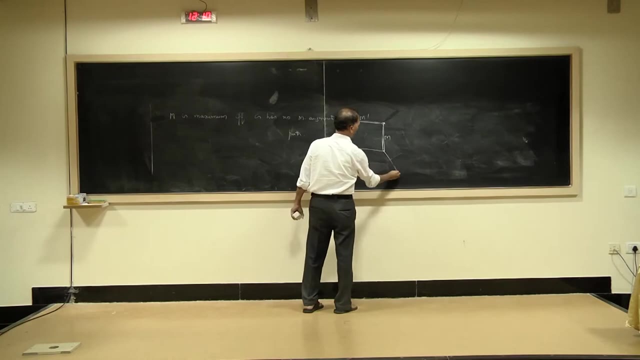 So, if we consider this path, it is a M- I am sorry, M unsaturated. this is M unsaturated, so we have to change the example. it is M unsaturated. we can take no, no, this cannot be M. if this is M, this can be M. it is a matching. 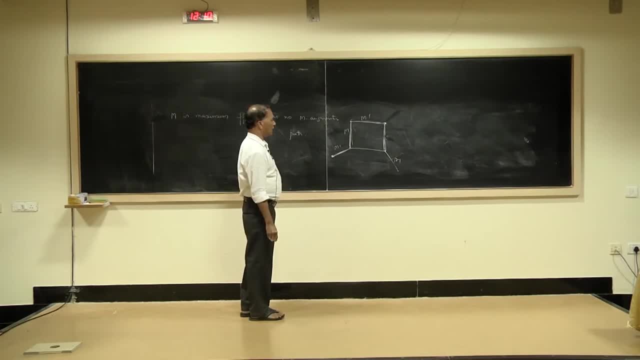 So that will be M, that can be M and this has an M. Last will have to be M. So that is M unsaturated. So that is M unsaturated. So we have to change the example. No, I am doing only this much. this, this, this, I am making this M unsaturated, right. 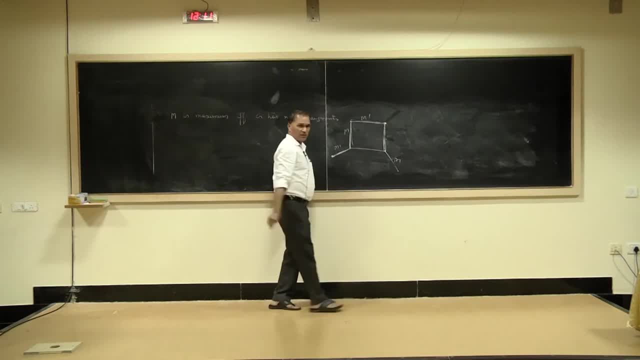 If you make, if you take this as M and this becomes M unsaturated. so this, this is a M augmenting path, right? So the theory says that if M, M is maximum if and only if G has no M augmenting path. 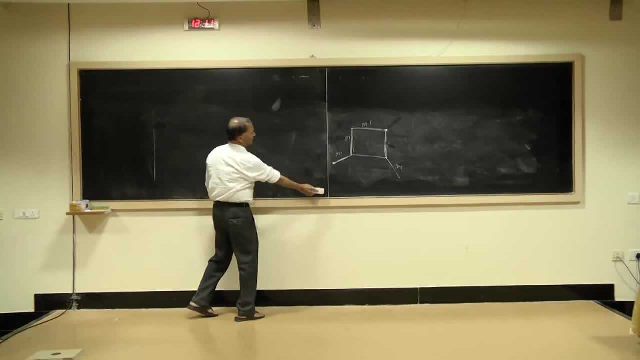 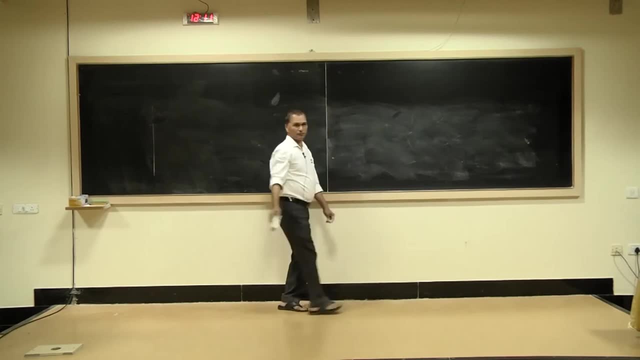 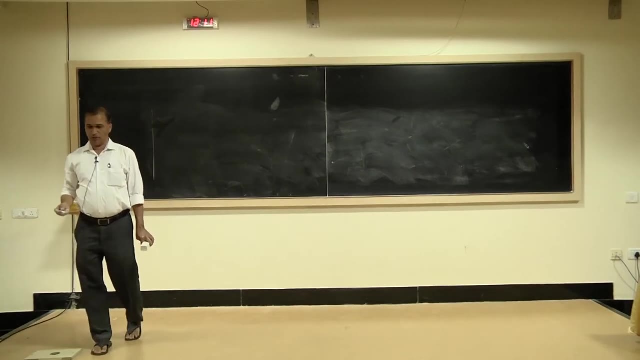 Right. This is simple proof, which again we do not do Right Now. three more concepts are important and we introduce those concepts and do one or two small, small results in those concepts. One is about strongly regular graphs- Right, Okay. 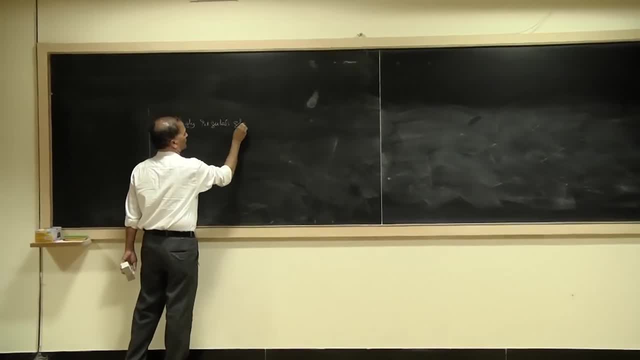 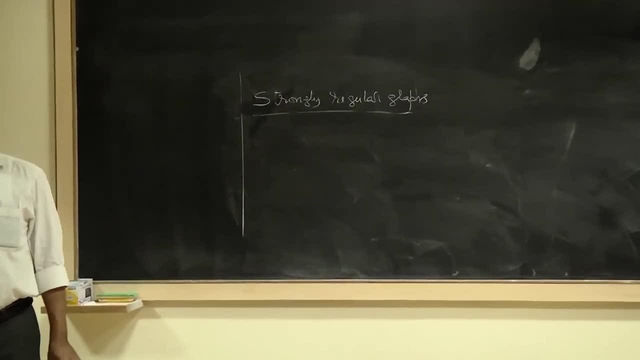 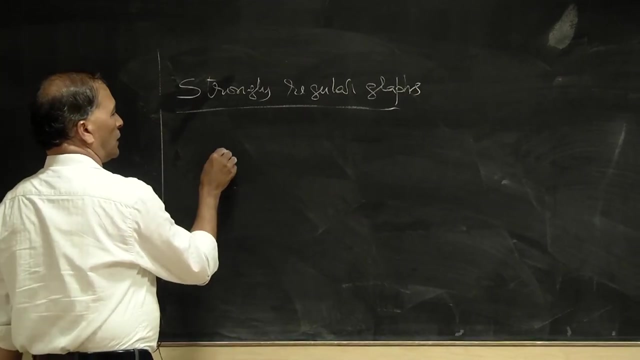 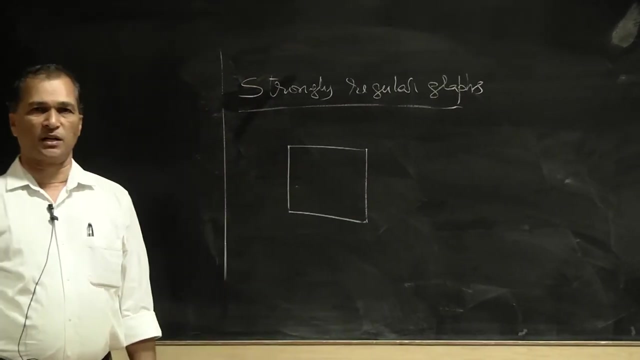 We know a regular graph. A regular graph is a graph in which all the vertices are of same degree. Right Now, you consider this graph. This is a regular graph. Not only that, it is a regular graph, It has some more properties. 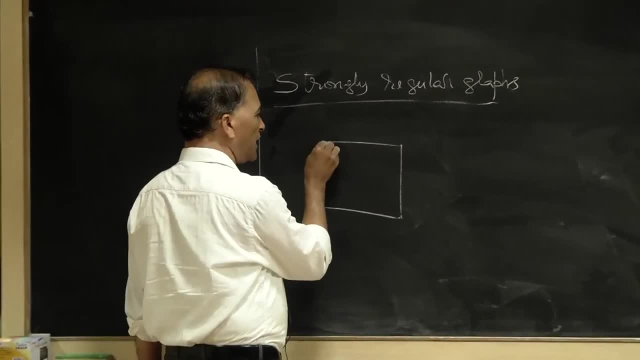 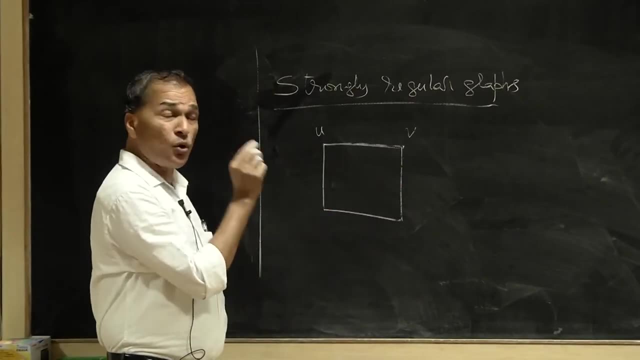 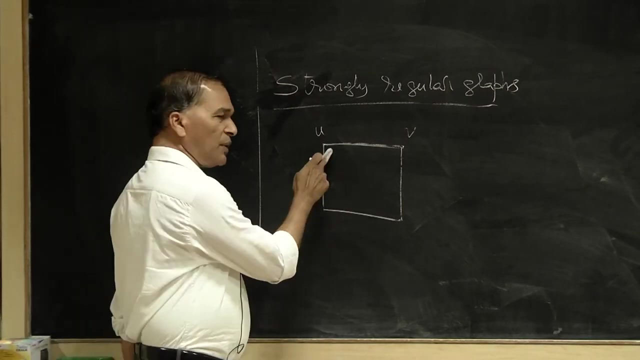 Right. It has some more properties. If you consider any two vertices, for example these two vertices U and V, which are adjacent to each other, there is no vertex which is commonly adjacent to both U and V. Is it not The number of vertices which are commonly adjacent to the vertices U and V which are 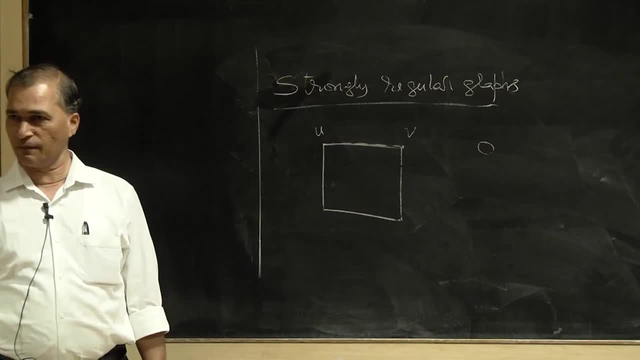 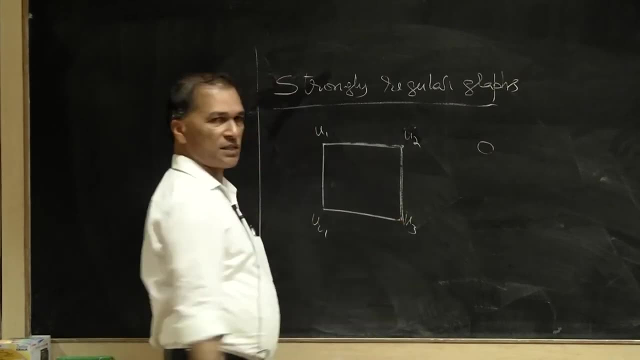 adjacent is equal to zero, Is it correct? Now let us take say: this is U1,, this is U2, this is U3, this is U4. U2 and U3 are adjacent. How many vertices are there which are commonly adjacent to U2 and U3?? 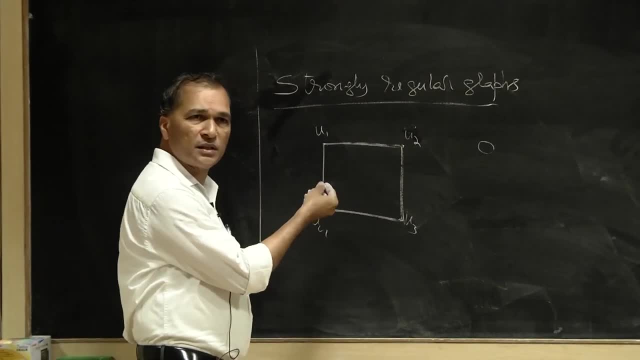 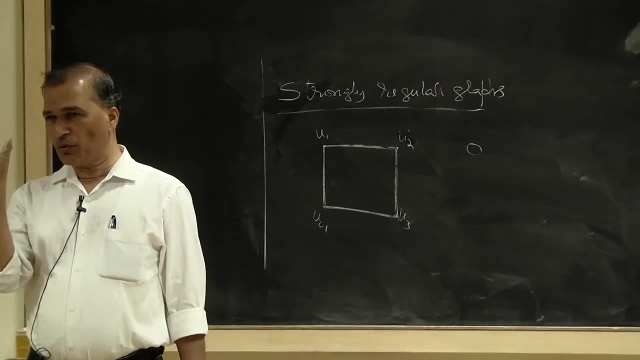 It is again zero. U3 and U4 are adjacent. How many vertices are there? Again zero. U1 and U4 are adjacent. That is again zero. So it has a property that for every two vertices which are adjacent to each other, there are 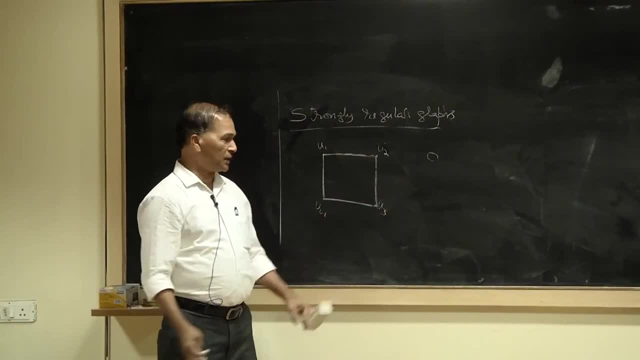 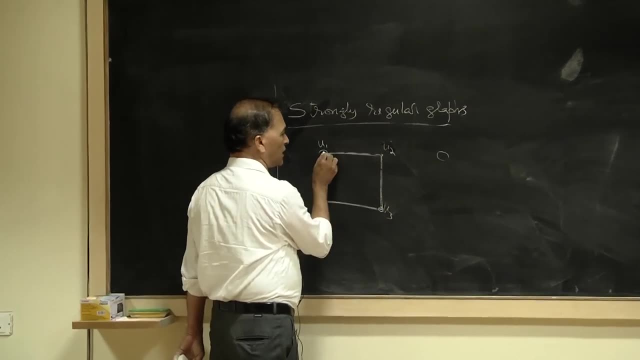 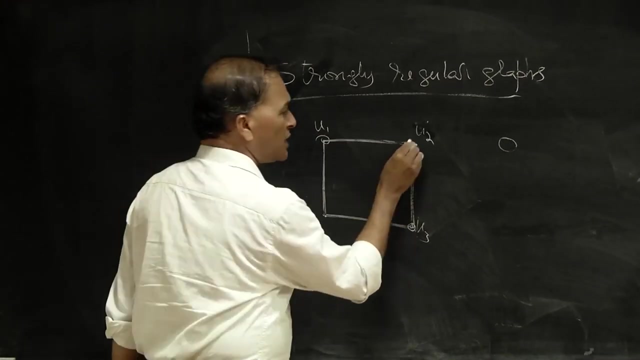 there is no vertex which is commonly adjacent to them. Similarly, you consider two vertices which are non-adjacent: Right. U1 and U3 are non-adjacent. There are exactly two vertices which are commonly adjacent to U1 and U3.. 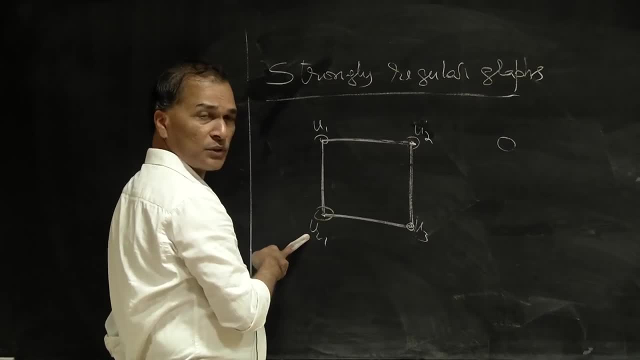 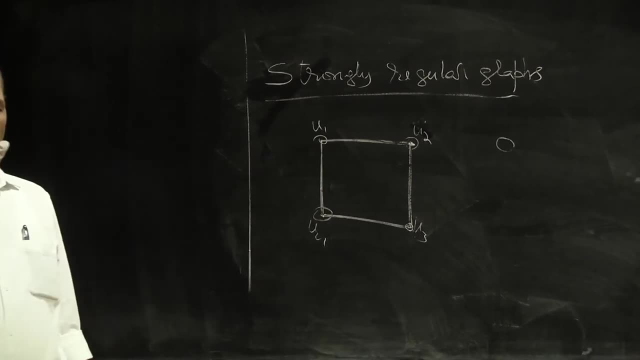 You consider two vertices which are non-adjacent- U2, and U1, U4. There are two vertices which are commonly adjacent to U2 and U4. So for every two vertices which are non-adjacent to each other, there are equal number of vertices. 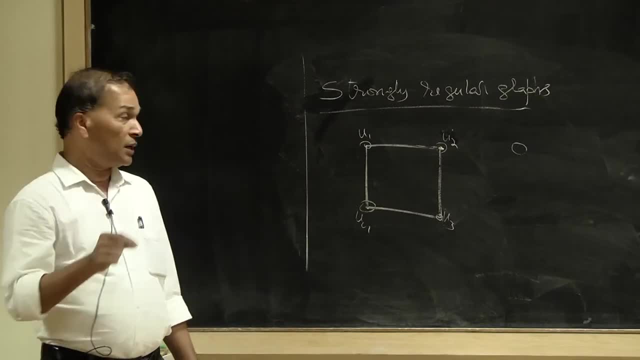 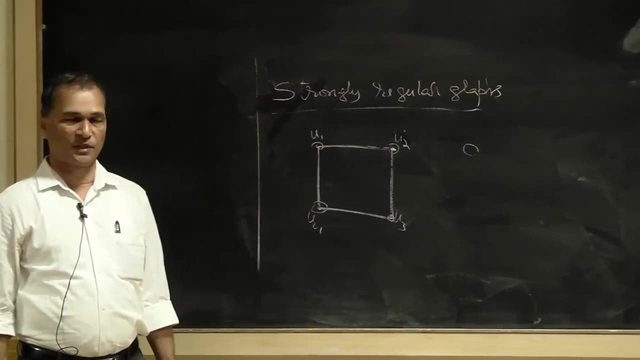 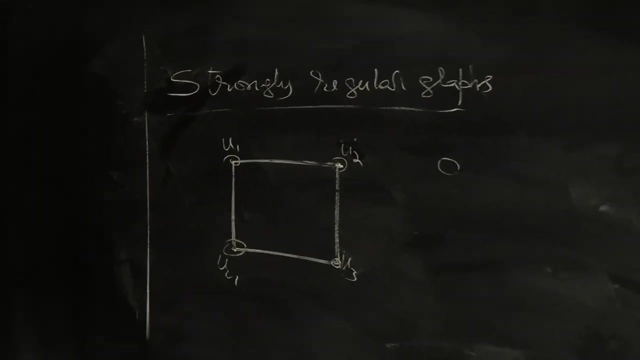 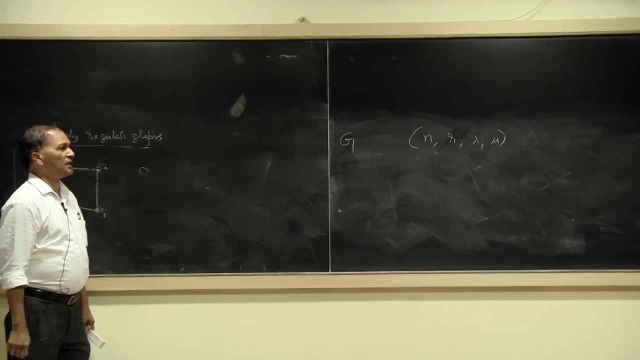 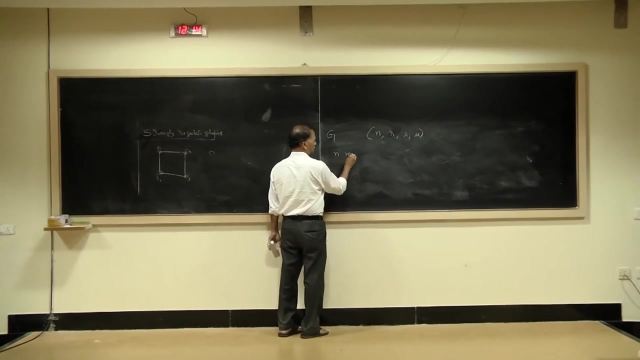 which are adjacent to both of them. Right. If this is true, we say that the graph is strongly regular graph Right A. graph G is a strongly regular graph with parameters n? r lambda mu. It is called a strongly regular graph with parameters n? r lambda mu if it has n vertices. 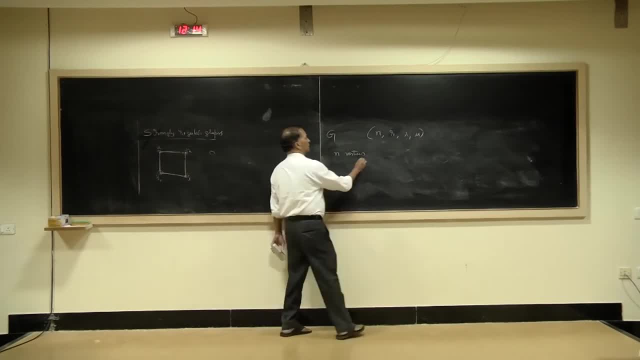 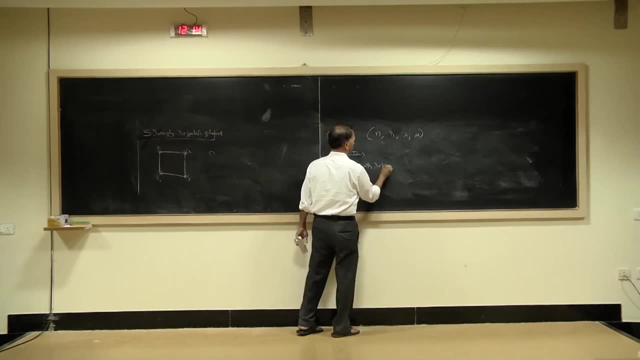 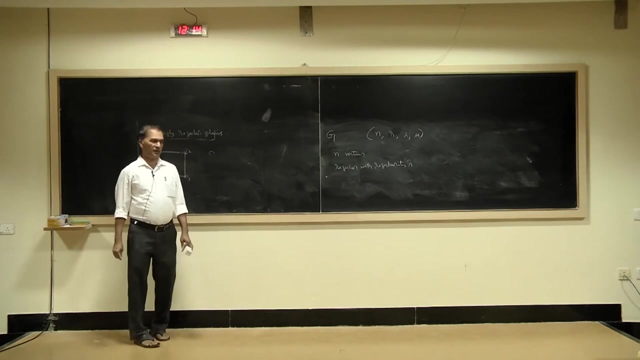 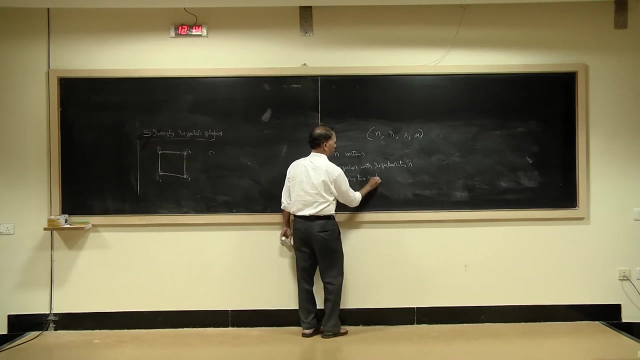 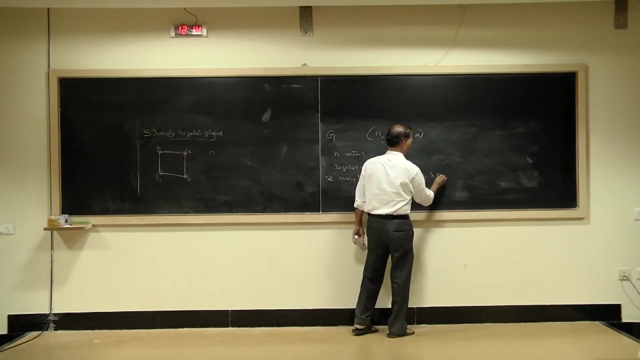 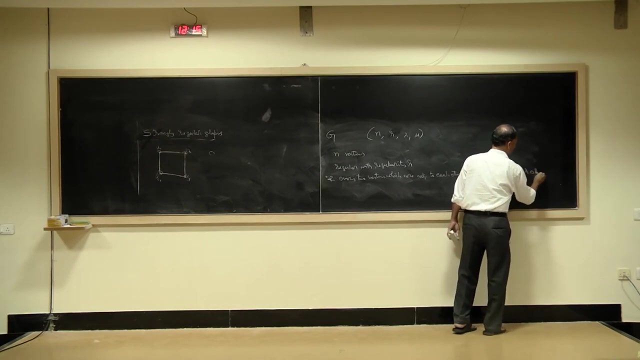 graph has n vertices and is regular with regularity r. it is regular with regularity r And every two vertices which are adjacent to each other. there are equal numbers of vertices which are non-adjacent to each other. Right to each other are commonly adjacent to lambda. other vertices: every two vertices which are: 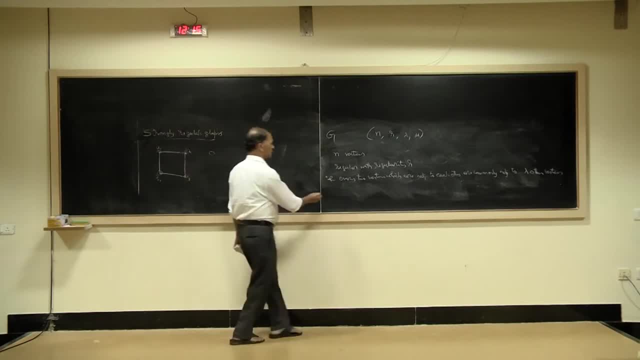 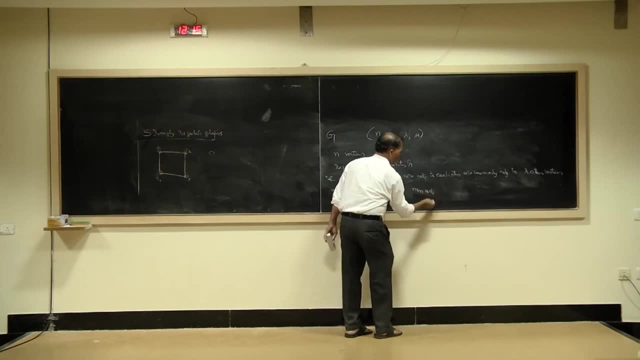 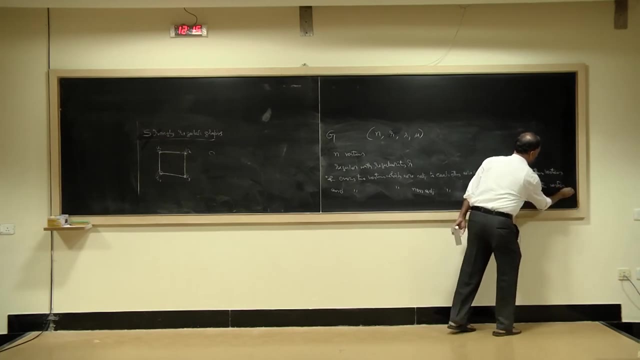 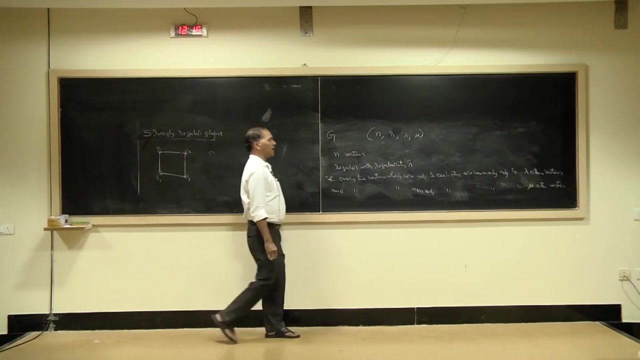 adjacent to each other are commonly adjacent to lambda other vertices, and every two vertices which are non-adjacent to each other are commonly adjacent to mu other vertices. right, It is said to be a strongly regular graph with parameters n, r, lambda, mu, if there 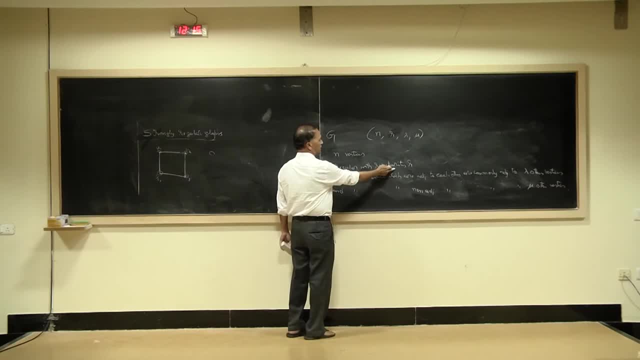 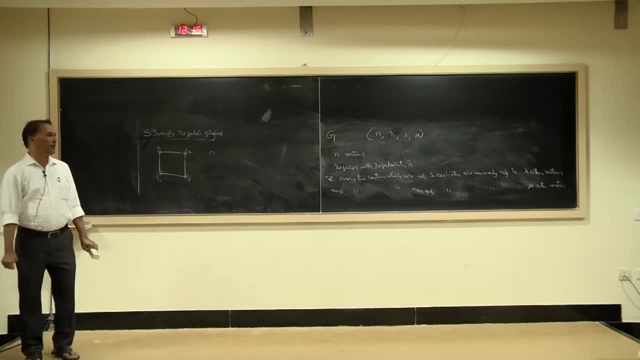 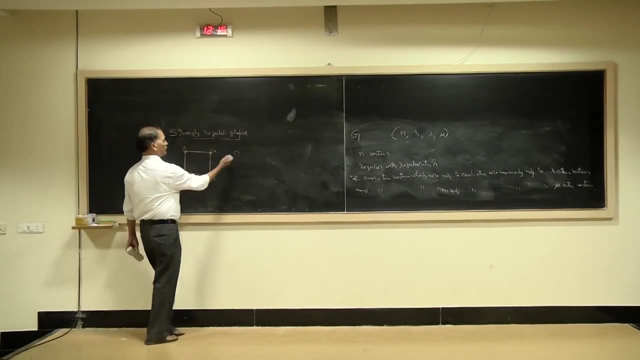 are n vertices And it is regular with regularity r and every two vertices which are adjacent to each other are commonly adjacent to lambda other vertices. and every two vertices which are non-adjacent to each other are commonly adjacent to mu other vertices. Therefore, in terms of that, it is a regular. it is a strongly regular graph with parameters. 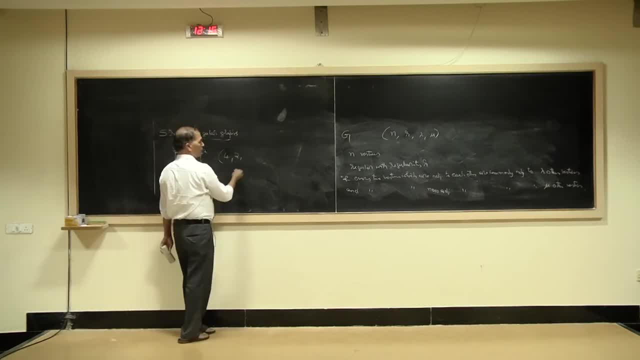 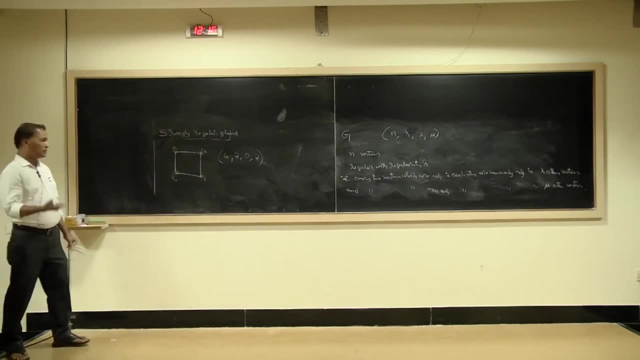 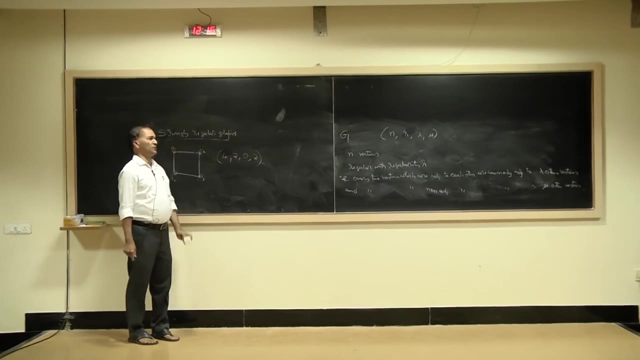 there are number of vertices: 4, regularity: 2, lambda is 0, mu is 2,. every two vertices which are adjustments to each other are adjacent to 0 vertices. every two vertices which are non-adjacent to each other are adjacent to two other vertices. 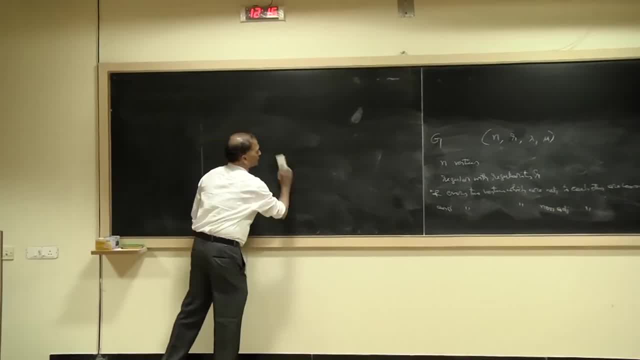 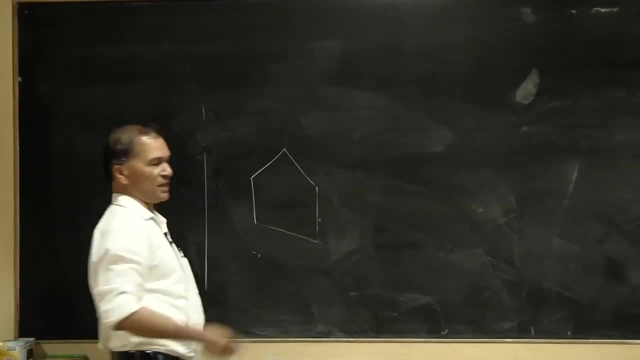 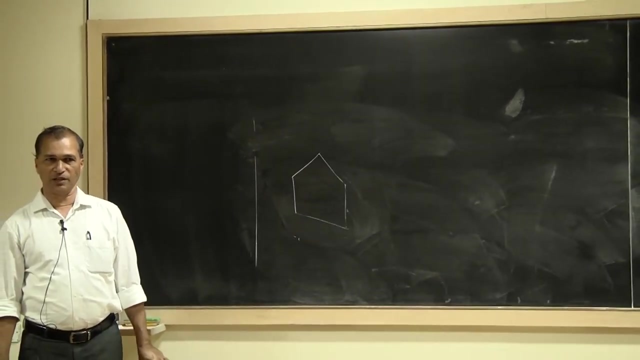 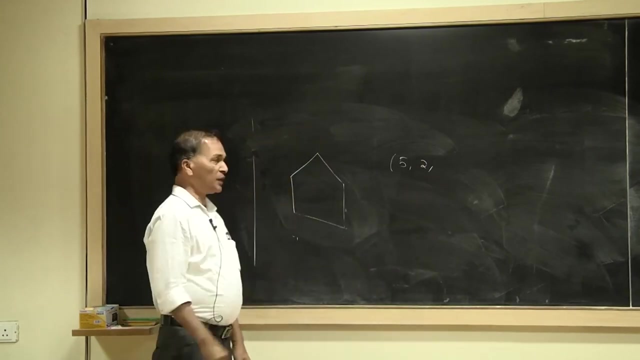 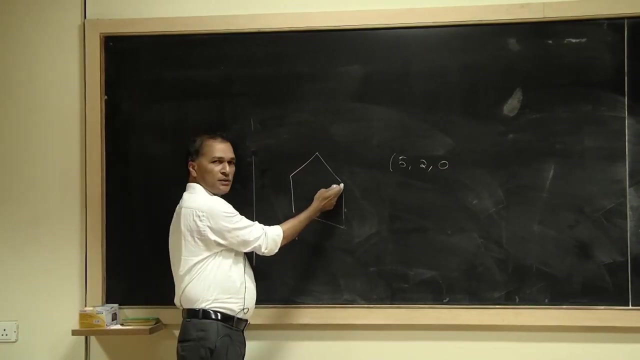 So this is an example for the strongly regular graph. If you take this cycle, Is it strongly regular? Is it strongly regular or not? Ok, There are 5 vertices. regularity to every 2 vertices which are adjacent to each other. adjacent to 0, it is true for every vertices which are adjacent to each other adjacent. 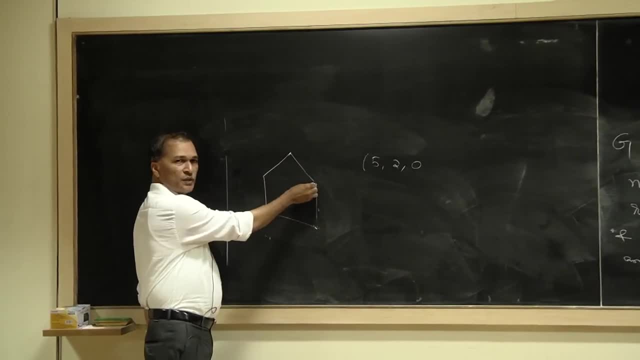 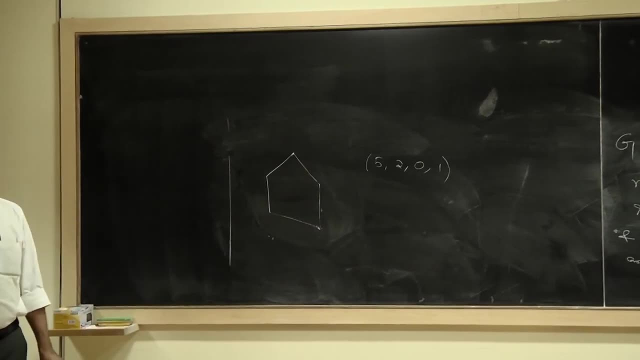 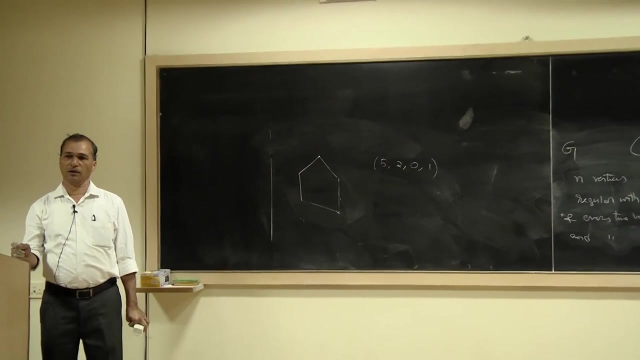 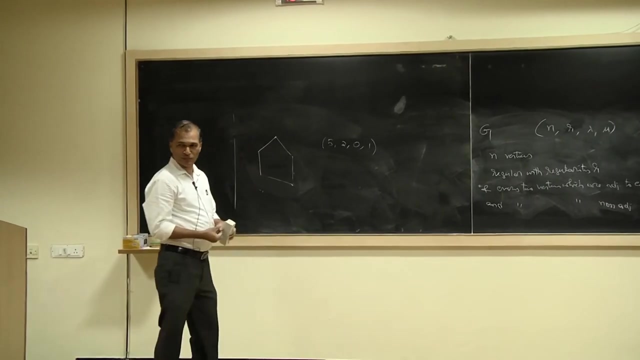 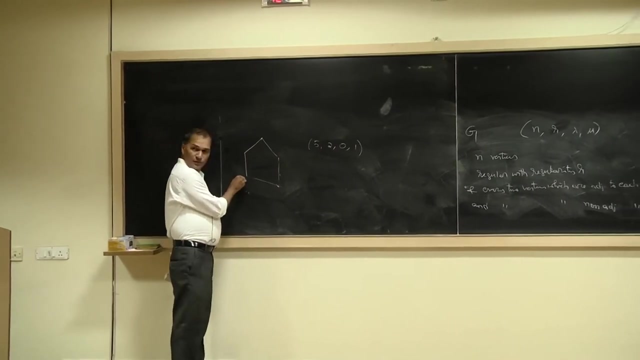 to each other adjacent. every vertices which are non-adjacent to each other is commonly adjacent to exactly one vertex. right, It is a strongly regular graph with parameters 5,, 2,, 0,, 1,. is it correct, David? which one 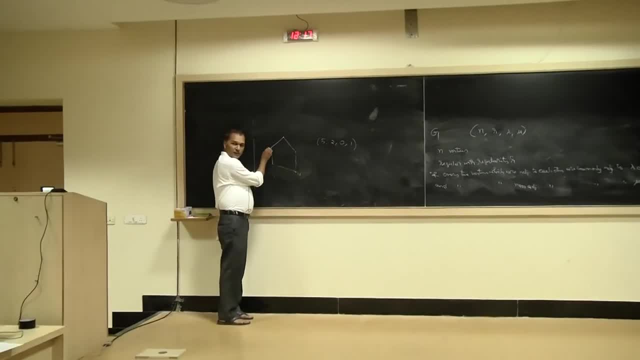 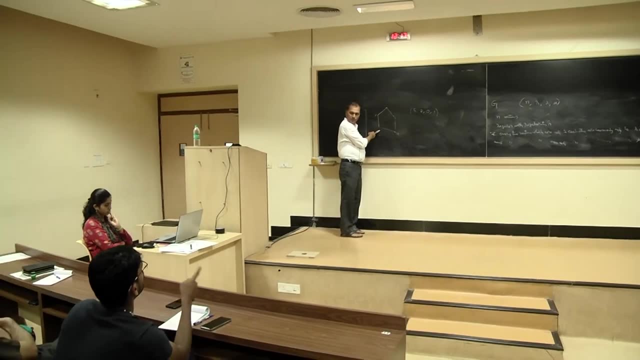 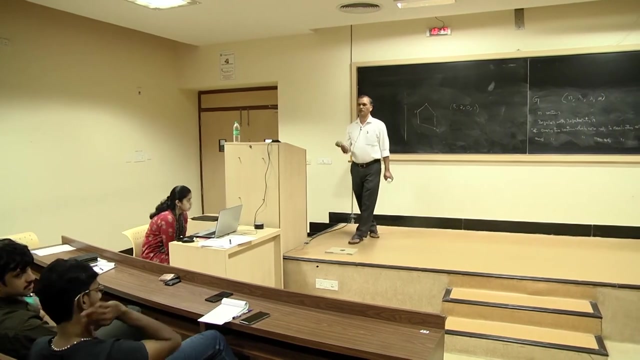 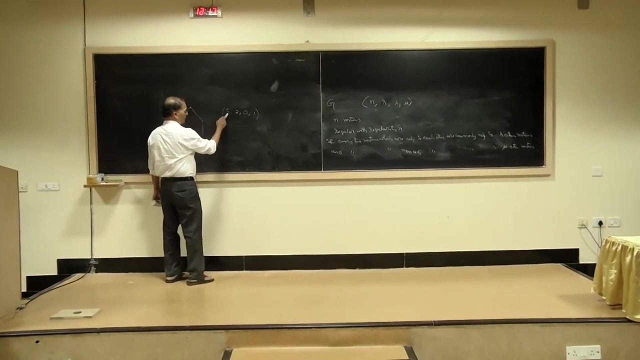 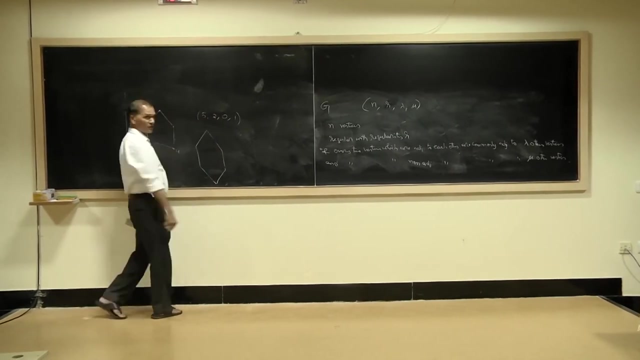 This vertex u, this vertex v. It is correct. So every 2 vertices which are non-adjacent to each other are commonly adjacent to exactly one vertex commonly adjacent to. So it is a strongly regular graph with parameters 5,, 2,, 0, 1,. is this a strongly regular graph? 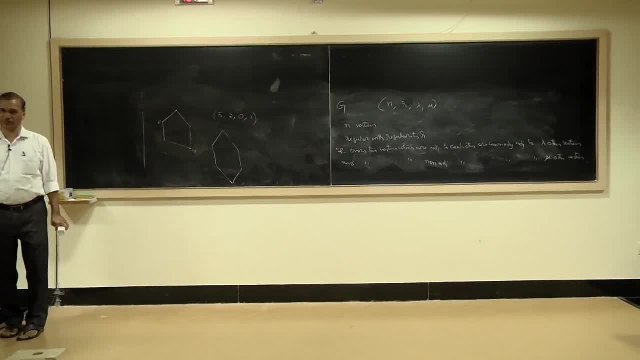 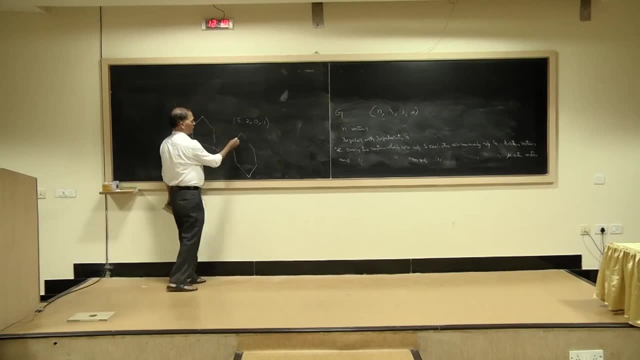 cycle on 6 vertices. Is it a strongly regular graph why These 2 vertices, which are non-adjacent to each other, is commonly adjacent to one vertex? these 2 vertices which are non-adjacent to each other is not commonly adjacent to any. 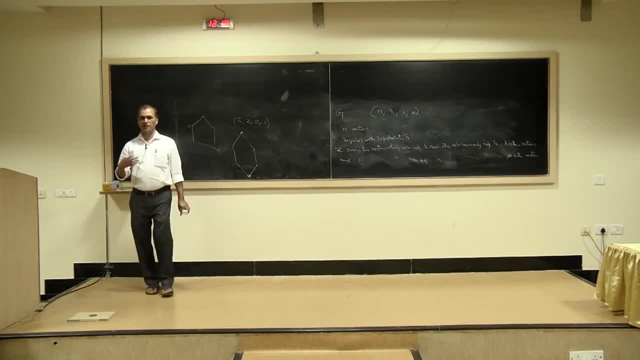 vertex, If at all, it is strongly regular. every 2 vertices which are non-adjacent to each other should be commonly adjacent to same number of vertices, which is not true here. 1 is 0, though, So up to C5.. 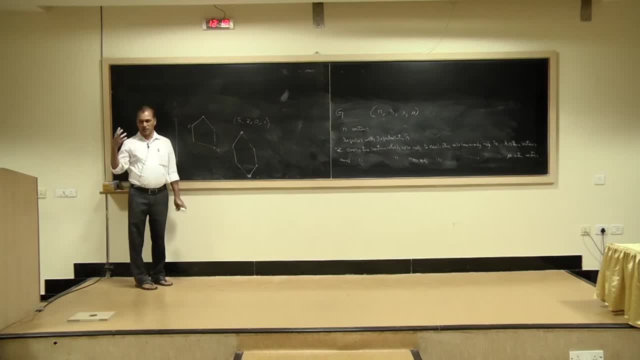 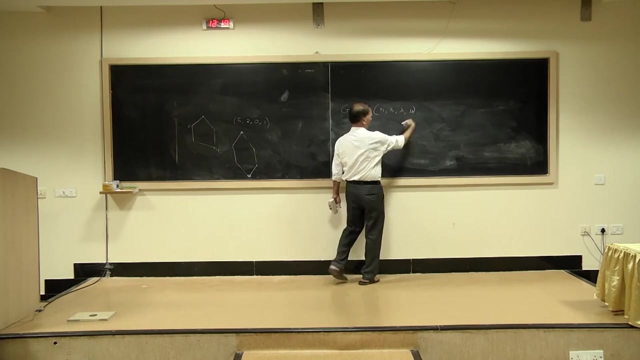 These are no cycle Cn, where n greater than or equal to 6 is strongly regular. for the same reason, right Suppose that G is strongly regular with parameters n? r lambda mu, that G be strongly regular with parameters n r lambda mu. 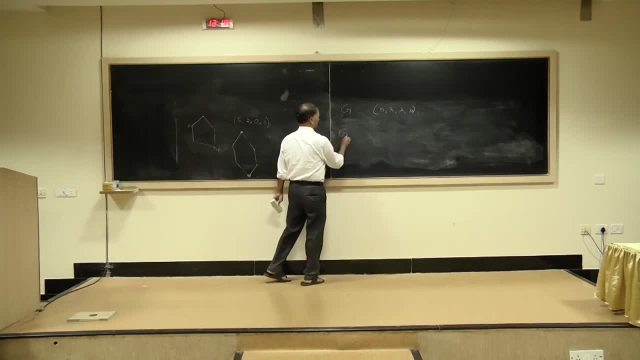 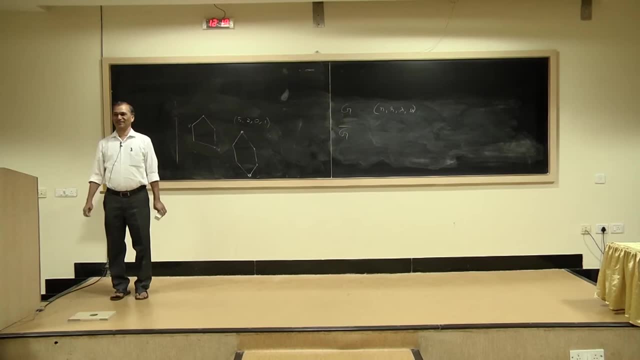 So this is a strongly regular graph. What can you say about G bar, Complement of G? do it, try check whether G bar is strongly regular. G is strongly regular with these parameters. you want to check? you do it, try it- whether G bar is also strongly. 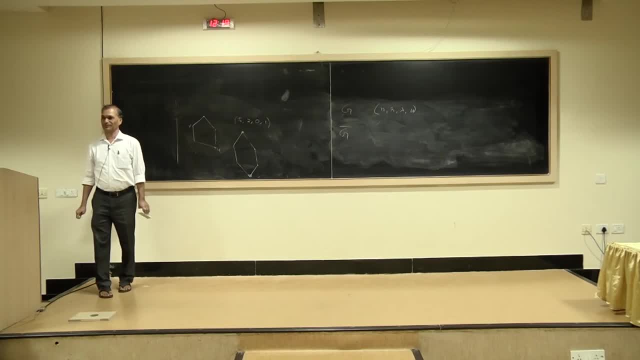 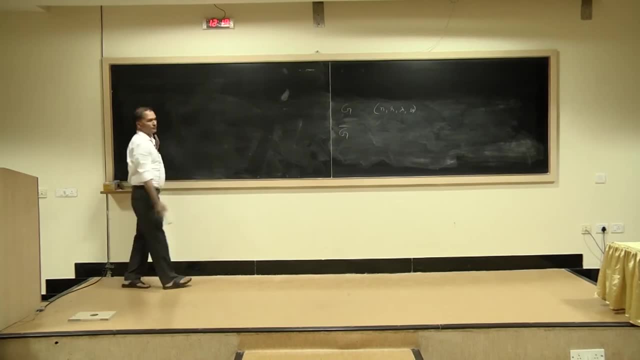 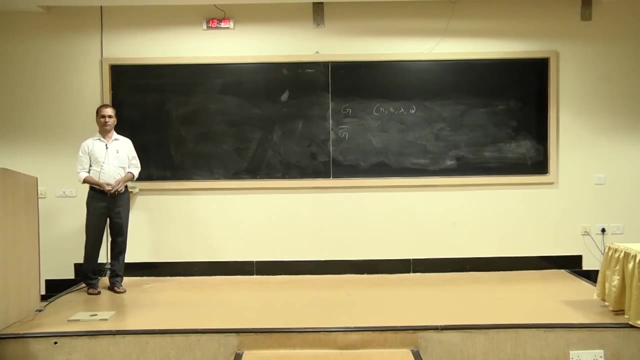 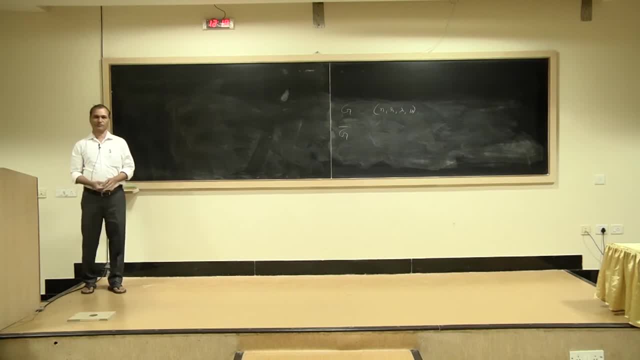 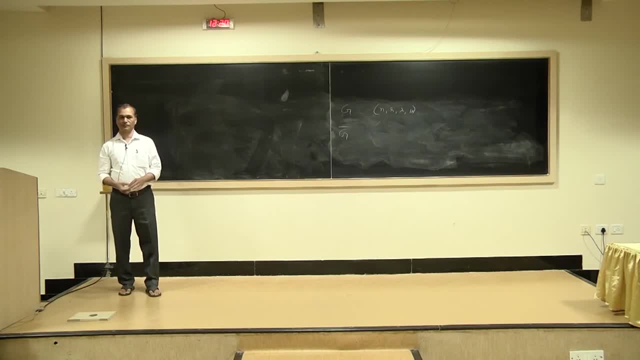 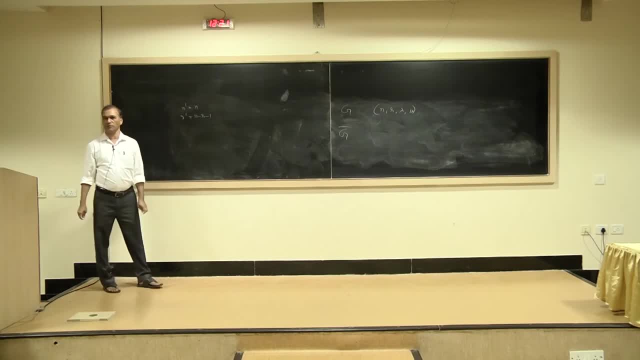 dash is equal to N R dash. if you take R dash is equal to N, So N dash is equal to N minus R minus 1, we just have to find out what is lambda dash and what is mu dash, if at all. it is strongly regular, ok. 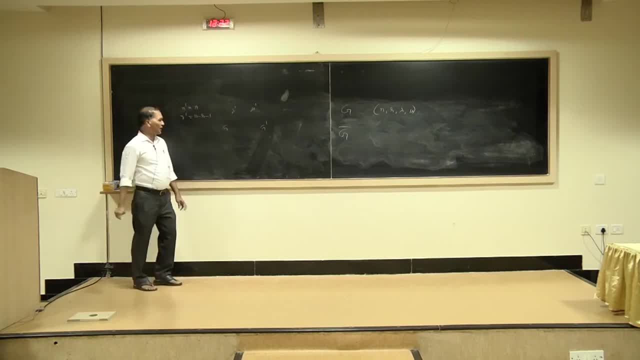 So lambda dash is equal to Lambda dash is equal to N minus N minus N minus, right, Ok, Ok, Ok, n minus lambda plus 1, you have to come and prove it here. So let us consider two vertices, u and v, which are adjacent in G. We know that they are commonly. 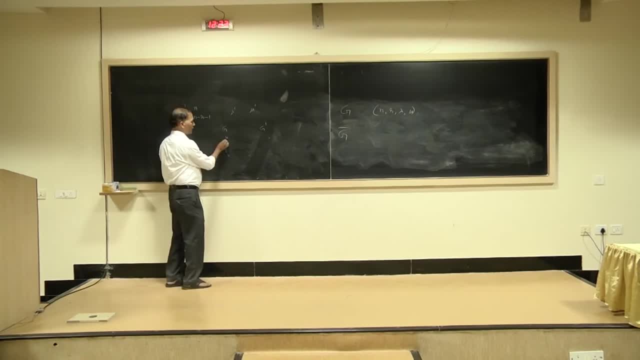 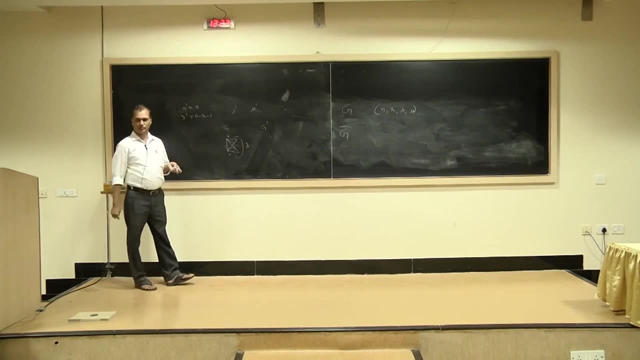 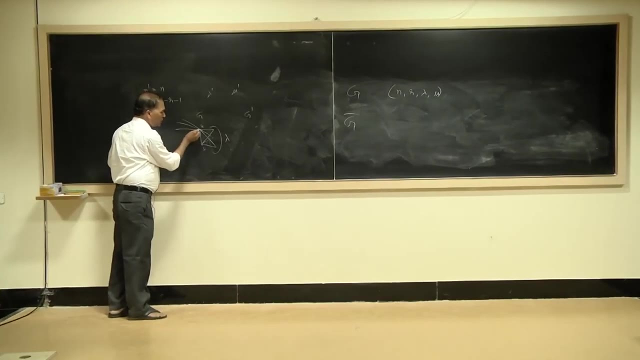 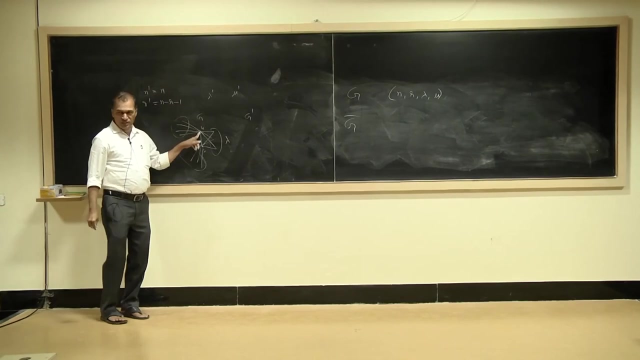 adjacent to lambda other vertices. So they are adjacent to lambda other vertices. commonly adjacent to This is lambda vertices. Degree of the vertex u is r. Therefore it is adjacent to these vertices. How many vertices are here? The same number of vertices are here, Degree. 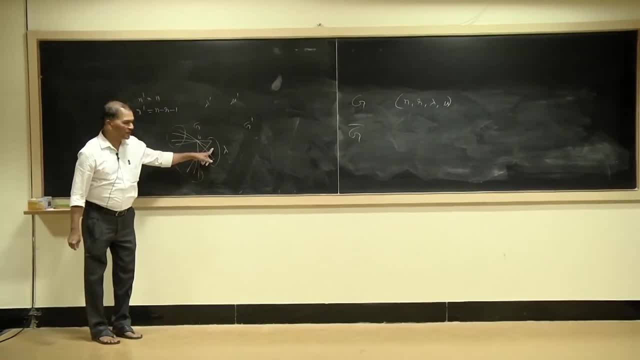 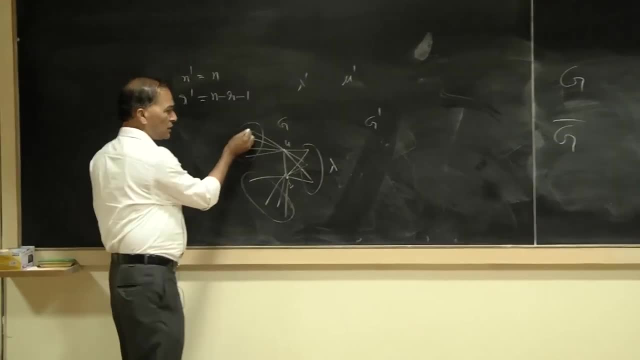 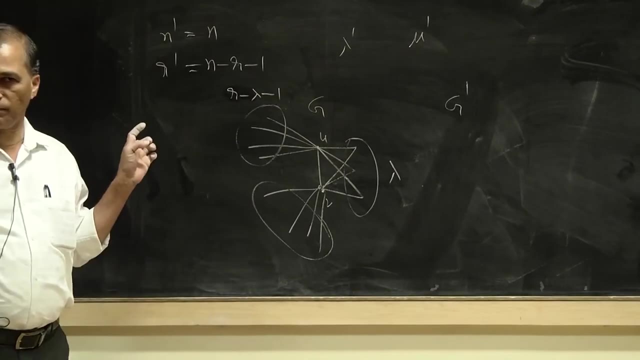 of u is r, because it is r regular Lambda vertices are here which are commonly adjacent to u and v. One is here adjacent to u. Therefore it is here. How many vertices are there? There are many vertex aqui. It is r minus lambda minus 1.. Here also there are r minus lambda minus 1 vertices You take. 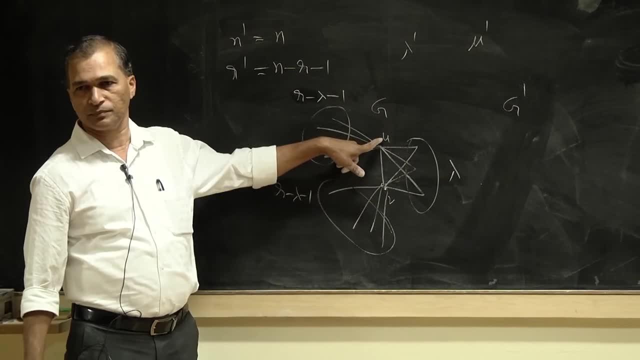 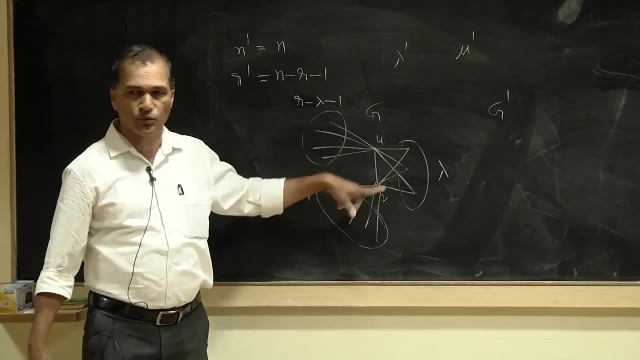 any vertex here in the complement it will be adjacent to u, not adjacent to v. And here every vertex is not adjacent to u and is adjacent to v in the complement. These vertices are neither adjacent to u nor is adjacent to v in the complement. So what are the vertices which are adjacent to both? So why does v go FREE? Uh, because both are adjacent to v, and v isiss me too. Ok, What is the only democracy there, and what else can we study here? which are adjacent? 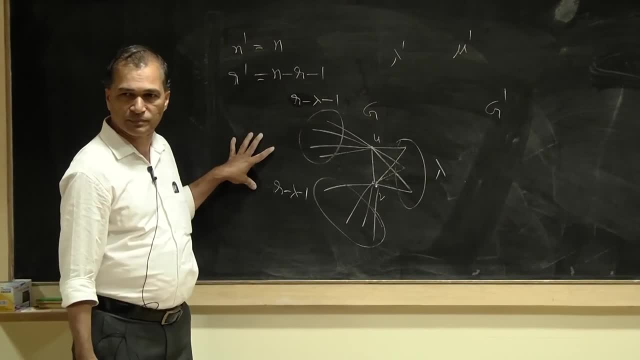 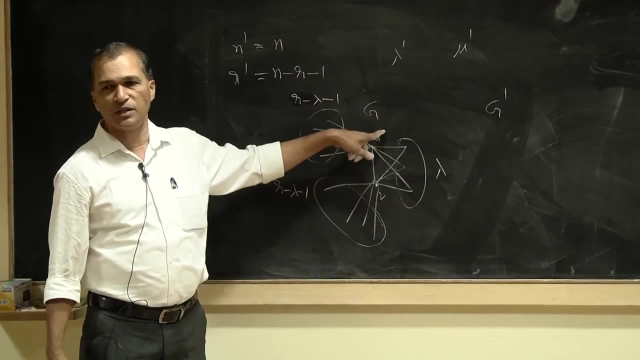 to v. so what does nature goes free can also be the complement. The remaining vertices: These vertices are neither adjacent to u nor adjacent to v. These vertices are adjacent to v, non-adjacent to u. These vertices are adjacent to u, non-adjacent. 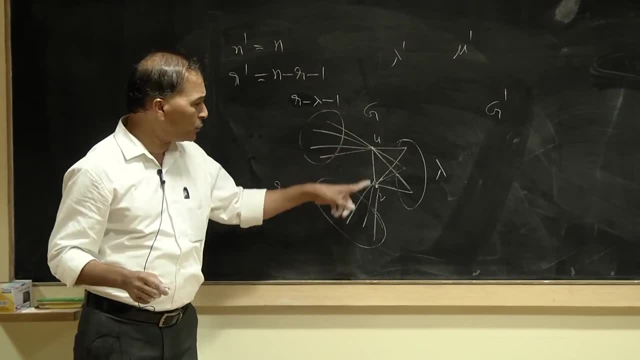 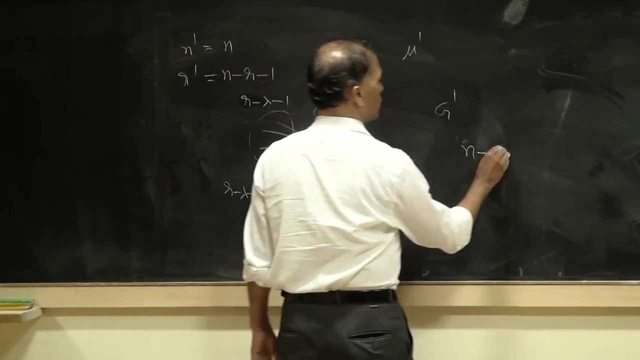 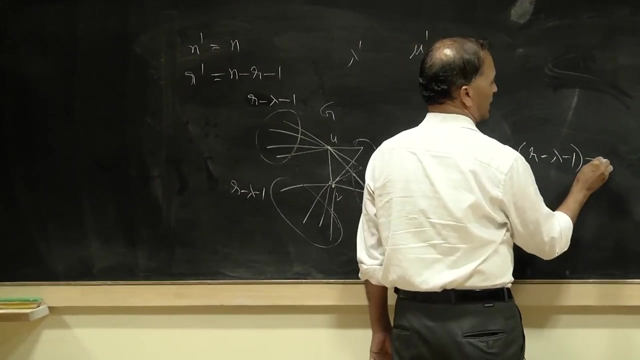 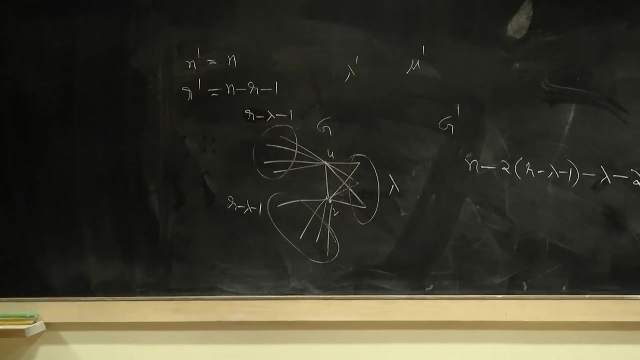 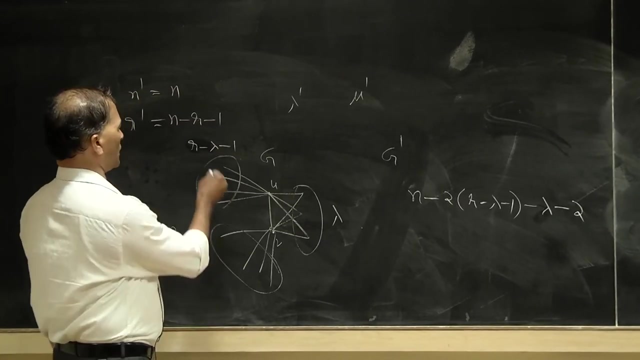 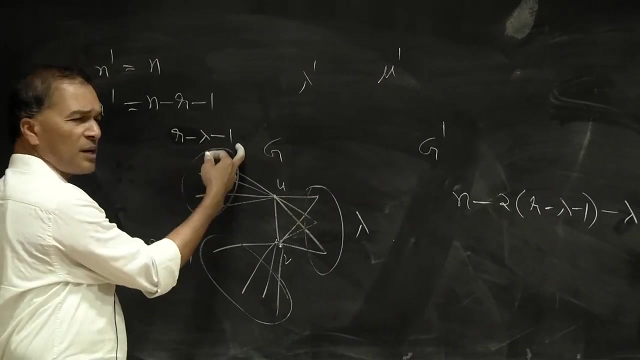 to v. So the vertices which are commonly adjacent to both u and v are the remaining vertices. How many vertices are remaining? It is n minus 2 times r minus lambda minus 1 minus lambda minus 2, u and v. Is it correct? What is it? r minus lambda minus r minus. 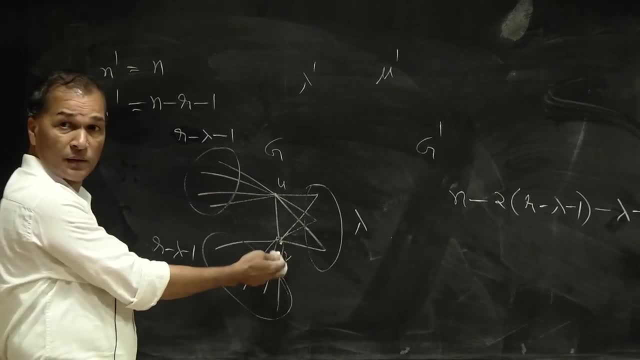 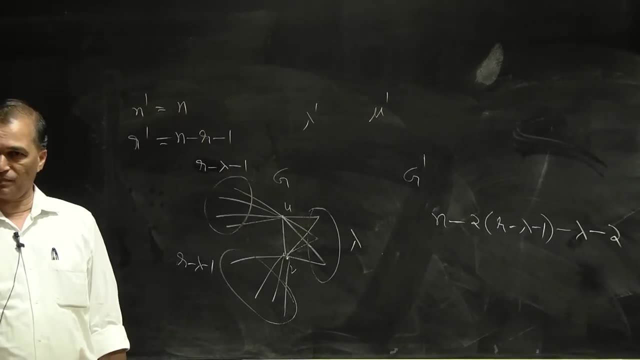 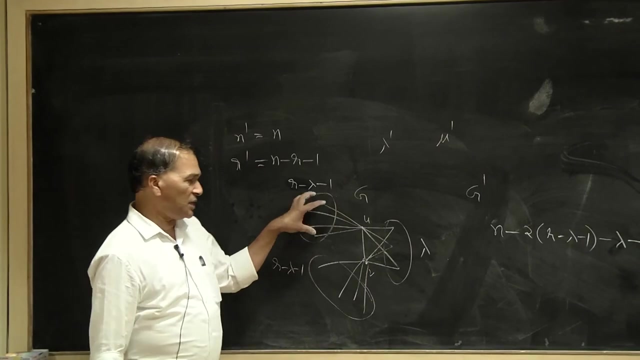 lambda plus 1, r minus lambda minus 1.. I have taken this separately: Minus 2.. All of these are subtracted from n. They are all been subtracted from n. These many vertices, these many vertices, these two vertices, and these vertices are to be removed. Only remaining 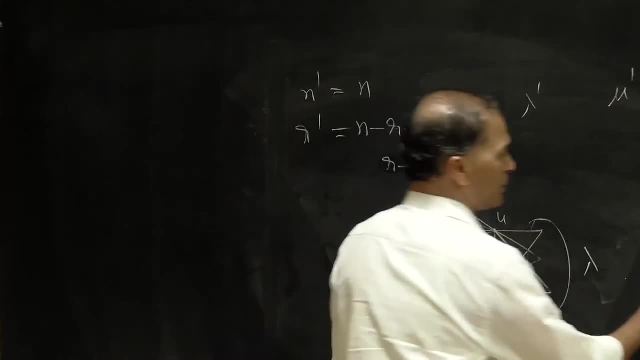 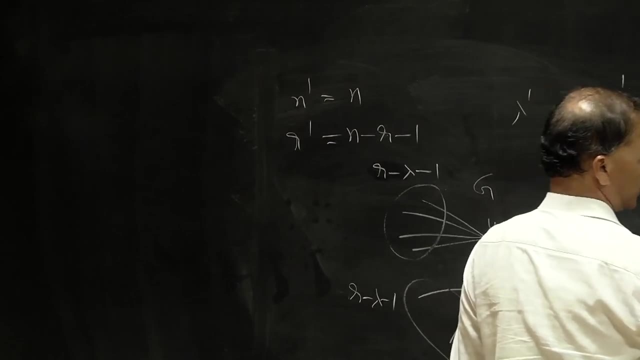 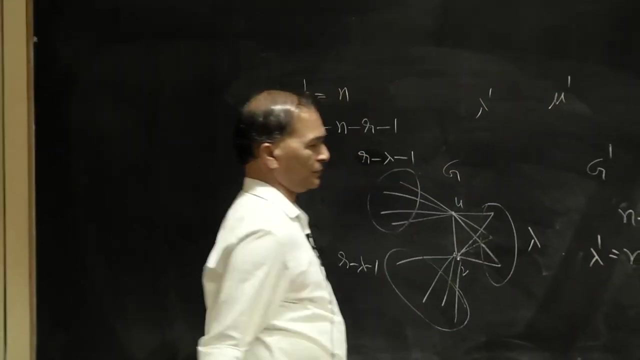 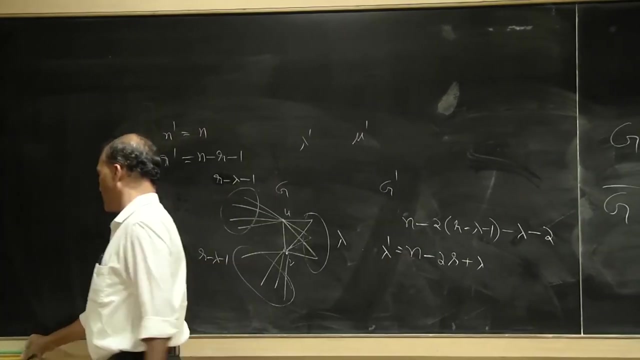 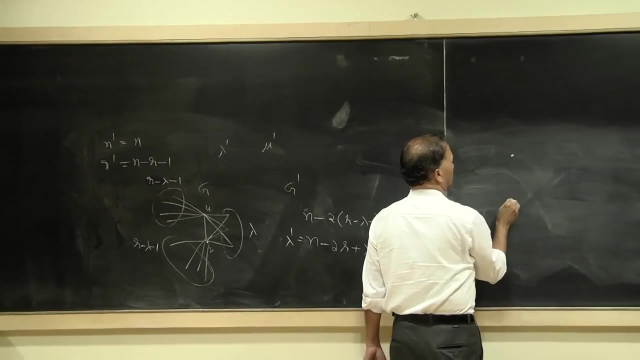 vertices are commonly adjacent to both. What is this number? It is n minus 2, r plus 2 lambda minus lambda plus lambda plus 2 minus 2.. This is what is lambda dash commonly adjacent to. Similarly, if you take two vertices, do it the other part. 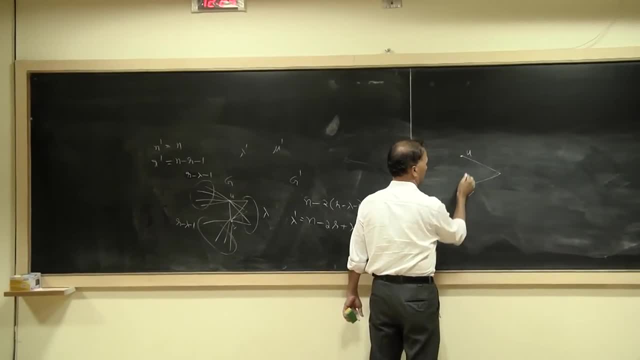 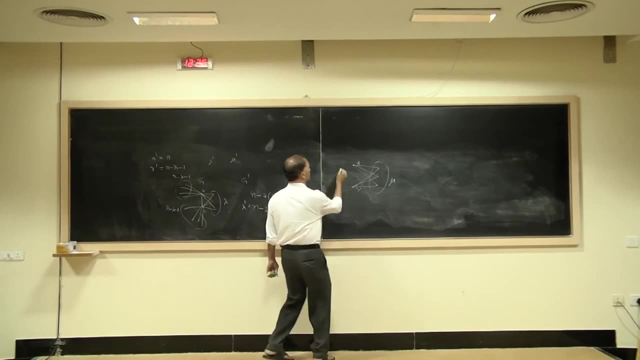 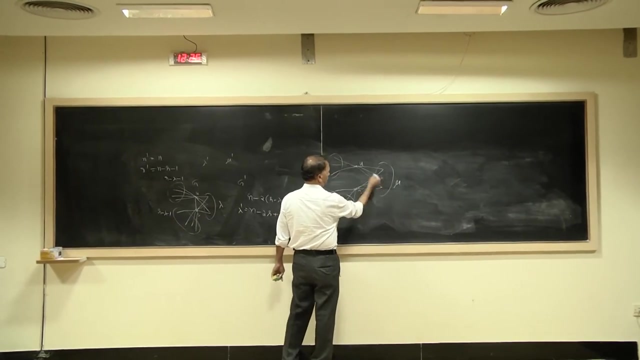 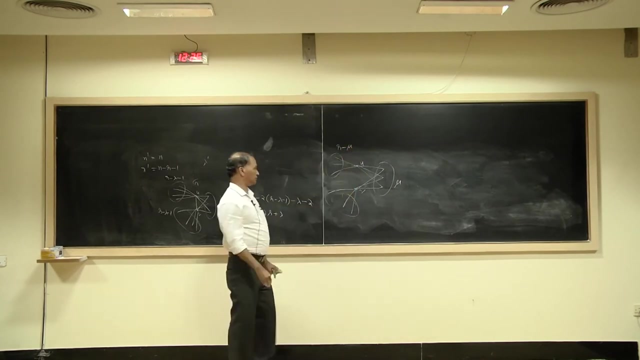 Suppose that u and v are two vertices which are non-adjacent to each other. they are adjacent to commonly adjacent to mu other vertices, and this is r minus mu right. So degree of this vertex is r, out of which mu are here, and this must be r minus mu, r minus mu plus. 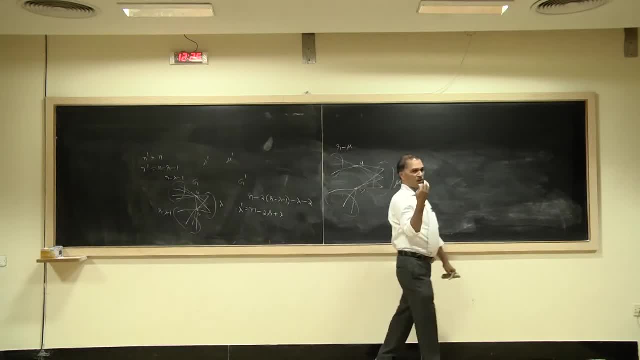 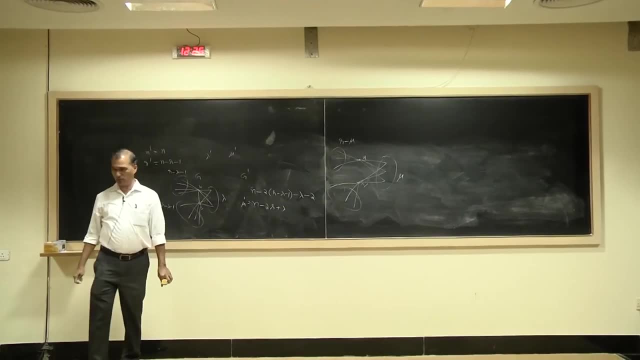 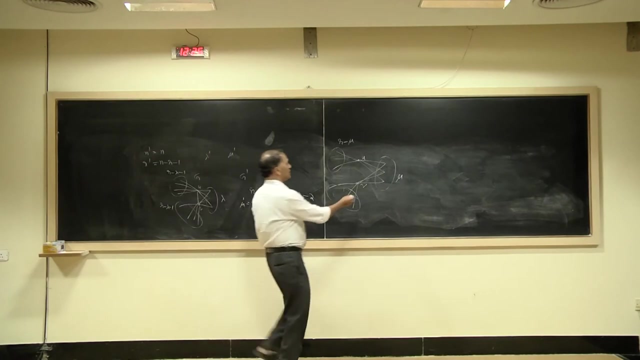 mu is equal to r total. Therefore, what is? what are the vertices which are okay? this is mu dash? because they become non-adjacent in the complement. you are right, This u and v become non-adjacent in the complement every two vertices which are non-adjacent to. So this is mu, So we. 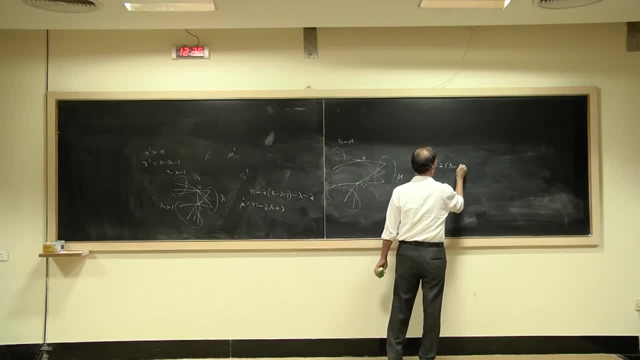 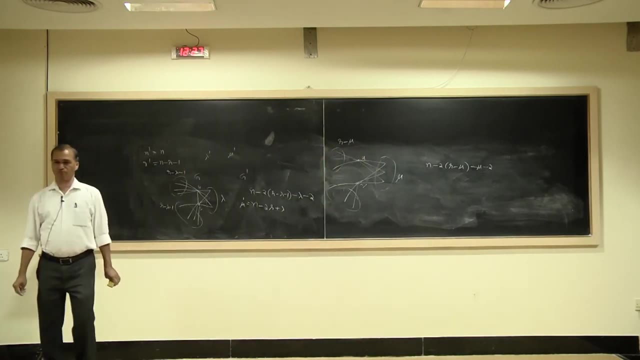 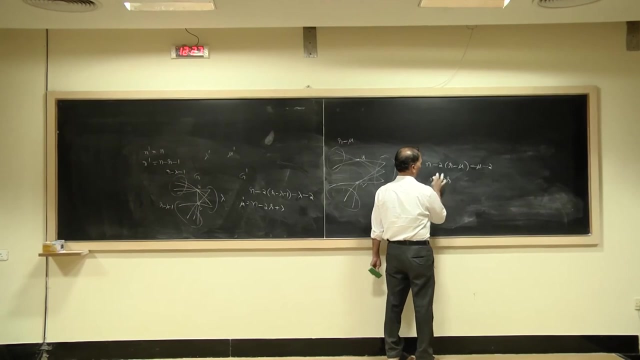 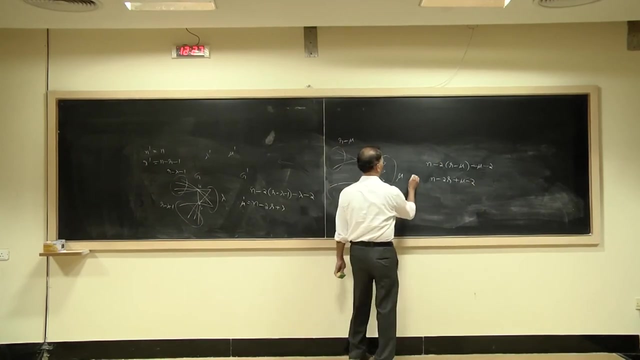 have what it is: n minus 2 times r minus mu plus mu minus 2, minus mu minus 2,, right, So it is equal to r minus 2 r, n minus 2 r plus 2 mu minus mu plus mu minus 2,. this. 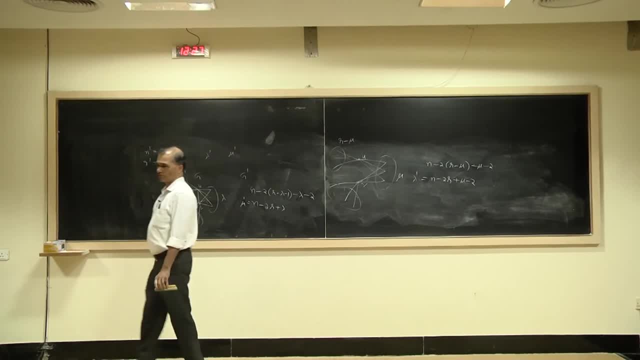 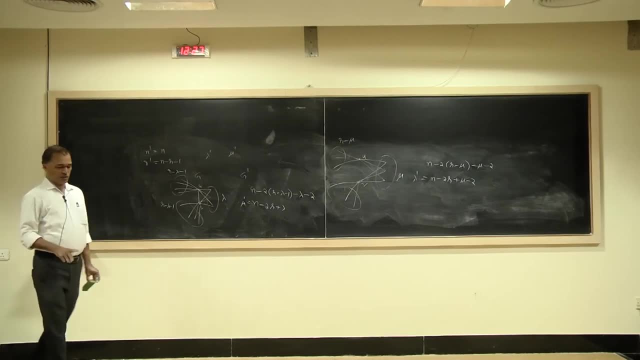 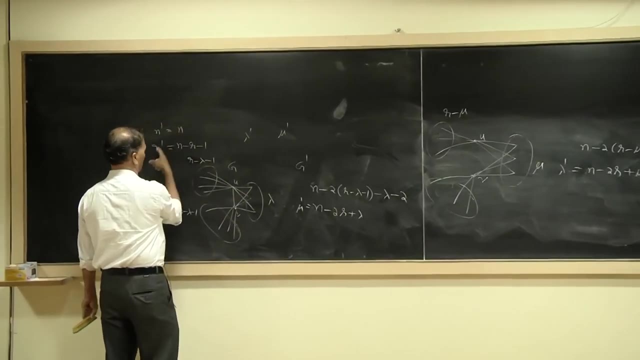 is lambda dash, they become adjacent in that right. So if g is strongly regular, g bar is also strongly regular and the parameters are this: n dash is equal to n, r dash is equal to n minus r minus 1 and lambda dash is equal to. 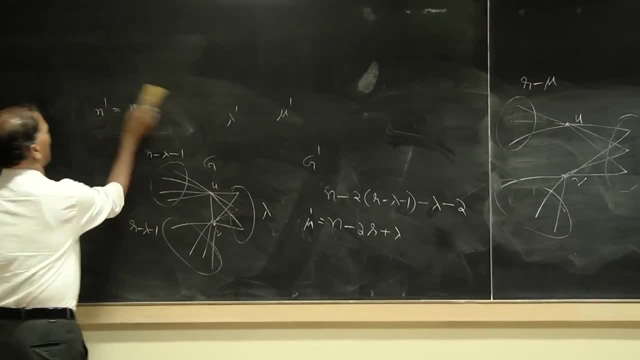 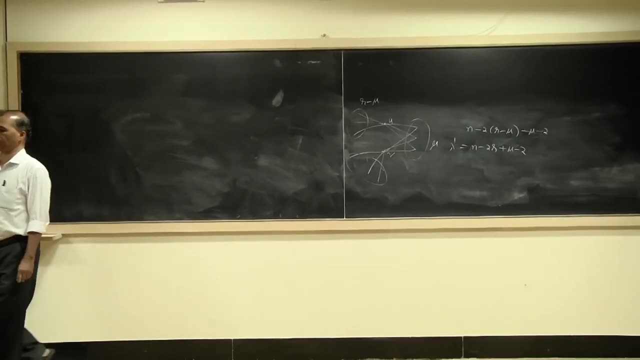 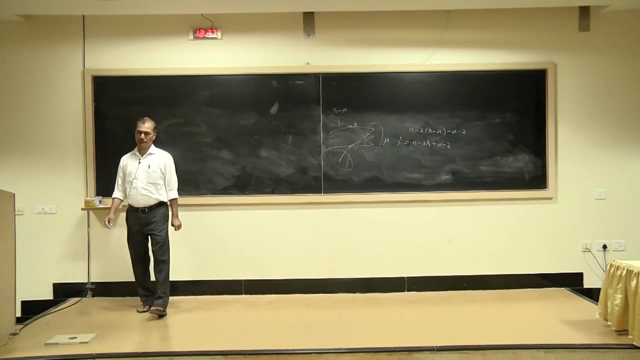 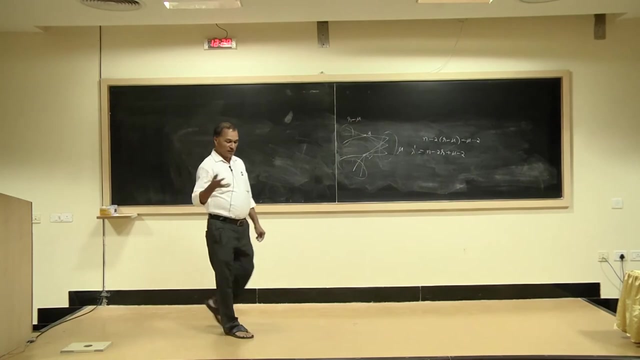 that and mu dash is equal to this. Then there is one special graph which is called friendship graph. There is a theorem which is called friendship theorem, which is related to the strongly regular graph. The strongly regular graph are characterized by the number of eigenvalues. 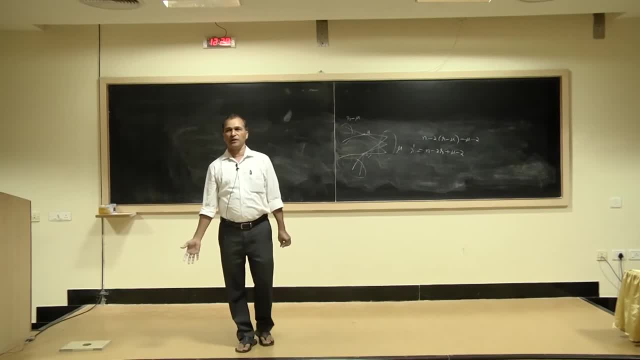 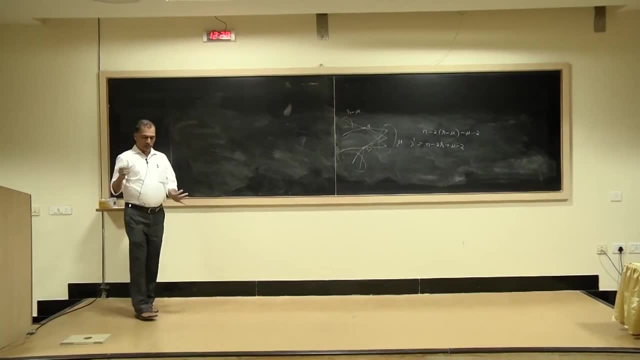 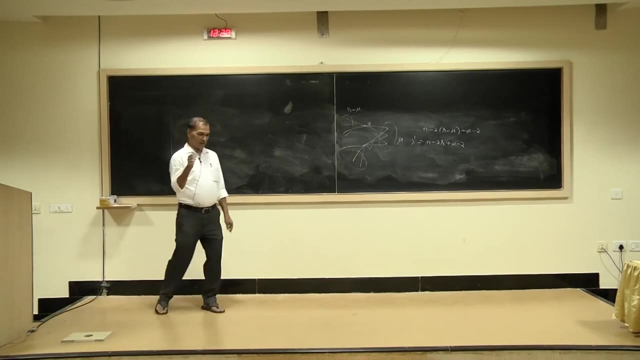 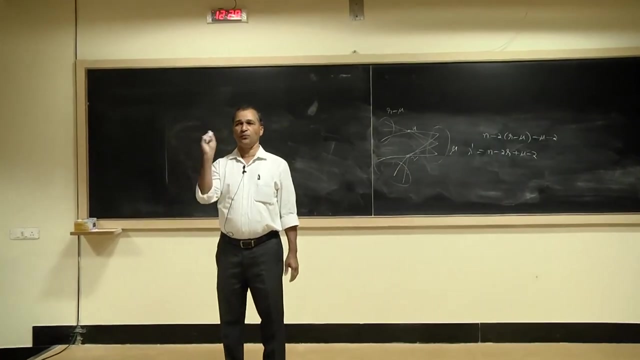 of the graph, which will be done later. A graph is strongly regular if, and only if, it has exactly three eigenvalues. right, That we do not anyway. that will be done later. This friendship theorem, it is a almost like a party problem. It says that if in a group of people, every two of them know exactly, 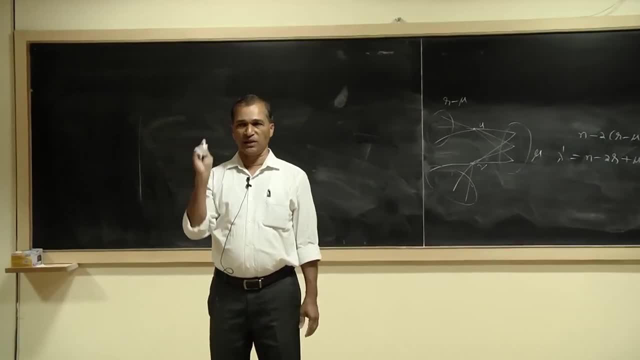 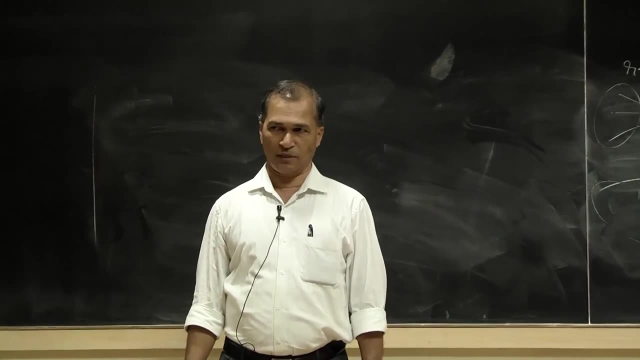 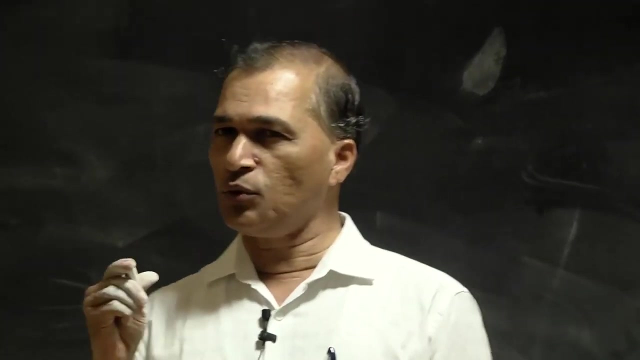 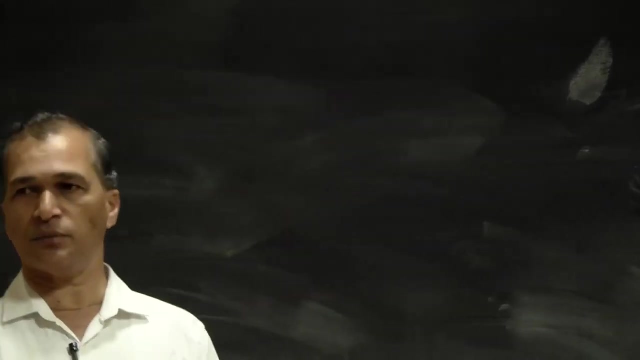 one other person. every two of them know exactly one other person. then there is a person who knows all other persons. right? In terms of graphs, it is that if in a graph every two vertices are adjacent to exactly one vertex, then there is a vertex which is adjacent to 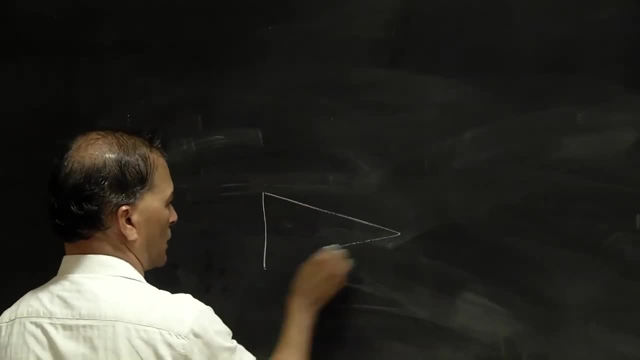 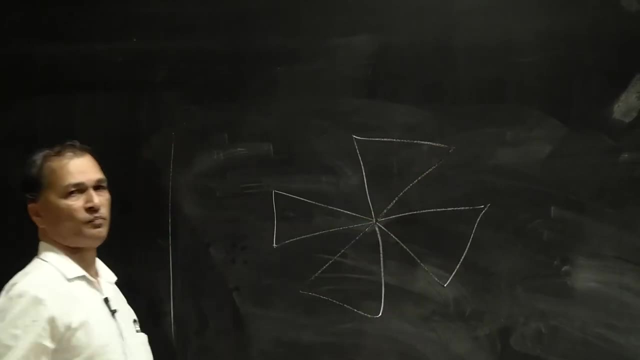 all other vertices, right, And it is this type of graph. We can add any number of triangles. Such a graph is called three-dimensional Industri中国的わか理学, right? Yes, It is a two-dimensional graph, where n is the three-dimensional matrix and y is the 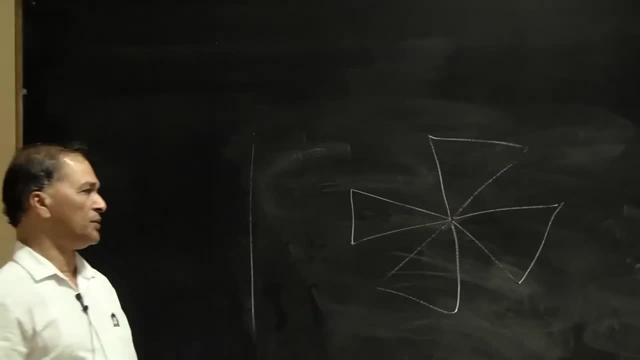 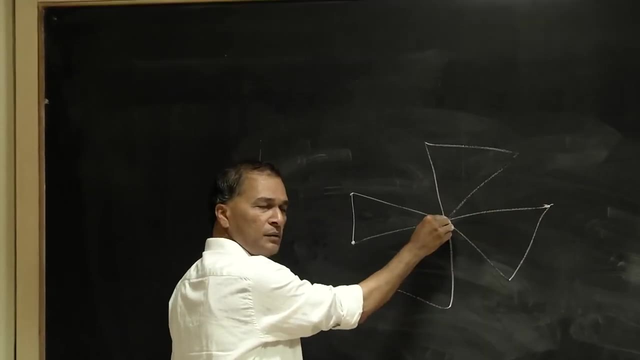 pressure boundary Right. Yes, Yes, Yes, this graph is called friendship graph. if you take any two vertices, exactly one. if you take any two vertices, it is exactly one. there is a vertex which is the same to all other vertices. 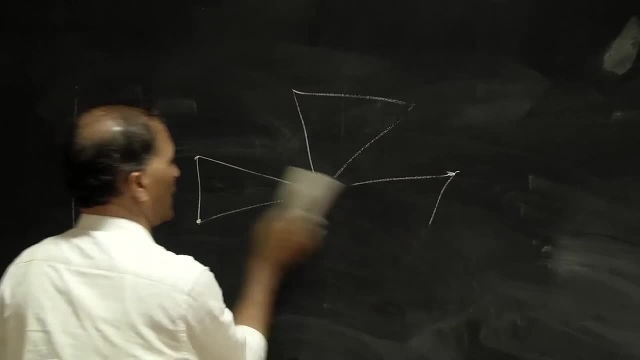 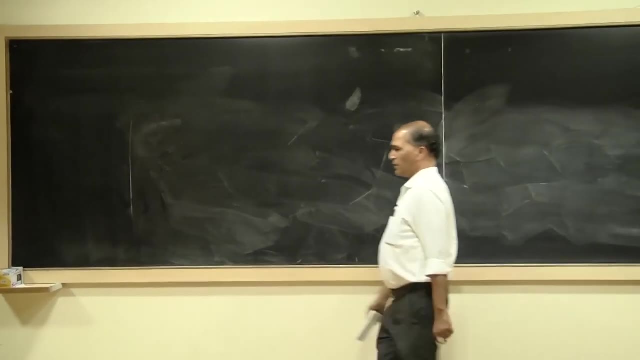 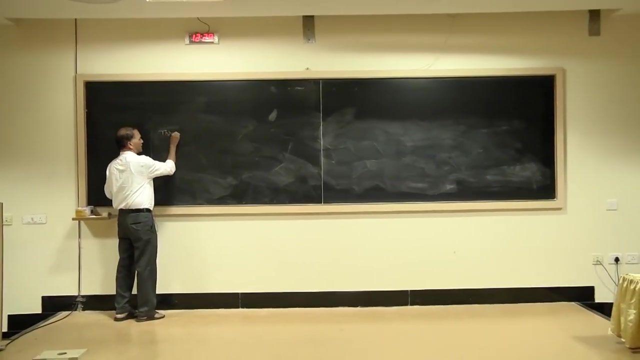 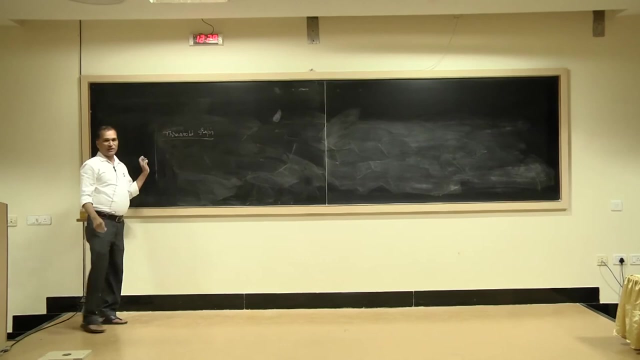 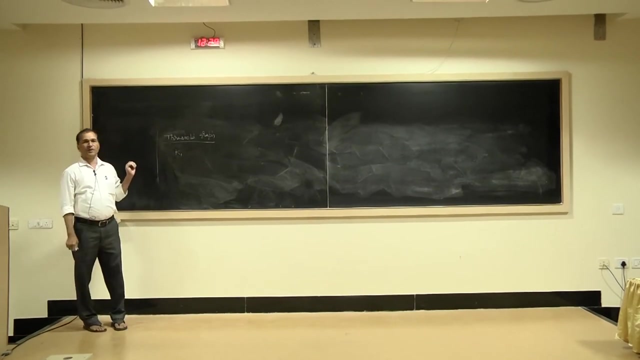 right again, friendship theorem will be proved later, which where we need the concept of eigenvalues and all will be done later, right? the next concept that is needed is that of threshold graph. what is a threshold graph? we start with the graph k1 and we apply the following to: 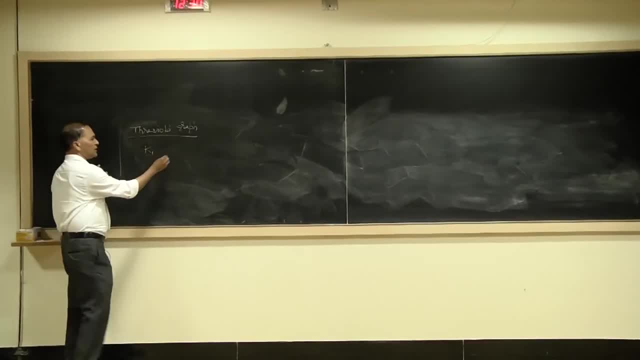 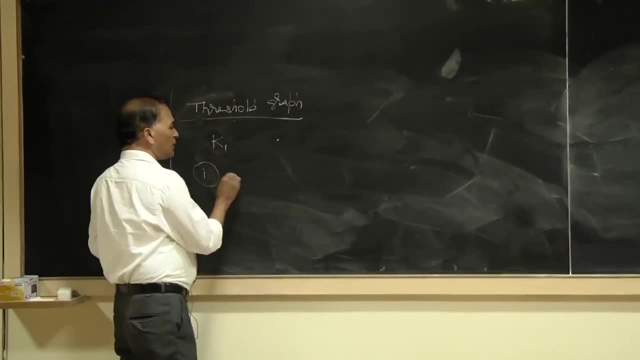 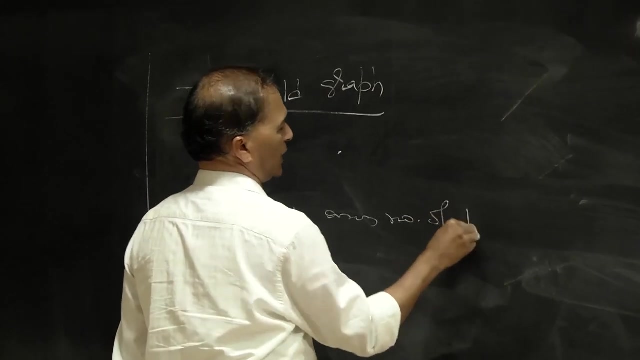 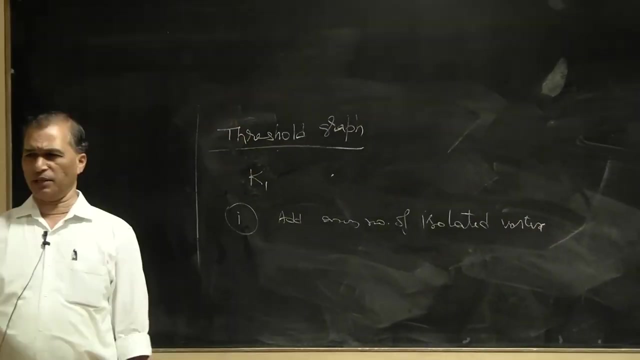 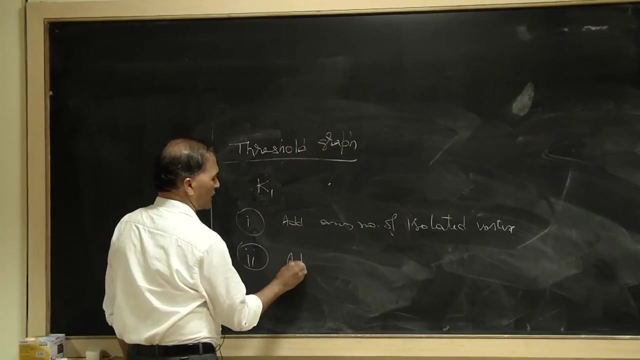 recursively to get the threshold graph right. k1 is a graph with just one vertex. right, you add any number of vertices, any number of isolated vertices. or you can say that: add an isolated vertex, repeat it. right, add a vertex and add a vertex, and add a vertex, and. 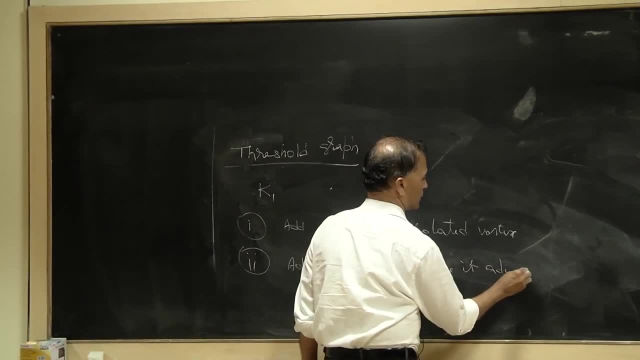 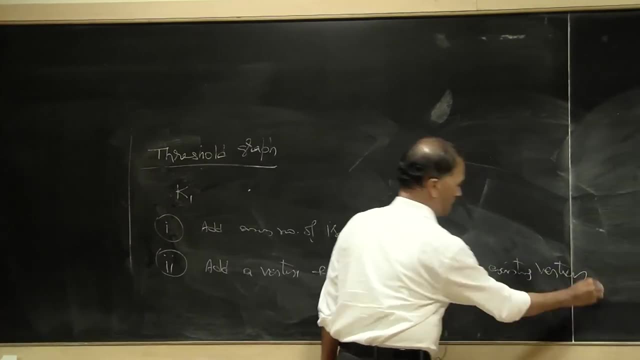 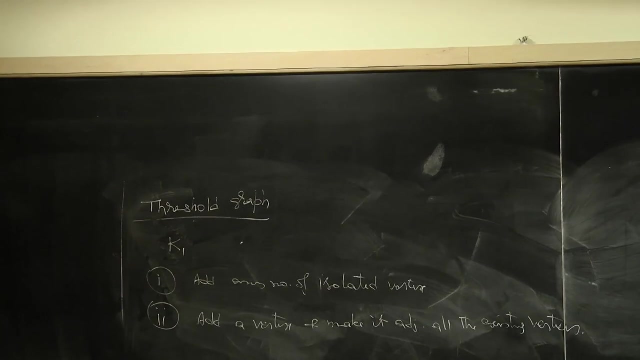 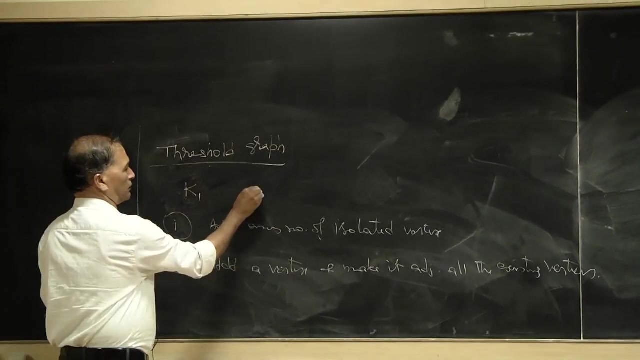 make it adjacent to all the existing vertices. right, we say that it's a dominating vertex. a vertex is said to be a dominating vertex if it is adjacent to all of the vertices, it dominates all of the vertices. right, you start with k1. add a vertex, isolated vertex. this is: 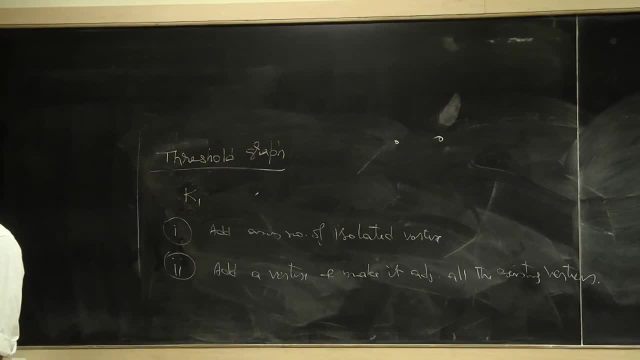 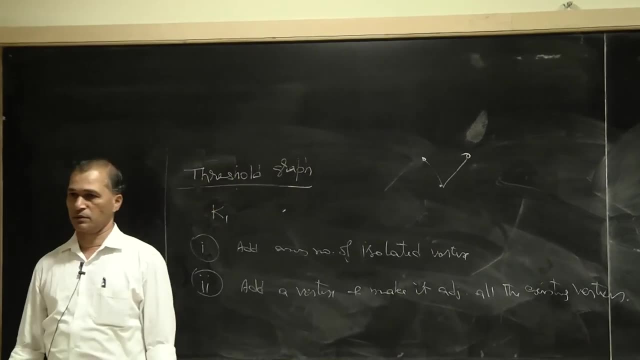 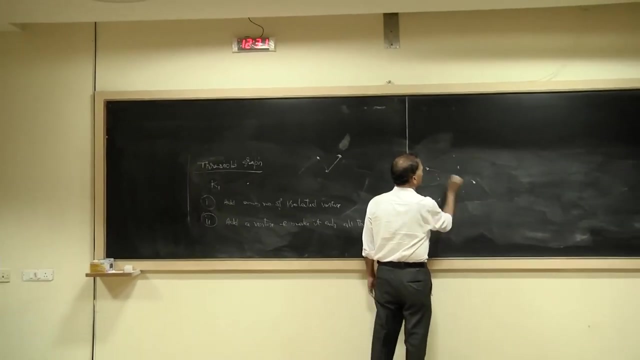 a threshold graph, right? you take a vertex, add a vertex and make it adjacent to all the existing vertices. this is a threshold graph. you take any number of vertices, take a vertex and make it adjacent to all of them, so you apply these in any order, any number of timeswhat result is a threshold graph. 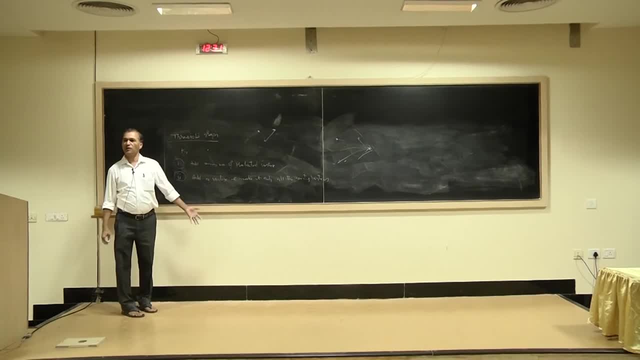 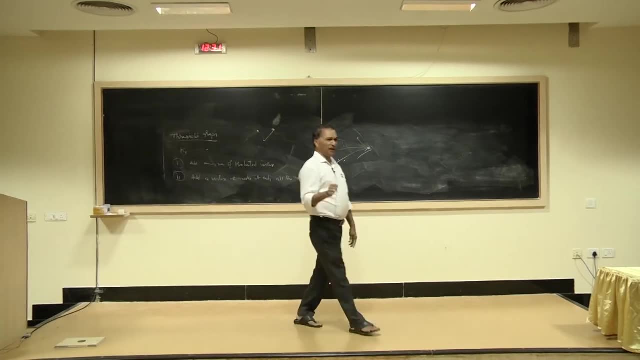 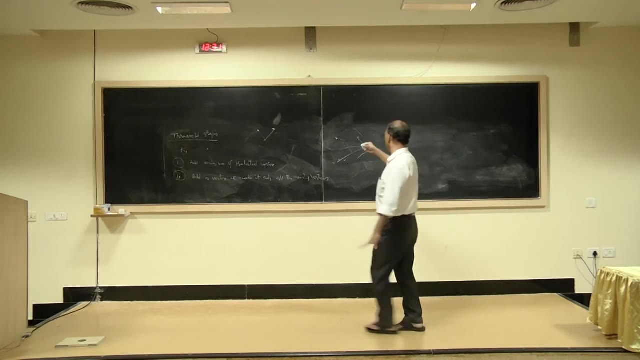 right. so if you take any number of vertices, take a vertex and make it right. If you consider doing this, the first connected threshold graph you get in the sequence is nothing but k1n, is it not? You take some vertices, start with k1, this is disconnected. 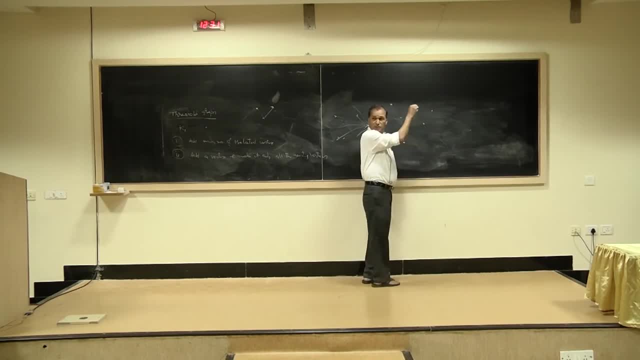 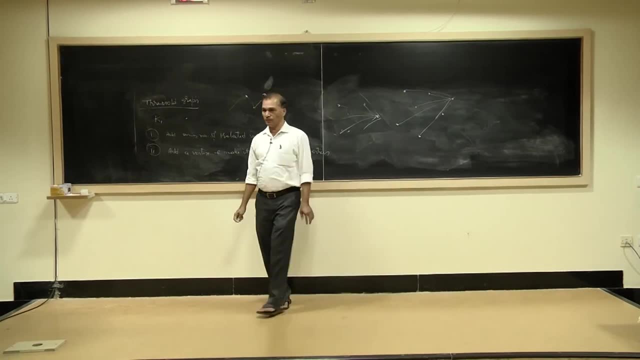 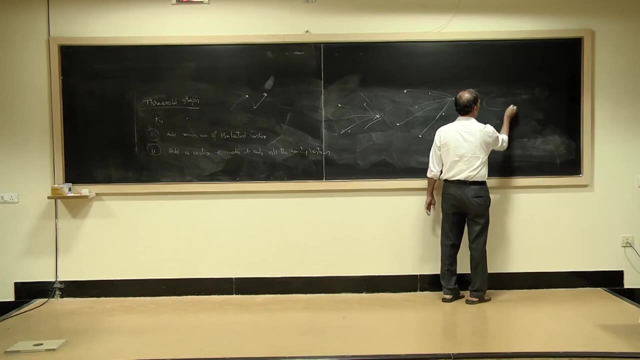 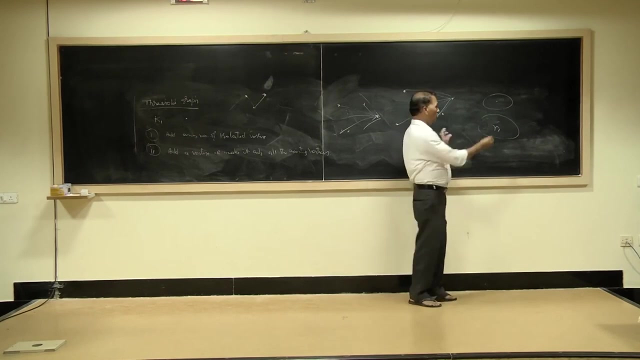 this is disconnected. disconnected. If we take one vertex and make it adjacent to all of them, what do you get is k1n. k1n. it is a star graph, it is a bipartite, complete bipartite graph, with one here and n vertices here. right, This vertex is adjacent to all. 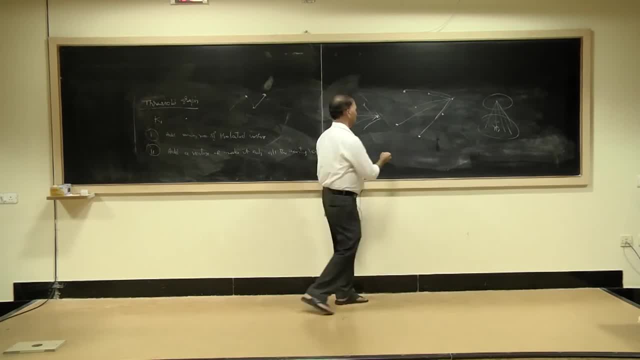 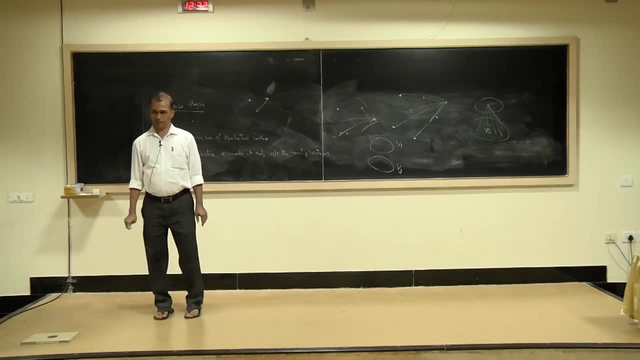 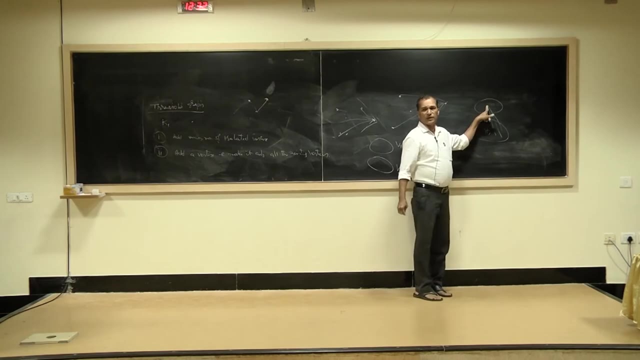 these vertices. a bipartite graph is said to be complete if every vertex of v1 is a vertex of v2 is adjacent to every vertex of v2, right. A bipartite graph is said to be complete bipartite graph. It is a complete bipartite graph where this has one vertex. 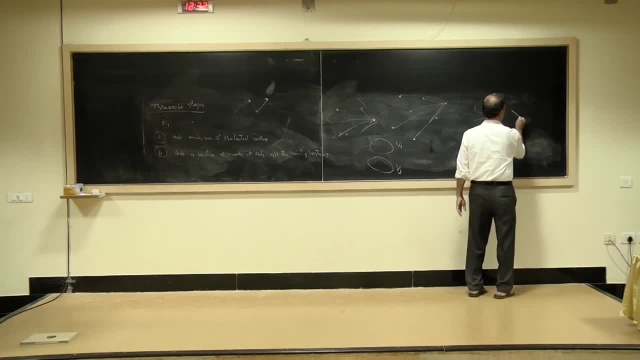 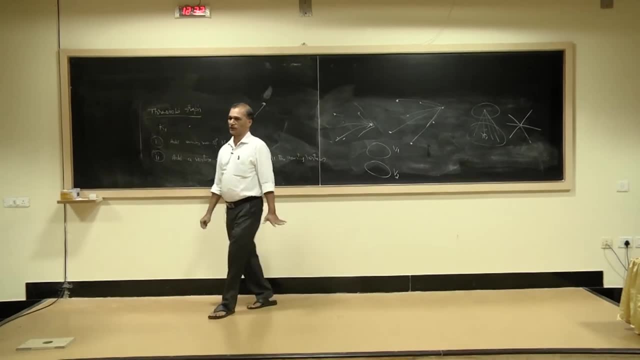 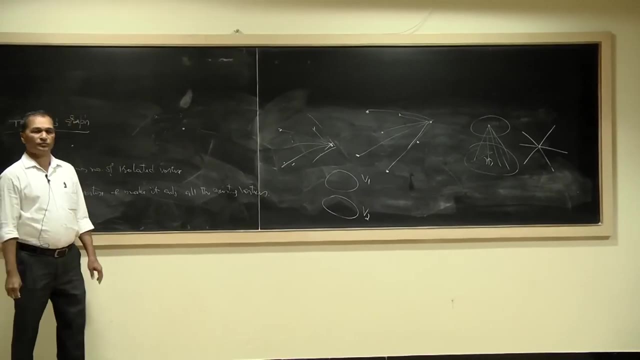 this has n vertices, right? Usually it is called a star graph because it looks like this, right, It is called a star graph. So if you take a vertex, this is a threshold graph- You add another isolated vertex. this is also a threshold graph. this is also a threshold. 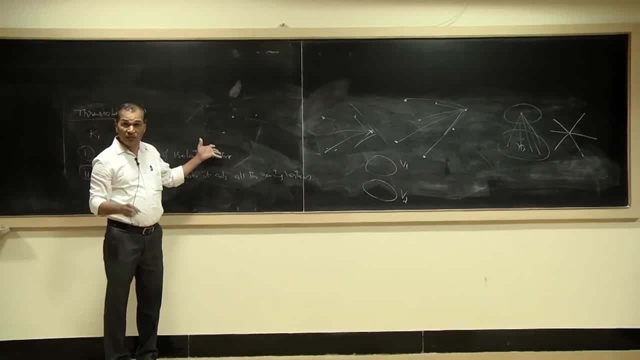 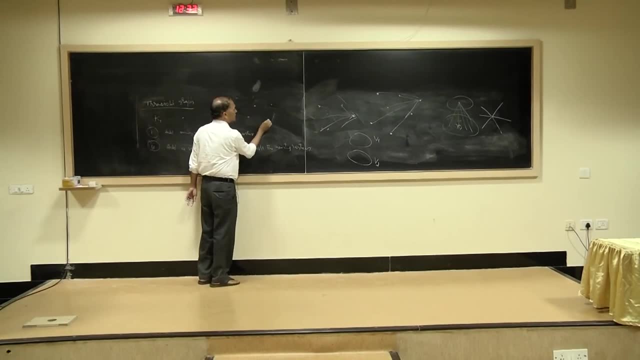 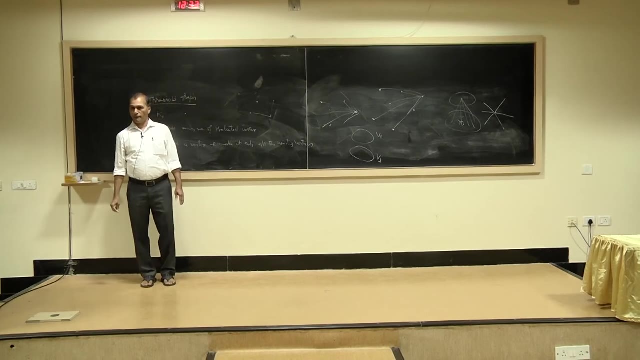 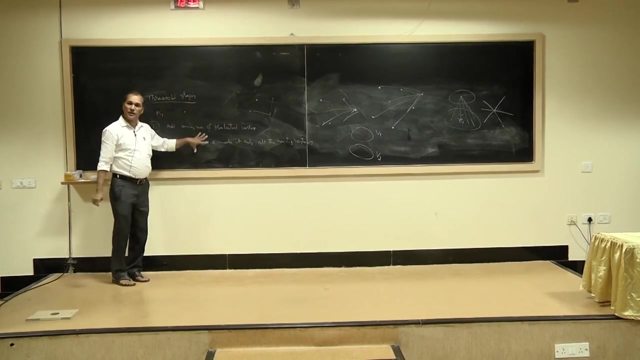 graph, but there it is a disconnected threshold graph. What is the first connected threshold graph? It happens when you add a vertex and make it adjacent to all the existing vertices. So it is nothing but k1n. You can keep, you can apply this one. 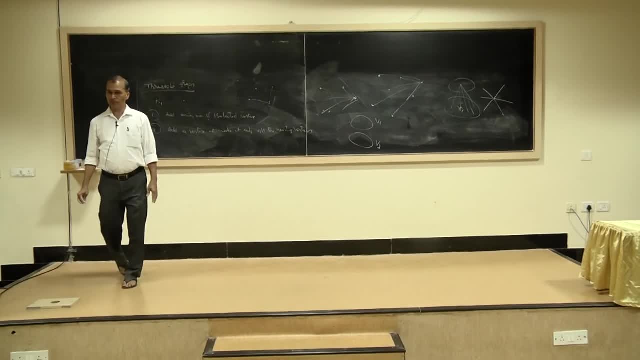 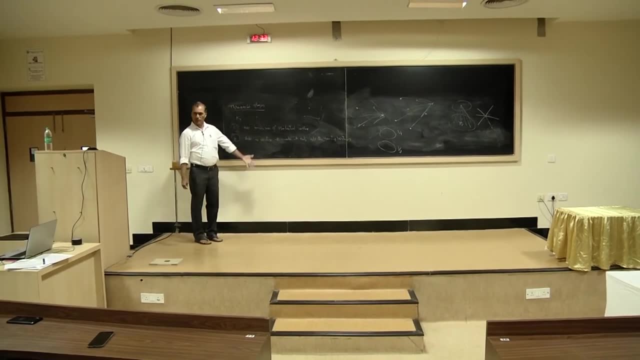 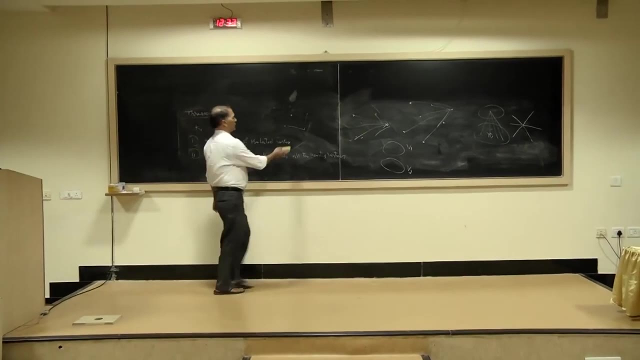 You can keep one in any order. You can apply only one step also, right? You apply this one 0 number of times, any number of times you can apply. right, Then? how to check whether a given graph is threshold graph or not. 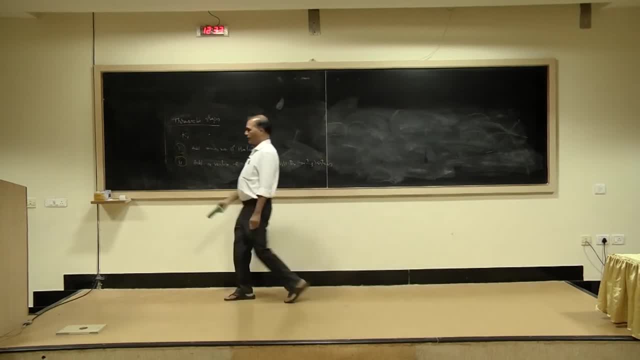 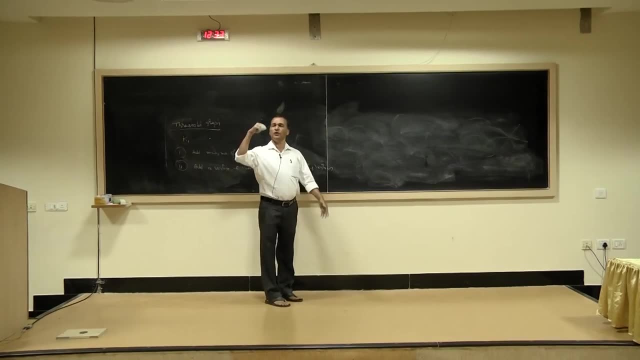 You can apply one more vertex, leave it as it is, Or you can take one more vertex and make it adjacent to all of them. Same thing. If you take, for example, this graph, This is a threshold graph. 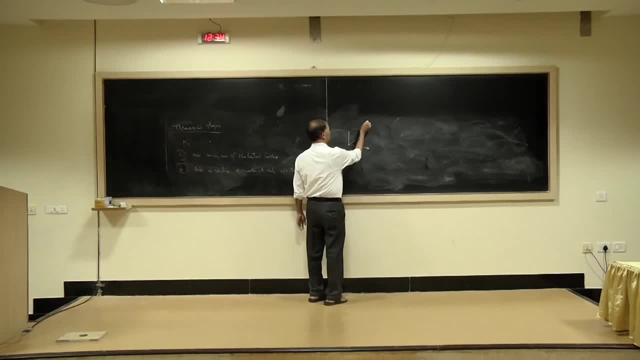 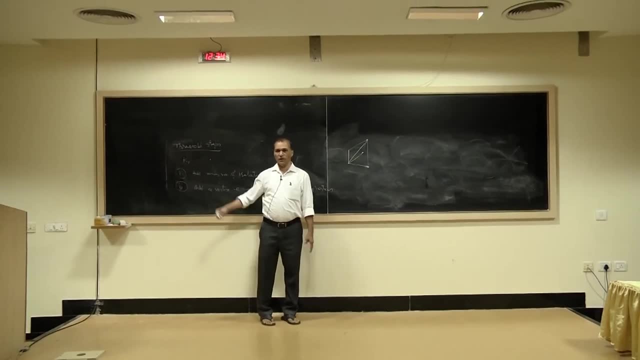 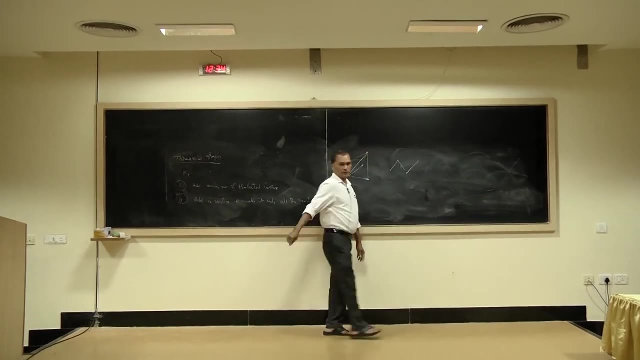 You take a vertex, this is also a threshold graph. You would make this vertex adjacent to all of the vertices. This is also a threshold graph, Right? You can apply any number of times. For example, if you consider this graph, Is it a threshold graph? 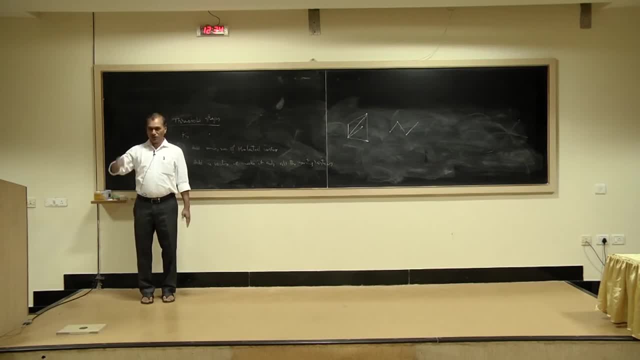 Therefore, the first observation is that If there is no vertex which is adjacent to all of the vertices And the graph is connected, Then it is not a threshold graph. If this, if you take this as a threshold graph- No vertex adjacent to all. 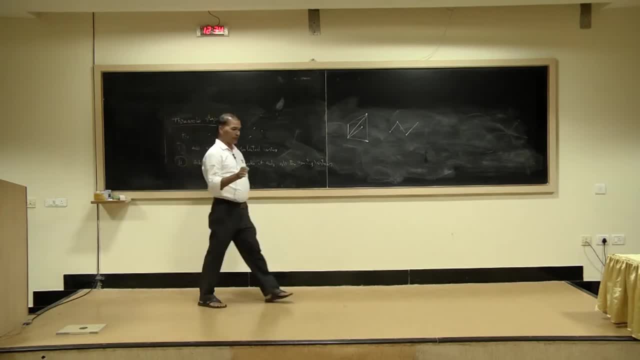 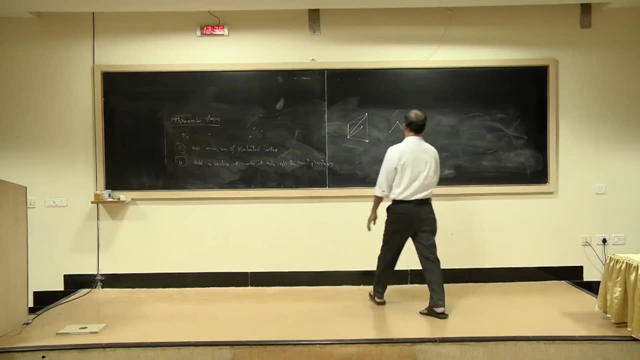 If it is connected graph. A connected graph is a threshold graph Only when it has a vertex which is adjacent to all of the vertices. Then maybe This graph Is it a threshold graph. Why? Why It is not if, and only if. 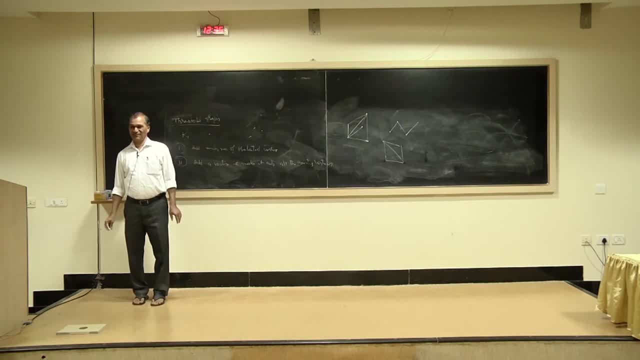 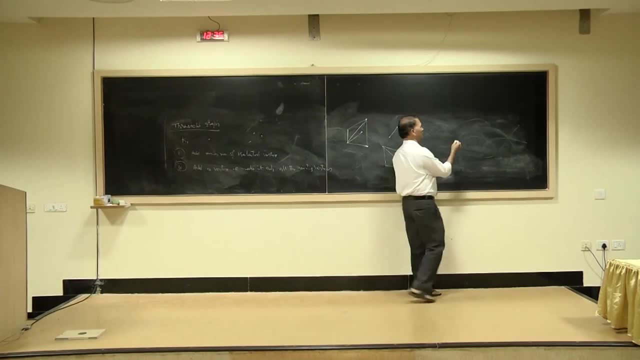 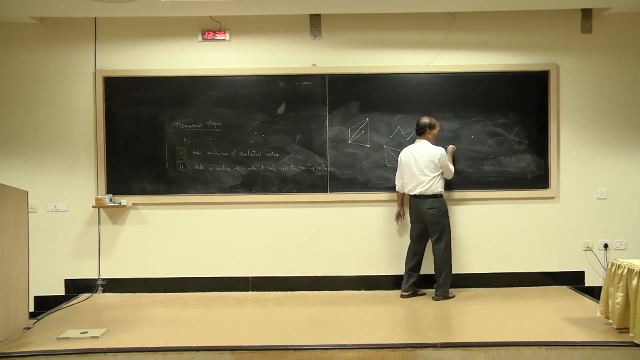 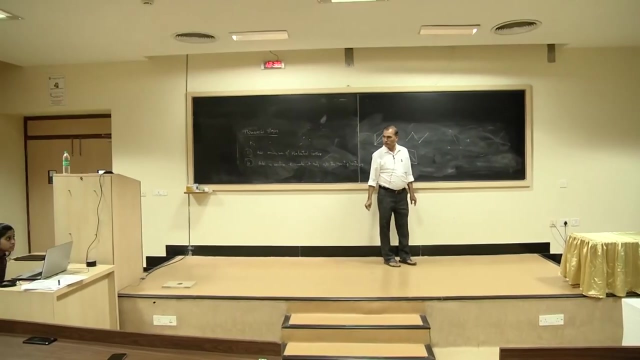 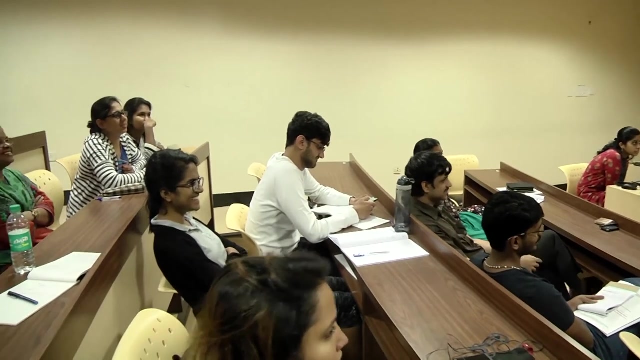 It has to have. Okay, How to construct? you tell me. You start with this: Add three isolated vertices And this one is connected to all of them. There are only four vertices. There are only four vertices. Yes, It can be done. 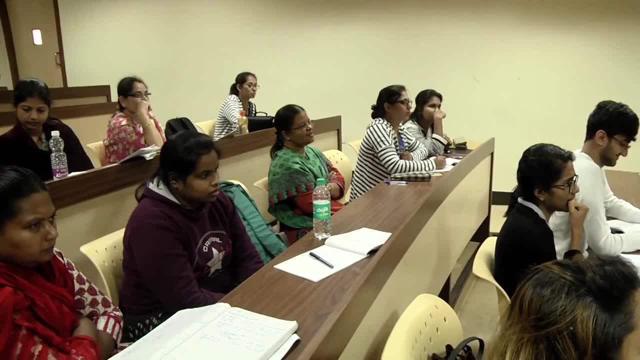 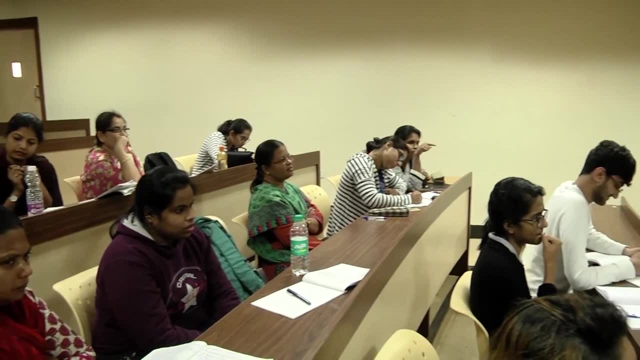 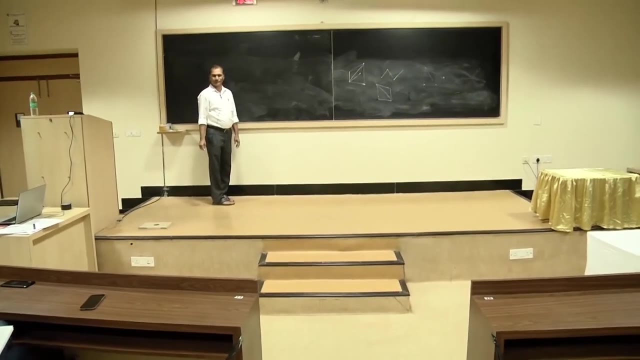 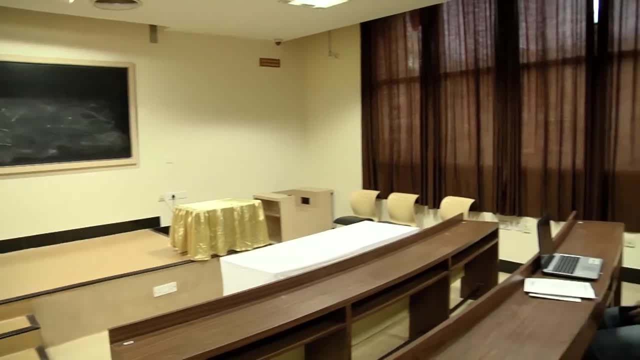 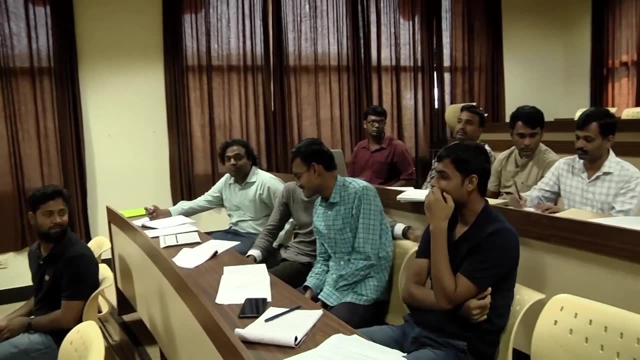 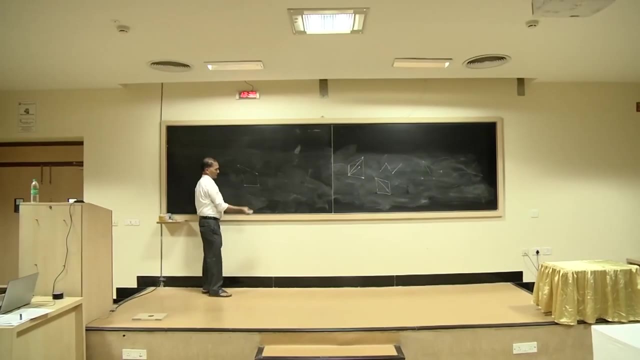 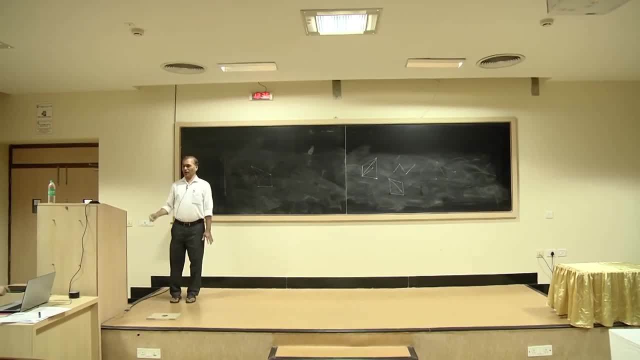 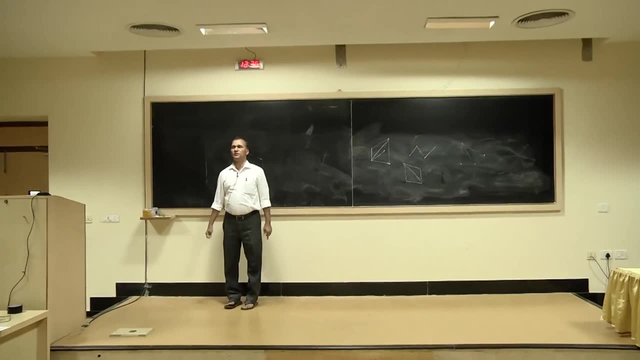 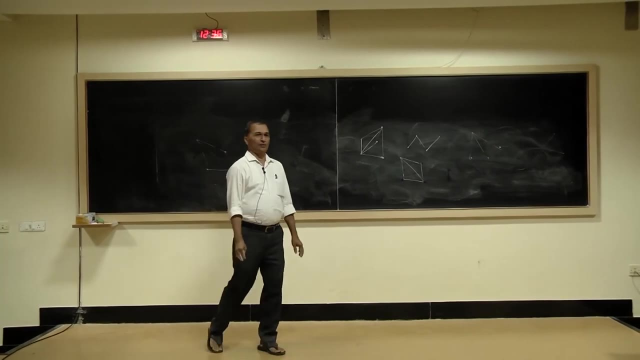 The other way. if you start, you get. So Can you tell me when is it true that a connected graph is a threshold graph? We want to check a graph is given. We want to check a threshold graph whether it is a threshold graph or not connected graph. suppose it is a connected graph. 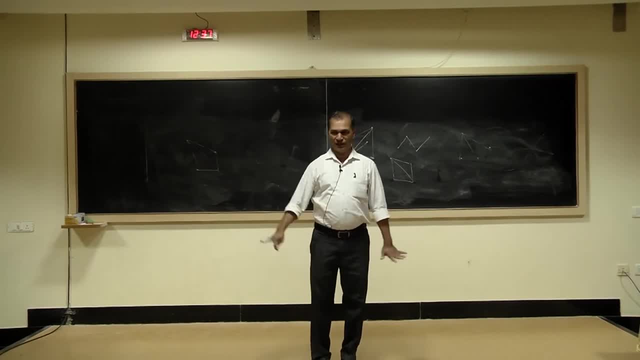 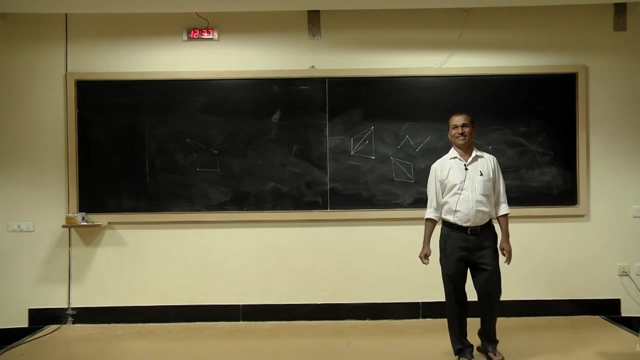 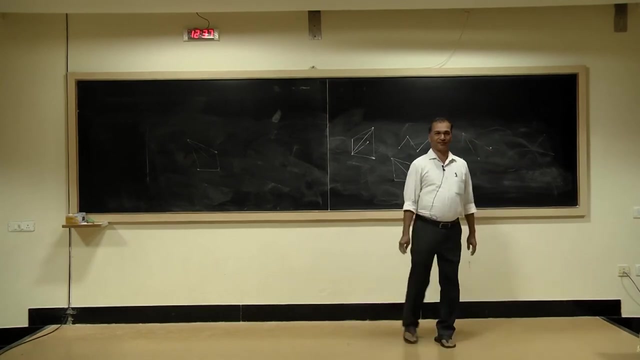 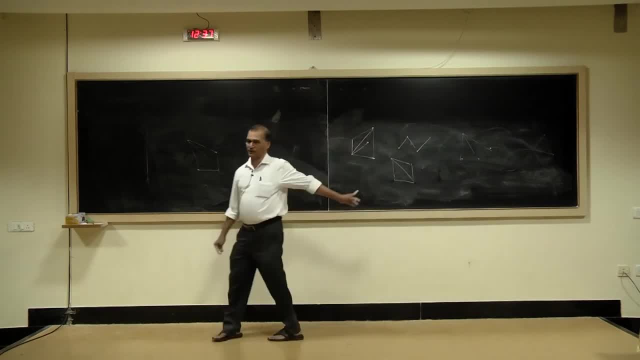 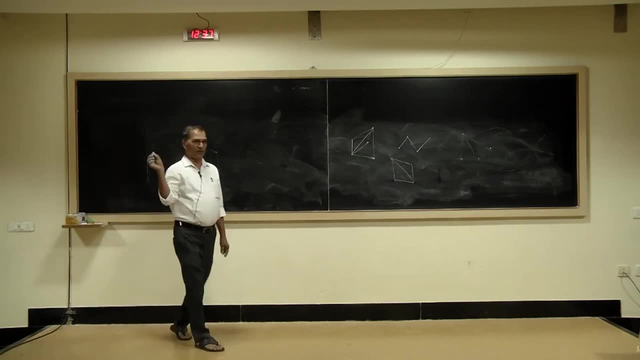 If it is connected. also, it need not be bipartite. right, There is a triangle. it is not a bipartite graph. So first step is that: search for a vertex which is adjacent to all other vertices. Then what we do? We remove that vertex. 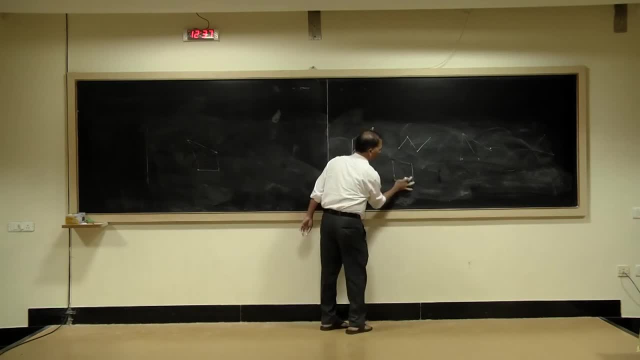 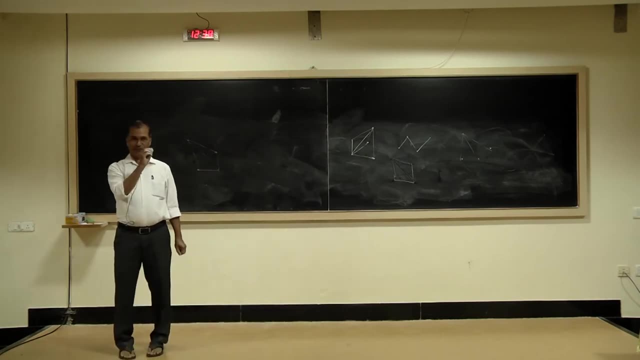 Remove the vertex. what you get- You have to get a threshold graph- may be with some isolated vertices There are. There are one component which is there may exist one component which is not isolated vertices. All other components are isolated vertices. That component, which may not be an isolated vertex, must be a threshold graph. 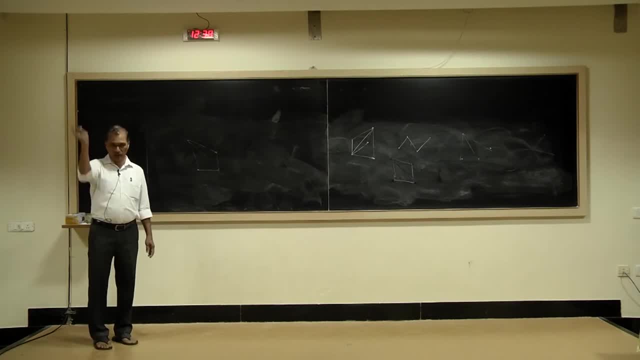 Sequentially May be that there may be a vertex which is adjacent to all of them. Remove that Till you get all isolated vertices. A graph with all isolated vertices is a threshold graph K1.. K1.. If it is disconnected. 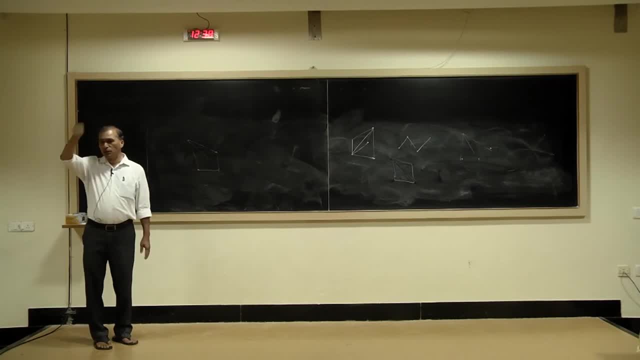 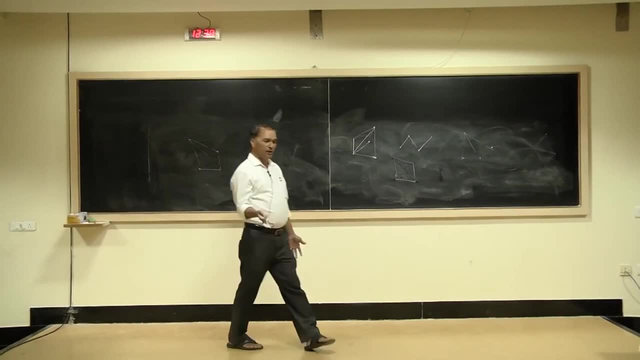 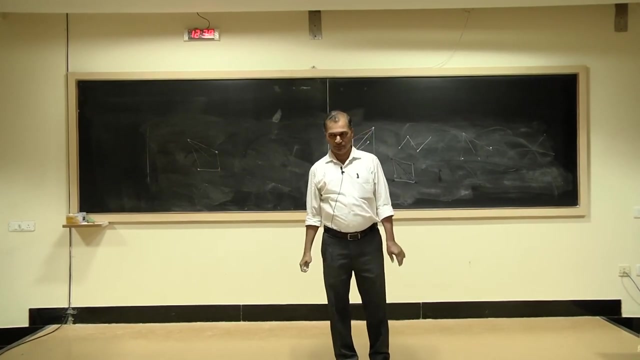 If it is disconnected. you take a vertex and make it adjacent to all of them and check whether it is threshold Or if it is disconnected in order that it has, then also it is true that there is a vertex which is adjacent to all of them, unless it is. all are isolated vertices right. 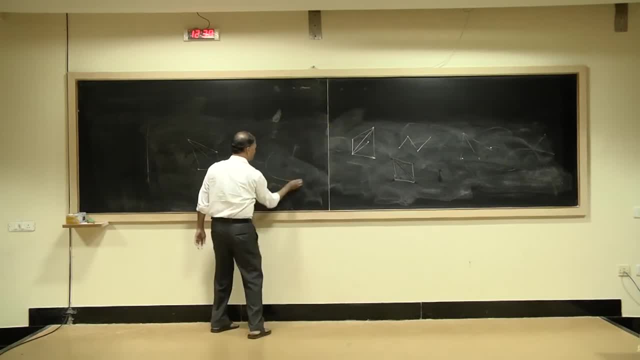 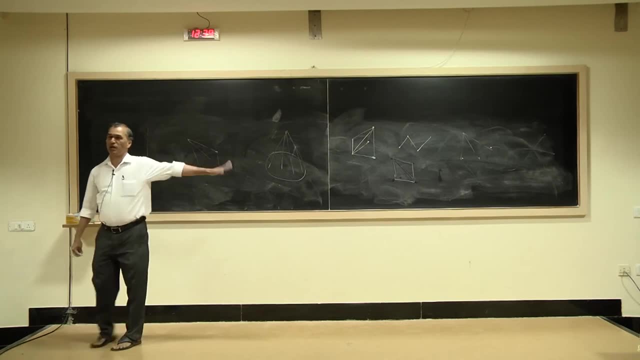 Or if it is a. the easiest way is, if it is a disconnected graph, take a vertex and make it adjacent to all of them. Check whether it is threshold. Check whether it is threshold because it comes back to the second step over there right. So this threshold graph has very good properties in terms of its eigenvalues. 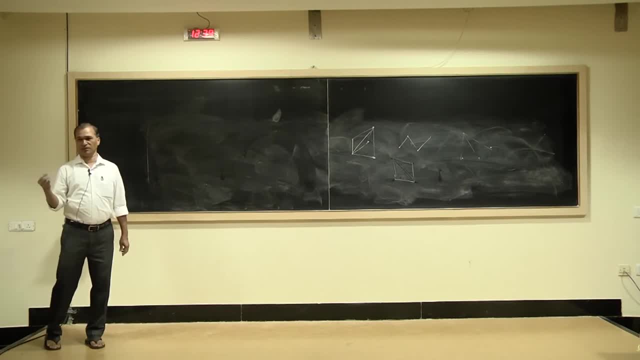 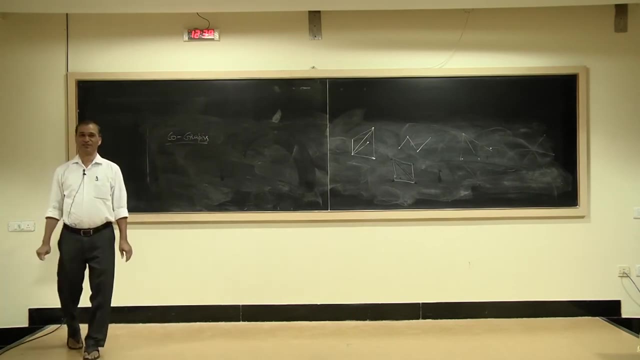 So, which will be done later, may be with by Manjunath Prasad. It has very good properties in terms of the eigenvalues, and next graph that is required for- Not for me to Bapat, sir- is co-graph. What is a co-graph? 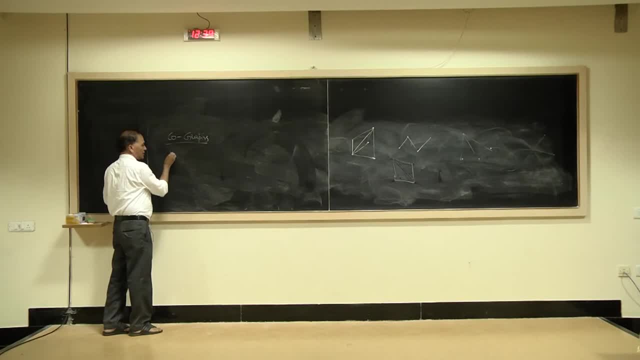 Again recursively. we define it like this: We start with K1.. K1 is a co-graph. Then the second step is that complement of a co-graph is a co-graph Right. The second sentence in the definition says that complement of a co-graph is a co-graph. 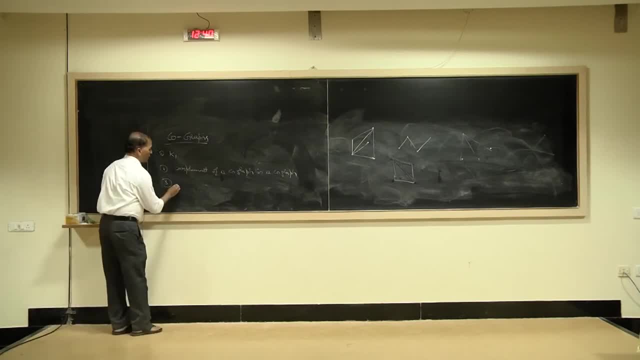 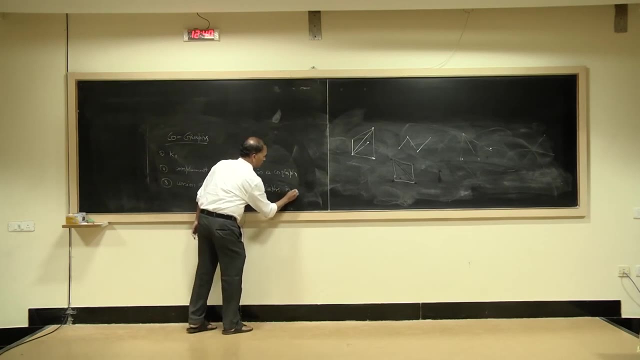 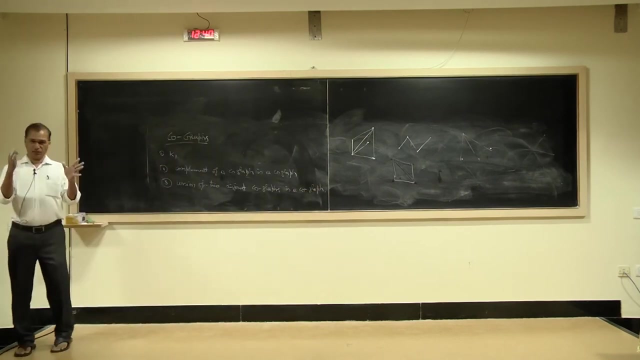 Then third sentence is that union of two disjoint edge, I mean vertex disjoint co-graphs, is a co-graph. Right Union of two vertex disjoint co-graphs is again a co-graph. This is the definition. Again I give an example for a co-graph other than one vertex. 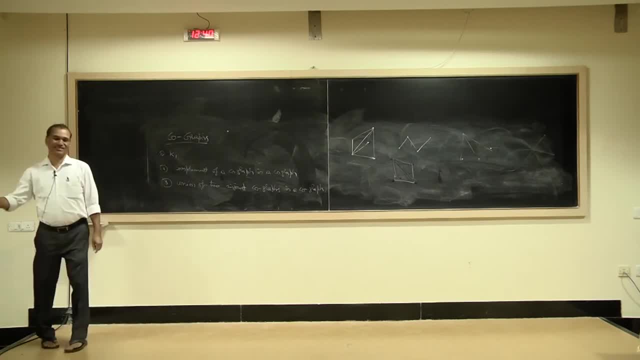 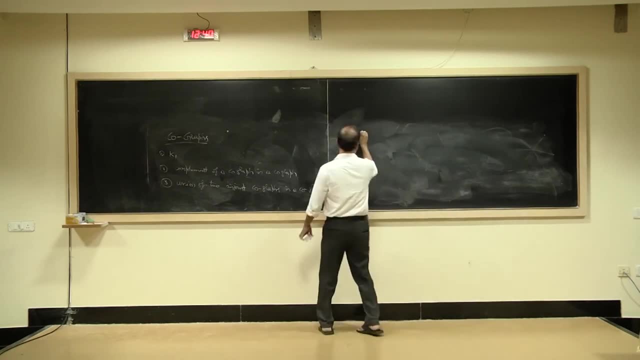 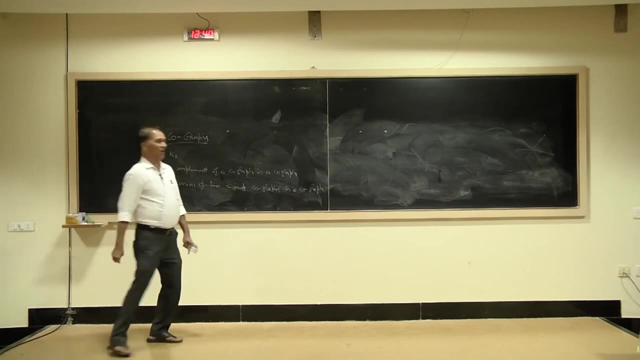 This is a co-graph. If this is a co-graph, then this is also a co-graph. Two disjoint vertex disjoint graph Right, Two point vertex disjoint graphs placed together is a co-graph. If this is a co-graph, then its complement is a co-graph. 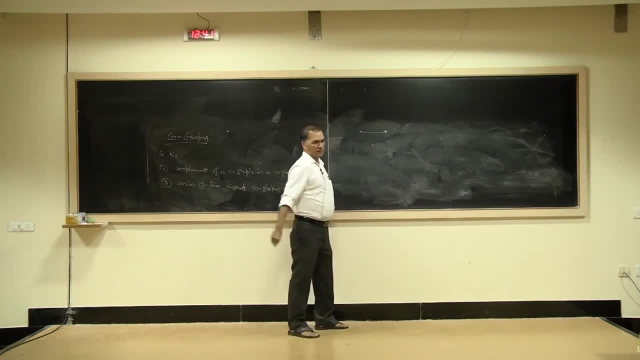 So K2 is a co-graph And add one vertex: Right, This is a co-graph. May be that you can consider this one. This is a co-graph. Complement is a co-graph, Right? Therefore every complete graph is a co-graph. 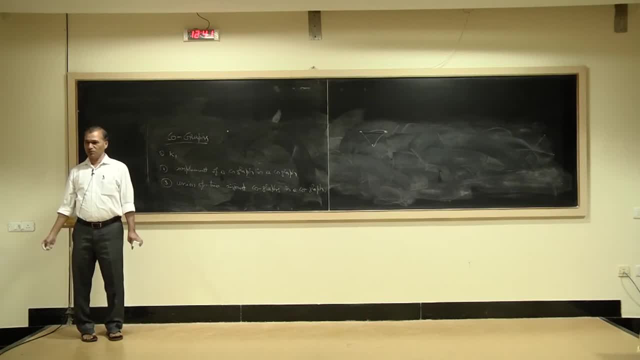 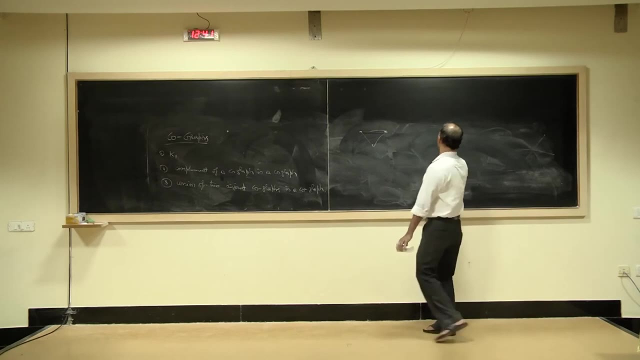 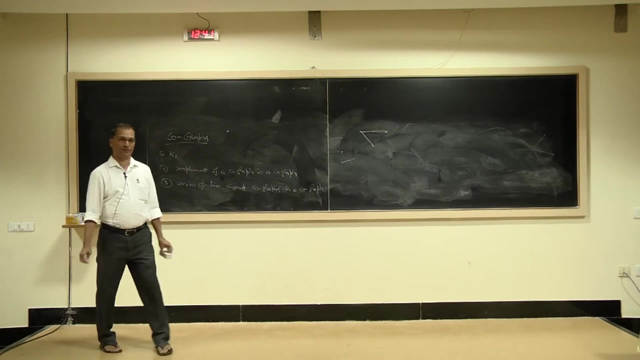 Every totally disconnected graph is a co-graph. Give an example which is not a co-graph. Delete one edge from this. What is the complement of this? Is it a co-graph? If this is, then a co-graph, If this is then a complement: is a co-graph. 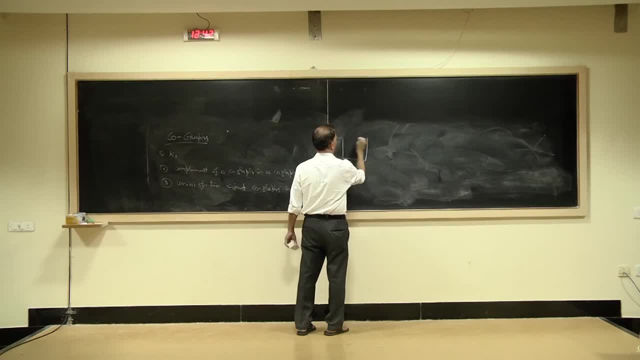 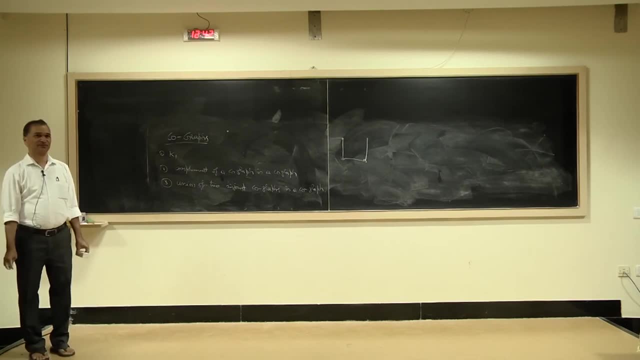 Sub-complementary graph. This one is a co-graph or not, Right? This is a co-graph. This is a co-graph. Can it be generated using this? Is it a co-graph or not? It is not a co-graph, Right? 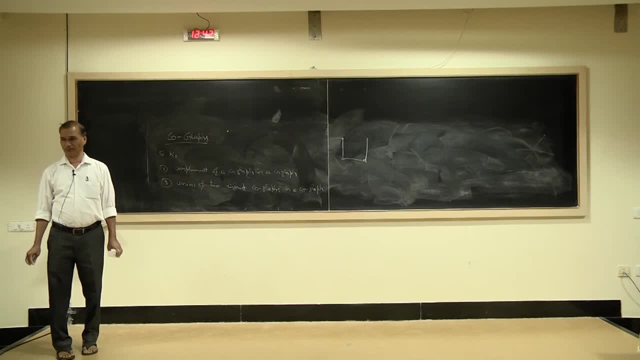 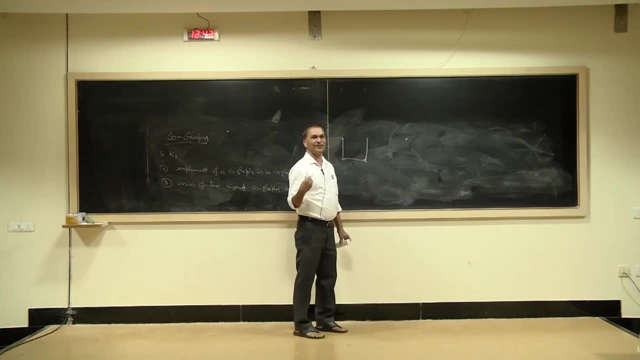 Now tell me: is it true that every threshold graph is a co-graph? In order that it is a co-graph, Suppose that we start with a vertex. I think so. this co-graph is nothing but a Kali graph. What is Kali graph? 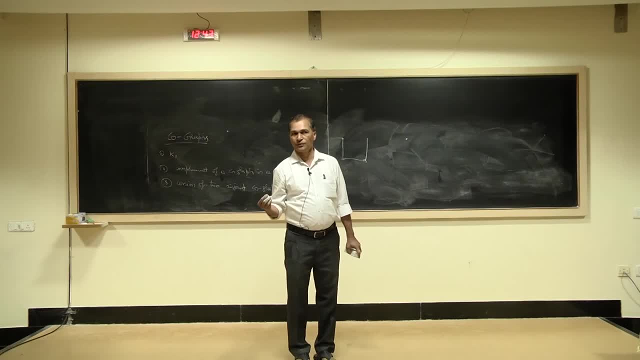 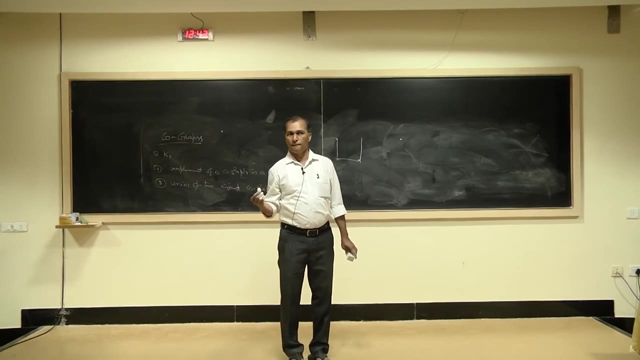 Kali graph is somebody creating a vertex. A Kali graph has a set of the graph, Magnetic graph. You create a Kali graph. So set of edges are the vertices of the vertex. Set of edges are the vertices of the vertex. 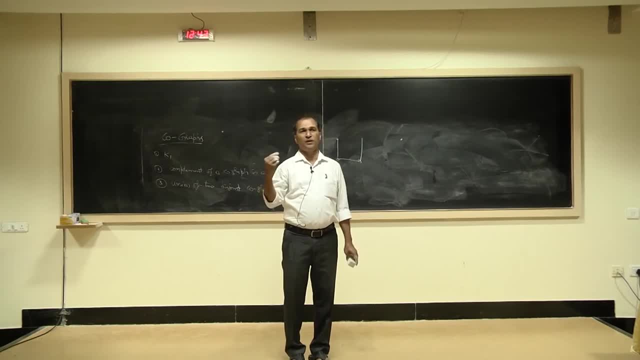 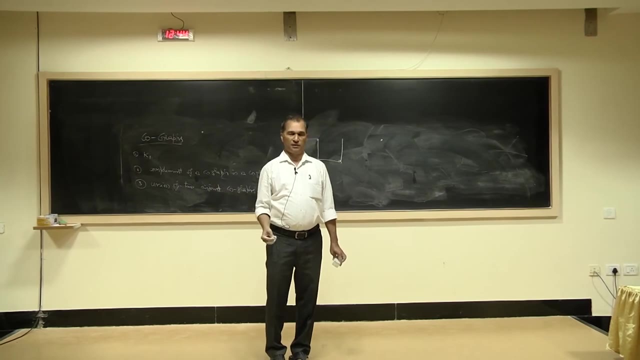 Set of edges are the vertices of the vertex. So set of edges are the vertices of the graph and we make them adjacent Line graph. you mean We make them adjacent. They are not lying in the triangle, They do not lie in a triangle. 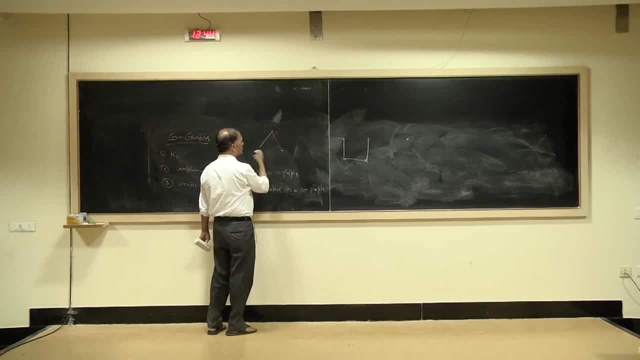 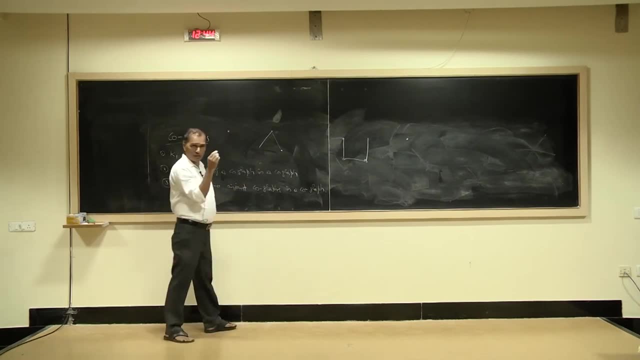 Two vertices are adjacent, Two edges are adjacent And that means this edge must be missing. Any two vertices are adjacent in the Kali graph to vertices are adjacent in a calligraph if the corresponding edges they do not lie in a triangle, then it is obvious. if you say that this graph and calligraphs are same, then co. 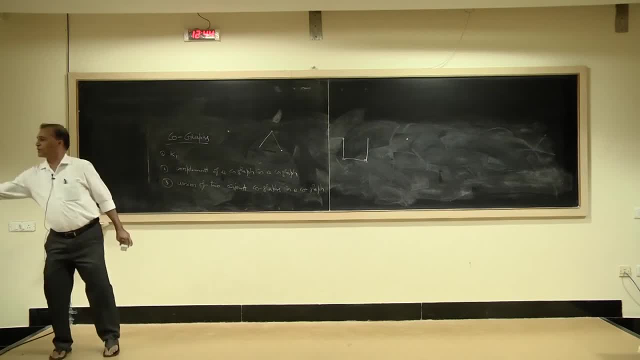 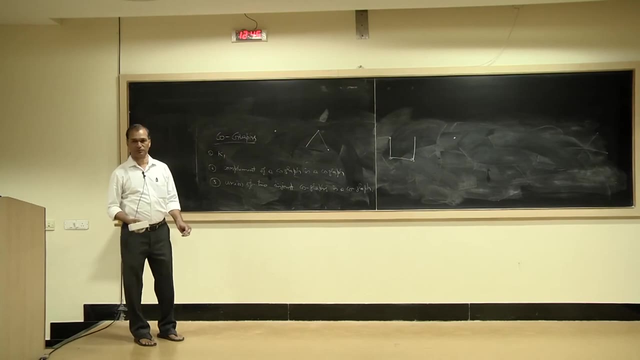 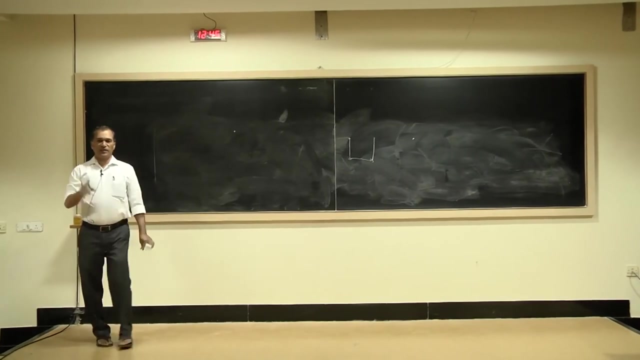 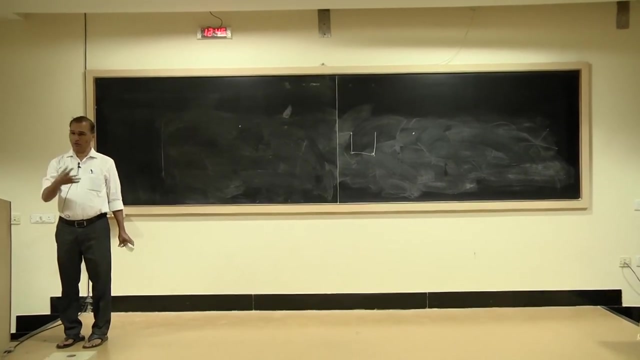 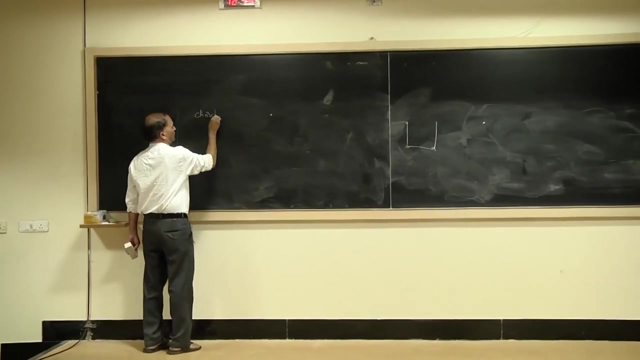 graph is well defined. it is there in- I am referring this book- graphs and matrices by RB Bapata. I am doing that part of graph theory which is required for doing this. ok, no problem. finally, we define one graph we will do, And that is called caudal graph. we will finish this and we may be we can discuss it afterwards. 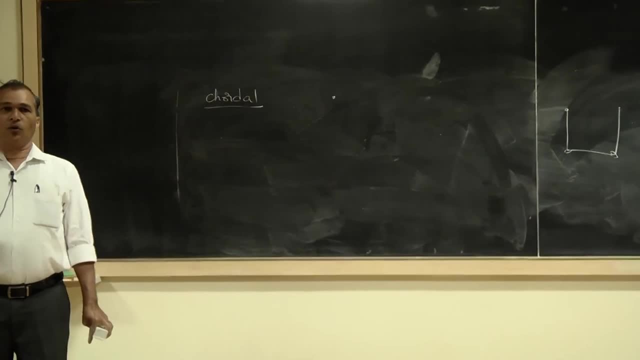 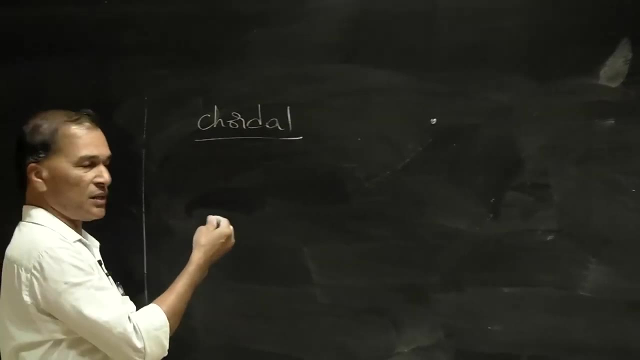 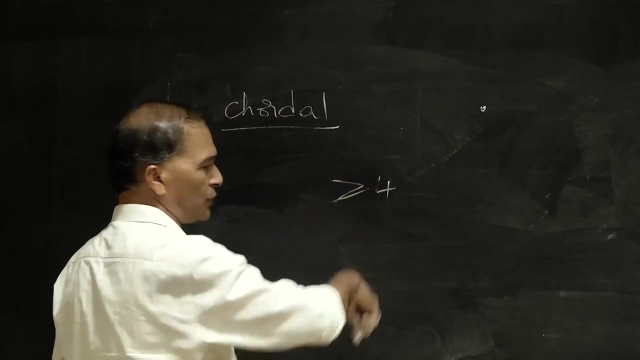 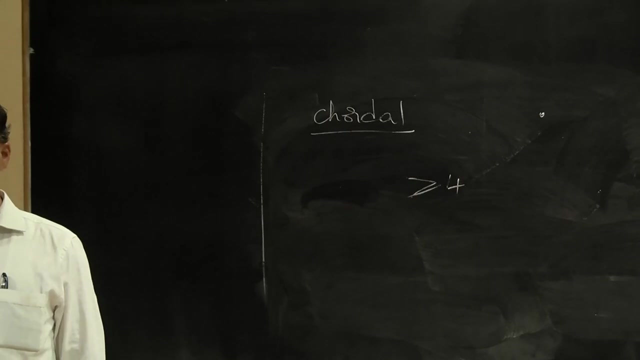 also we will be here only right. What is a caudal graph? caudal graph is a graph which in which every cycle of length greater than or equal to 4 has a caudal. A graph is called a caudal graph if every cycle in the graph of length greater than 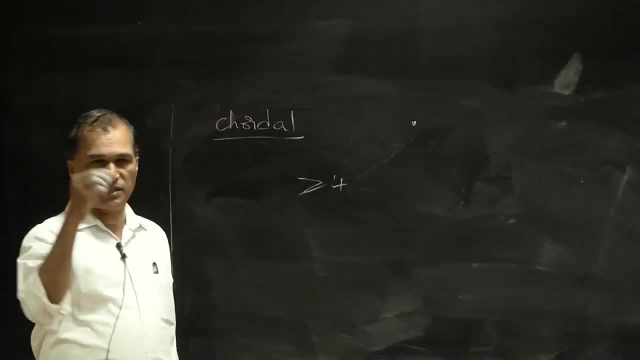 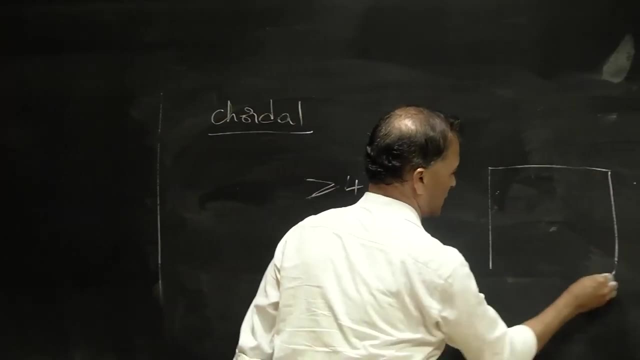 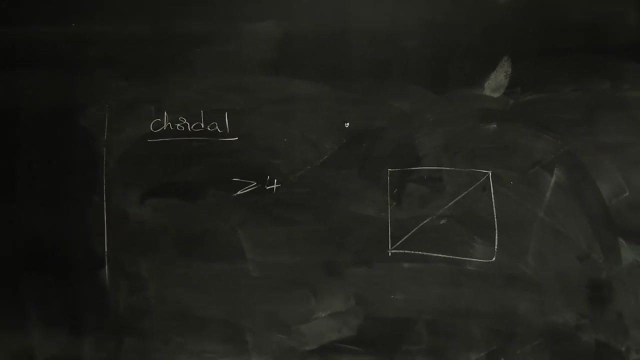 or equal to 4 has a caudal. caudal means what it is: the edge joining two vertices which are not adjacent in the cycle. For example, if you take, consider this one, this is a caudal right. or you can say that: the graph does not contain. 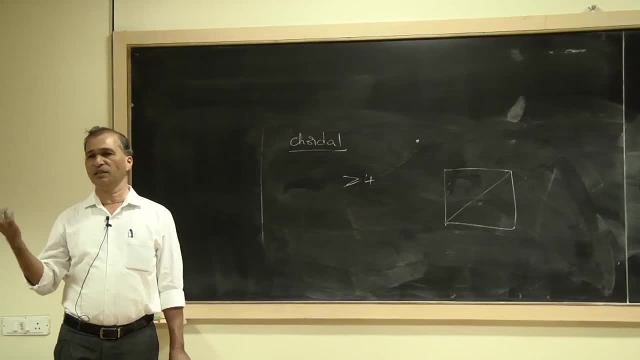 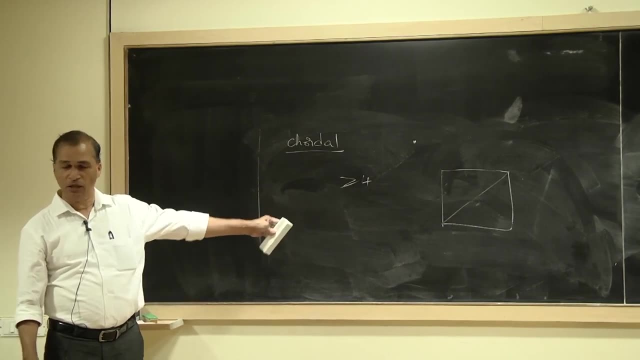 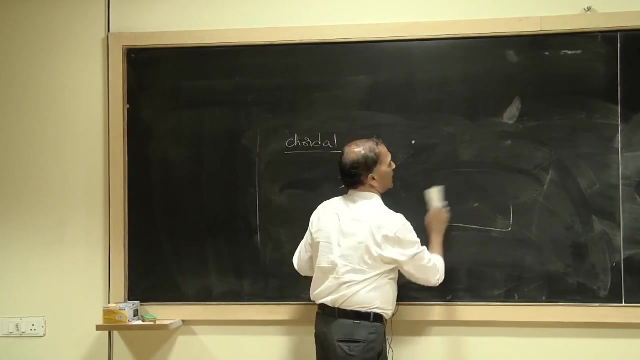 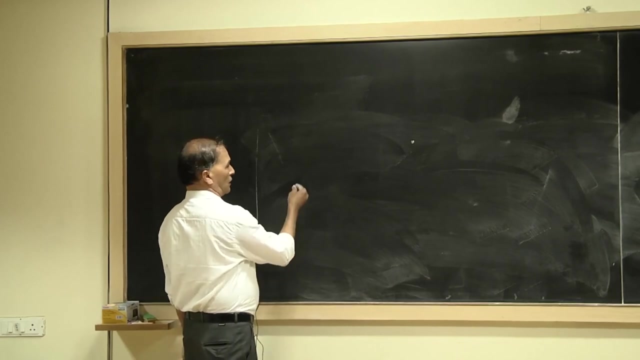 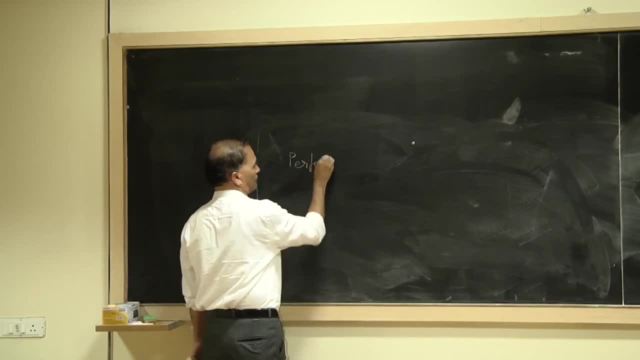 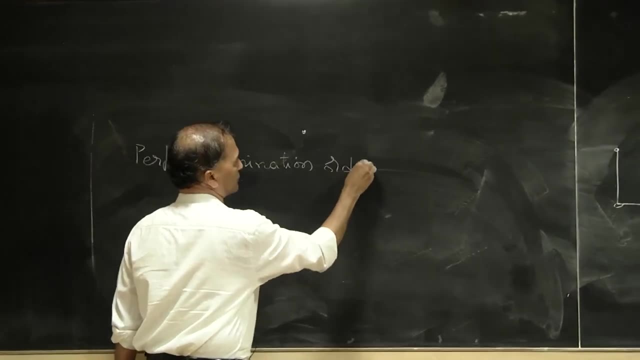 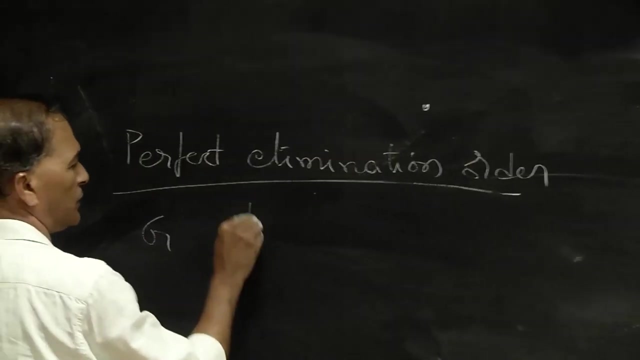 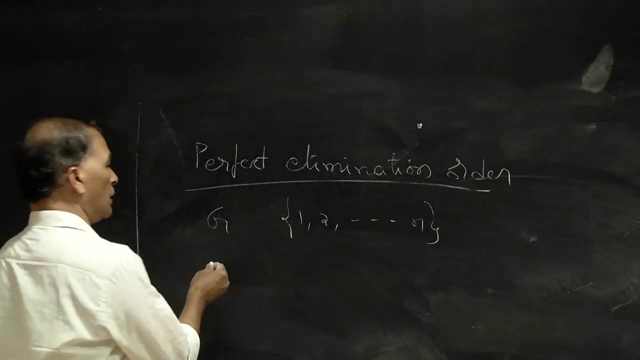 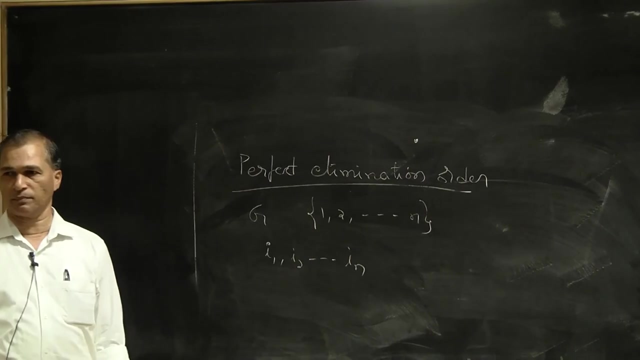 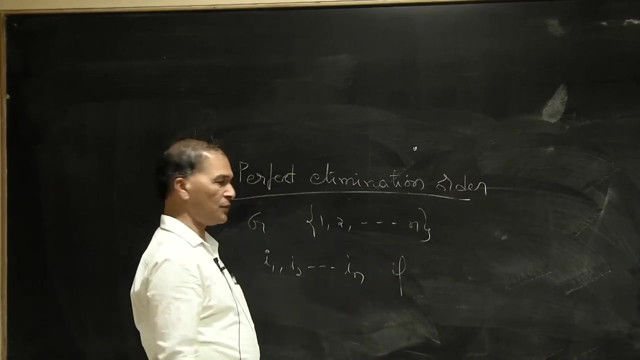 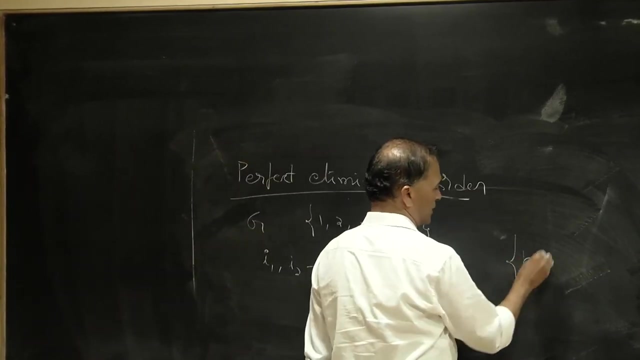 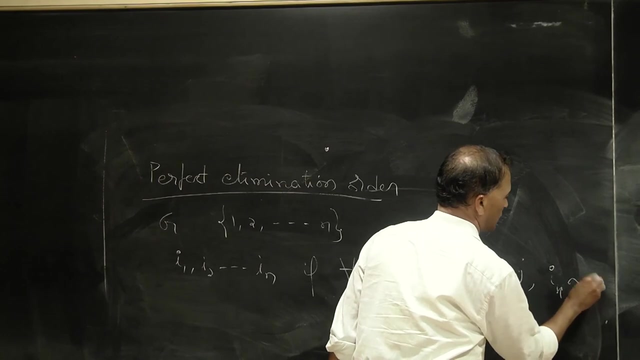 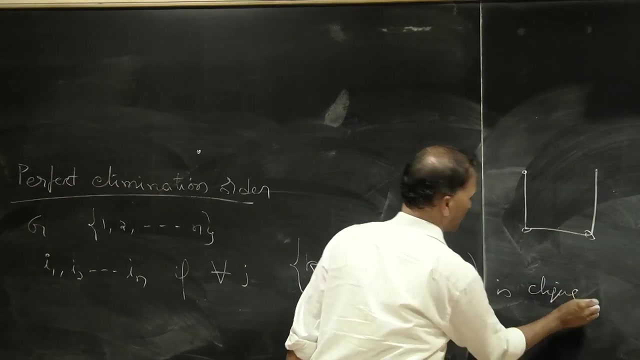 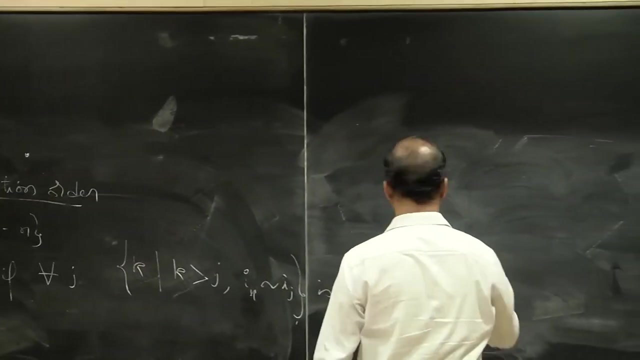 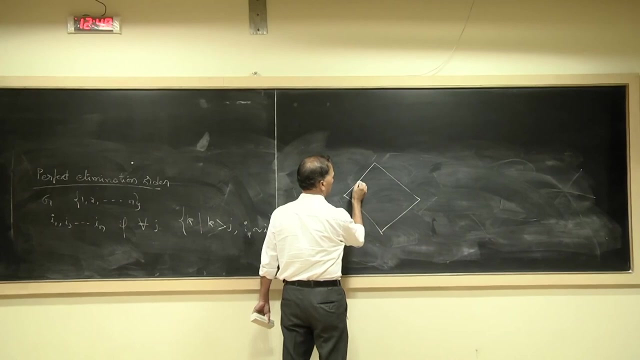 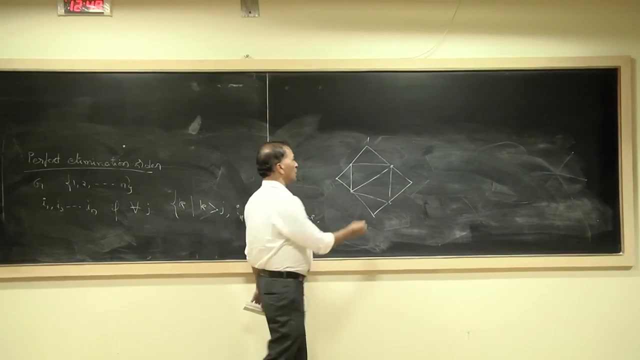 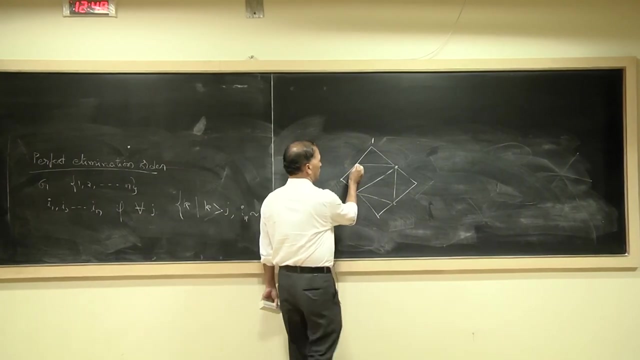 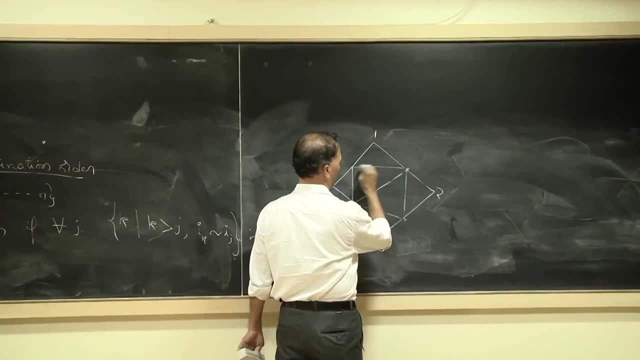 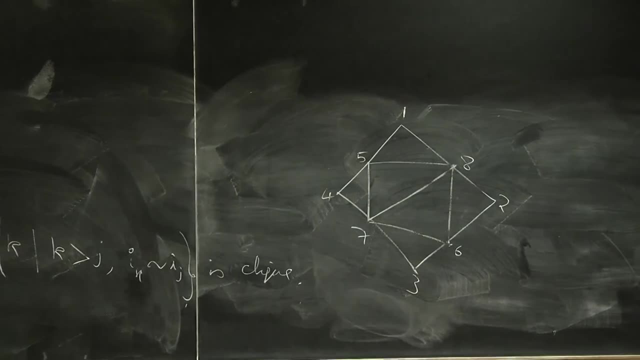 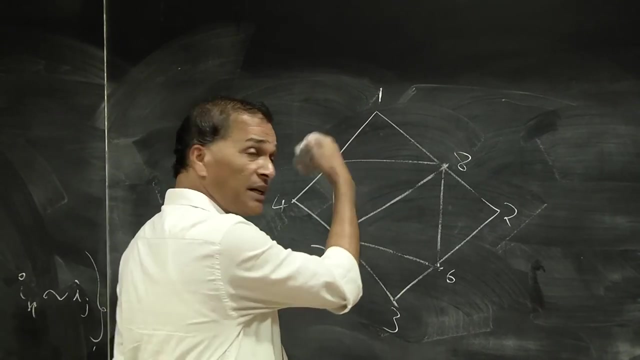 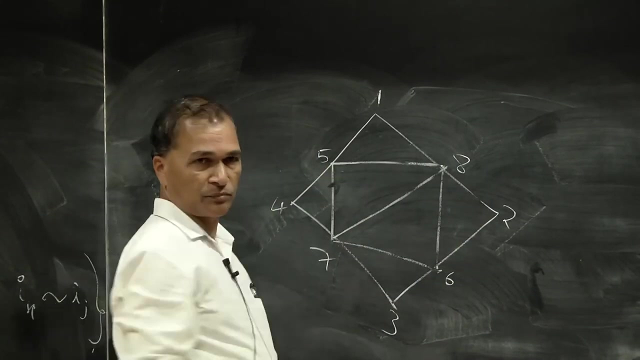 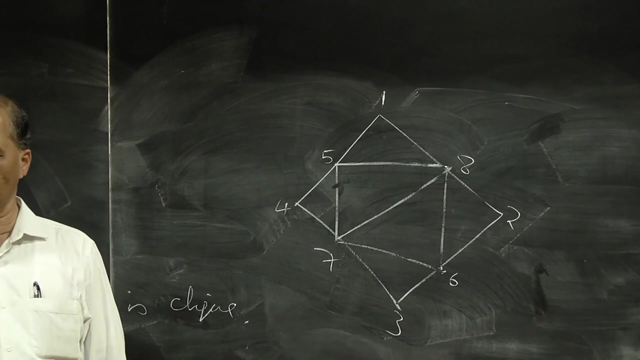 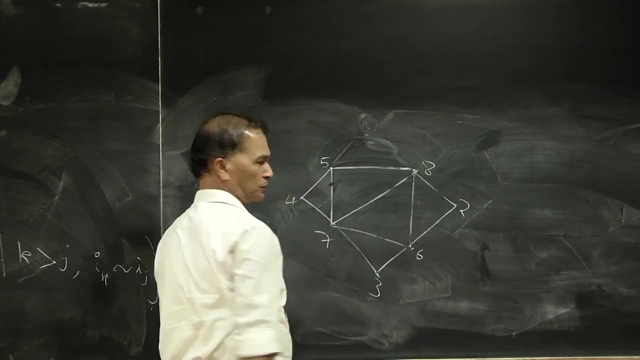 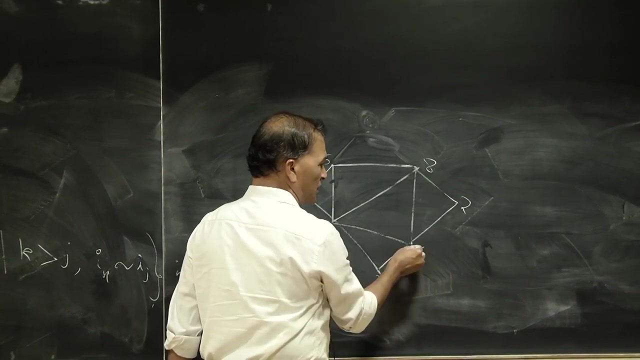 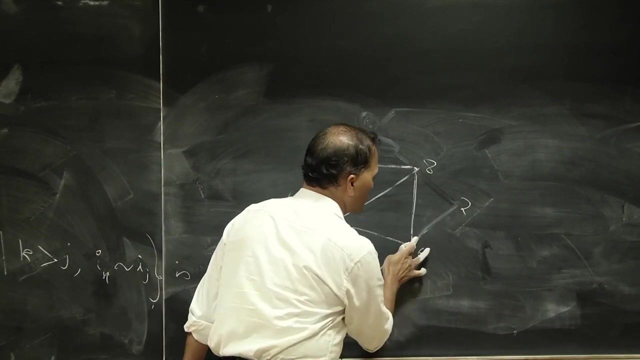 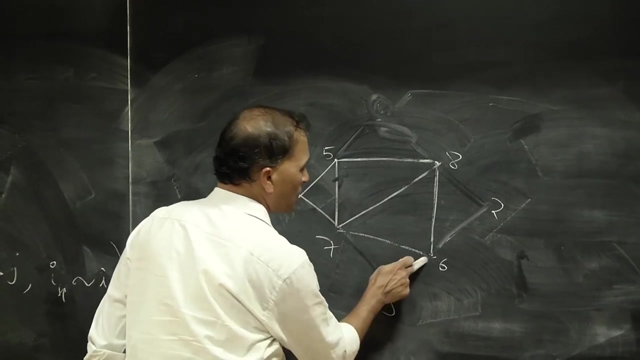 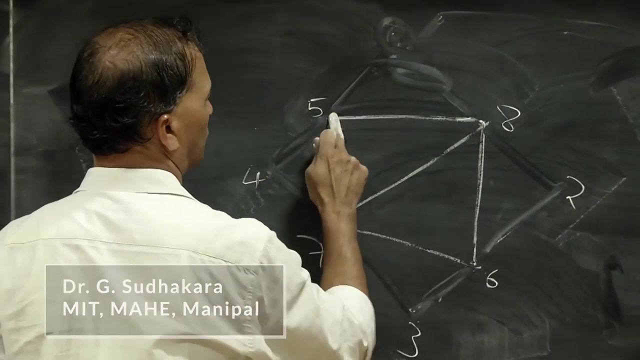 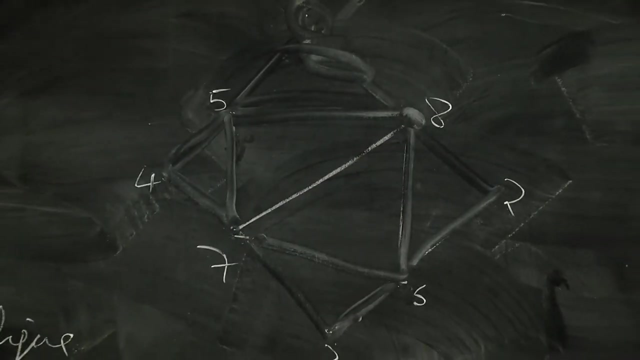 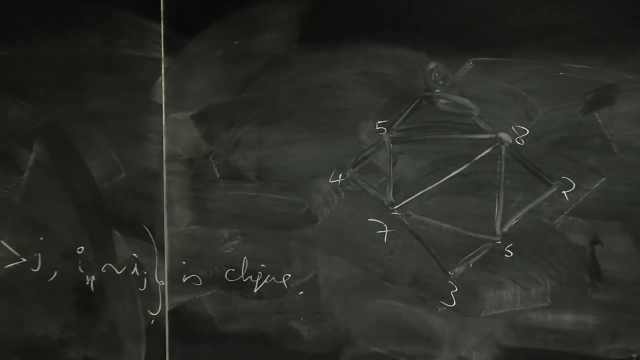 So, So, So, So so for every j I k. 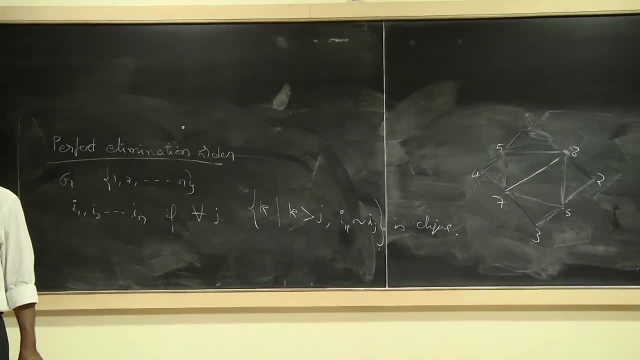 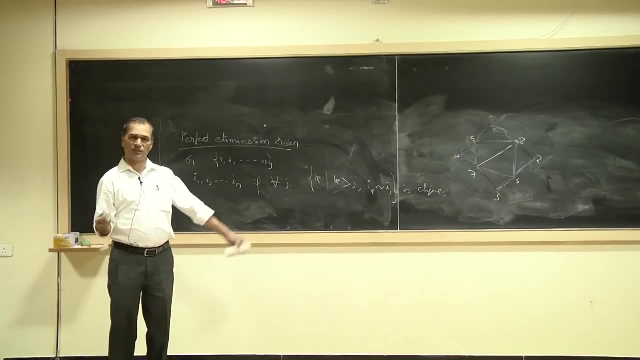 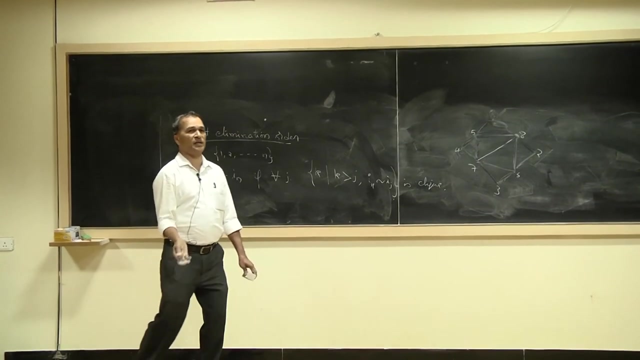 where k greater than j and I k adjacent to I, j should induce a clique. It is a clique in the sense that it induces a complete graph. different definitions of clique. this is one definition. clique is the subset of vertex set which induces a complete graph, sometimes even complete graph. themselves are called cliques, right. 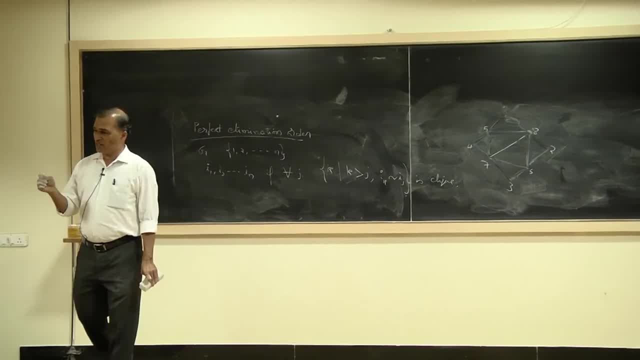 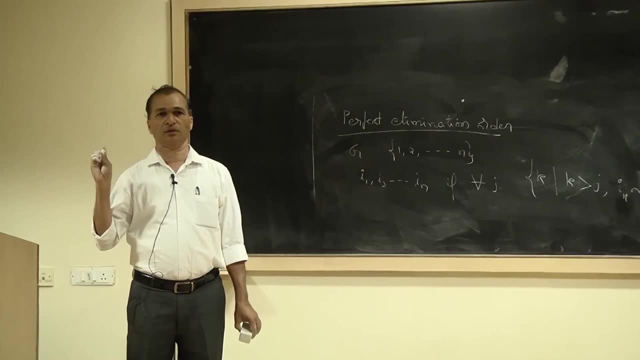 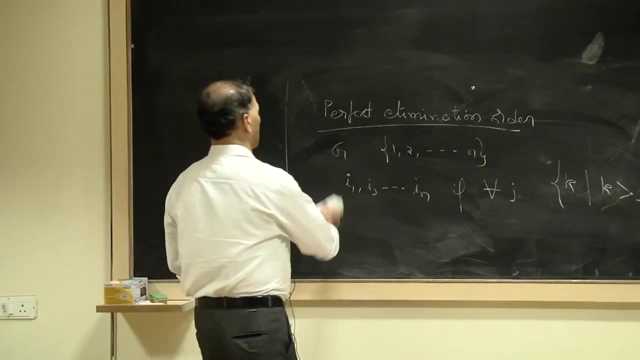 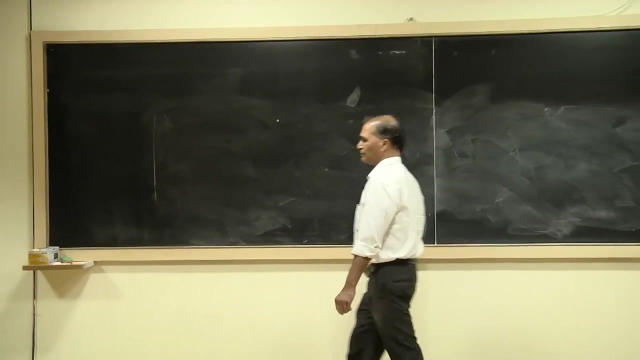 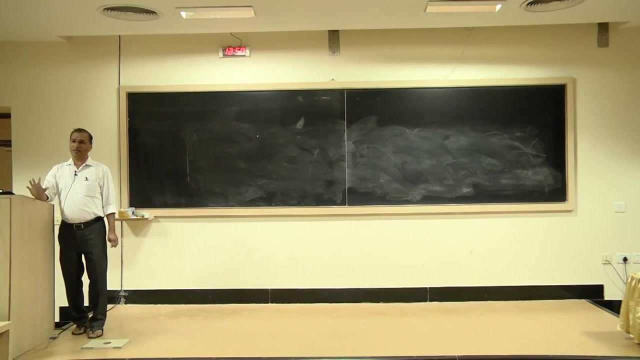 So this is a perfect elimination order, and there is a theorem which says that a graph is caudal if, and only if, it has a perfect elimination order or elimination sequence right. These are the basic things which are required to do for graphs and matrices. 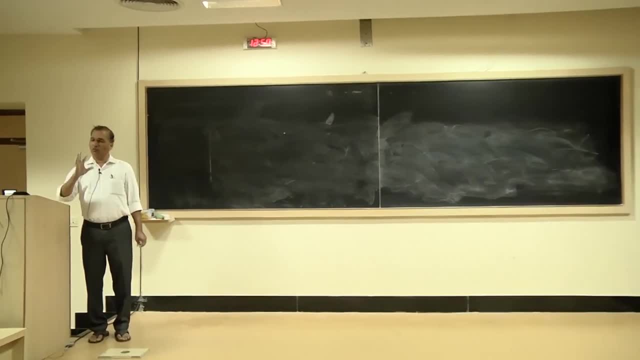 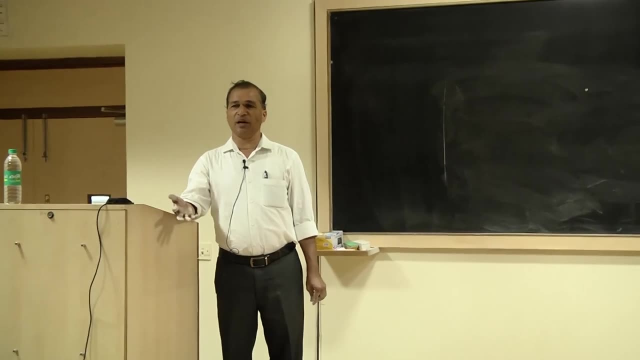 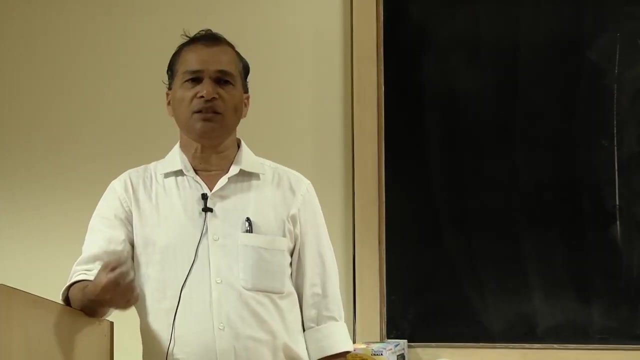 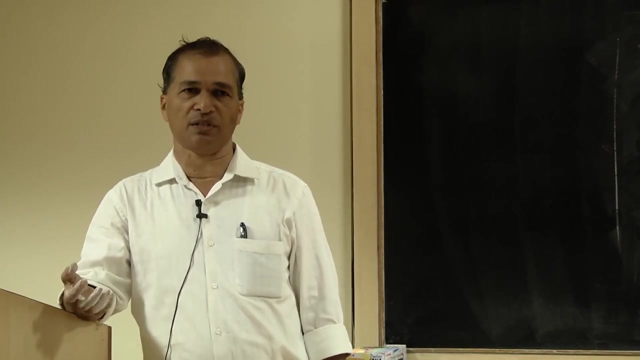 In the next this one, almost every such concept, whatever we have defined here, can be extended using the matrices right. The basic strength of graph theory is that the graphs can be represented in computers, So we can do the computations If we take a graph. 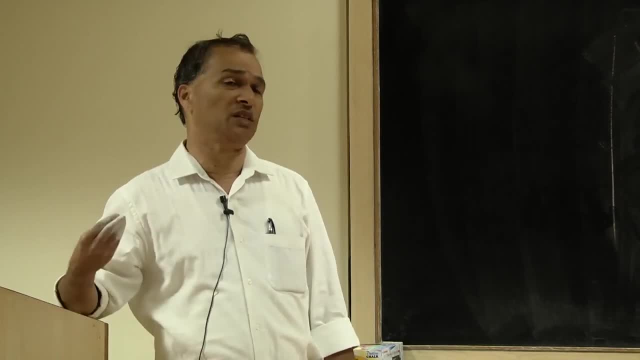 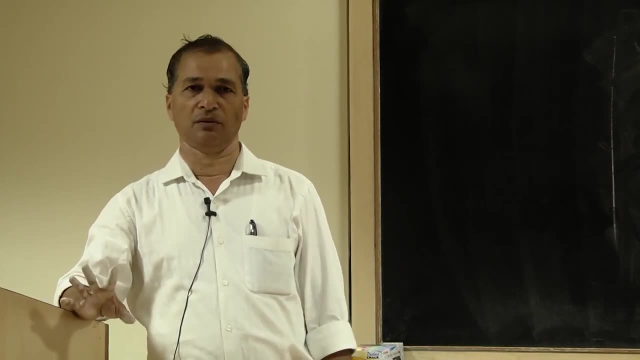 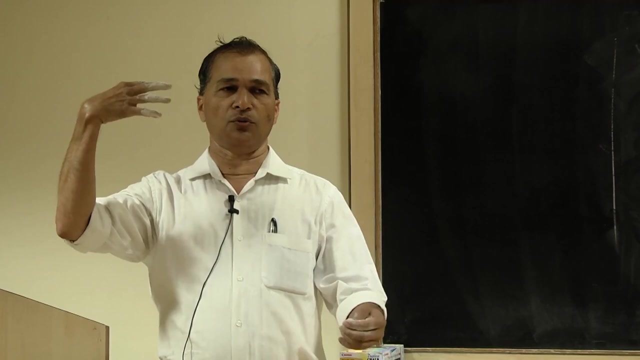 Graphs with very small number of vertices and very small number of edges. we can do the computations without using any computer. If you take a computer with, if you get take a graph with 100 vertices and 200 edges, and even if you want to find out the length of the shortest path between- I mean distance- 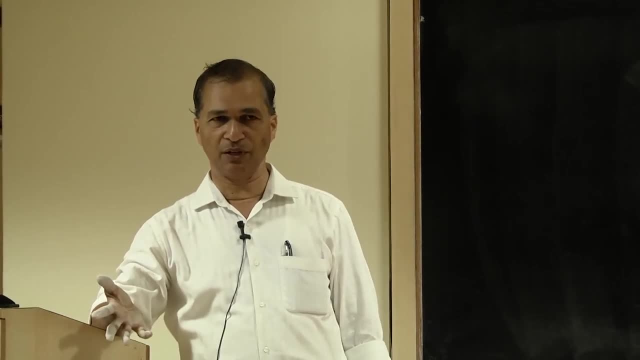 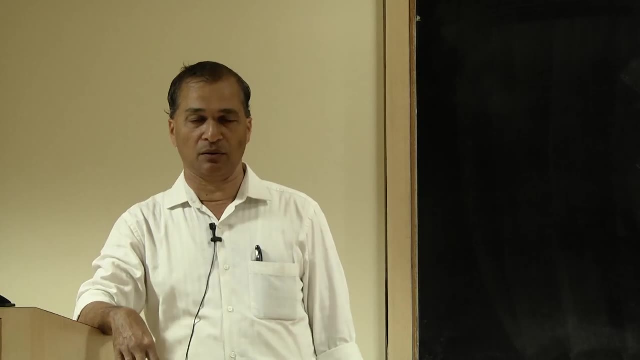 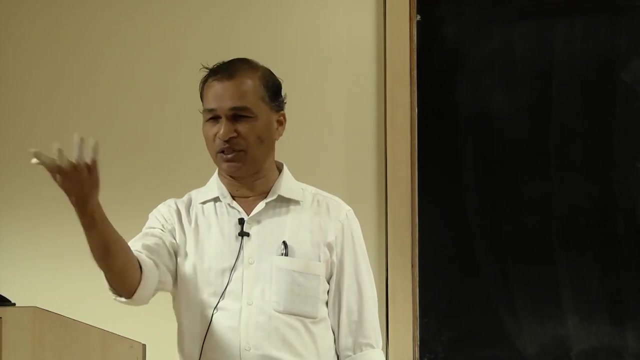 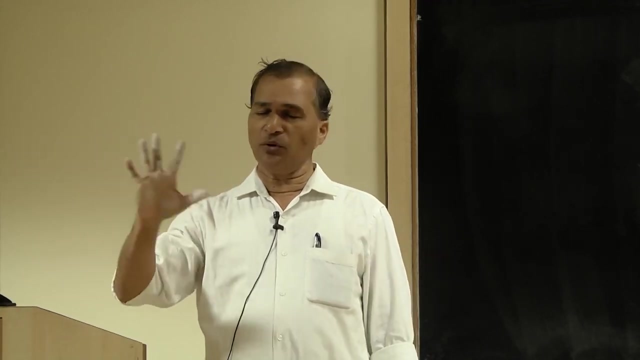 between two vertices. it is almost impossible, right? Suppose that we want to construct a Network with some 400 vertices, maybe some 4000 or 400 nc to 400 c, to that many edges can be there, some very number of odd number of edges, and we want to see to it that any 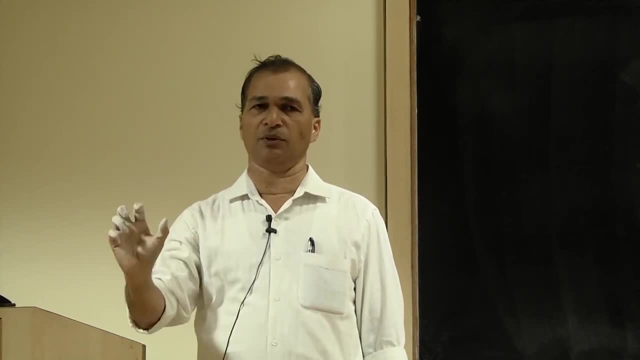 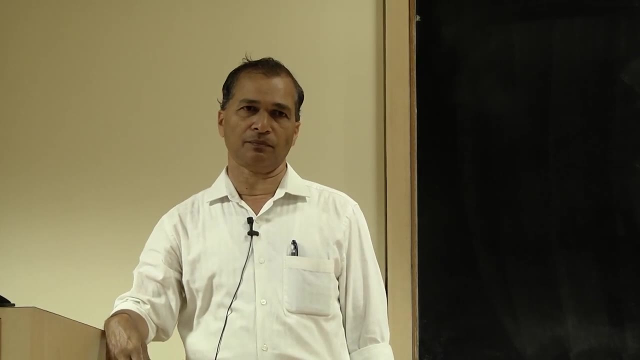 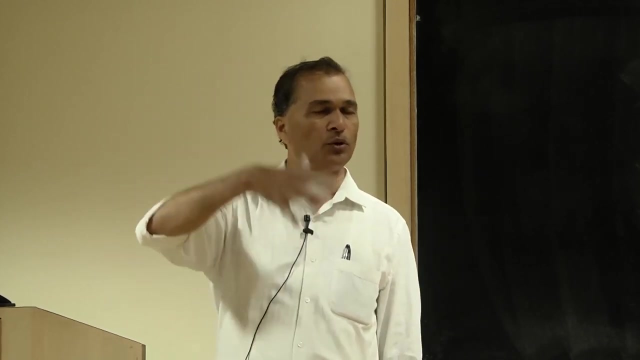 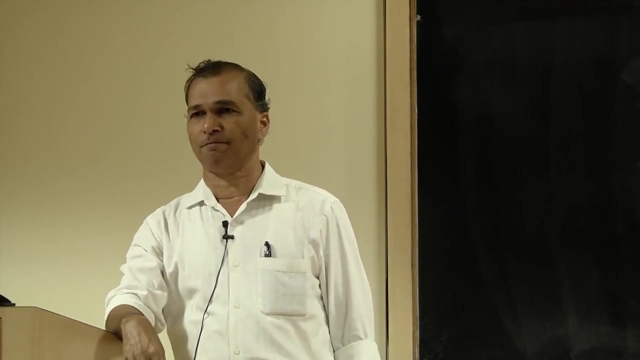 two vertices, any two nodes in the network. the distance between them should not be greater than 30.. Right The hop count. if you say the hop count to reach from one node to another node should not be greater than three, it should be either one or two or three. how will you do it? 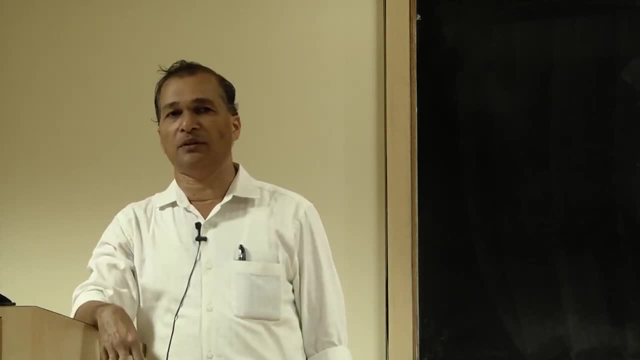 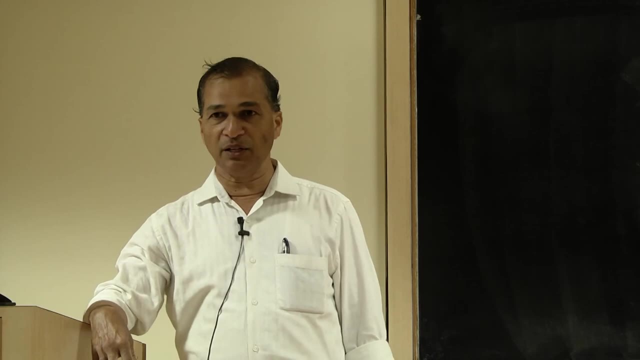 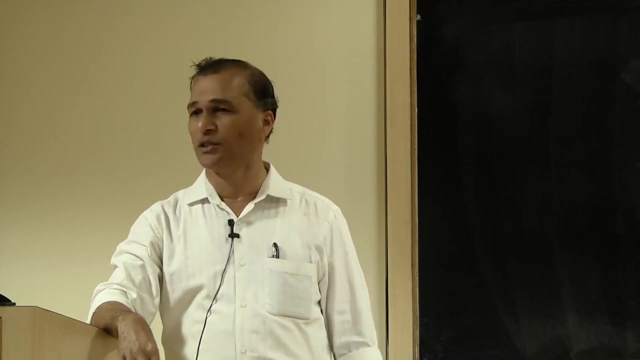 How can we do it with that many, very some. two to the power of n vertices. two to the power of n is possible. N can be anything. two to the power of n vertices, are there any number of edges? may not be exactly any number of vertices. it is two to the power of nc to by two that many edges suppose that. 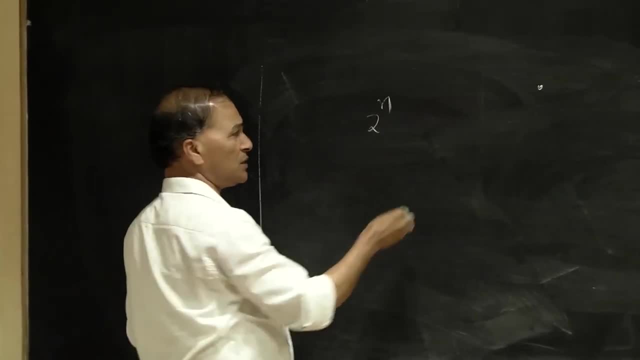 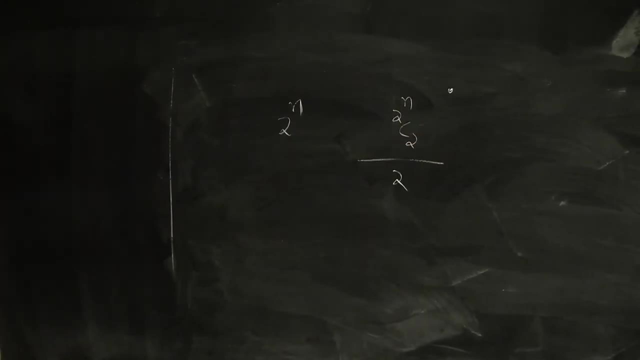 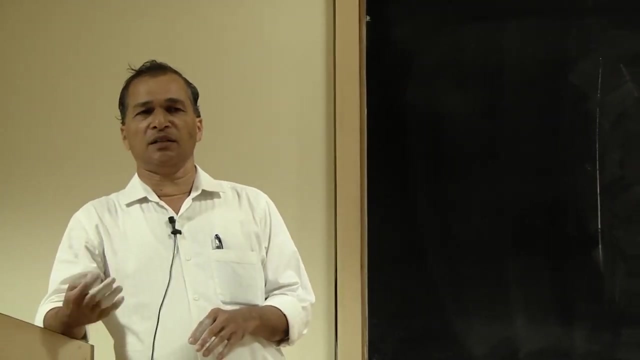 we have a network with two to the power of number of n vertices and two to the power of n c to divided by two edges. these many edges are there and we want to see to it that no two vertices Right. No two vertices Right. 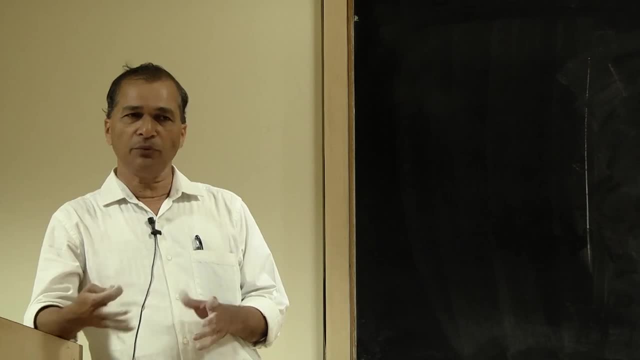 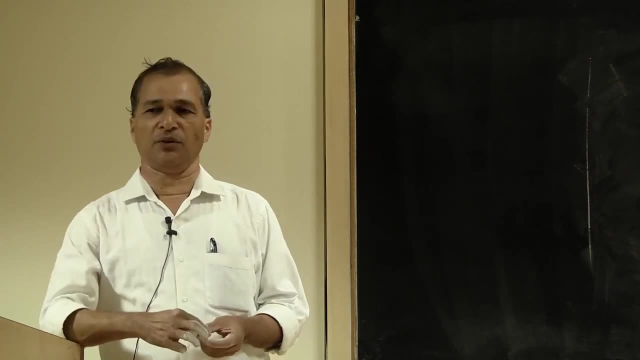 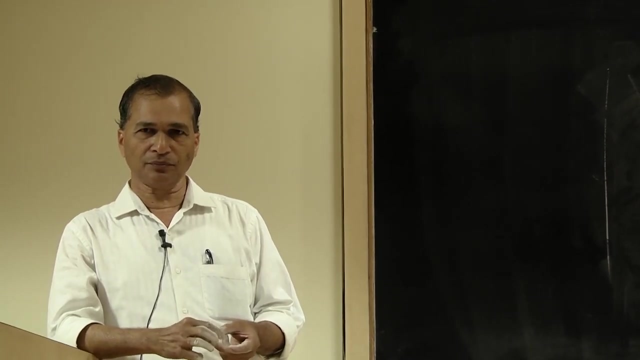 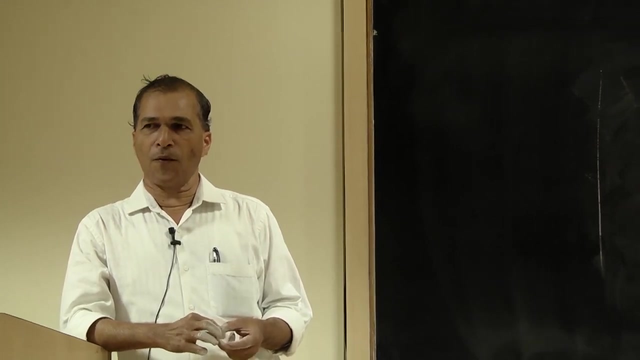 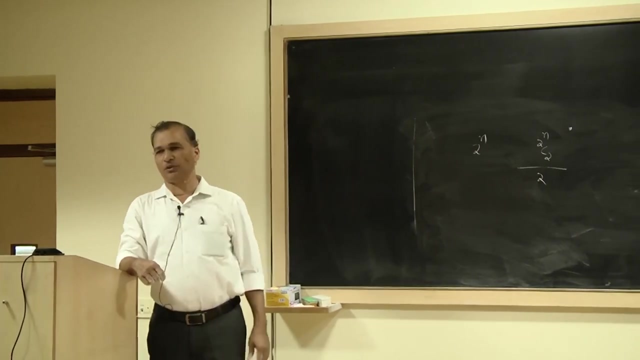 Two vertices are at distance greater than three. can we do it? if at all we can do. how to do it? it is one simple property of graph theory. one possibility is that two to the power of n vertices Right. Two of them are adjacent, but there will be two to the power of n c, two edges. we do not. 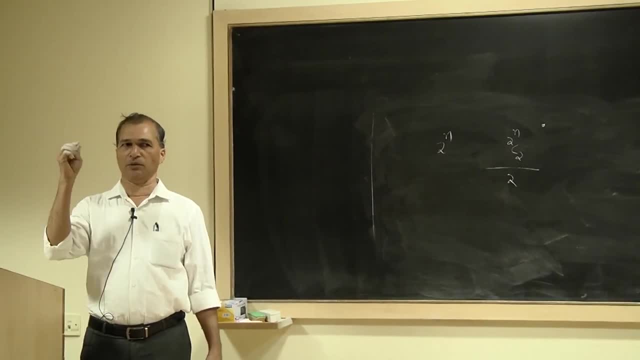 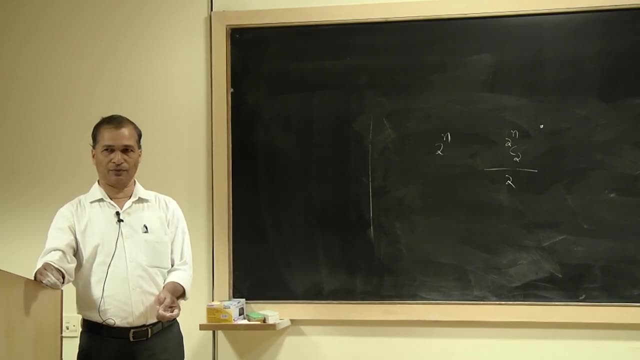 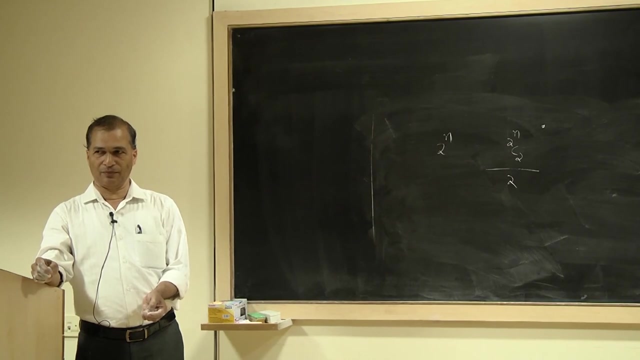 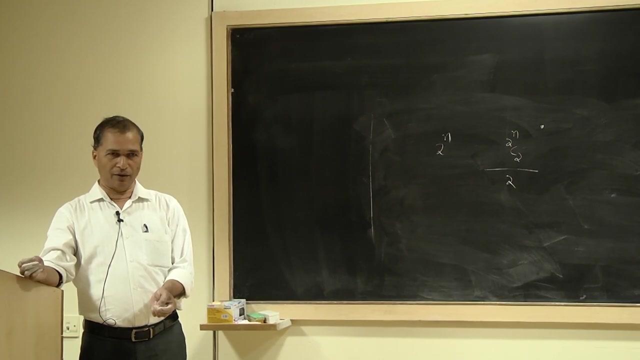 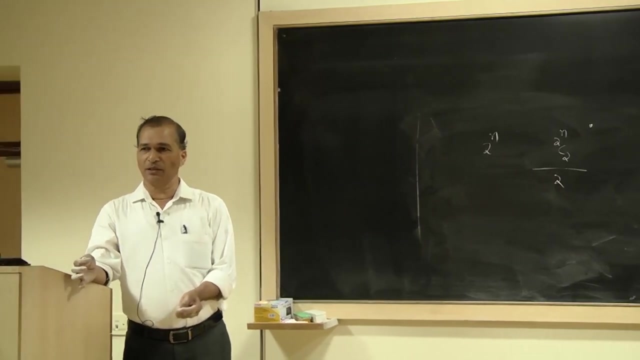 want to have that many edges. we want to have two to the power of n, c, two divided by two edges. that, divided by two edges, should tell you what we have to do. Right, It makes use of the fact that, Right, Every self complementary graph is of diameter either two or three. is it not every self complementary?